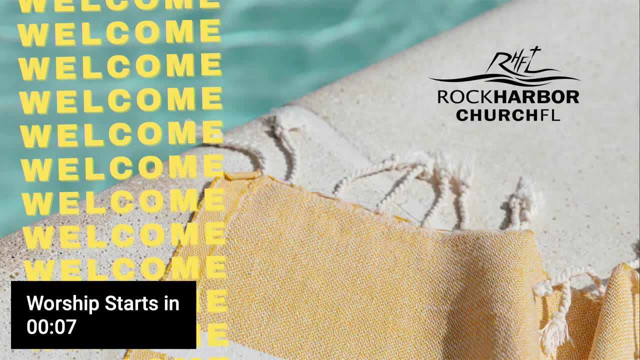 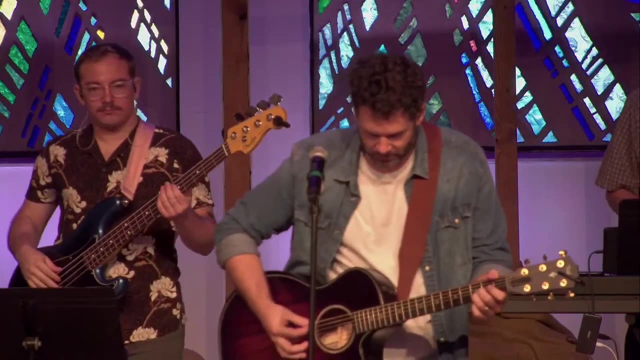 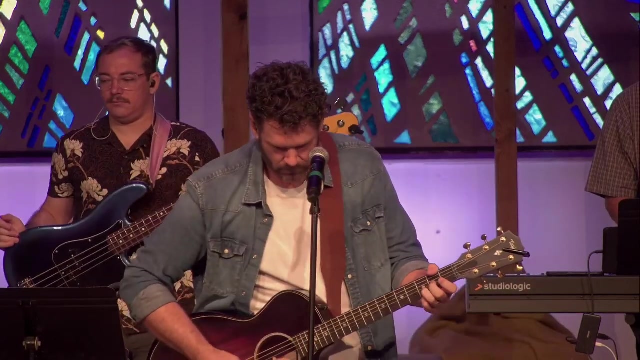 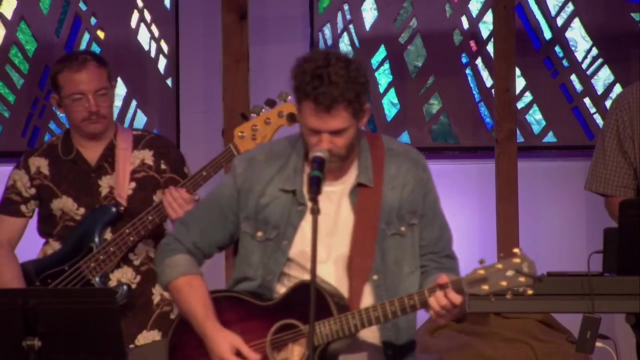 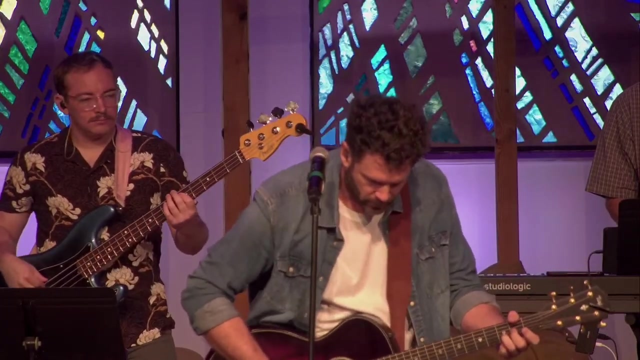 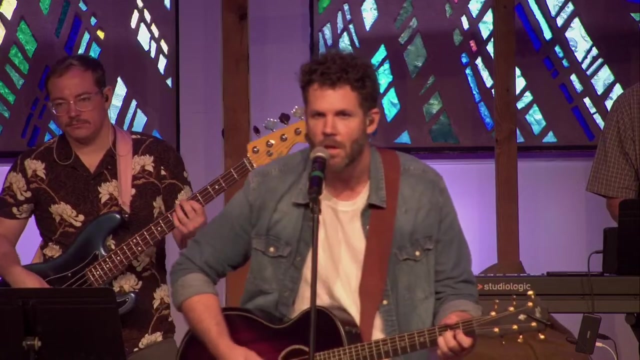 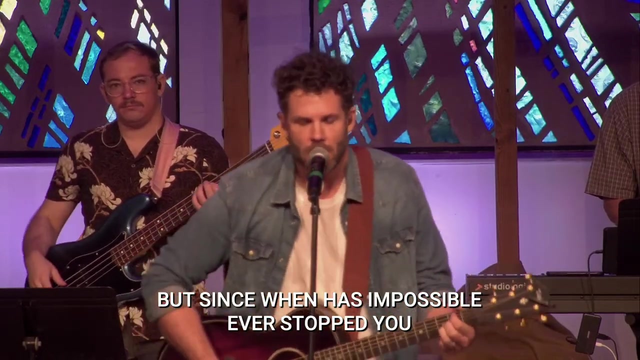 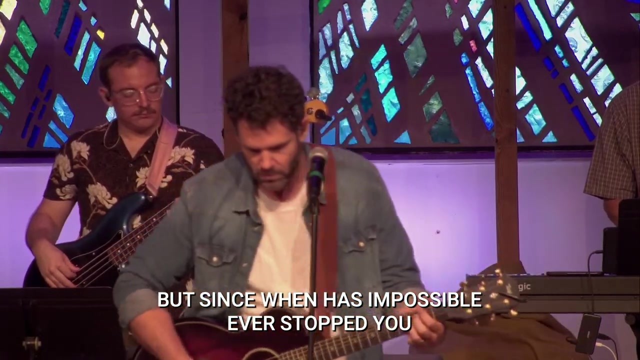 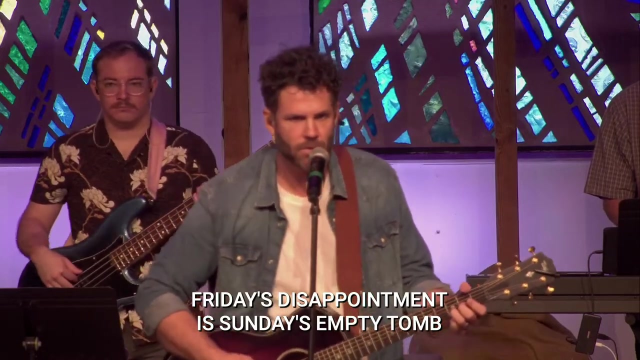 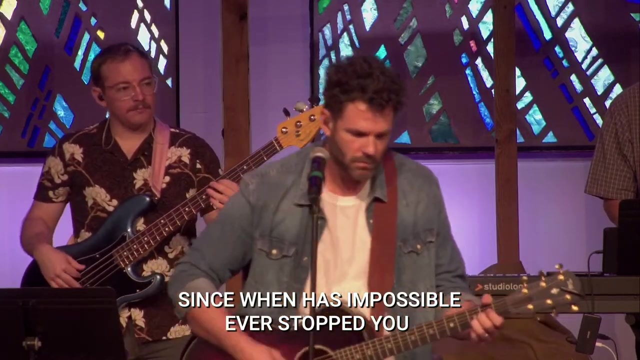 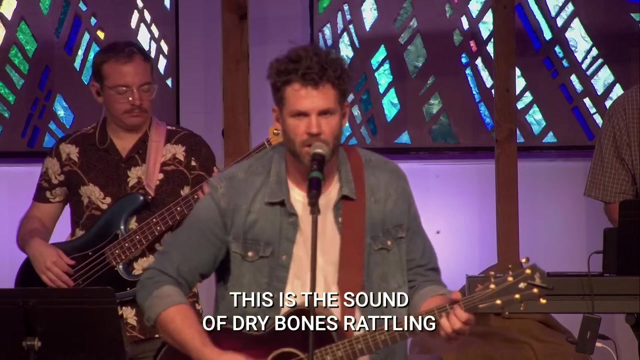 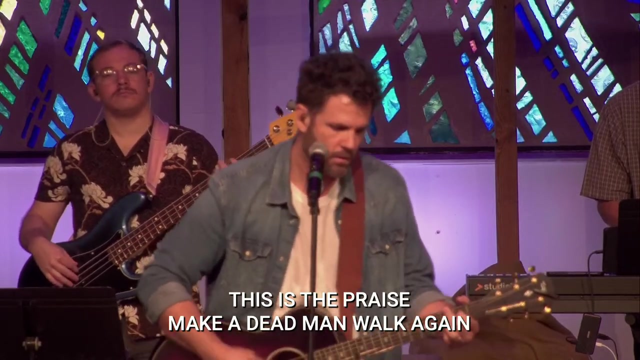 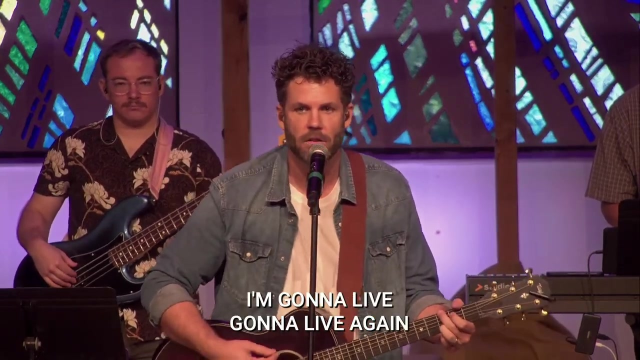 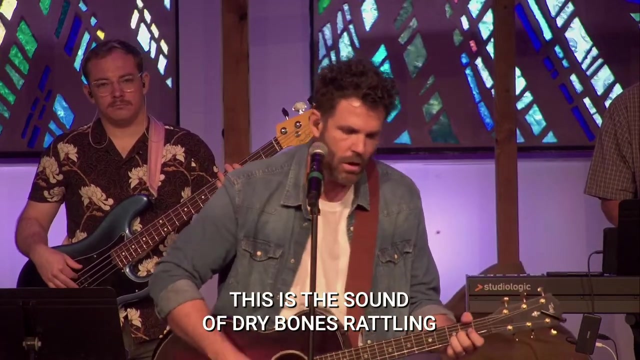 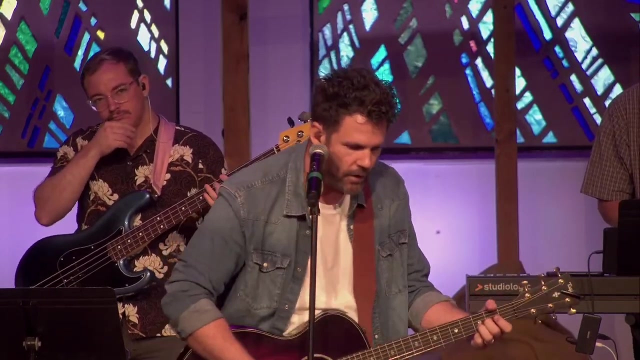 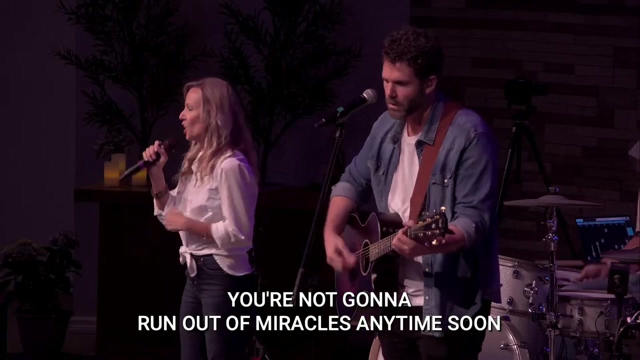 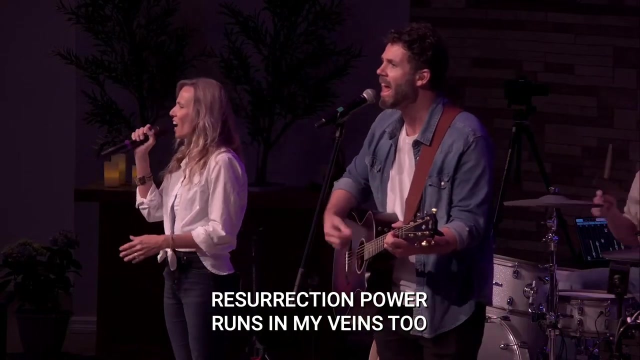 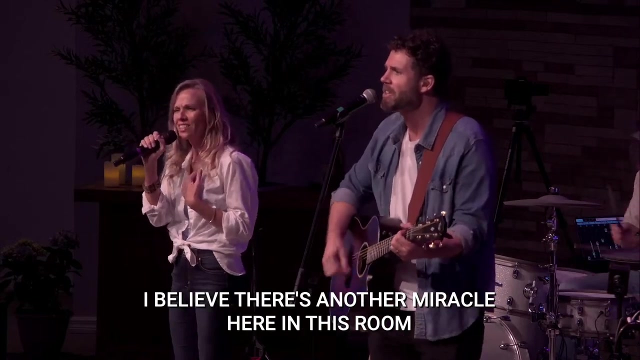 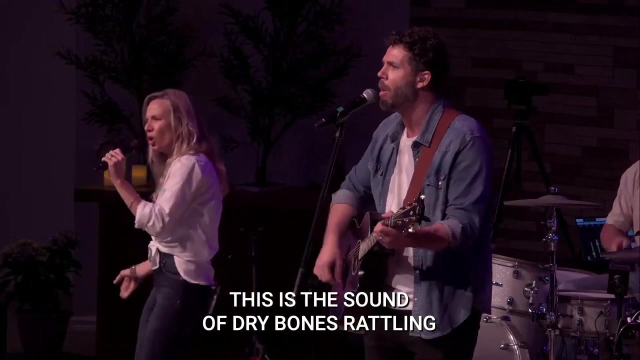 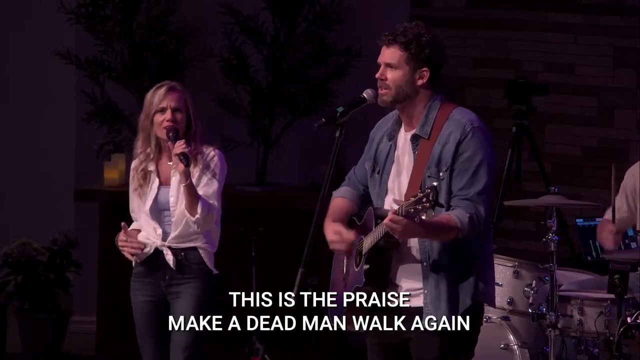 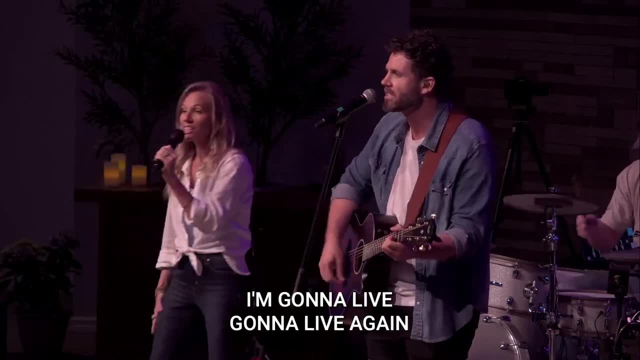 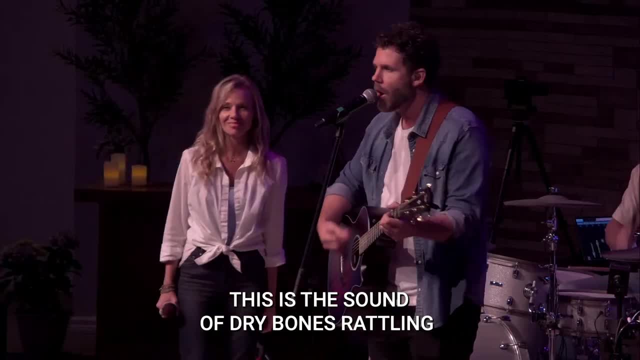 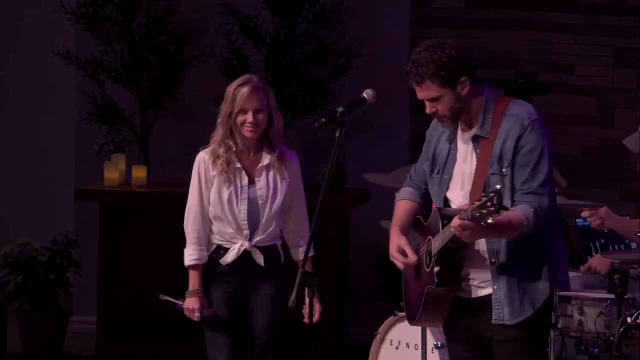 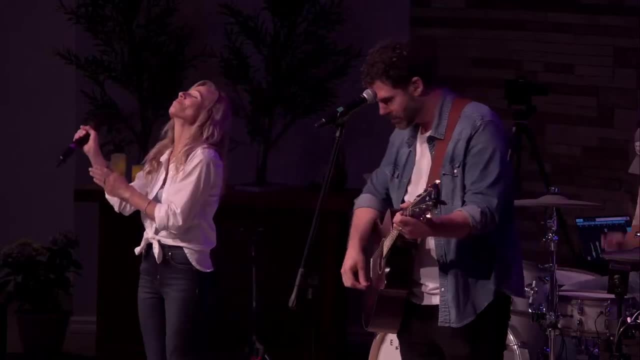 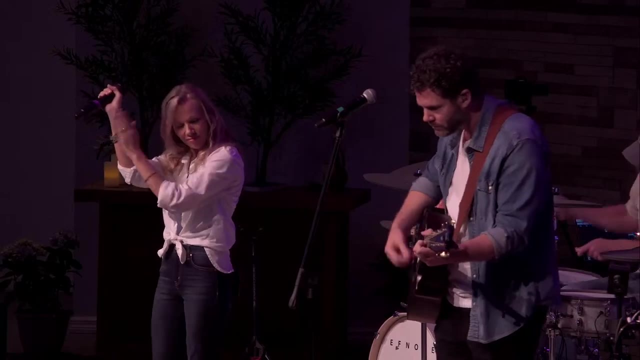 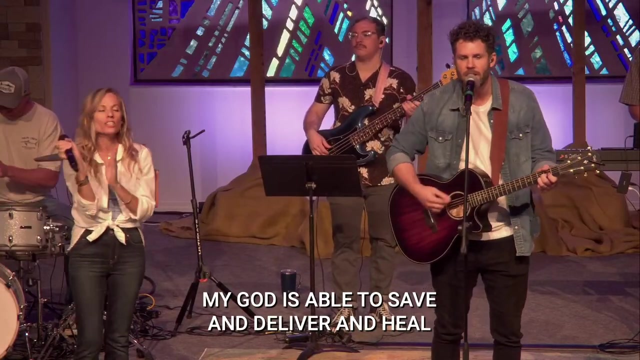 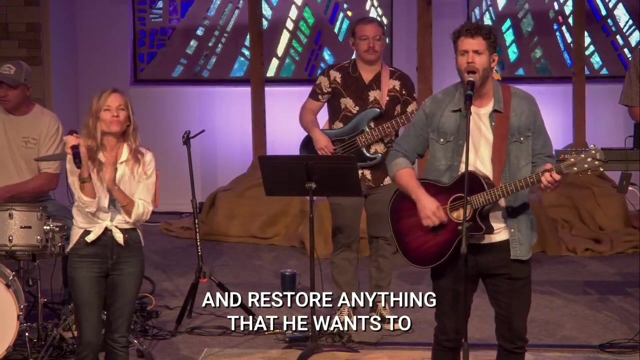 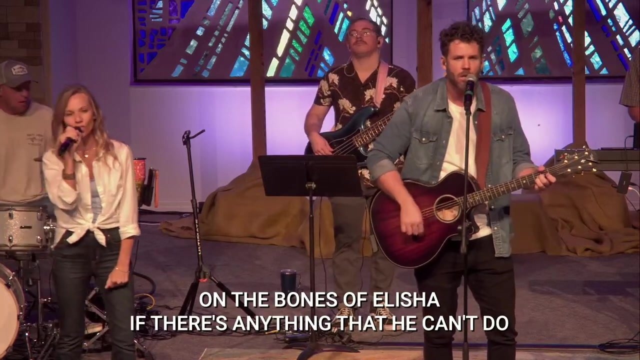 Let's stand on our feet and worship this morning. Let's stand on our feet and worship this morning. My God is able to save and deliver and heal And restore anything that He wants to. Just ask the man who was thrown on the bones of Elijah. 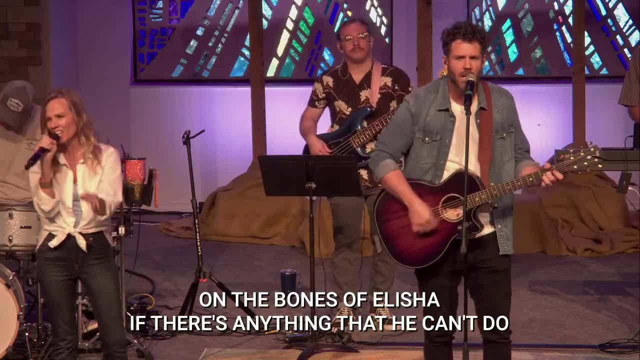 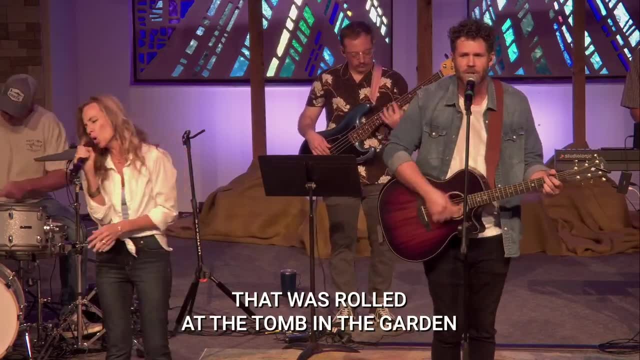 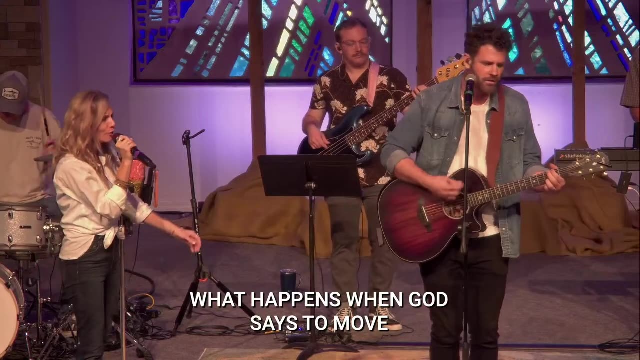 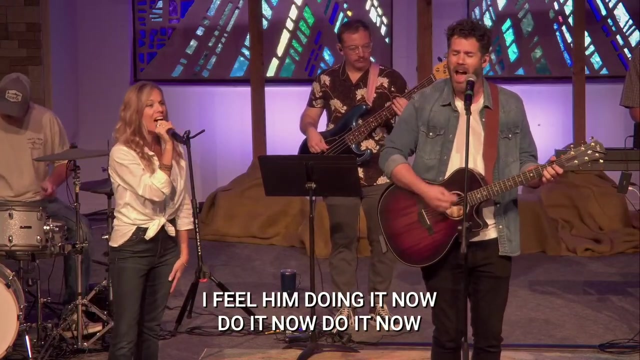 If there's anything that he can do, Just ask the stone that was rolled at the tomb in the garden. What happens when God says to go? I feel it moving, and now I feel it moving, and now I feel it moving, and now I feel Him doing it now. 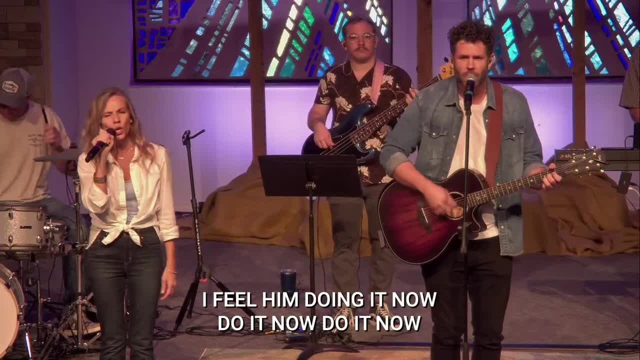 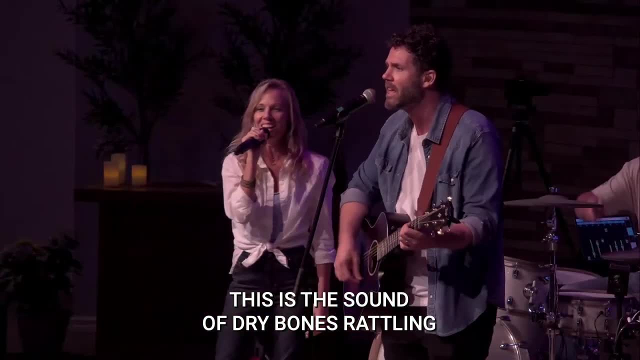 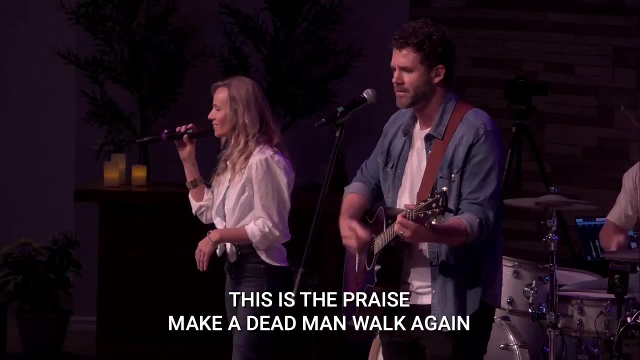 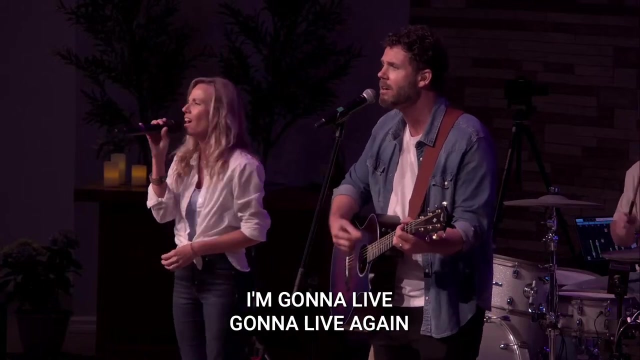 I feel Him doing it now. Doing now, doing now. This is the sound of dry bones rattling. This is the grace making dead men walk again. Open the grave. I'm coming up. I'm gonna live, gonna live again. Open the grave. I'm coming up. 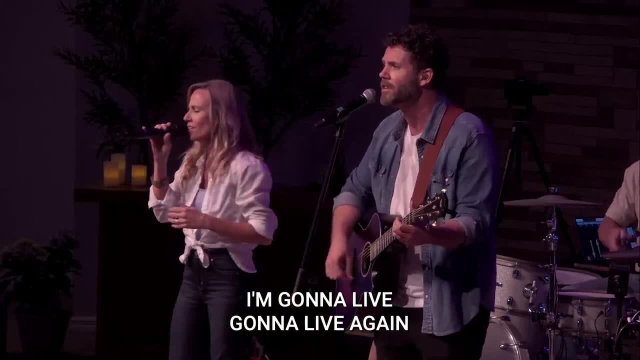 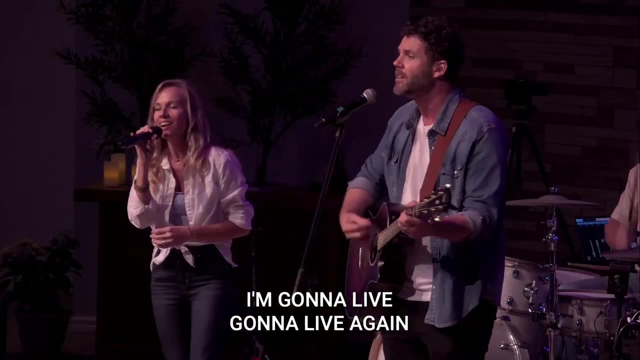 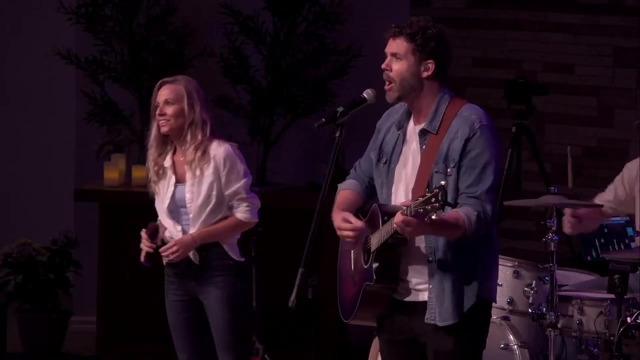 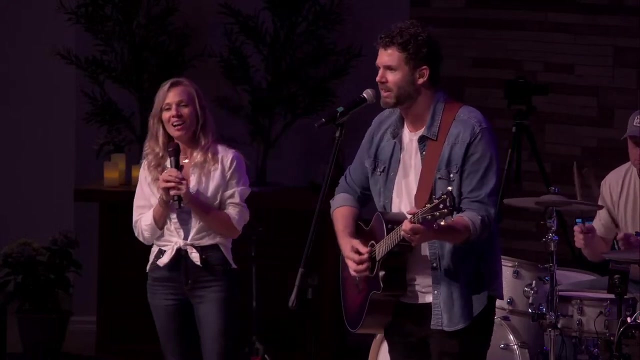 I'm coming up, I'm gonna live, gonna live again. Open the grave. I'm coming up, I'm gonna live, gonna live again. This is the sound of dry bones rattling Right on, right on. Let's hear it for Him in this place. 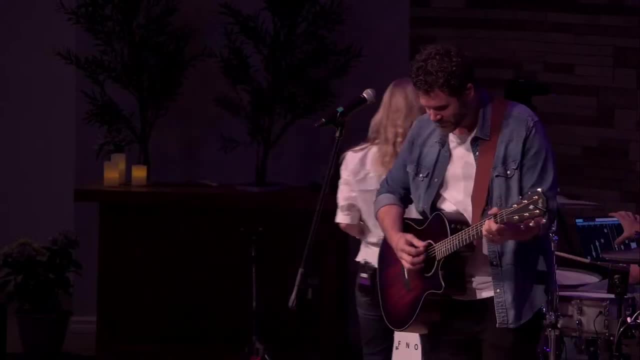 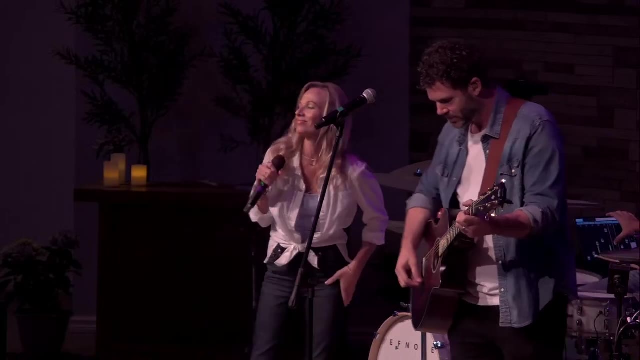 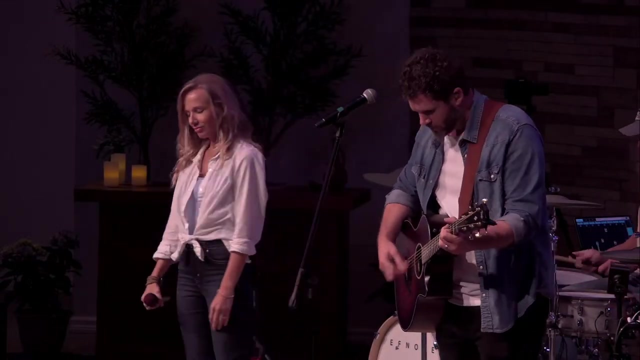 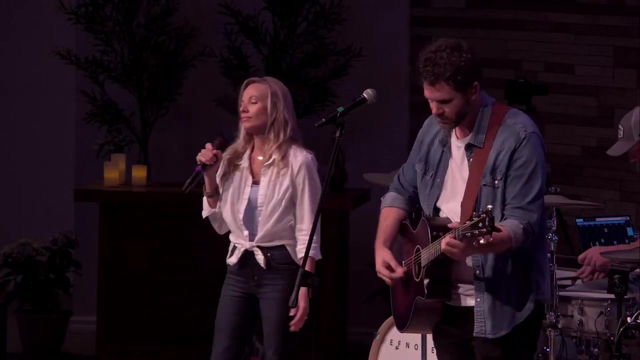 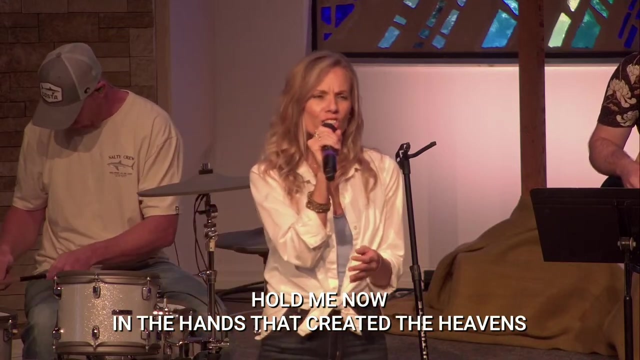 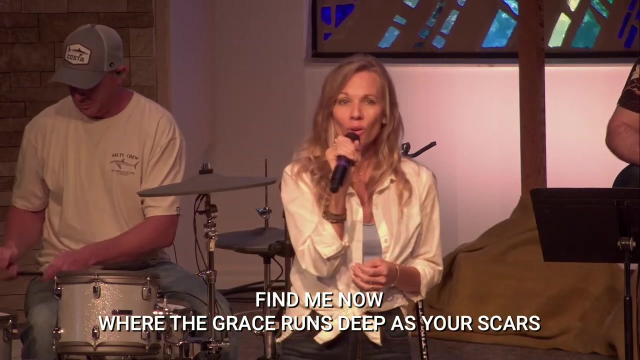 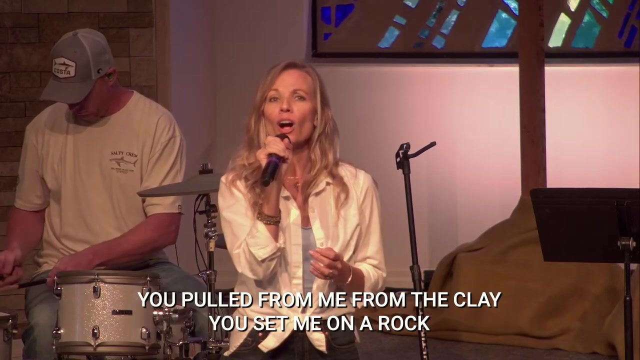 Amen, amen, woo, Which I had to worship the risen King this morning. Hold me now In the hands that created the heavens, The hands that created the heavens. Find me now Where the grace winds as deep as your scars. You pulled me from the clay, You set me on a rock. 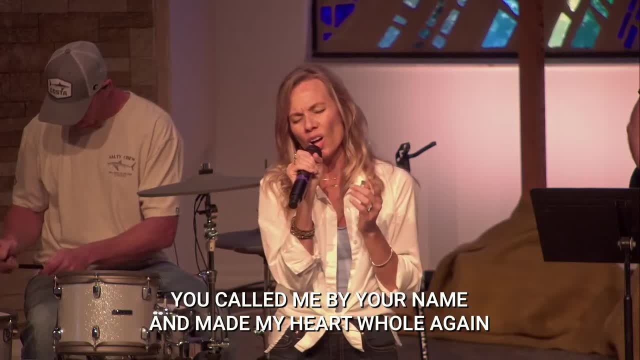 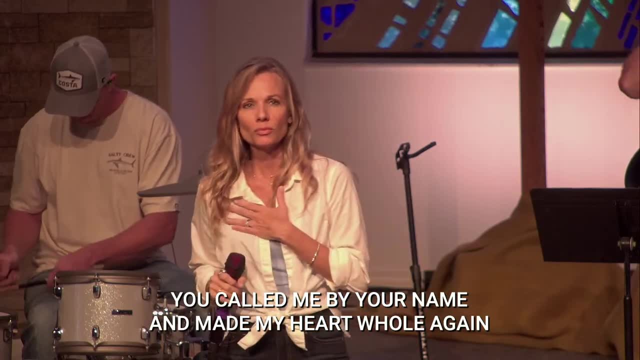 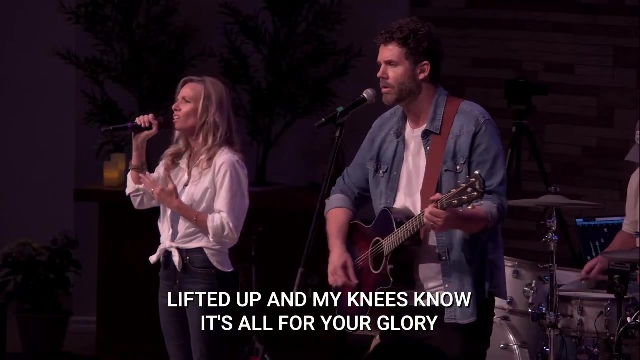 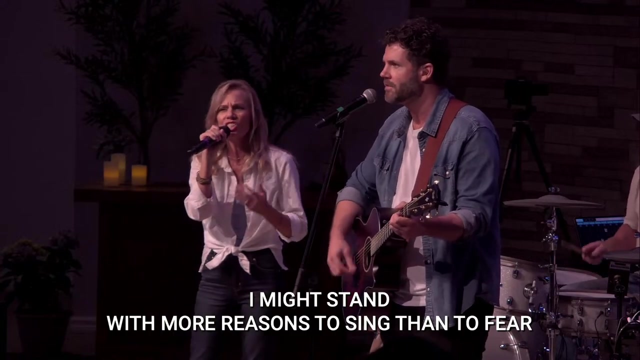 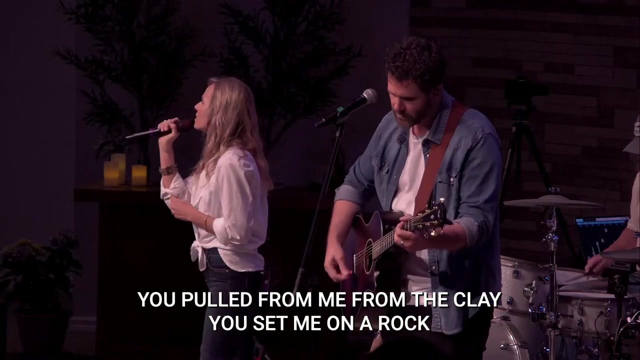 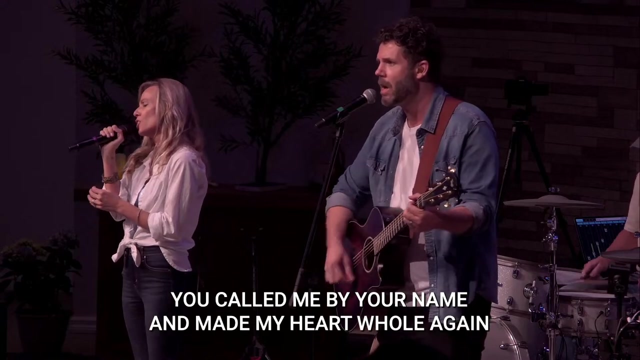 You called me by your name, Made my heart whole again Lifted up and my knees low. It's all for your glory That I might stand With more reasons to sing than to fear. You pulled me from the clay. You set me on a rock. You called me by your name. 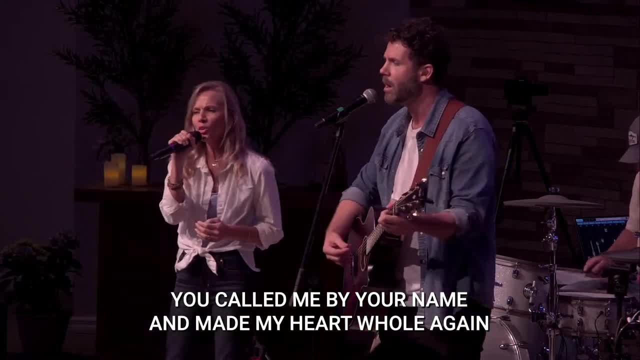 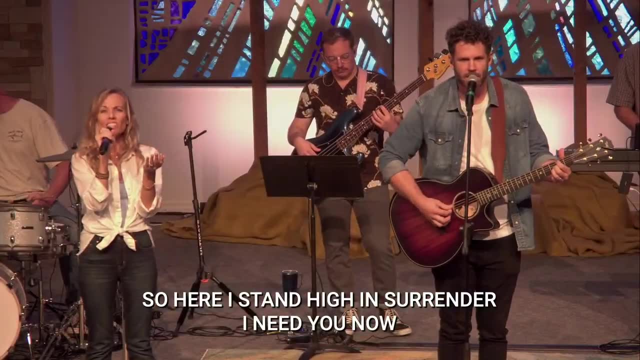 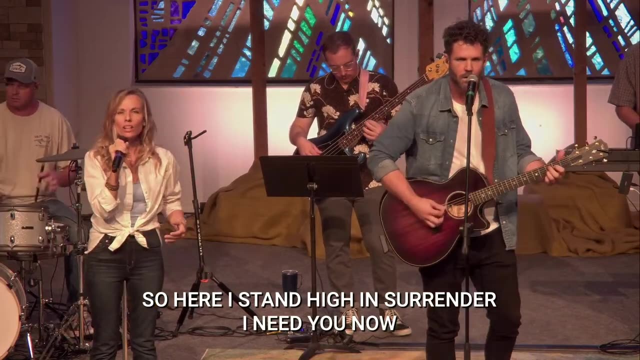 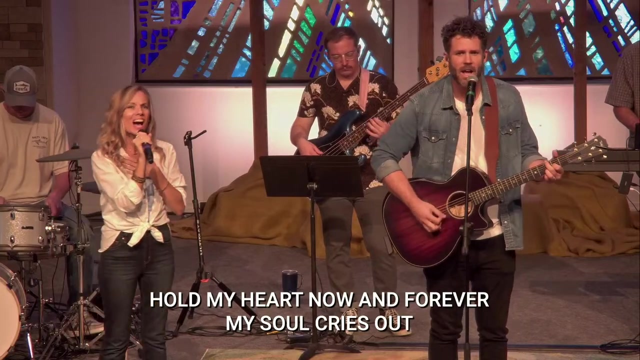 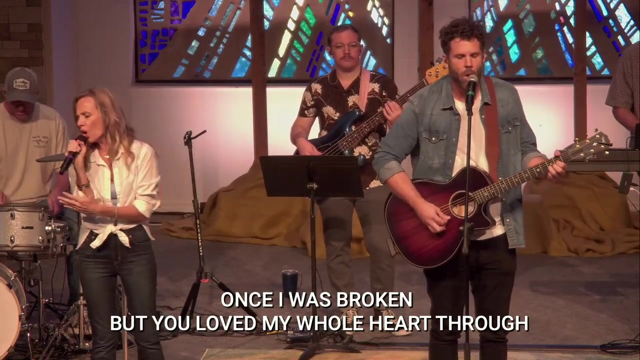 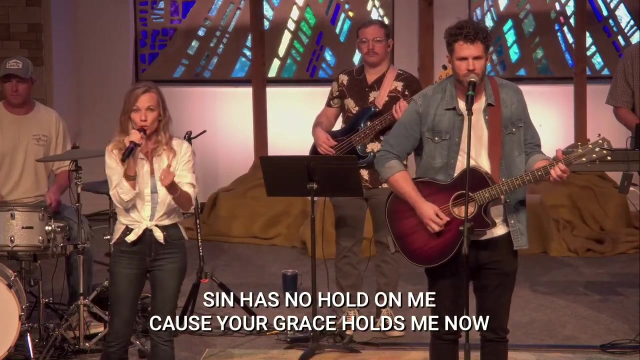 Made my heart whole again. Here I stand, High in surrender. I need you now. Hold my heart Now and forever. My soul cries out As I was broken And you made me whole. You loved my whole heart. full Sin had no hold on me, But your grace holds me now. 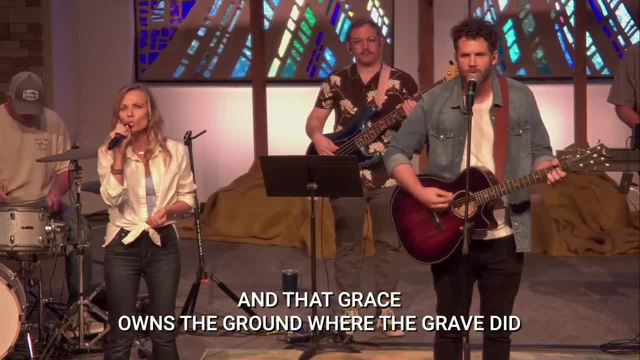 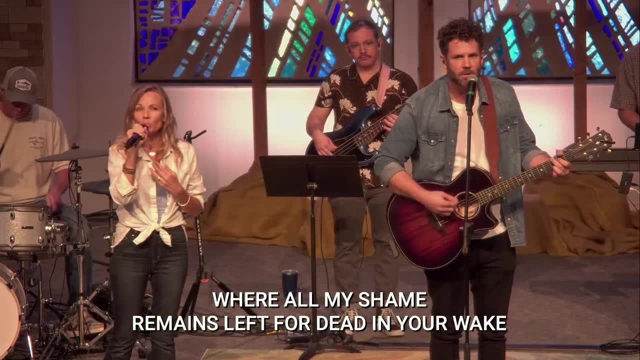 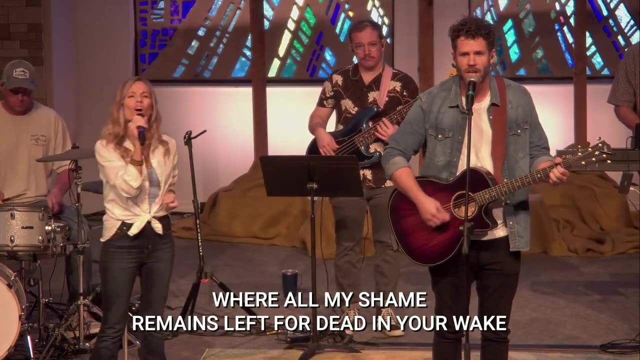 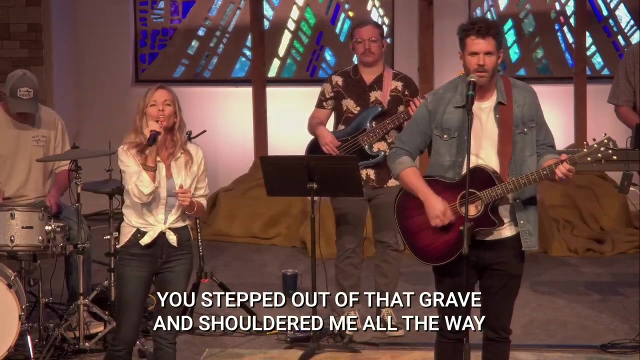 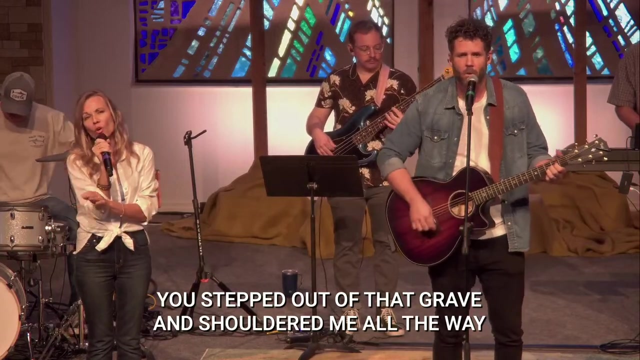 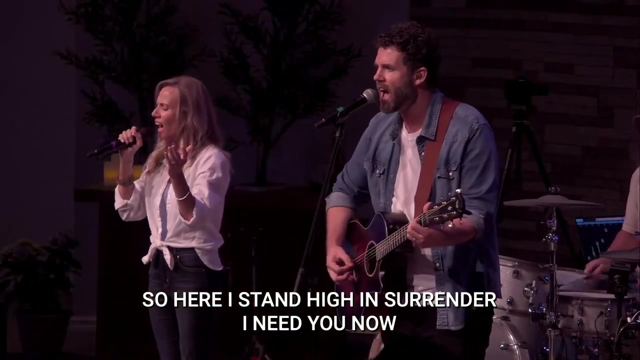 And that grace Owns the ground where the grave did, Where all my shame remains, Left for dead in your wake. Whoo, You crushed those empty gates, Left for stone unturned. You stepped out of the grave, Showed me all the way You're insane. Here I stand. 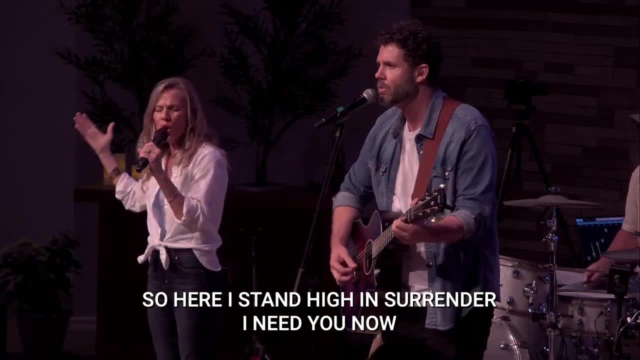 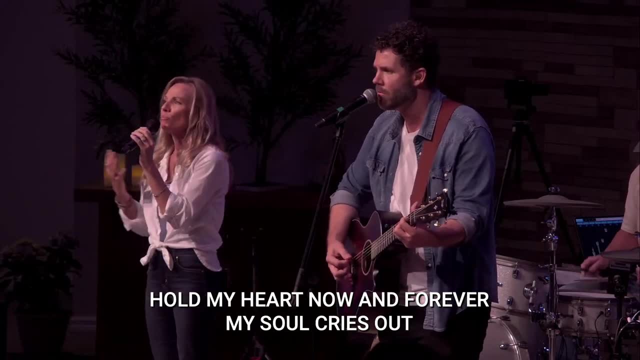 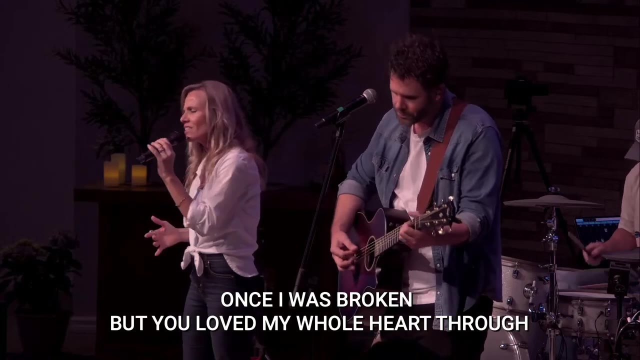 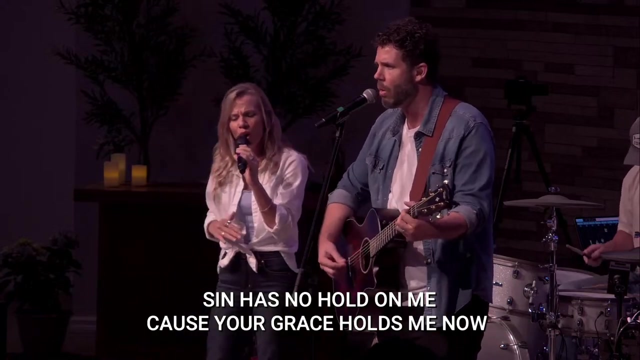 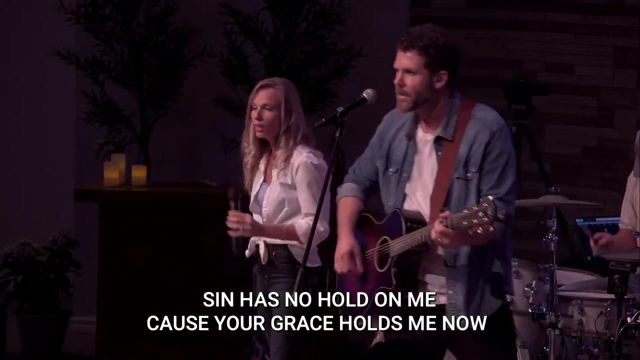 High in surrender. I need you now. You're insane. I need you now. Here I stand, Hold my heart Now and forever. My soul cries out As I was broken. You loved my whole heart. full Sin has no hold on me, But your grace holds me now Feeling forgiven. 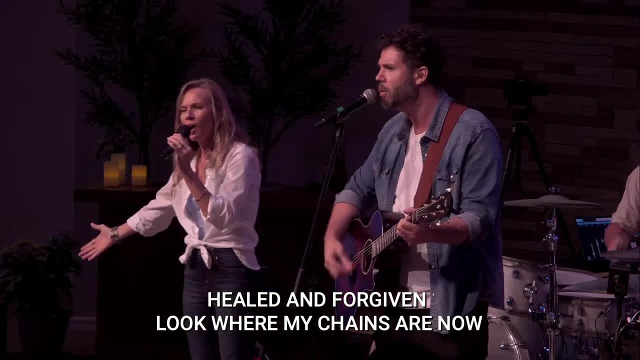 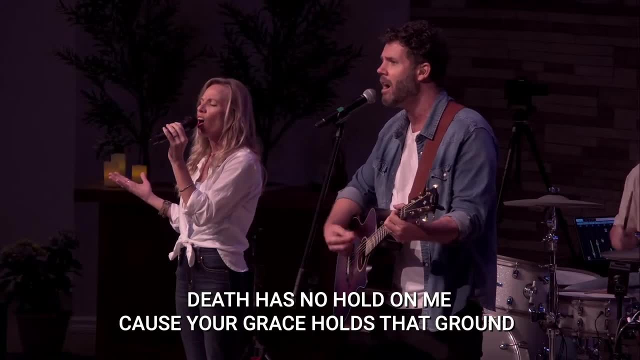 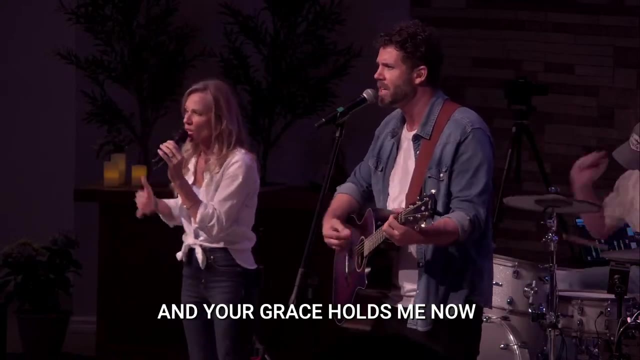 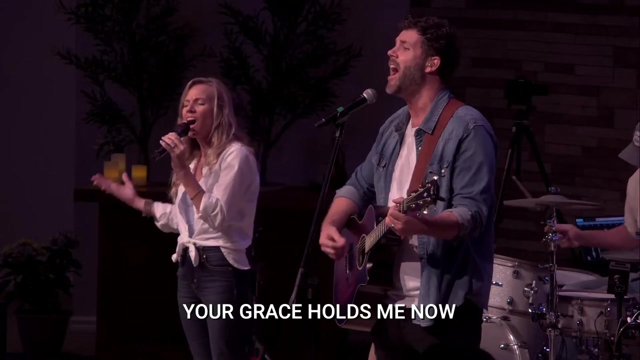 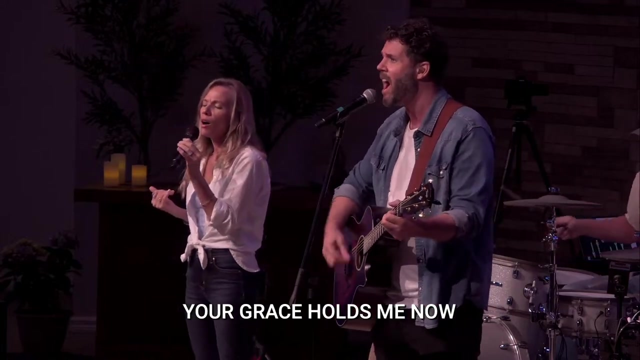 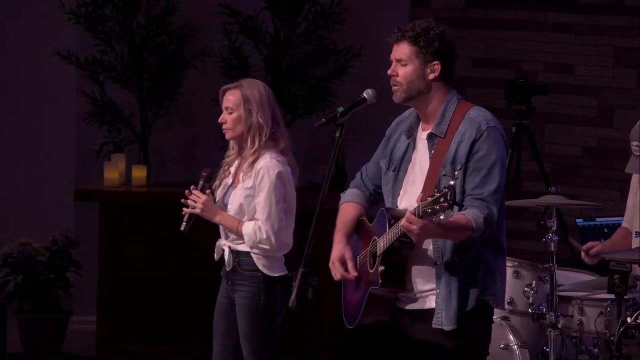 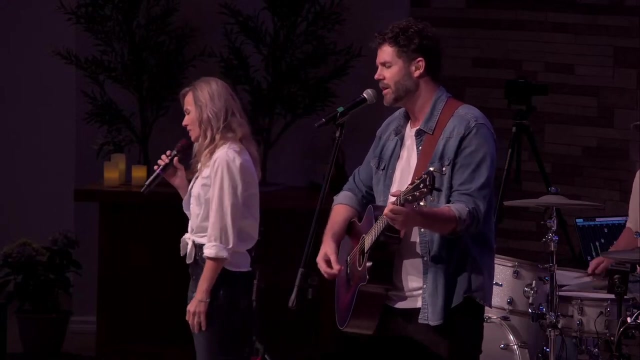 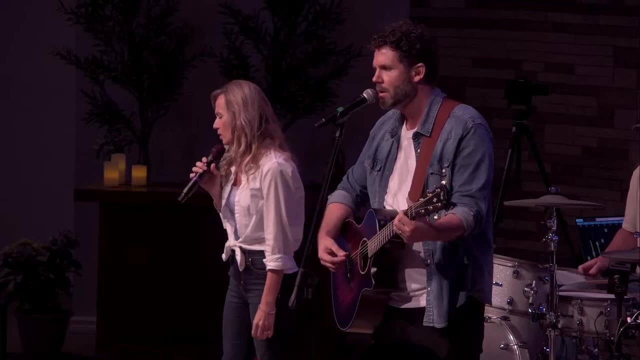 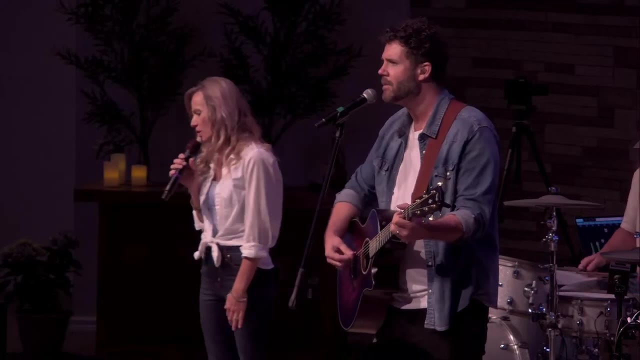 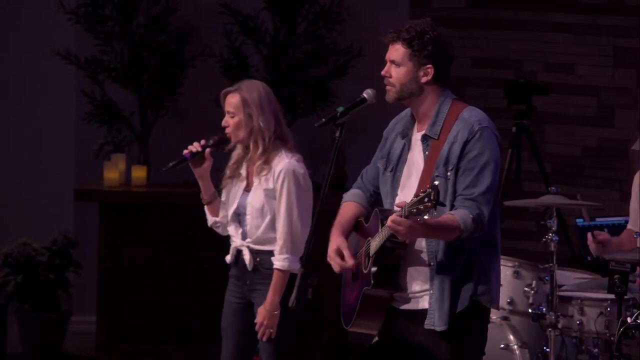 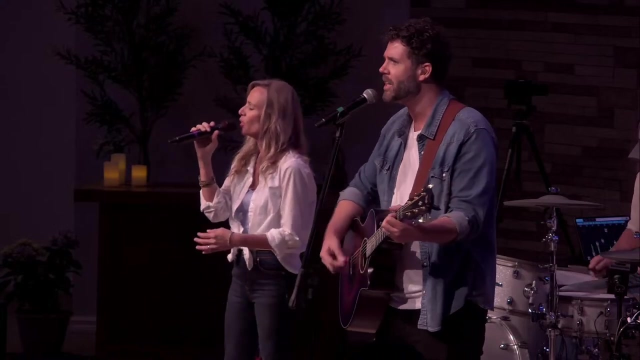 Amazing grace, how sweet the sound. Saved a wretch like me. Amazing grace, how sweet the sound. Amazing grace, how sweet the sound. I once was lost, but now I'm found, Was blind, but now I see. Amazing grace, how sweet the sound. 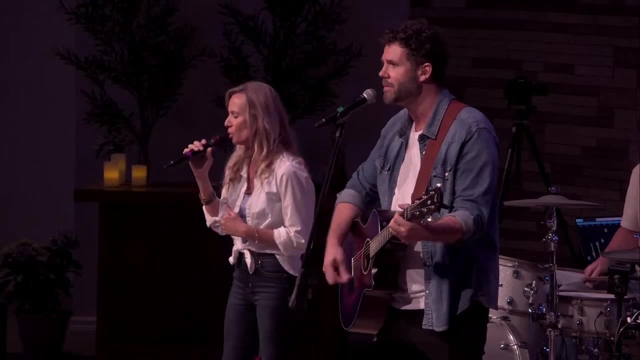 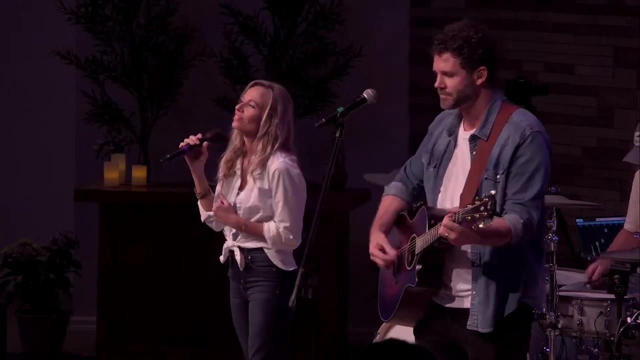 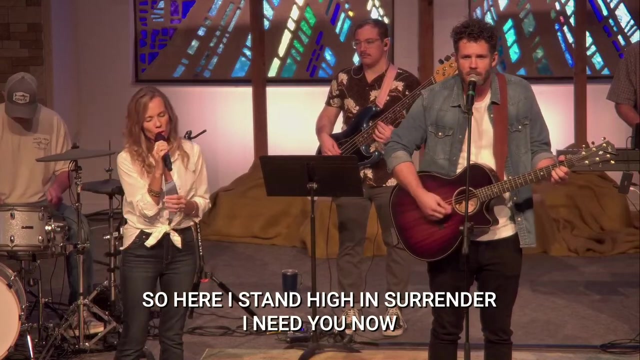 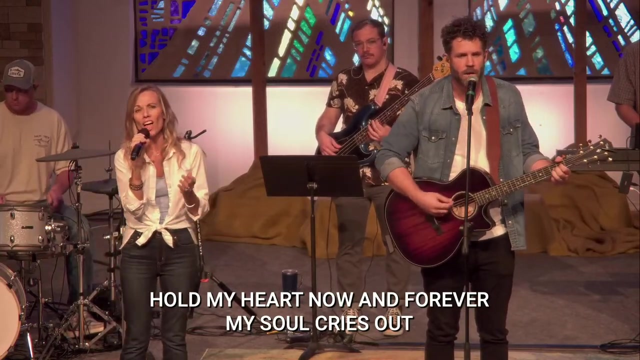 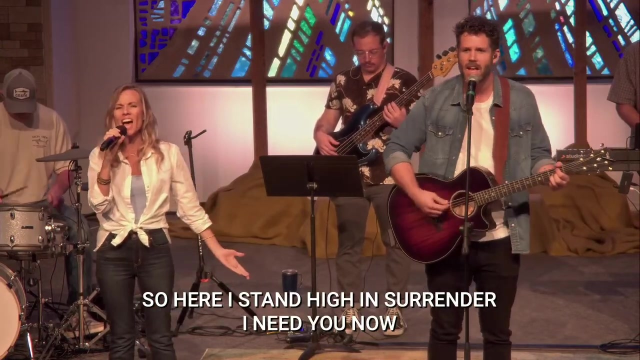 Saved a wretch like me. I once was lost, but now I'm found. Here I stand. So here I stand, High in surrender. I'm found. I need you now. Hold my heart Now and forever. My soul cries out. Let's sing that. Here I stand, High in surrender. 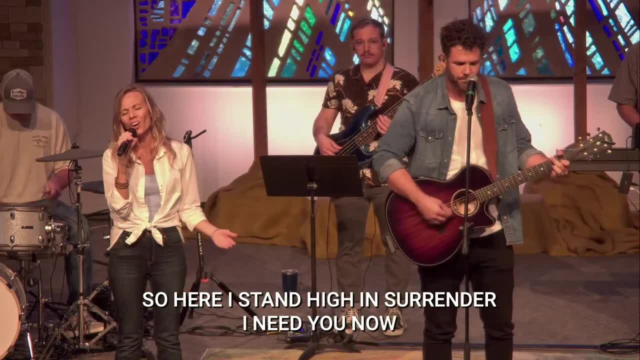 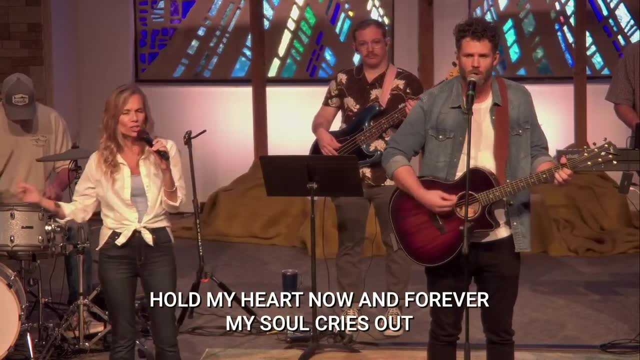 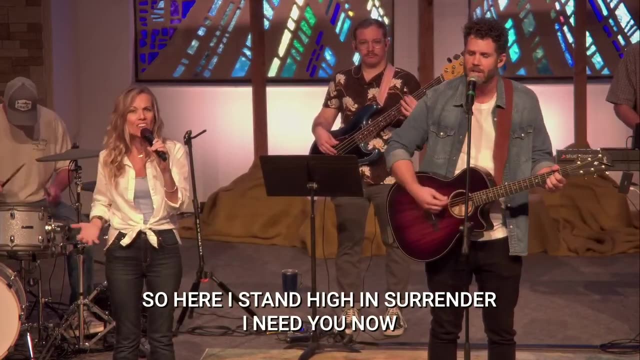 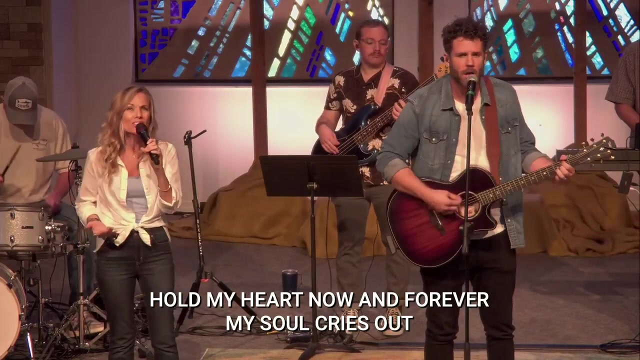 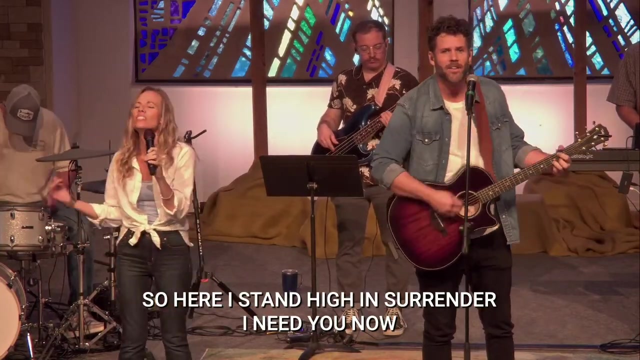 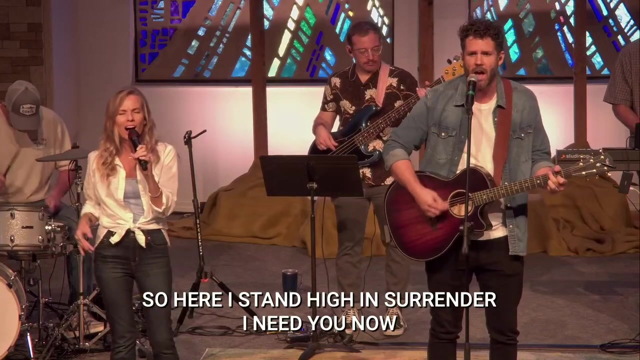 I need you now. Hold my heart Now and forever. My soul cries out: Here I stand High in surrender. I need you now. Here, I stand High in surrender. I need you now. Hold my heart Now and forever. My soul cries out: Here I stand High in surrender. I need you now. 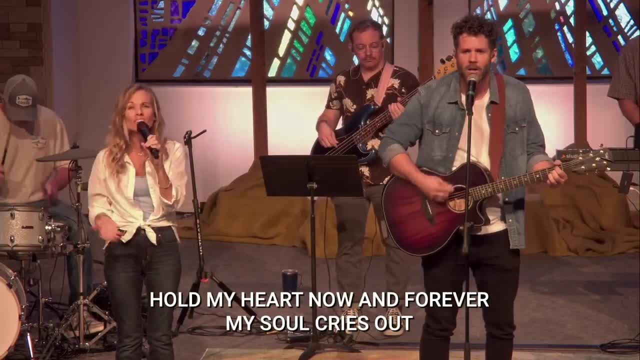 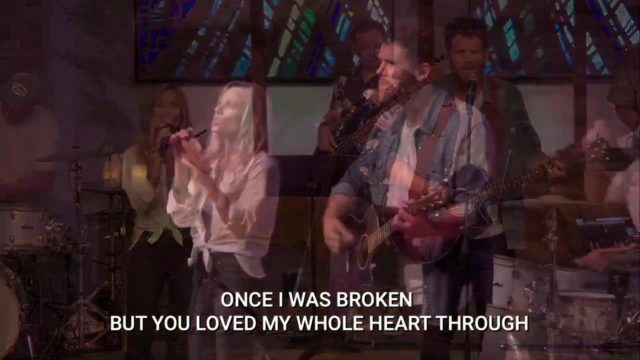 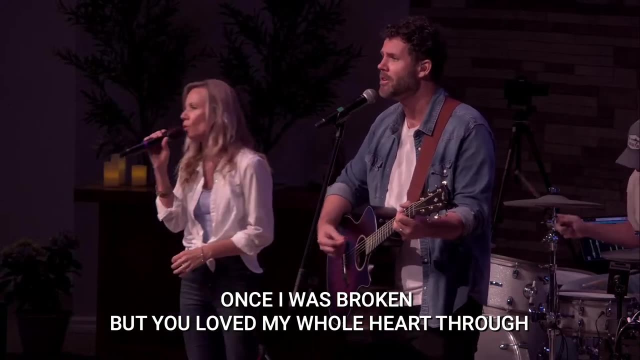 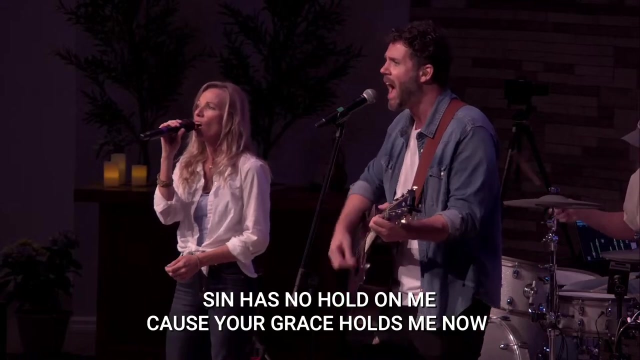 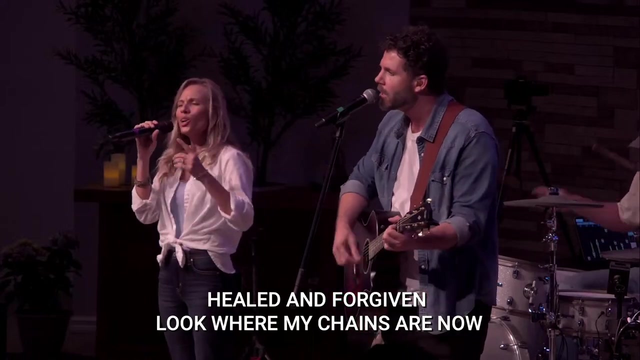 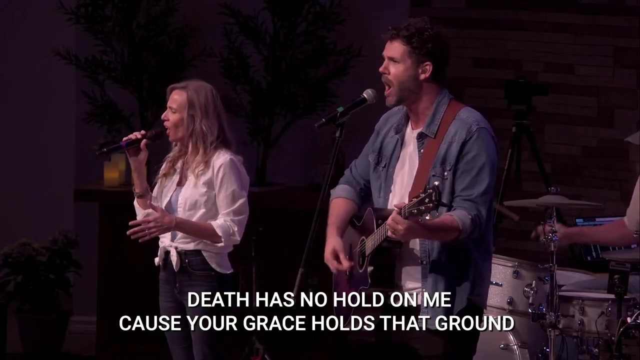 Oh, oh, oh. Hold my heart Now and forever. my soul cries out. Once I was broken, You loved my whole heart. blue Then. has no hold on me. Cause grace holds me now. Heal and forgive, Heal and forgive. Look where my chains are now. Death has no hold on me. 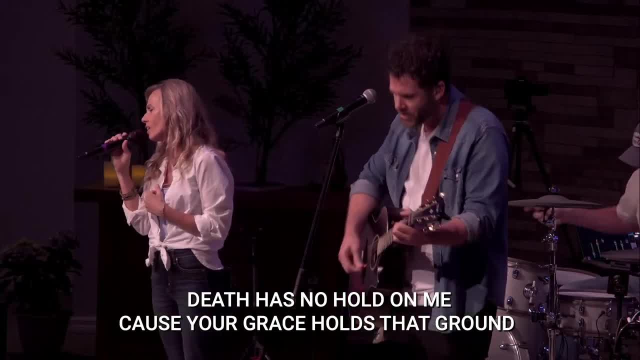 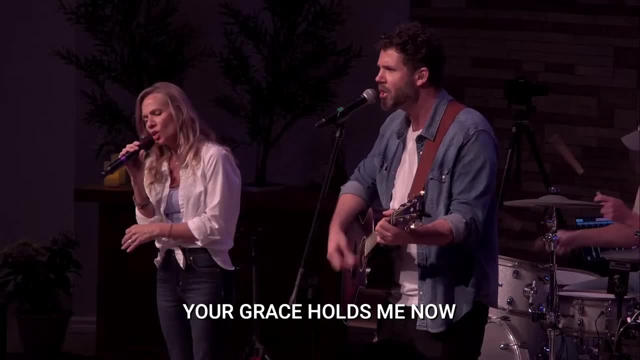 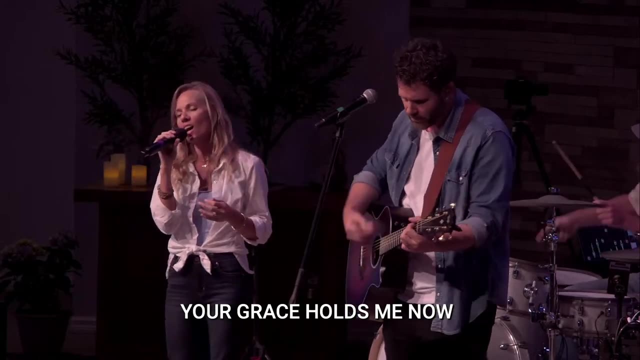 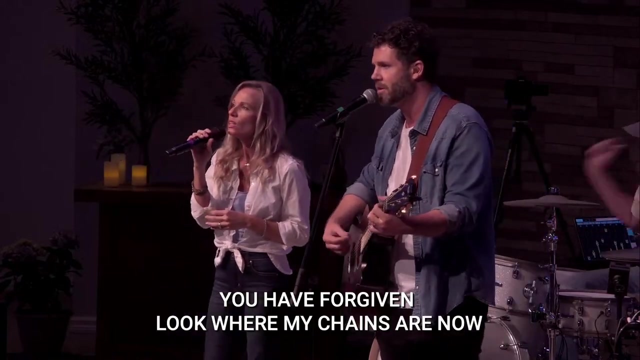 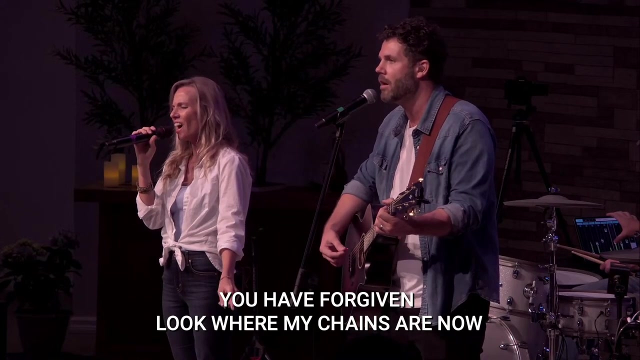 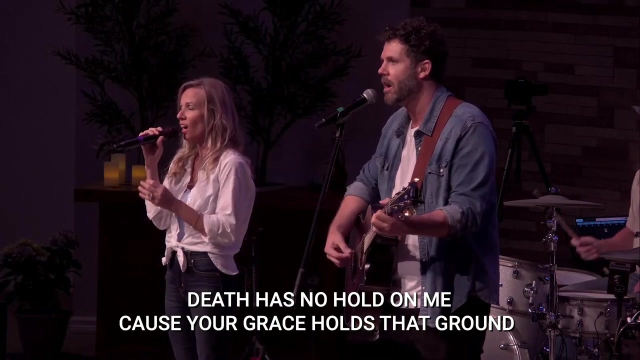 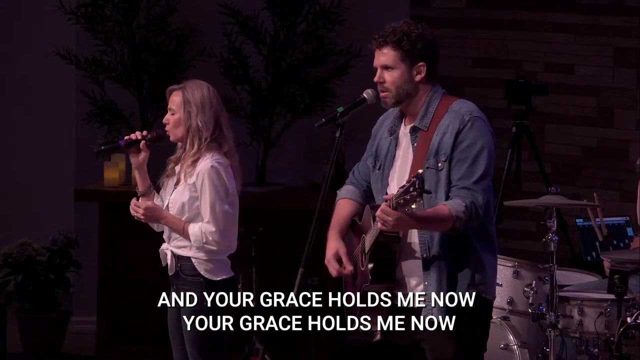 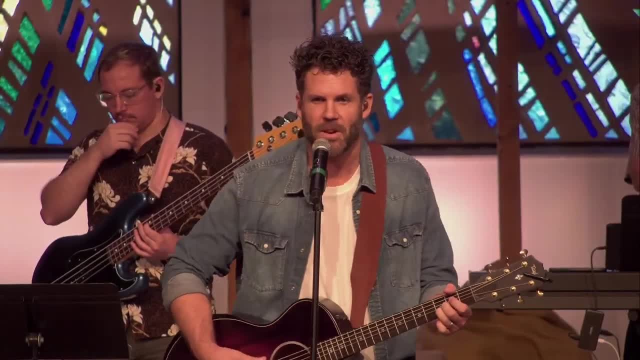 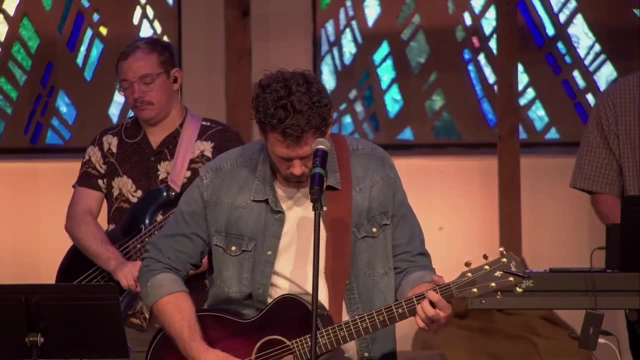 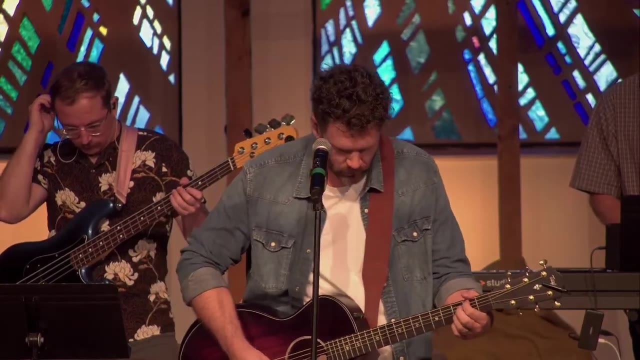 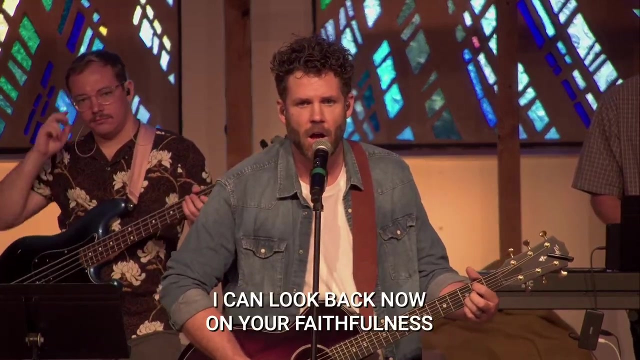 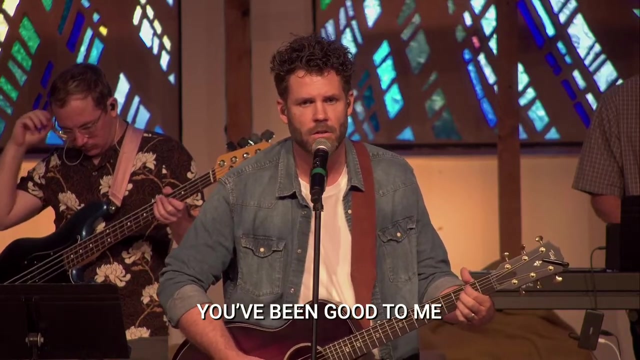 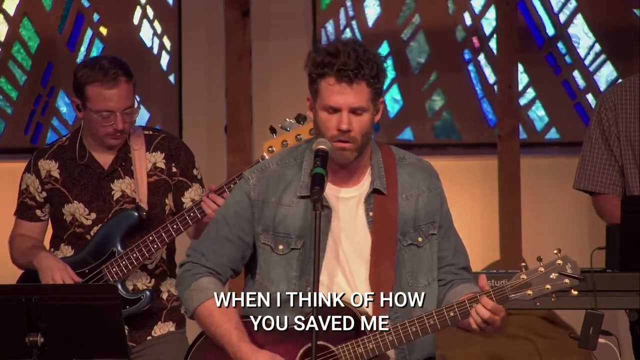 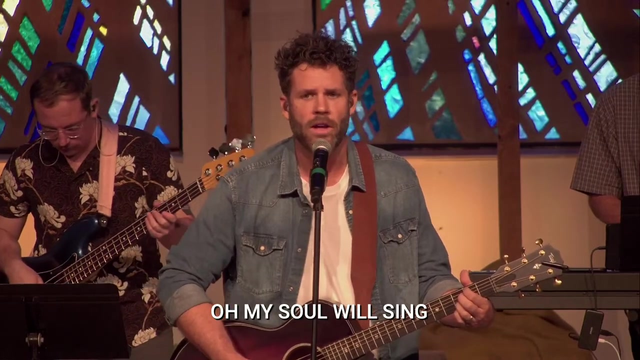 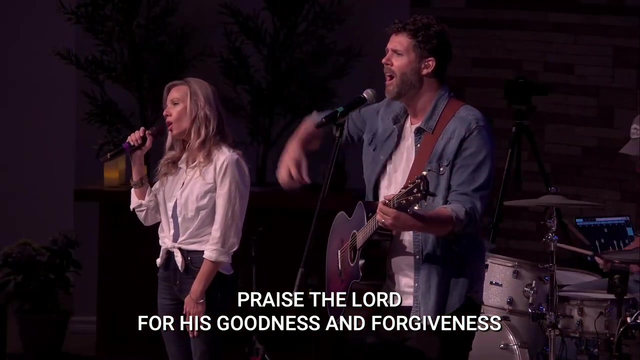 Amen. His goodness is here. His presence is with us. Let's continue to worship. I can look back now On your faithfulness. You've been good to me. When I think of how You saved me, All my soul will sing: Praise the Lord. 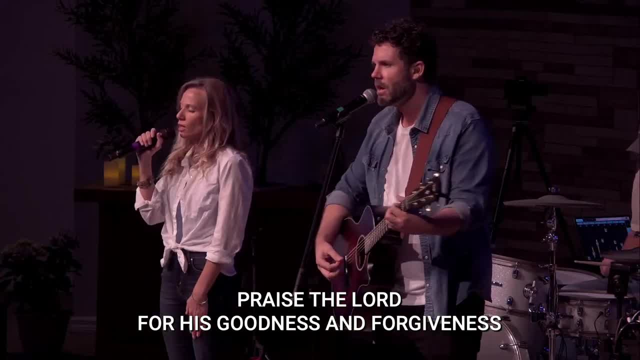 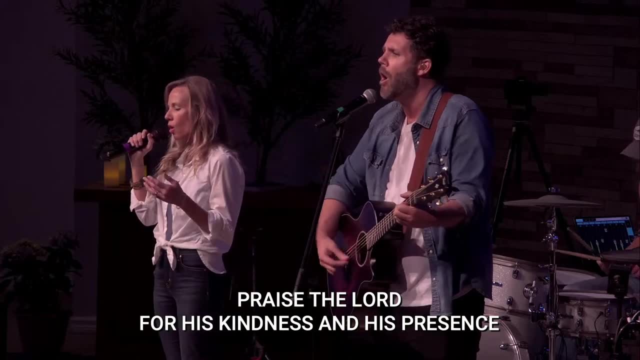 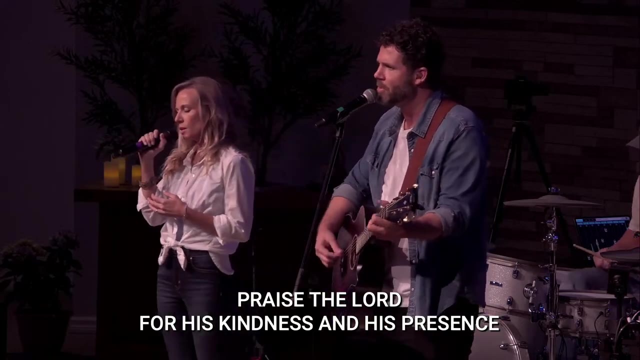 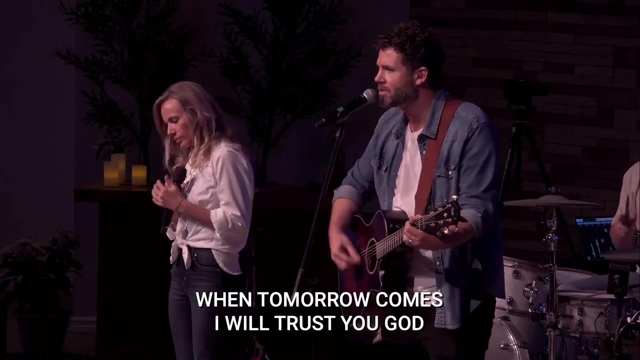 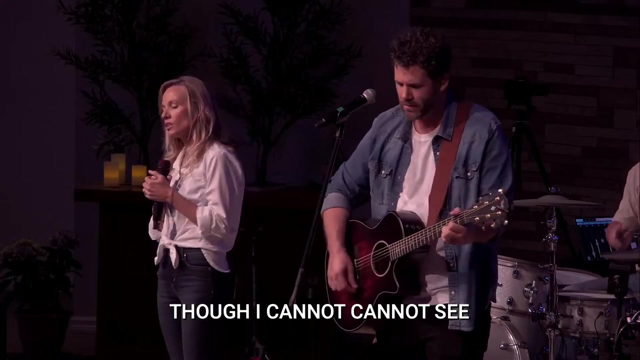 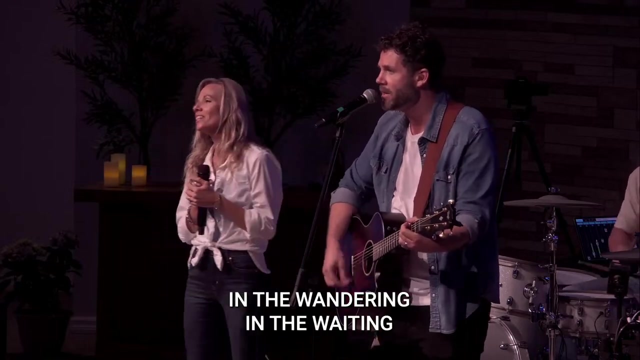 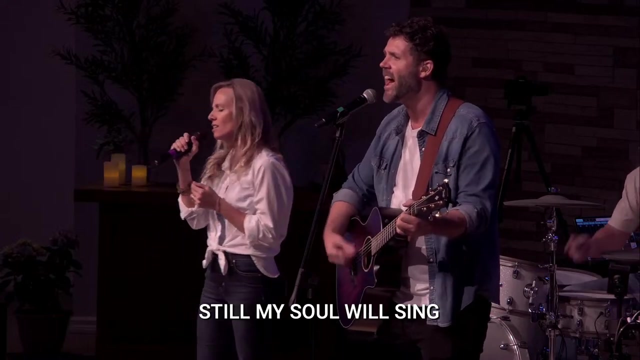 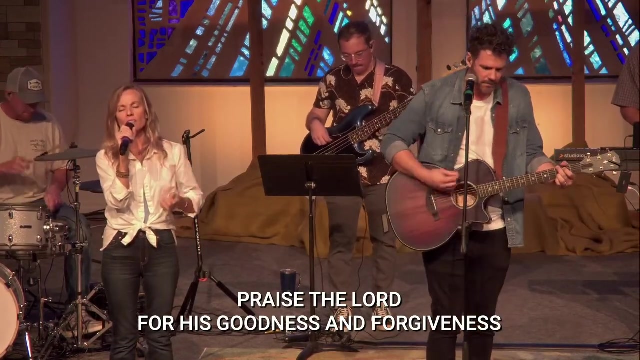 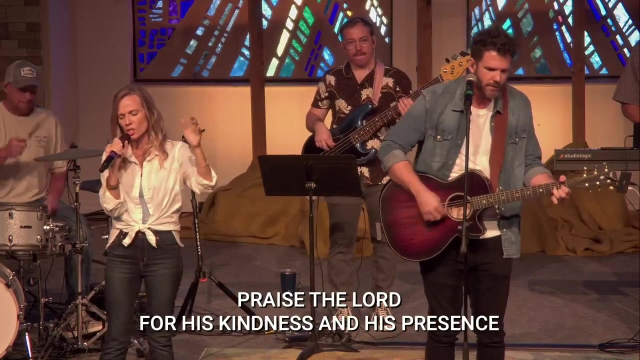 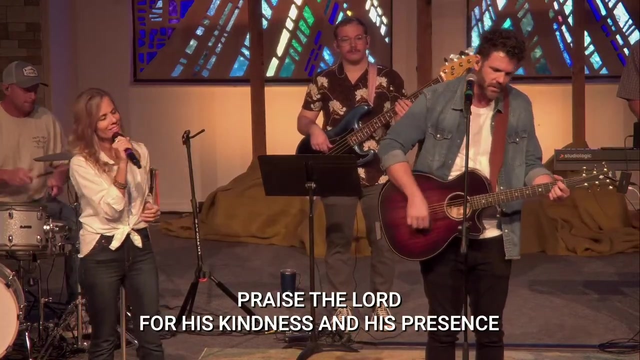 For His goodness And forgiveness. Praise the Lord For His kindness And His presence. When tomorrow comes, I will trust You, God. Though I cannot see, In the wandering, In the waiting, Still my soul will sing. Praise the Lord For His goodness And forgiveness. Praise the Lord. 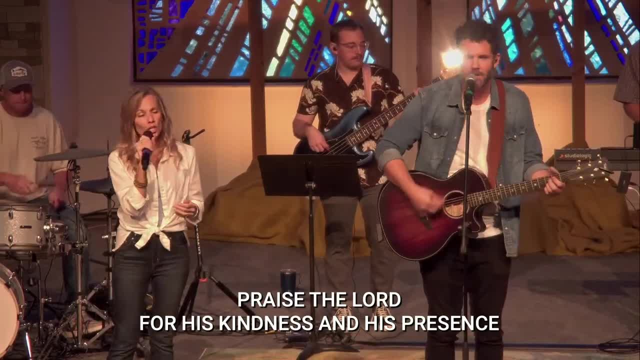 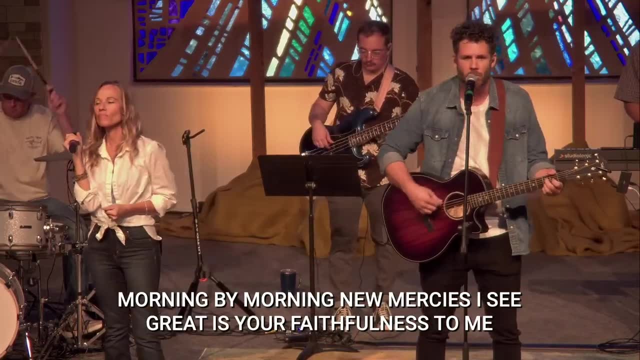 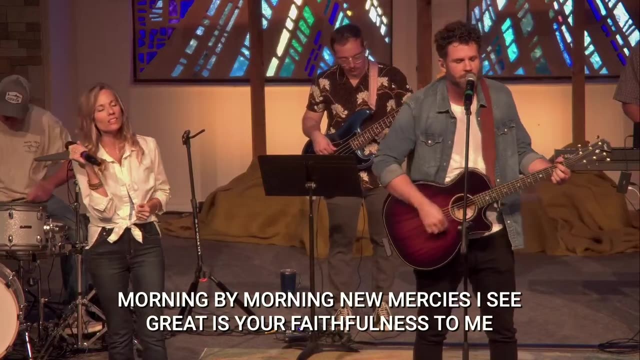 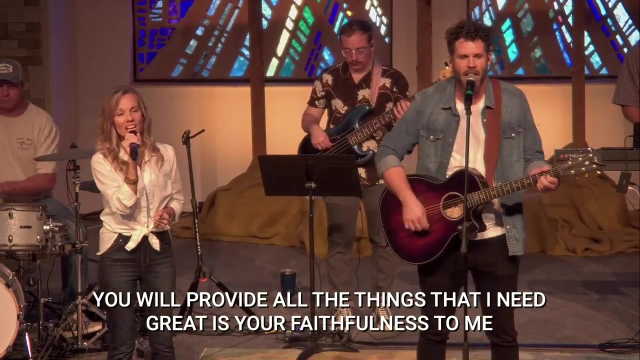 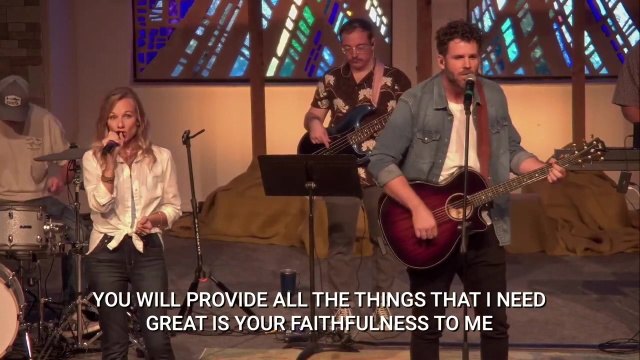 For His kindness And His presence. Praise the Lord, Morning by morning. New mercies: I see How great is Your faithfulness to me. Praise the Lord, You will provide all the things that I need. How great is Your faithfulness to me, Morning by morning, Morning by morning. 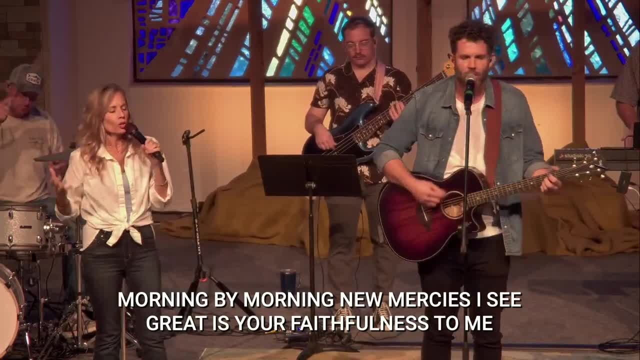 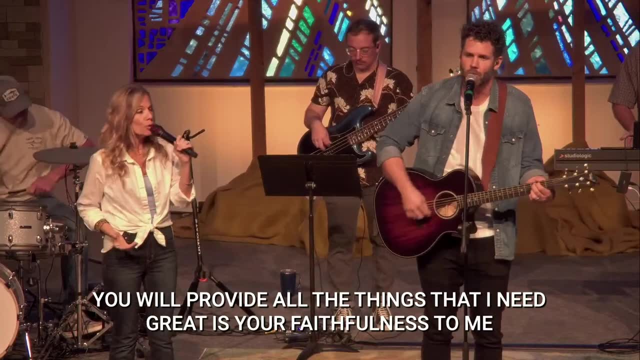 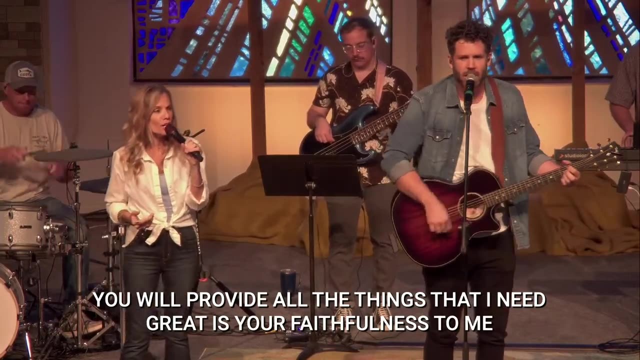 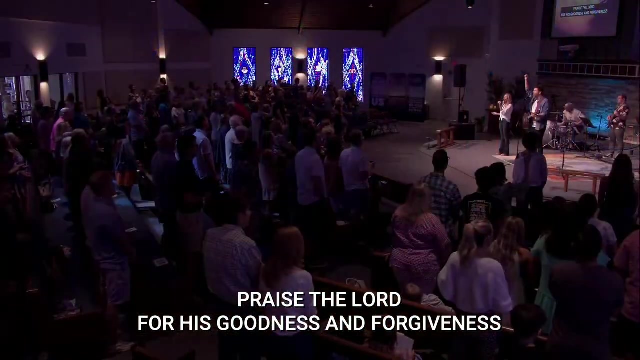 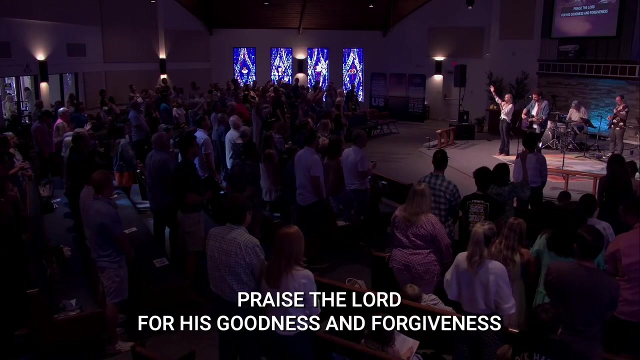 New mercies. I see How great is Your faithfulness to me. You will provide all the things that I need. How great is Your faithfulness to me. How great is Your faithfulness to me. Praise the Lord For His goodness And forgiveness. Praise the Lord. 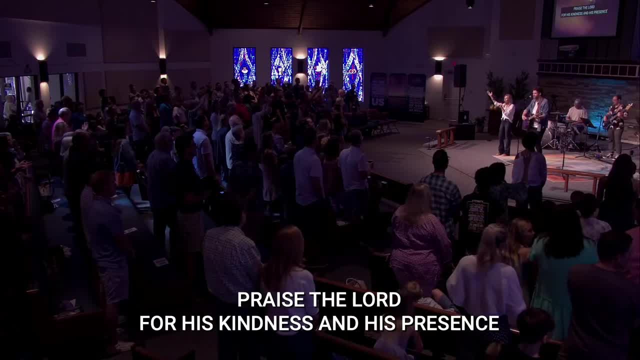 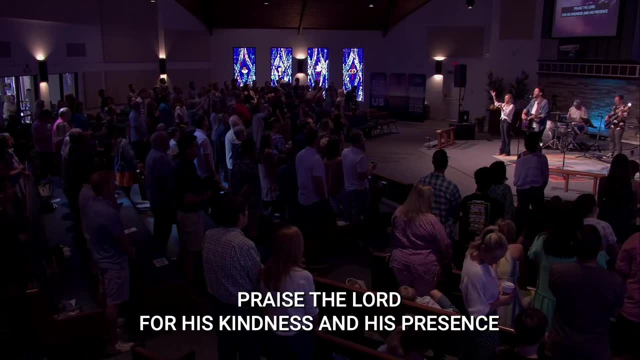 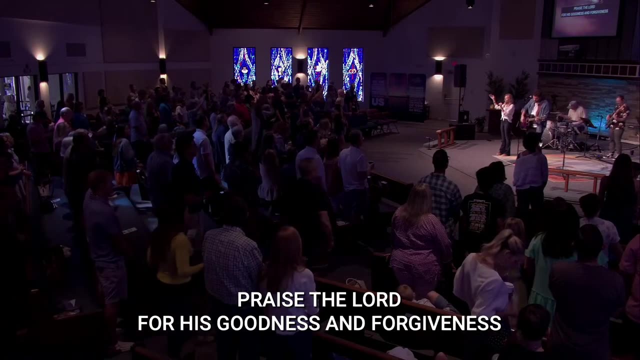 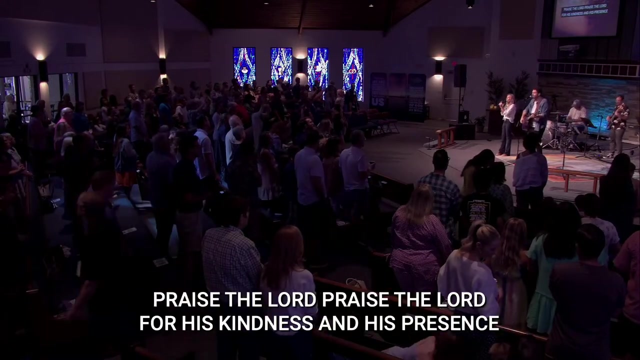 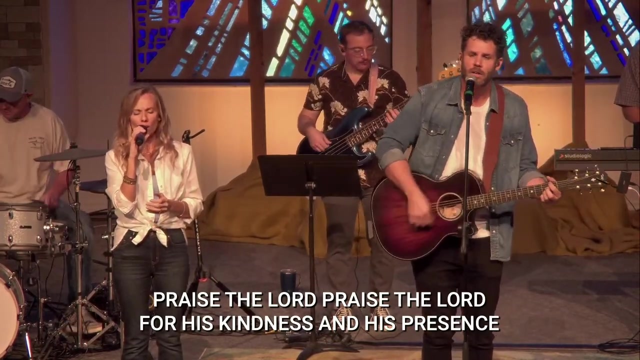 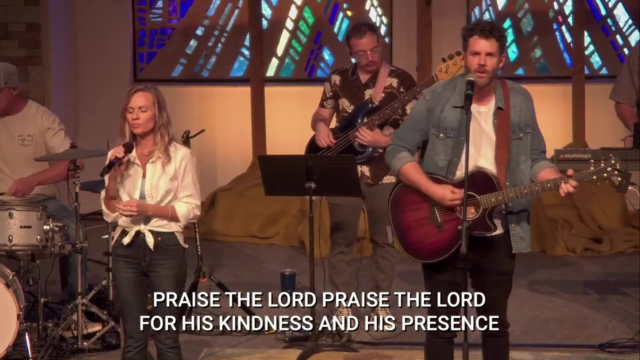 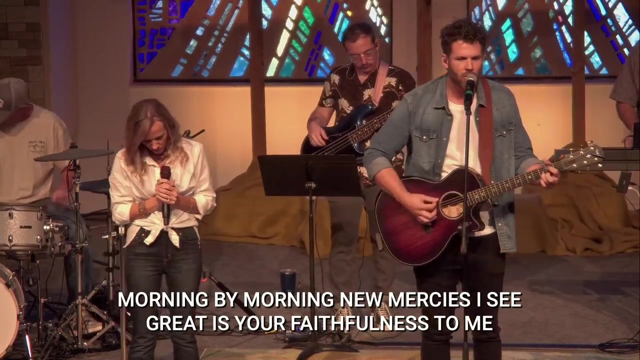 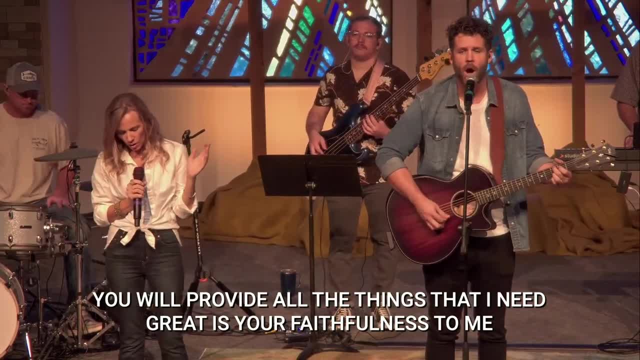 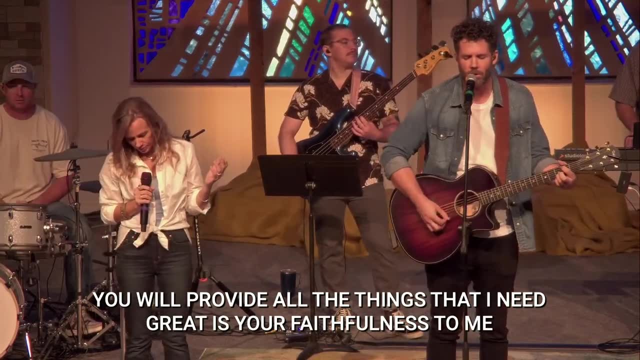 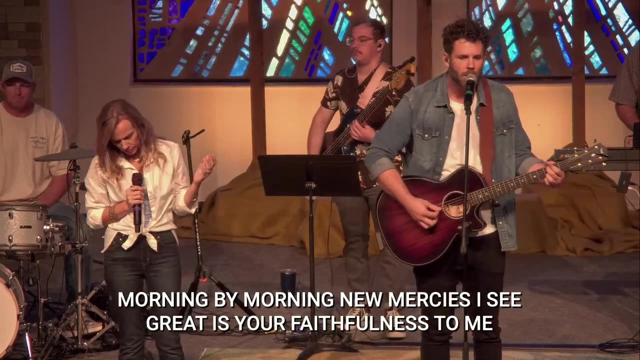 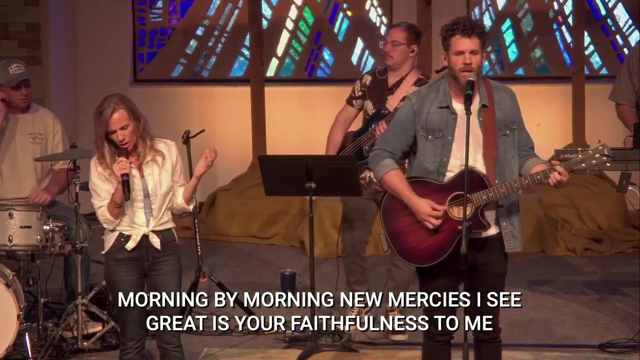 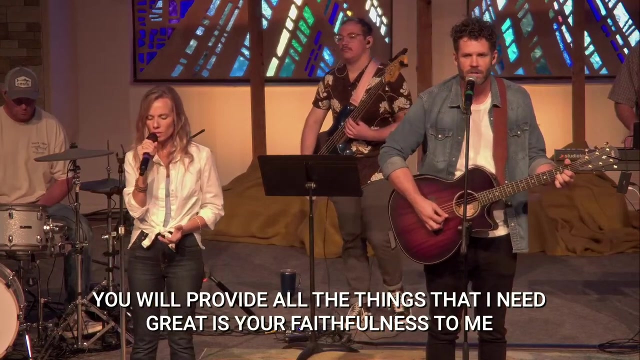 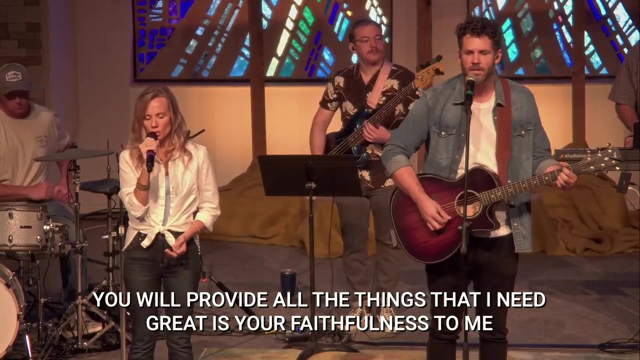 You will provide all the things that I need. Great is your faithfulness to me. Morning by morning, morning by morning, New mercies I see. Great is your faithfulness to me. You will provide all the things that I need. Great is your faithfulness to me. 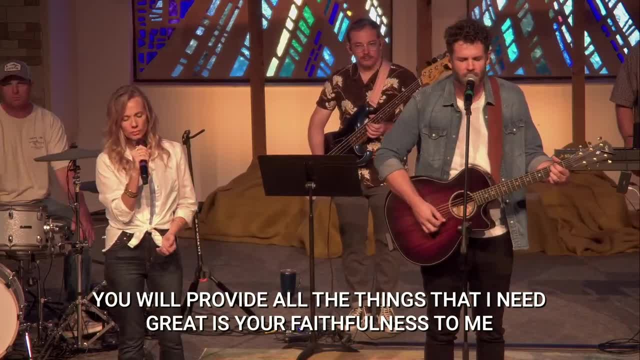 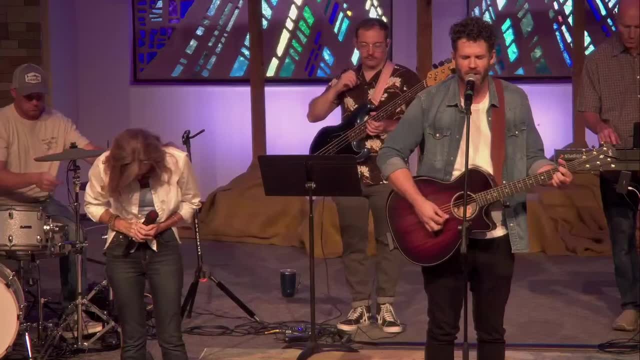 Jesus, we believe that in this place, We know that you're for us, We know that you're with us, We know that you provide all that we need, God. But as we'll dig into your word today, God, not let us make it about us. 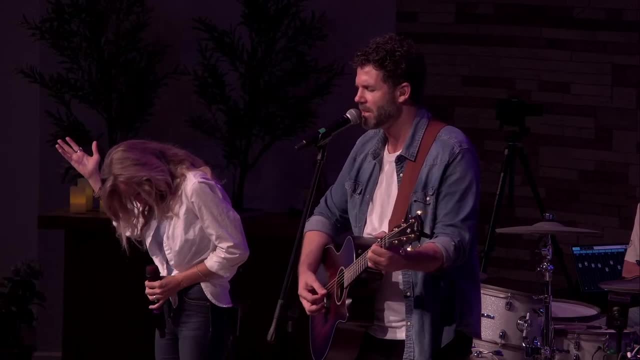 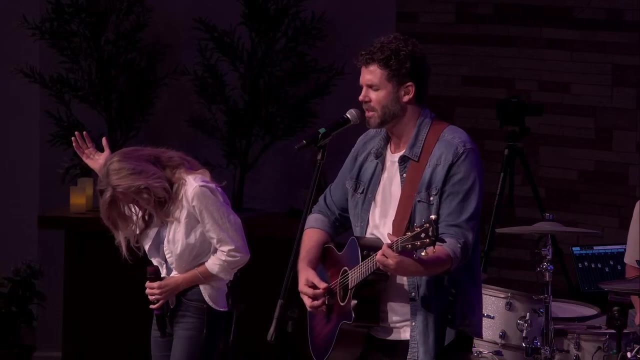 but let us be highlighted into the things that you're trying to speak to and through us, Because, ultimately, we're here to speak to you. We're here to speak to you. We're here to spread your word, to spread your life, to spread your love to those who need it. 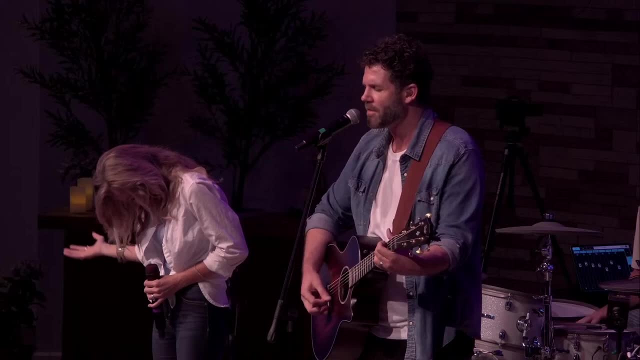 And that's everybody, God. So we thank you for calling us to be a part of this day. We thank you for your faithfulness, your never-ending faithfulness. We thank you for the victory that we can find in you, God. 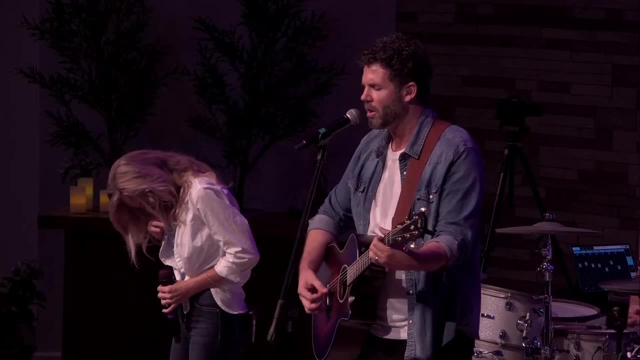 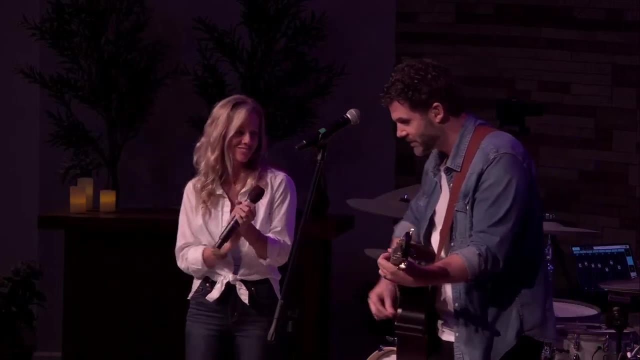 And it's something worth celebrating. God, And we give you all the glory, for you're worthy of it all. In your name, we pray Amen. Hey, let's lift up a shout of praise for him in this place. All right, good morning, Rock Harbor. 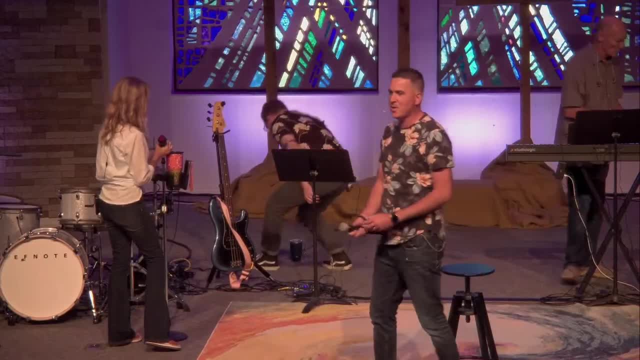 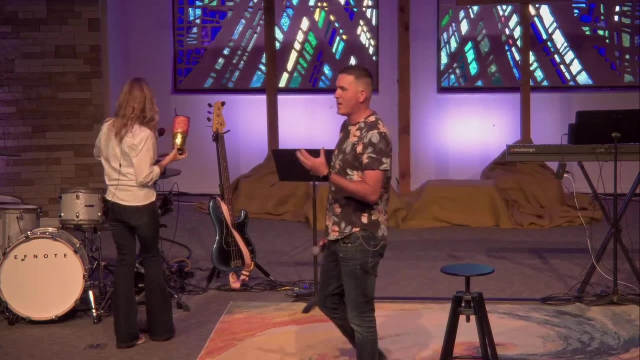 We are so excited and so glad that you are here this morning And it's just been such a great weekend and God has been moving in some incredible ways. I actually just want to highlight something for you that God has been doing kind of amongst just the ministry here. 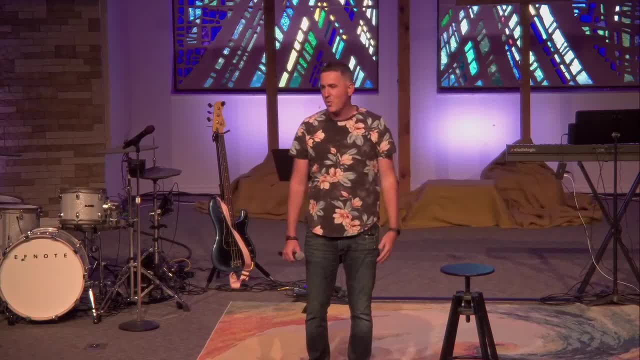 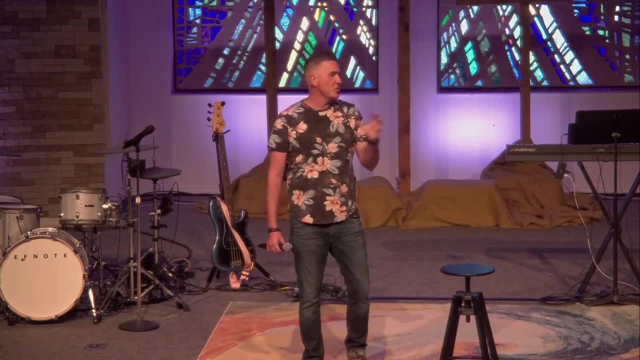 For one. you may not know, but we actually have a new soundboard back there which I'm excited about because the old one's going to go into the fellowship hall where we do youth group and children's church and so many other events for the church. 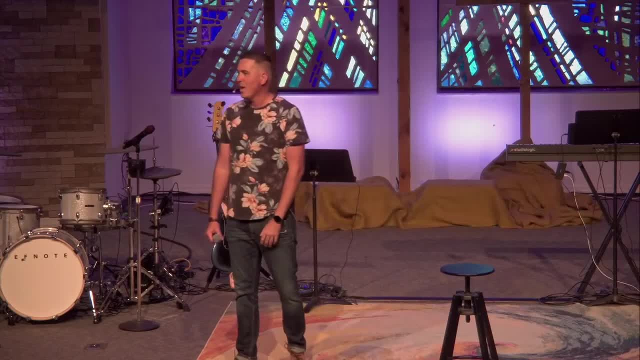 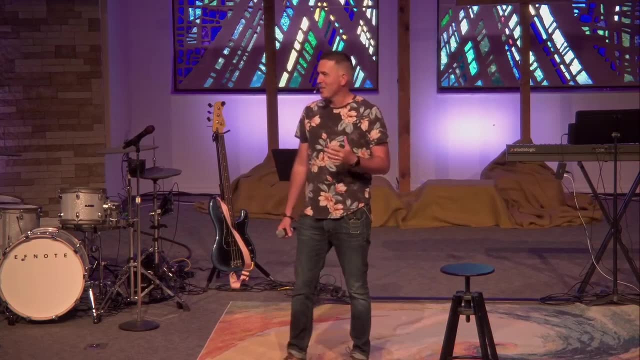 And I just want to highlight just a ministry that God has just been pouring into, And so I think it was about Thursday around 4.45 pm I got an email and it was a connection card, which was odd because you know it's 4.45 on a Thursday. 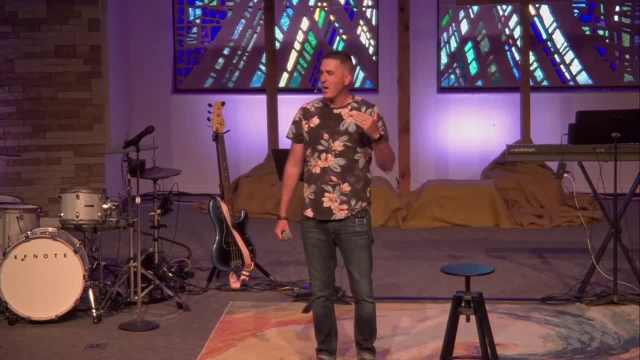 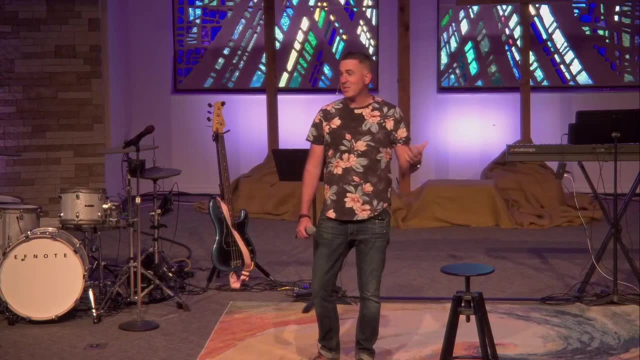 And I looked at the connection card and the person was from Melbourne. And then they had checked the box that said: I made my first time decision to give my life to Jesus And I was like man, that's incredible. And so we texted, reached out to them. 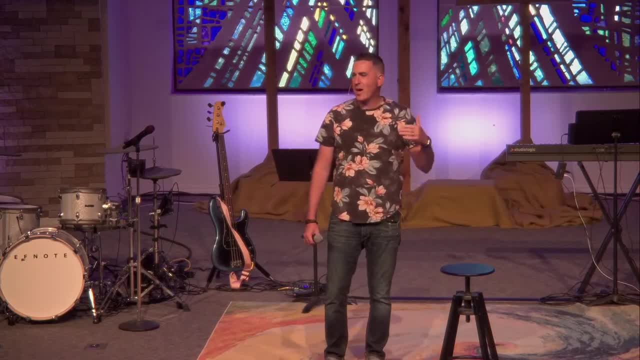 and they were watching the Easter service online. And then we got a text about four hours later And I noticed that it was a male name from the same last name and same address, And so you know. we haven't had a chance to hear the whole story. 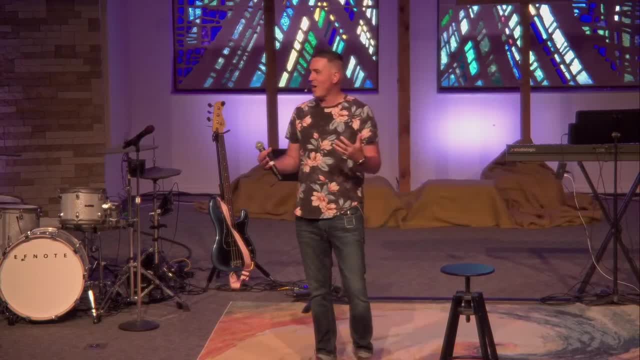 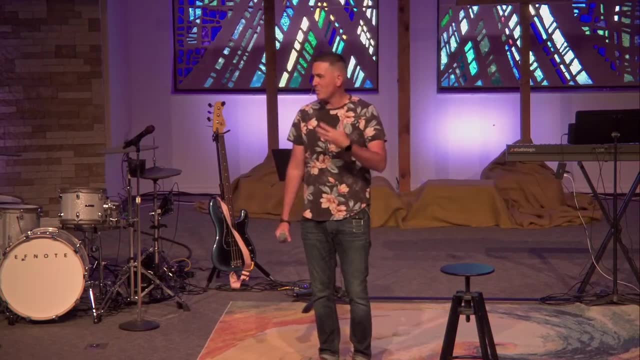 but family came home and they continued to just watch the services online And we're just so thankful that all these little things that we've been investing, we don't spend money on technology. We invest in the ministry tools so we get the opportunity to share the gospel of Jesus Christ. 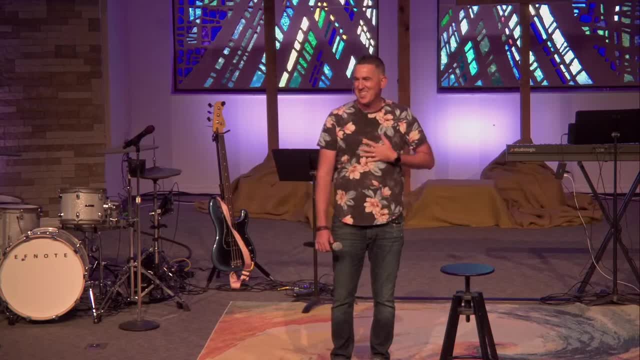 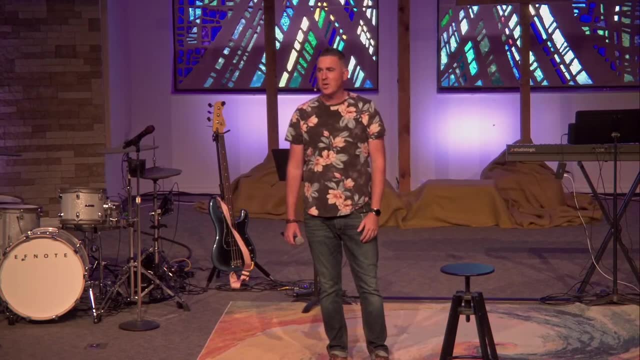 And so we're just so thankful for our team. Yeah, we can praise God for that for sure. So praise God. So I was just so thankful for all the team that has worked so hard, especially this this week, to bring in a whole new system. 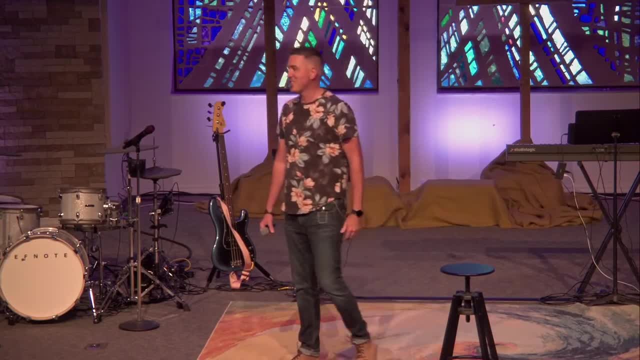 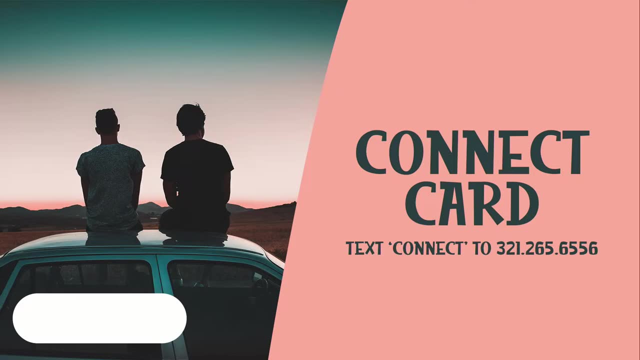 and get things organized. We praise God for you, So connection cards are such an important way for the church. Next week we have a baby dedication and that conversation was started through a connection card And we just continue to just use it as a great tool. 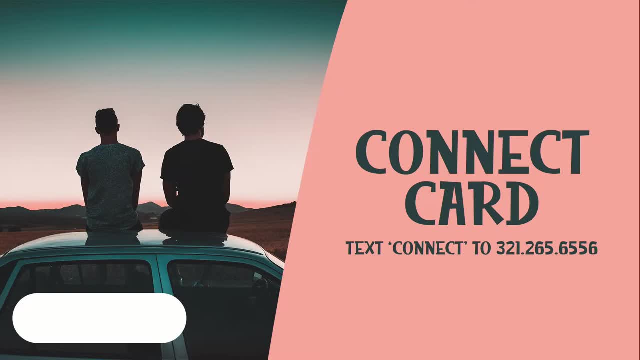 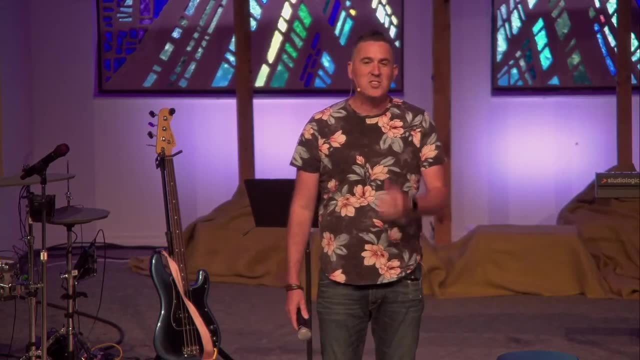 because Sundays, when you have ADD- which you haven't noticed in my sermons, I do- we get the opportunity to follow up with you during the week, when things are a little bit slower. Ladies and gentlemen, would you invite my wife on stage? 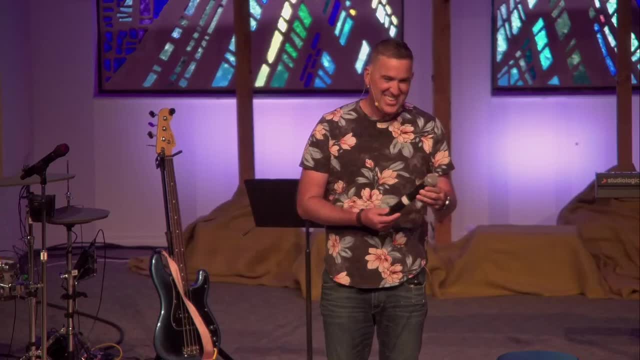 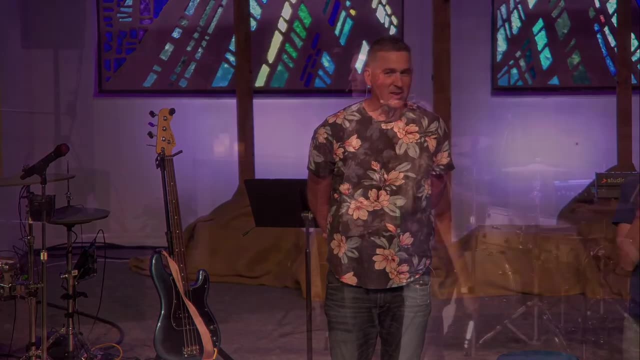 Angie Diamond. It's just not the same without you. We missed you up here. So welcome. We'll blame Scott Dwyer back there. He got me chatting. I'm so sorry. Good morning, I'm so glad you guys are here. 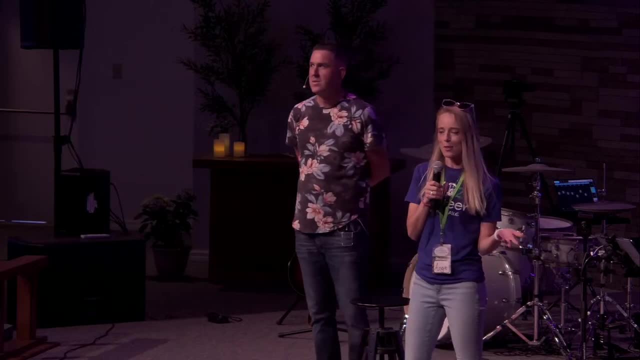 So what's going on with Children's Church today? All right, So three-year-old through sixth graders are invited to join us for Children's Church. We have three years of kinder together and then first through third and then four through six. 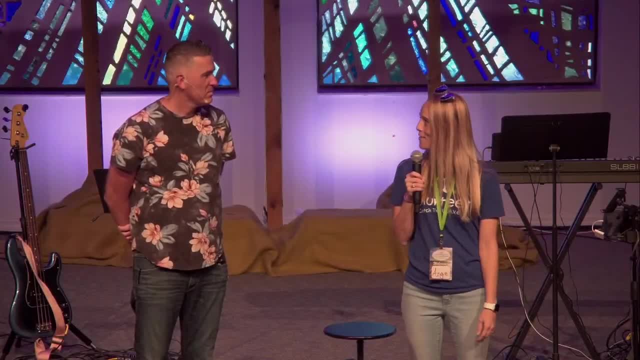 And it's going to be a great. we're like an act, So it's a great time of just hearing what happened next right After Easter. it's great, So your kids are invited If you do not know where to pick them up at. 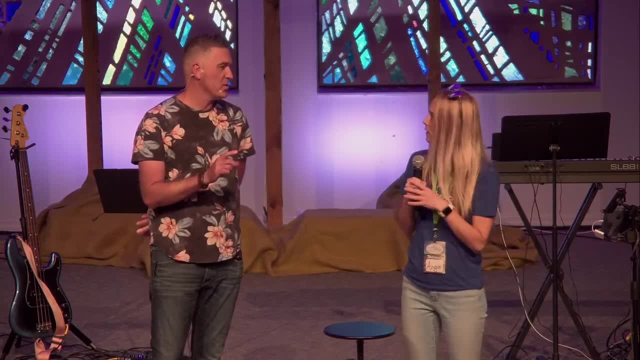 you can ask them with a lanyard. Yeah, I'm so excited. What was the story that you guys are doing for four, five, six? today We're doing Dorcas and Aeneas. Yeah, just a story that maybe some kids 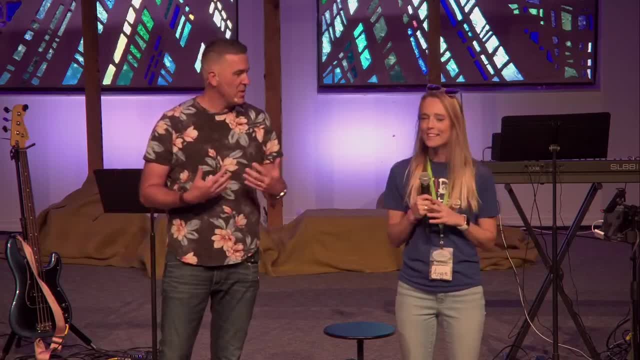 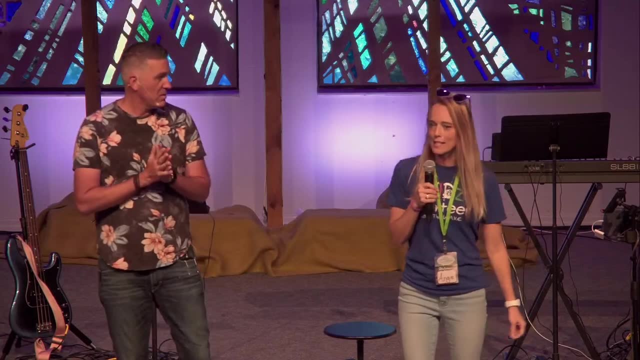 The Holy Spirit. Yeah, that's what it was. Yeah, So it's just an amazing story that some kids maybe have never heard before. Maybe some of us have never heard before, And so it's great to hear that. And we've changed the date on Club 456.. 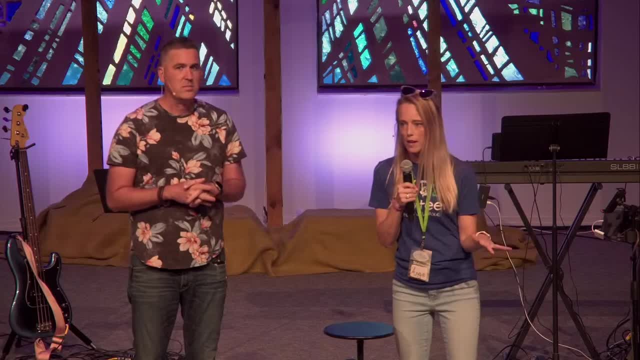 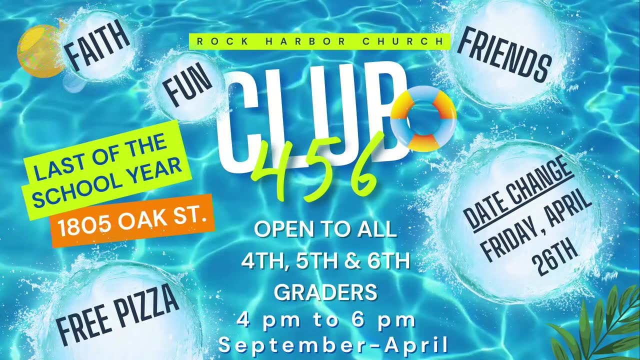 So if you have a fourth, fifth or sixth grader, once a month we have an event during the school year. So this month it's going to be April. 26th is our four, five and six. We had to change the date. 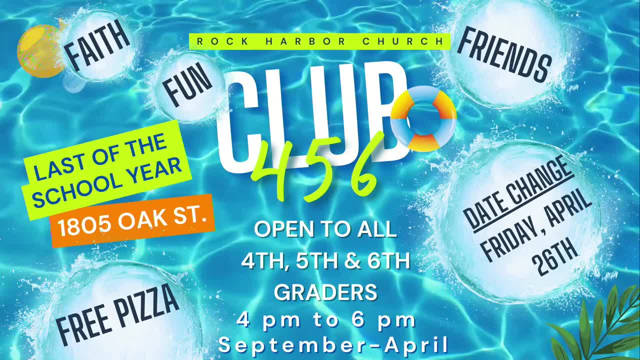 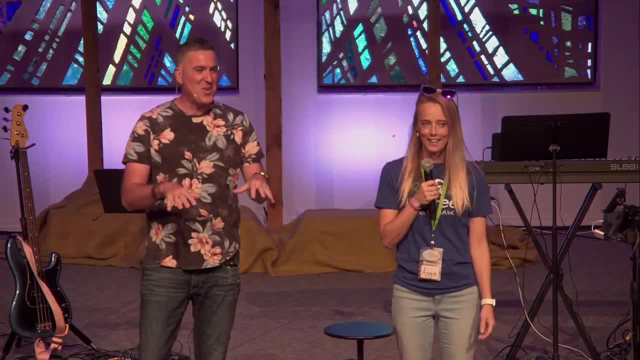 due to an awesome wedding that's happening this Friday. Yeah, and they're here. We got Matt and Madison with us. Yeah, Eminem getting married. There's a wedding right here on Friday. It's actually the first Rock Harbor wedding in the building. 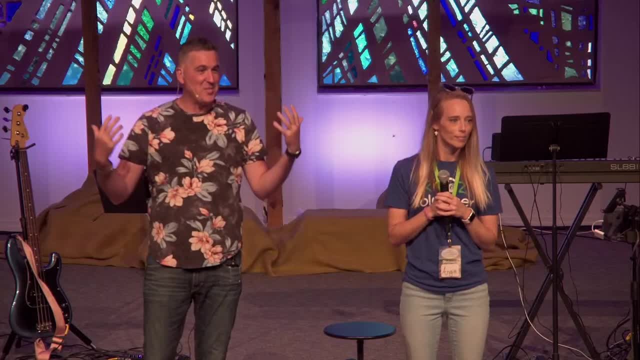 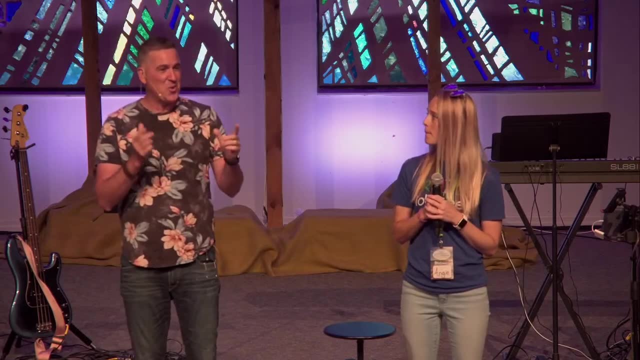 And then what's so cool is that Matt's dad built this building like back in the 80s, And so just an amazing story of God that we are just seeing. God, bring you guys together. Oh, and the the quarter three strands is arriving tomorrow. 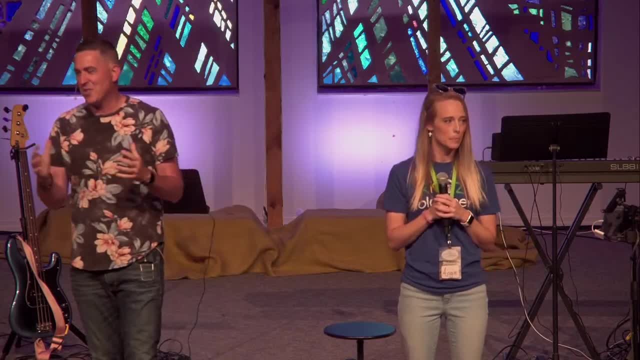 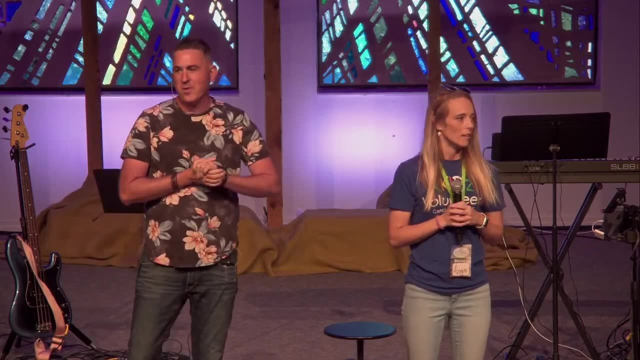 I got the confirmation. So we're just so excited for what God is doing in so many different ways and that we get a chance to be a part of that, And and also tonight we're having a glow party for youth group And so it's going to be kind of a finale of this series. 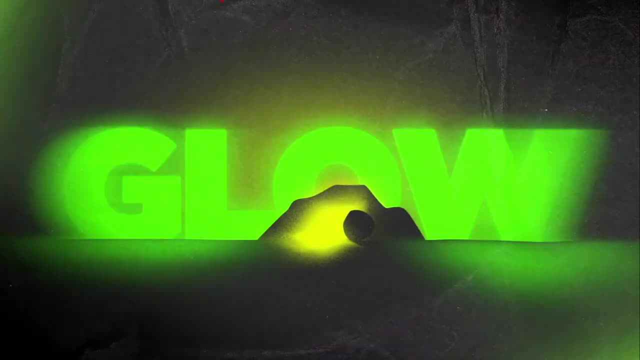 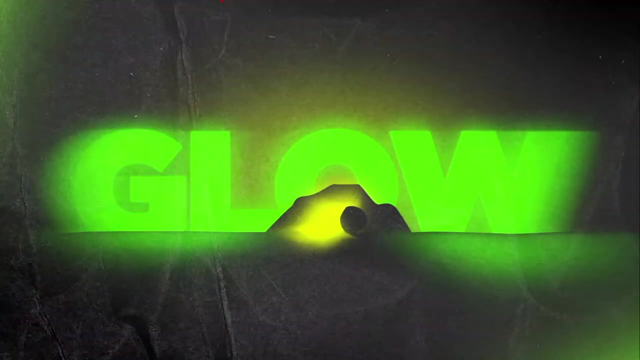 on understanding how we can live in the light of the resurrection. And so for our seventh through 12th graders, you are invited tonight to come in for our glow party. So Friday night I DJ'd a dance in the fellowship And we left everything set up. 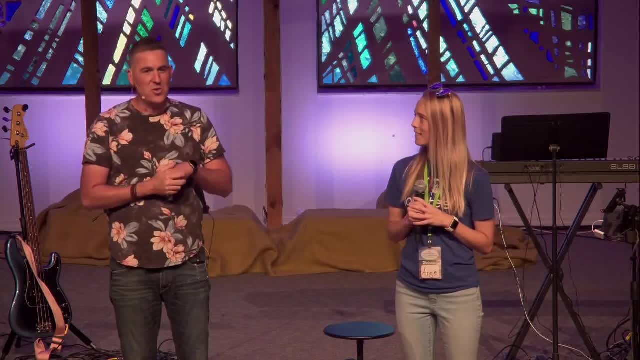 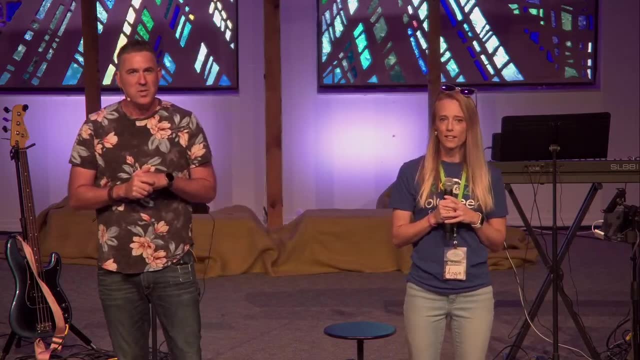 And so we're going to have a kind of a glow party dance at the end of youth group tonight, And so it's a great time to bring friends. If you are a middle school high schooler and you want to come, you are welcome. 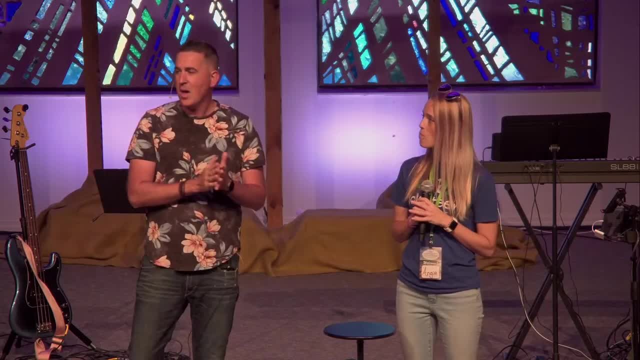 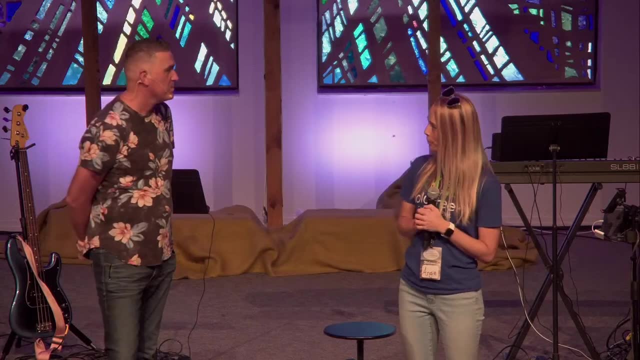 And so Friday night was the dance with coastal community, And we are so thankful to be able to partner with that amazing ministry that. what grades do they have? They're preschool through eighth grade. Yep, Yeah, So they got preschool through eighth grade. 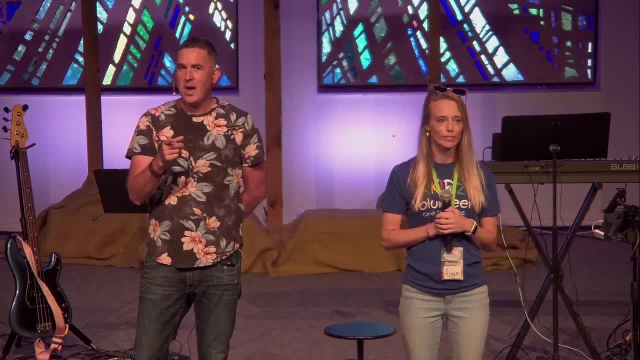 and then they have a 5K that is coming up And so we're going to have a dance with them, And it's called the Moonlight 5K because it's at North, it's at Spencer Holland, And so you get a chance to go to the golf course. 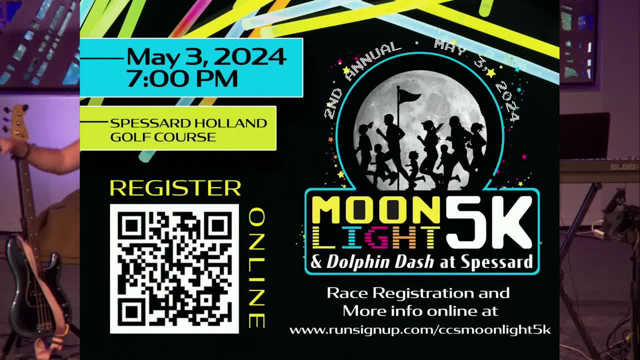 run the golf course at night And we've got a bunch of black lights and glow stuff for that We're going to be providing the sound. What else do we need to know for that event? Hey, just if you can register by today. 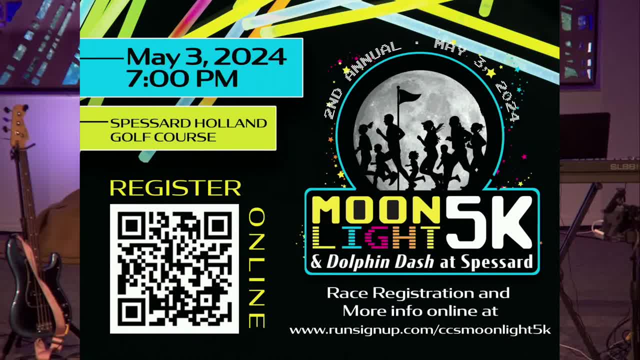 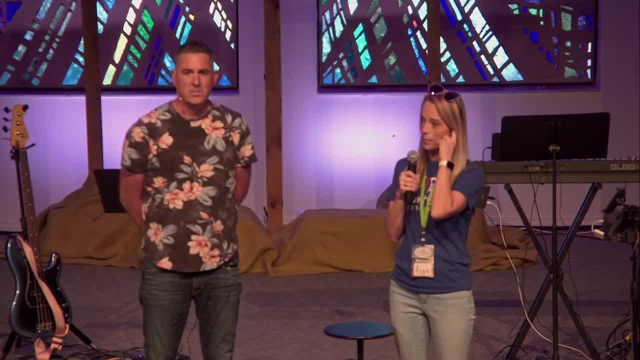 if you want to do it, in order to get your shirt and your medals, you know, ordered and stuff. So because you guys are all going to win. So if you can register today, there's actually flyers out there if you want to grab a flyer. 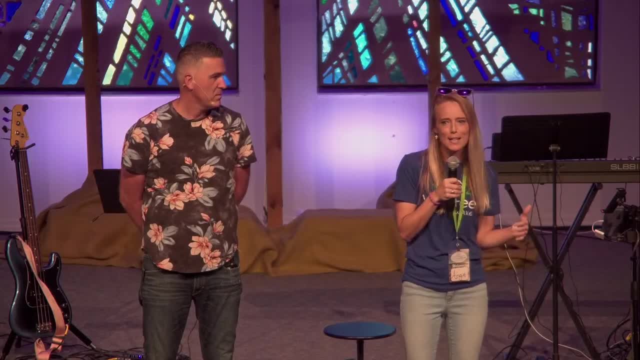 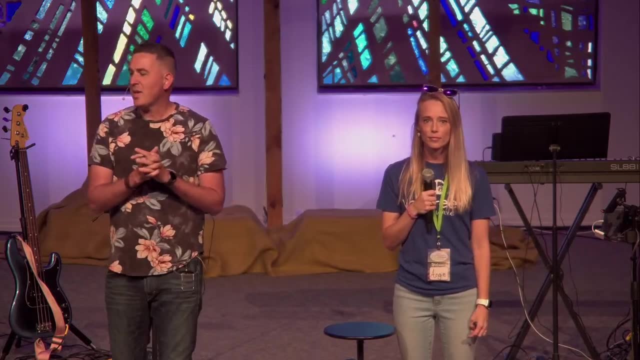 But this is a great time that Kevin DJs. we come together as a community at North Spencer, Holland, golf course. It's so fun. So bring your family. Yeah, it's going to be good. So last thing is, we always like to go before the Lord. 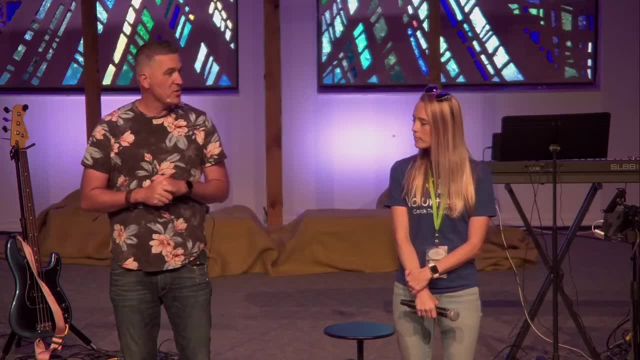 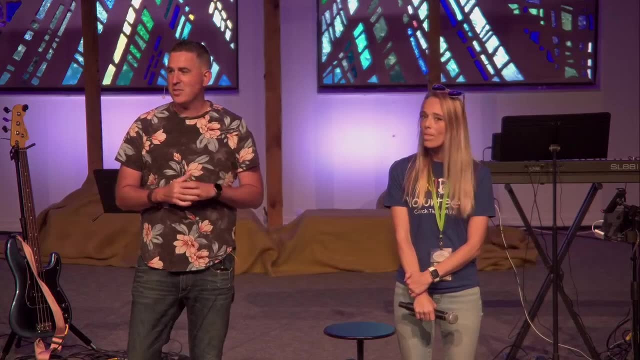 and mention just the fact that our tithes and offerings have been brought to the Lord. Some of you are like us and you give online, And so I don't know exactly how, but ours isn't on Wednesday, And so every Wednesday we see our online giving. 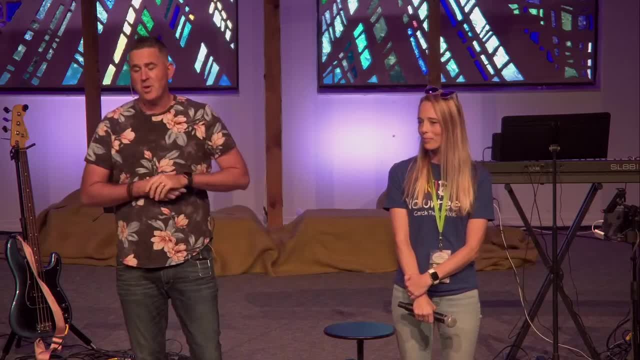 Some have using. we have collection box at the back. It's also a great place to put your connection card, And so we just want to go before the Lord, And this verse from Galatians was on my heart this week. that says: 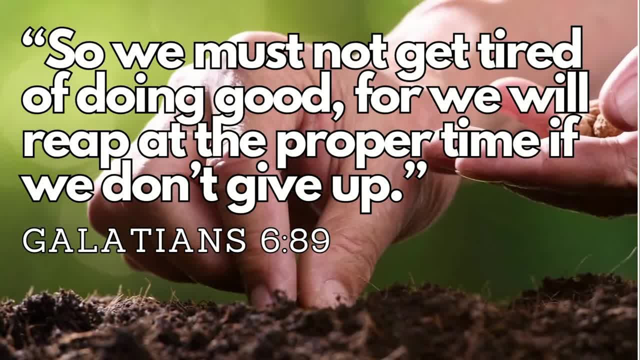 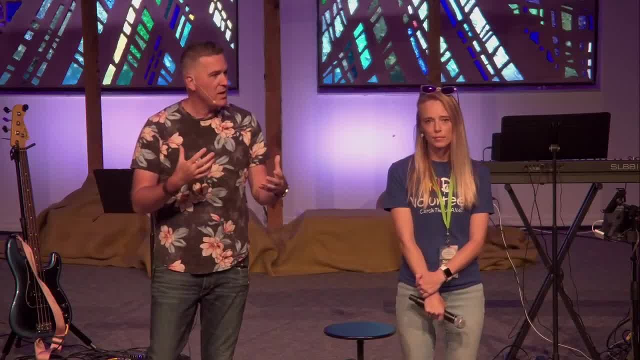 so we must not get tired of doing good, for we will reap the proper time if we don't give up. And so I've just been thinking about all this ministry that we've been pouring in, And now, for these past few weeks, we've been seeing such a harvest. 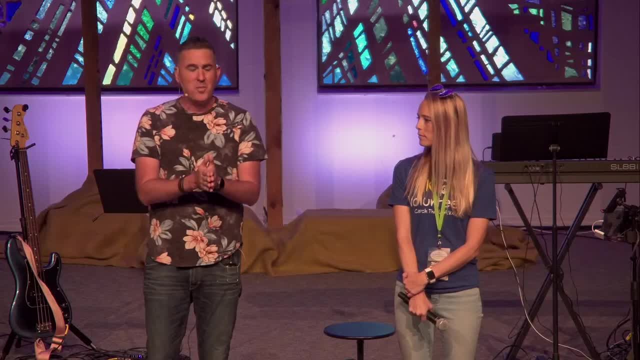 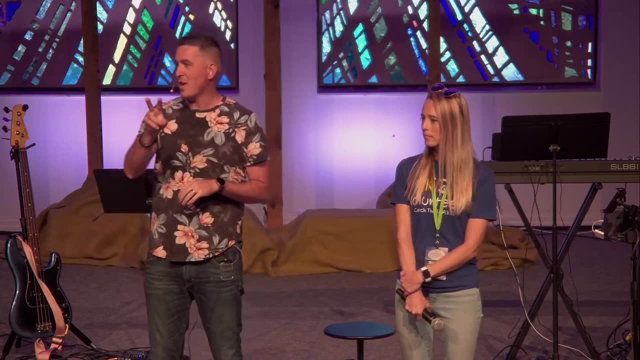 that we've been reaping from that And one of the beautiful things is, as we're preaching on the Bible, our church has given away. I saw two Bibles left. We had 47 Bibles on Easter morning And now we're down to two. 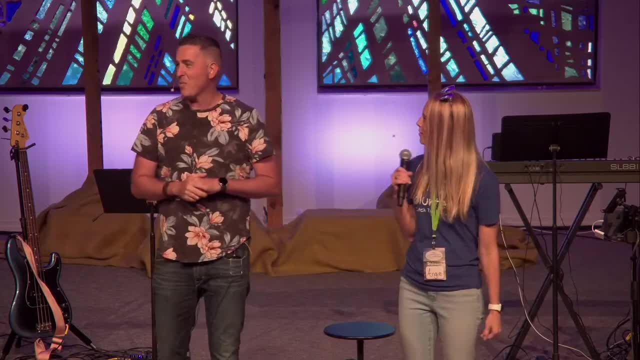 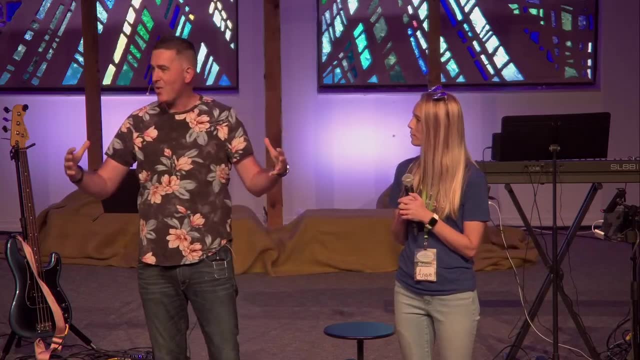 I've ordered two new boxes, So we've got 48 more. Our Bible's coming, but we've been able to give Bibles And you think about that, planting the seed, and then we're going to water by learning how to read it. 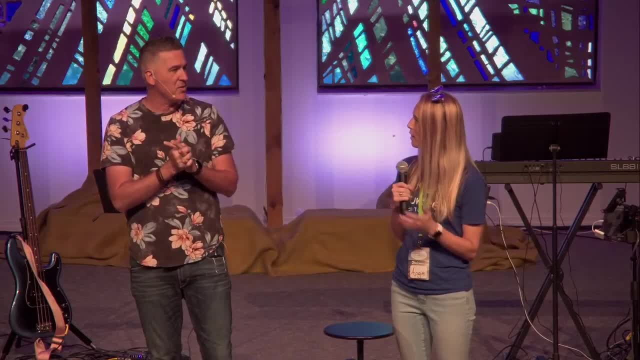 And then we're going to watch it go into people's lives And that's where we see that verse come to life, And so we praise God for that. Yeah, Speaking of Easter morning, I see a lot of you guys. would you stand up if you got baptized on Easter morning? 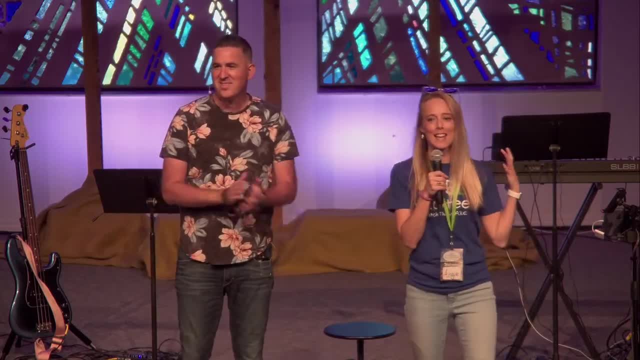 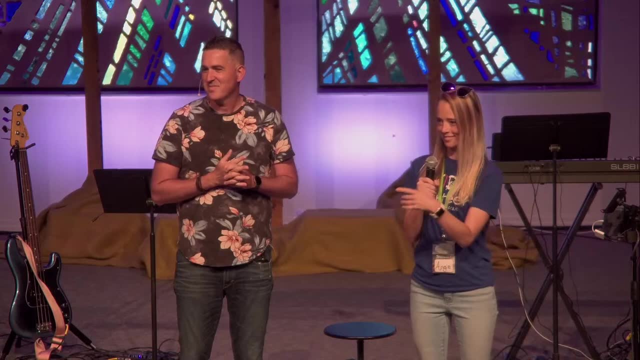 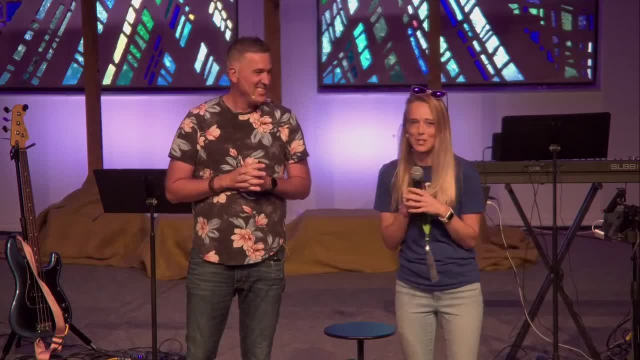 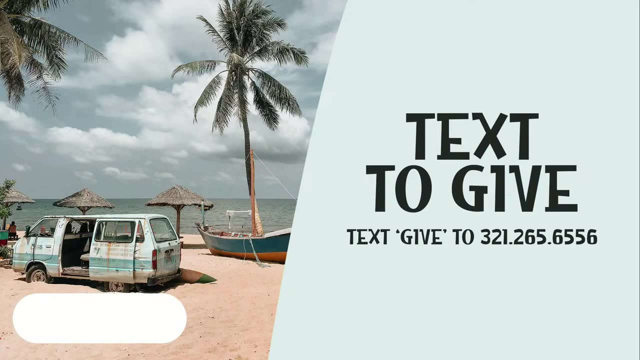 How fun is that Perfect? Yeah, Sorry I interrupted your prayer. Oh, it's okay, We'll pray God. we're so thankful, Lord, that you live in the midst of interruptions, Lord, that you live in the midst of life. 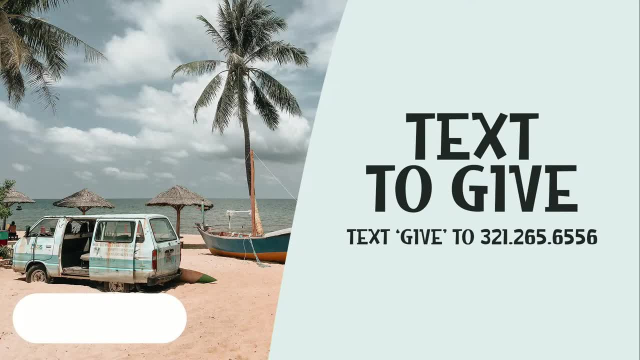 and that we get a chance to celebrate. I'm so thankful that our greeting's going longer than we planned, because we're celebrating all this different ministry that you're doing, from online to on the beach to giving out Bibles, and that you're meeting us. 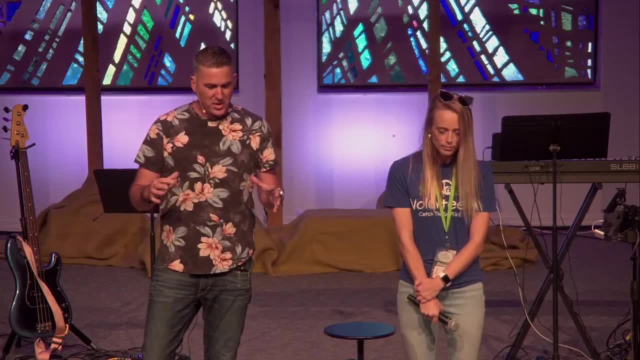 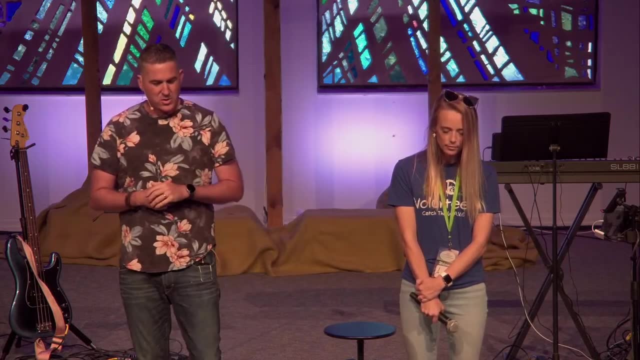 that we continue as a church, we say to give you our blessing, To give you our best, and that you bless the rest. And, Lord, we see the same thing true, as we recognize our tithes and offerings, that, Lord, we give you our first. 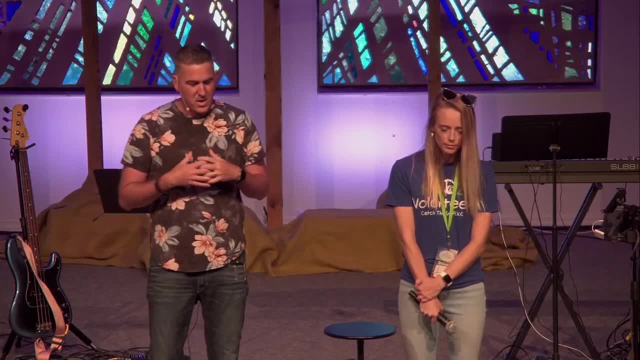 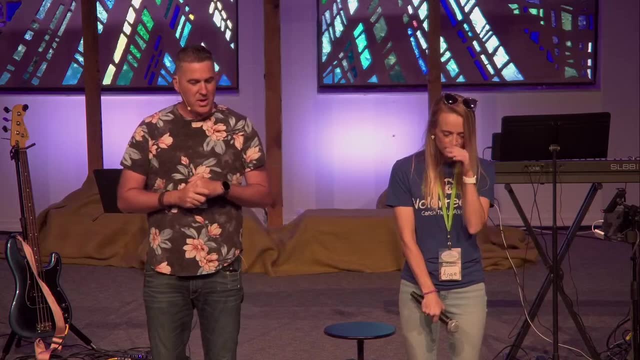 and we know, then, that you can bless the rest. And I know from my life, when I realized that I could live 100% of my own, or I could give to you what is yours, and that you will bless everything in my life, and that it becomes the life that we wanna live. 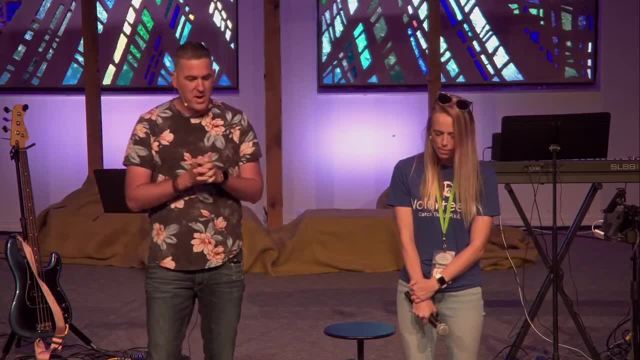 And so, Lord, we're just so thankful that we can bring this before you And we pray this in the name of the Father, the Son and the Holy Spirit: Amen, Amen. All right, And Kenzie Kenzie's got the brown box. 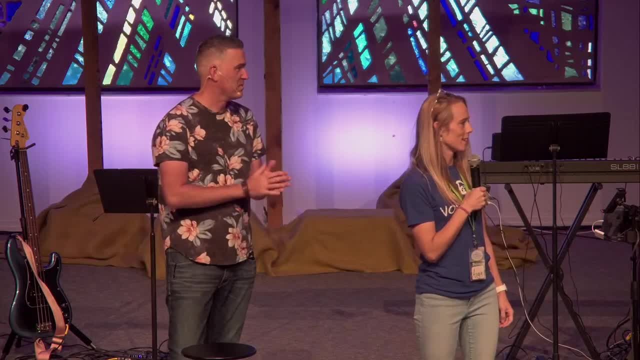 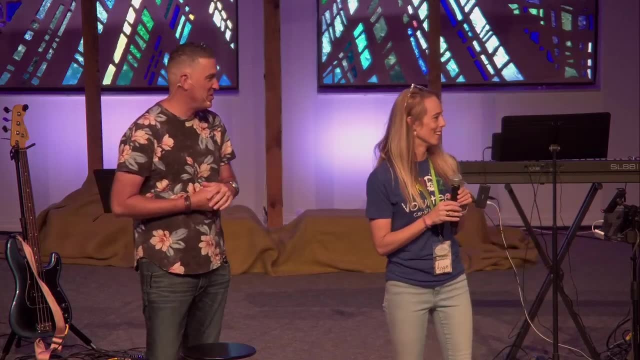 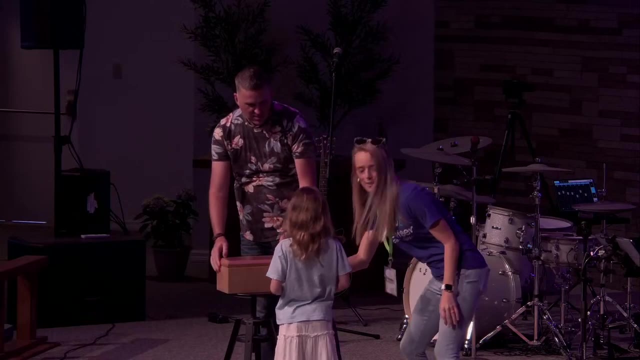 And so let's hear it for Kenzie. Kevin, take off that hat, man. All right, Kenzie, I'm excited to see what you've got in the brown box today. All right, there you go. Thank you, All right, Kenzie, how old are you? 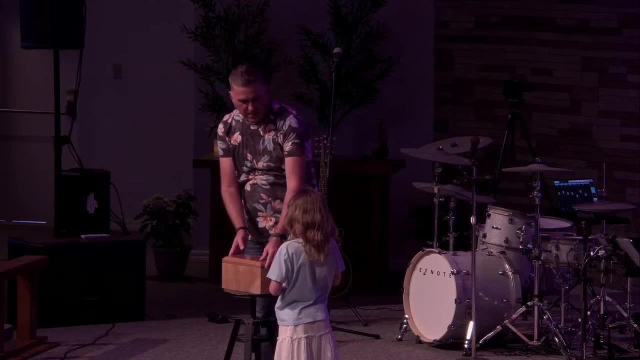 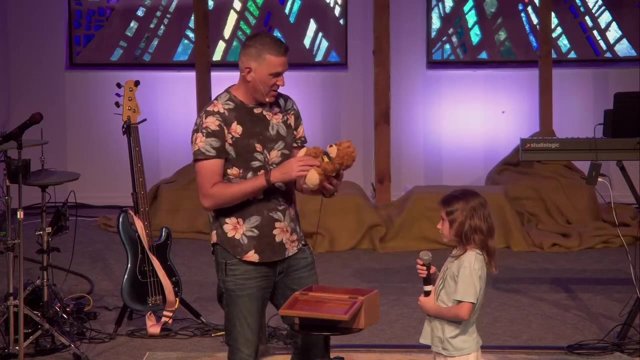 Seven. You are seven, All right. Where do you go to school? at Costa, Okay, very cool, Very cool, All right. How are you feeling? So we're gonna, we've got a teddy bear and it's got a bad word on it. 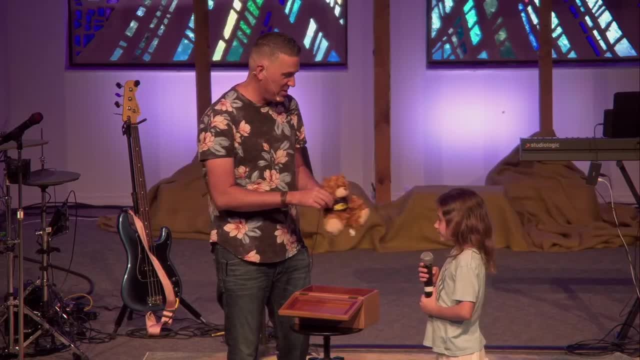 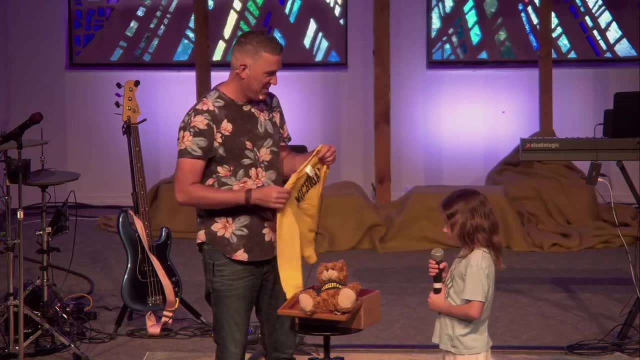 And that's something that we're not allowed to do when it comes to things. So, what's it say on the teddy bear? Michigan? It says Michigan. And then what is this? A sweatshirt, Yeah, So oh, and there's something else in here. 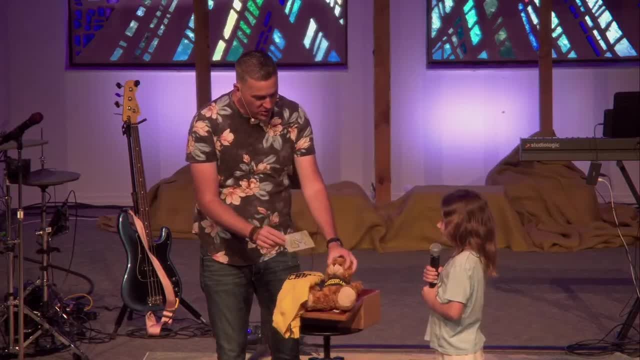 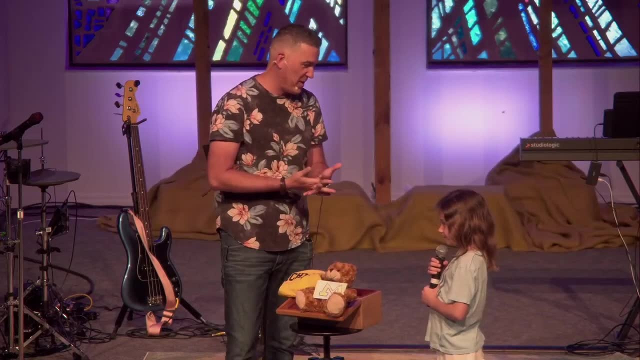 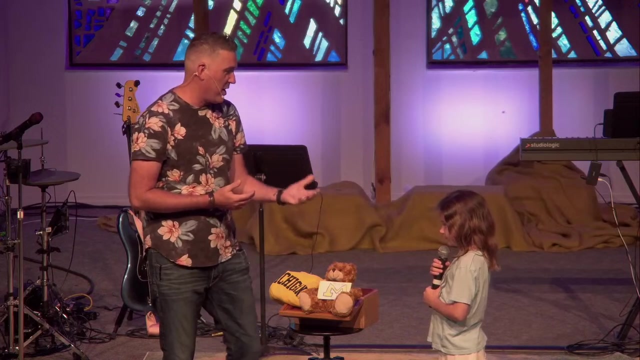 Who wrote who made this? I did, I did All right. Well, the good news is, the truth can set you free, And today our message is on forgiveness, And that's gonna be the heart of our message. And so, when I was about your age, 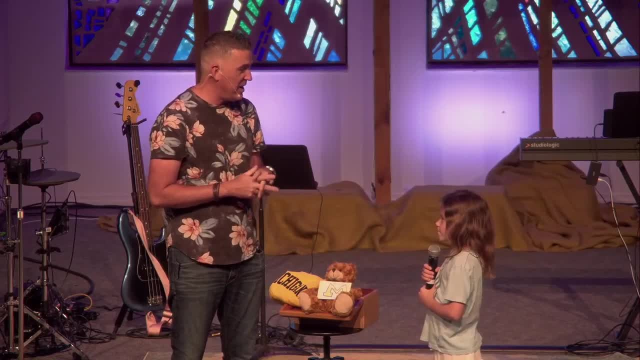 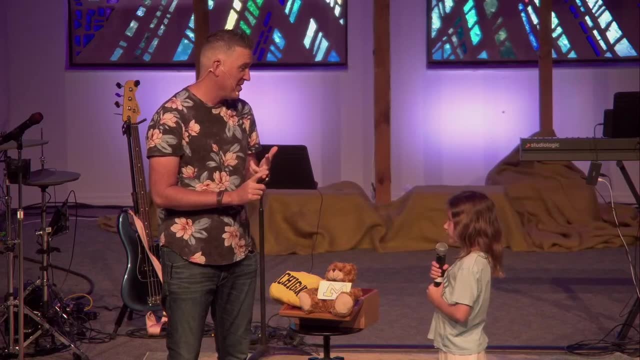 I went and I asked my dad a question and I said, dad, can you be a Michigan fan and love Jesus, And what do you think? he said Yes And he said no. Why? Yeah, I'm pretty sure he was kidding. 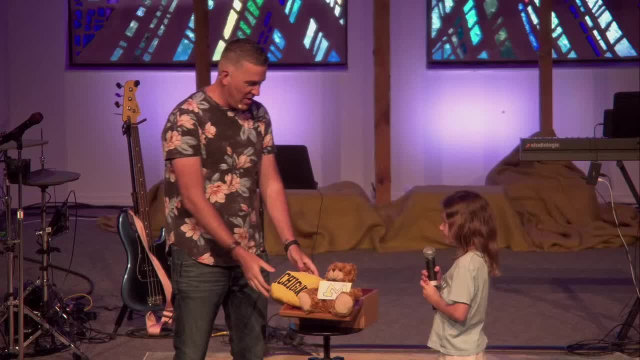 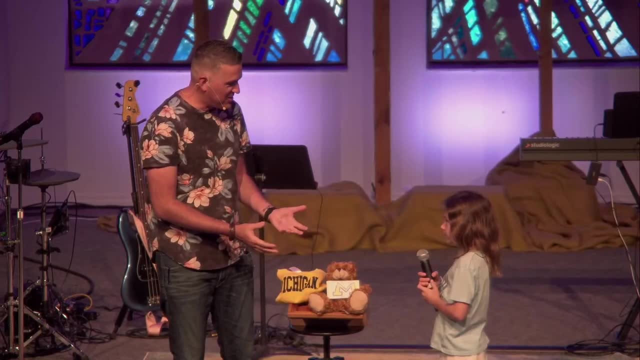 Maybe I'll ask him later this afternoon, And so, all right, what do I do with this? All right, I should have thought of this beforehand. So my question is: did you decide to put this in here, or did your dad put you up to this? 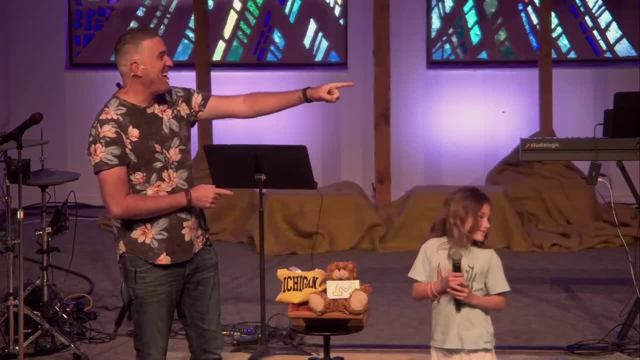 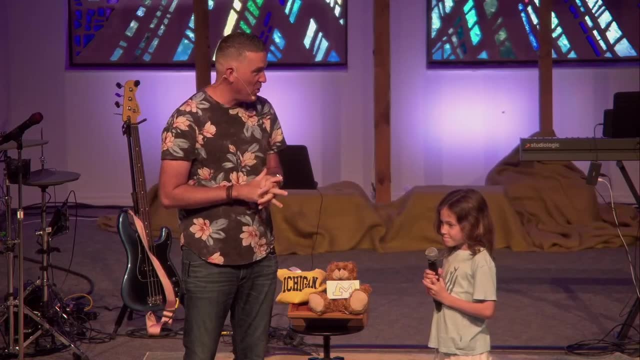 Oh, that's it. She gave it away. She gave it away. That's awesome, All right. so whatever he's bribing you with, I'll double it if you wear an Ohio State shirt to church next week. No, No. 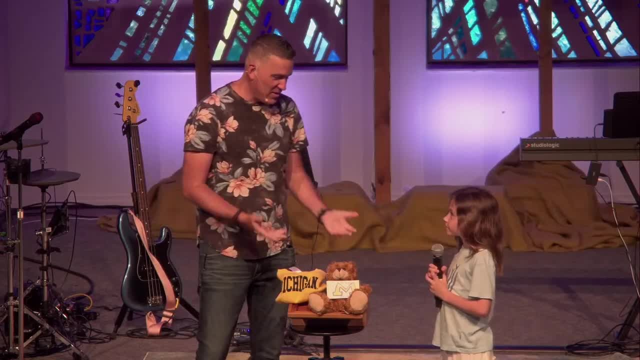 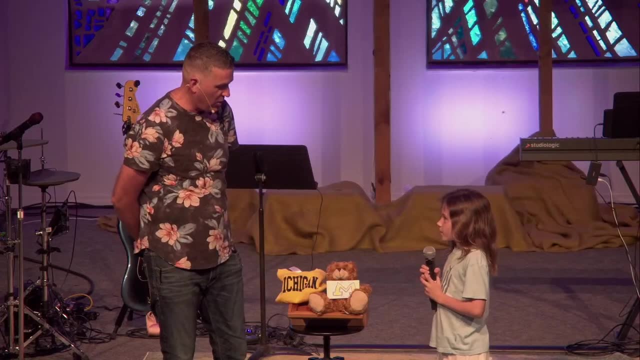 All right, Okay. Well, Kinsey, let me ask you: what message about Jesus or the Bible or God do you want to share with all of the stuff that you put in the brown box? That God loves Ohio State? That God loves Ohio State. 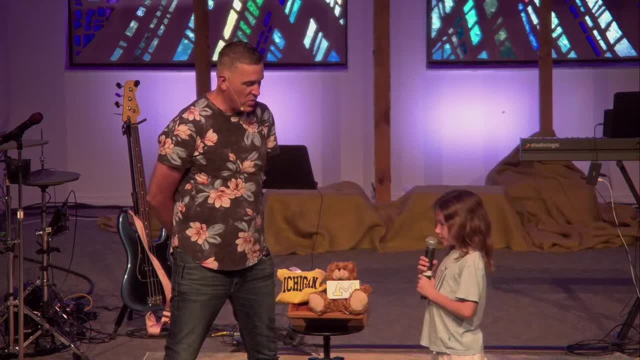 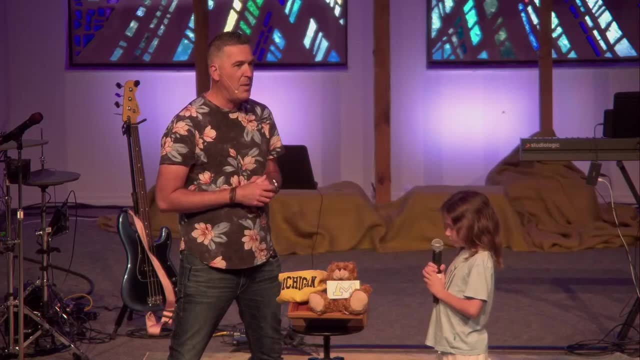 Yes, I like it, I like it, And so the reality is. I think what we can talk about is, as a church, is that we've recognized that we have fun. How many people are Gator fans here? All right, we got a lot of Gator fans. 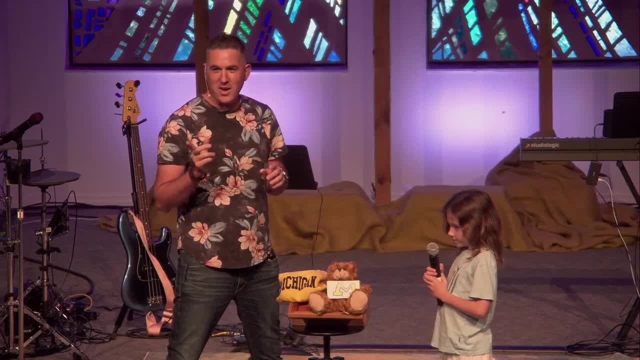 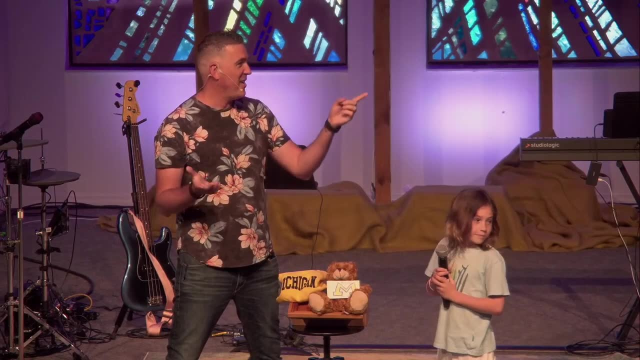 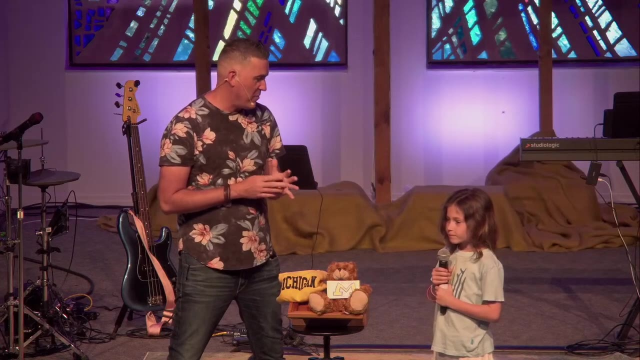 Do we have any Seminole fans here? All right, A lot less Michigan fans. Who else is a Michigan fan? All right, we got a few here, And then Ohio State fans. There we go, All righty. So, Kinsey, you know what I love about this. 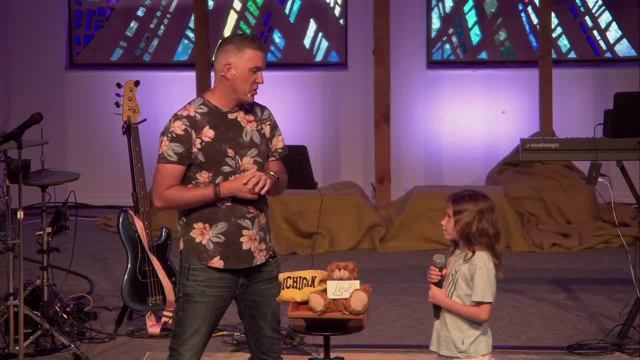 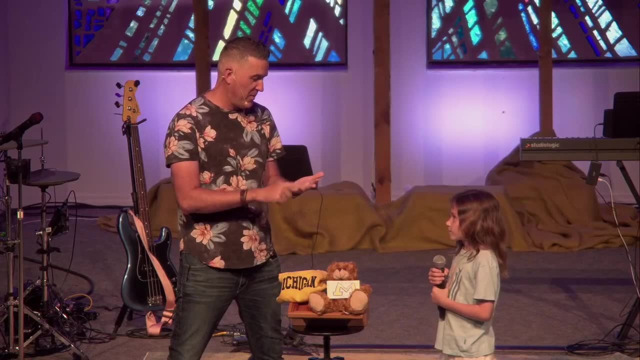 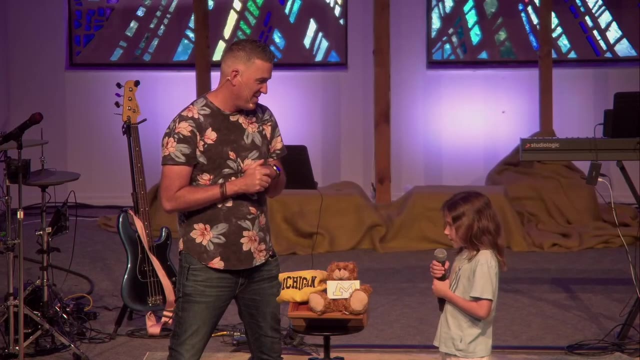 Is that this is the church that we want to be. We want to be the church that everybody can come together. because why are Gator fans, Seminole fans, Wolverine fans and Buckeyes? why are we all together, all in this place right now? To love God, To love God And to worship, And to worship. 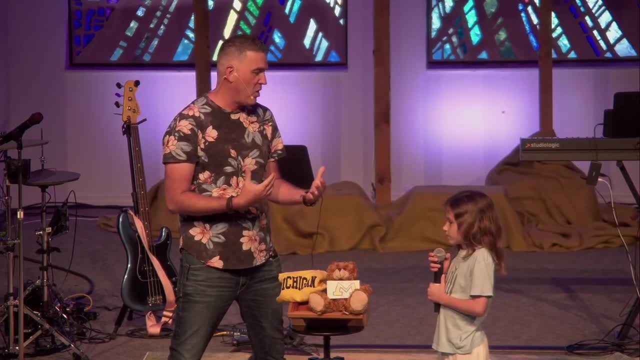 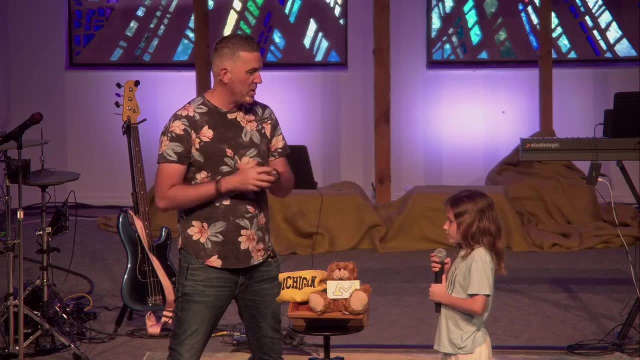 And so, even though we're having some fun with this, for me this is really the heart of who we are as a church. This fall there's going to be an election. I'm so thankful that we've got people who are voting in opposite directions that come together in our church. We've got 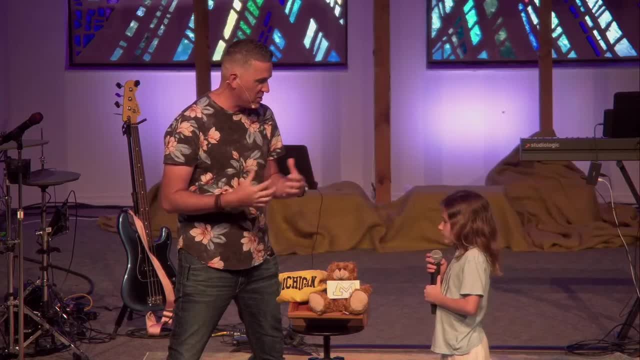 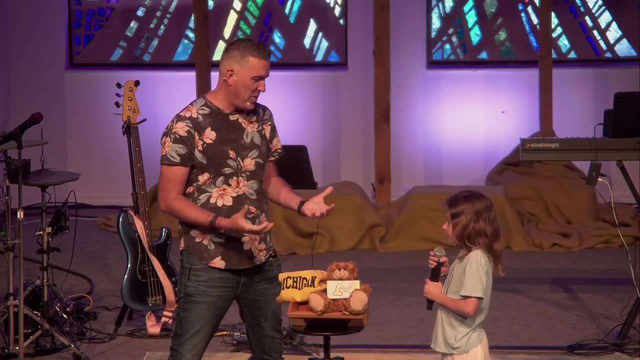 different people who have different passions and different priorities in their life and different things, And God calls us all in different directions, but we all come together because we love Jesus. right, Yeah, Yeah, And so I think this is actually a really fun thing to talk about. 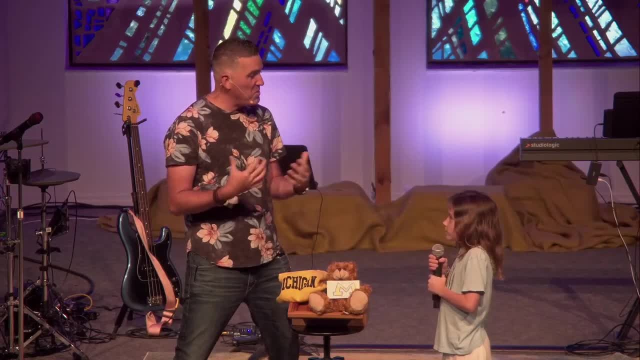 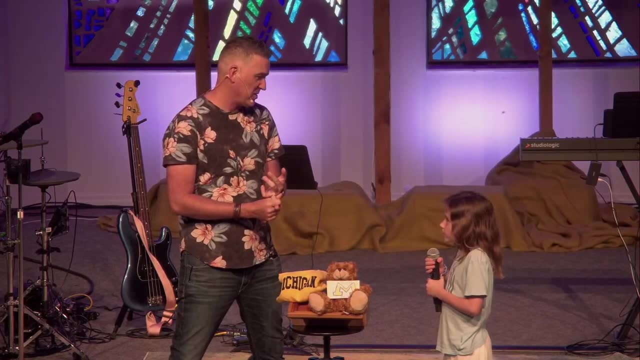 one of our core values as a church, And that is that we can all be different, We can all be unique, but we can all come together in God's word, God's truth and in God's love in Jesus. Does that work? Yes, All right, I won't ever forget this brown box. Kenzie, Can I pray with you? 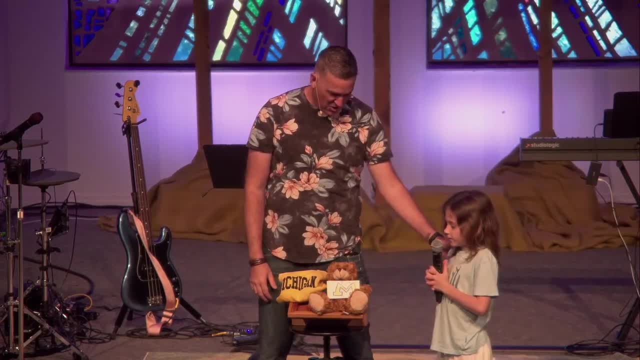 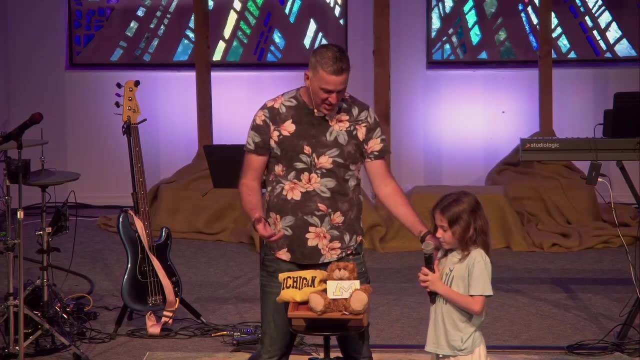 All right. Lord, we're so thankful for Kenzie. Lord, we're so thankful that she is made on purpose and for purpose. I'm thankful that she has a love for her dad, She has a love for her family and that she's. 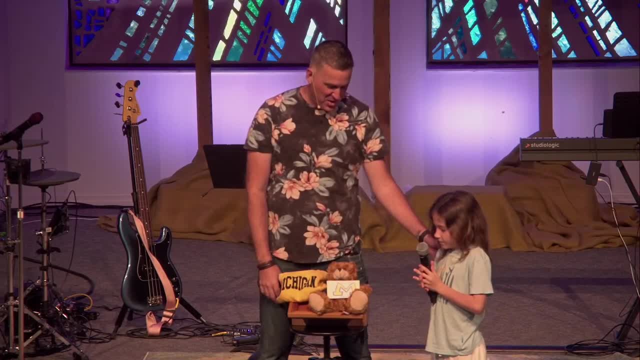 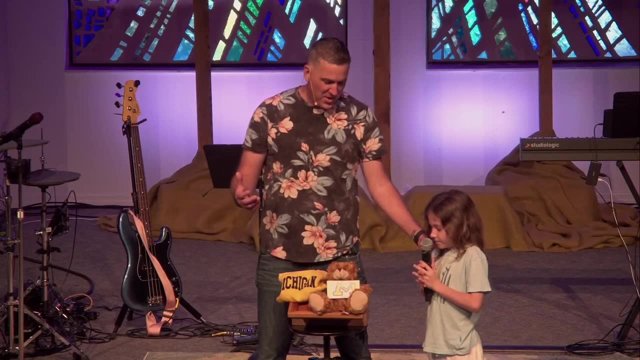 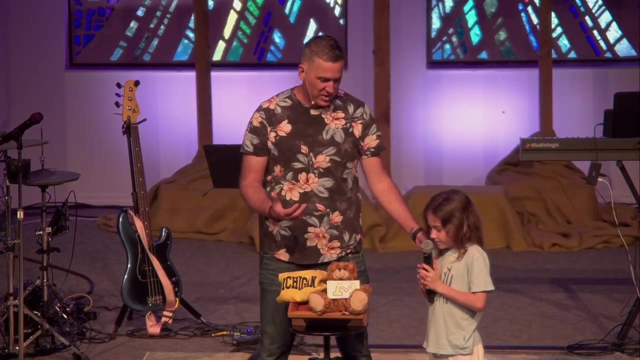 getting a chance to put that they love Michigan and the brown box, Lord, And we get a chance to understand that, God, that you call us all together and we all have different things that are unique about us, but we all can stand together on the truth of God's word and the love of Jesus Christ. 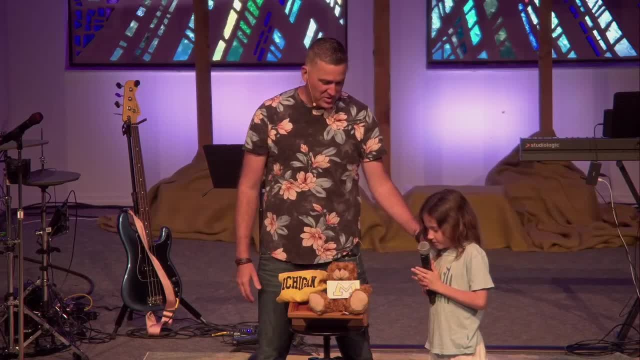 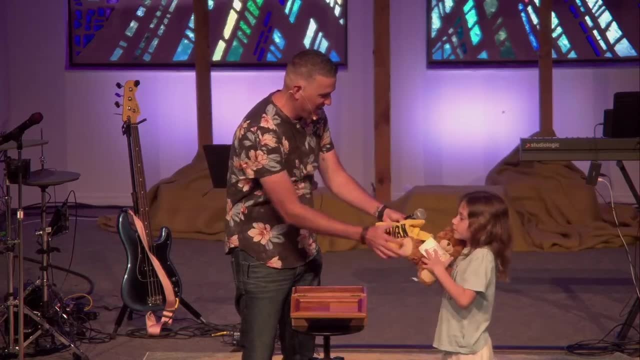 And that is the community that we can be known for, And so we pray this in Jesus' name: Amen. All right, Can I keep all this stuff? No, You want it back. All right, There you go, I'll let you have all that. 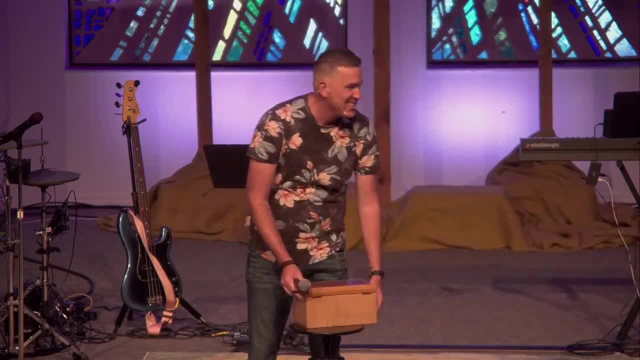 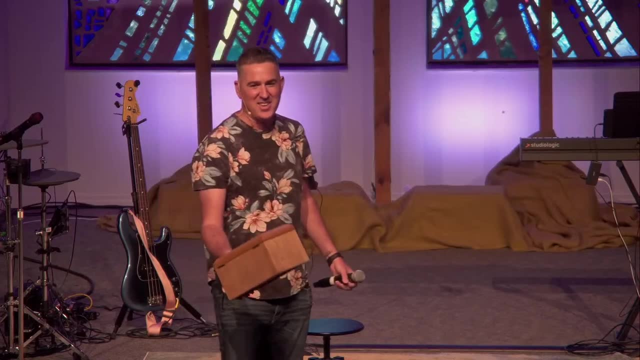 back. All right, And let's hear it for Kenzie. And that brown box is coming to Jack. There he is. All right, Jack, All right, We'll see that next week At this time we're going to invite all of. 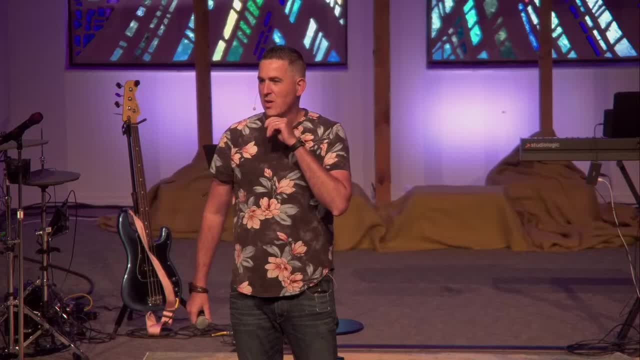 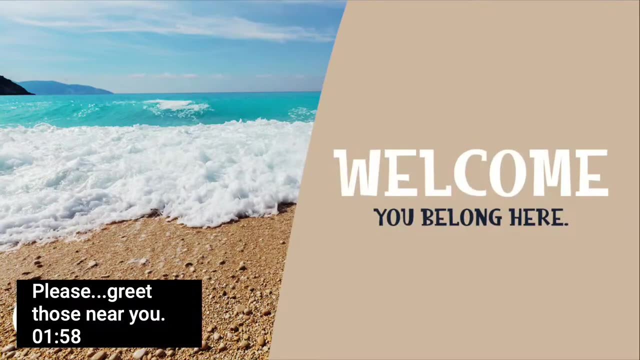 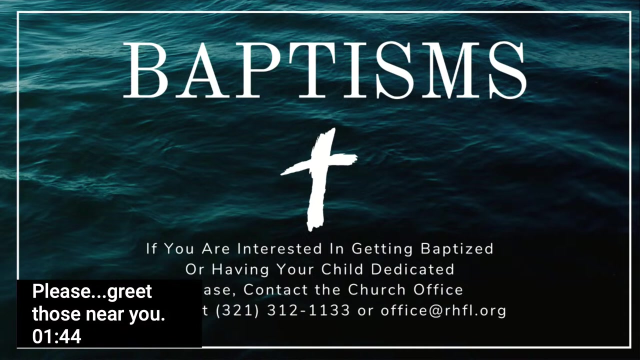 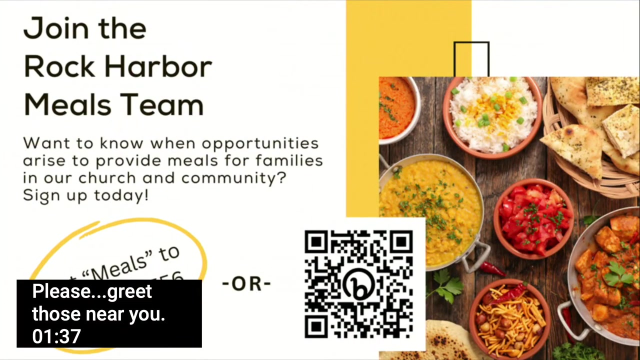 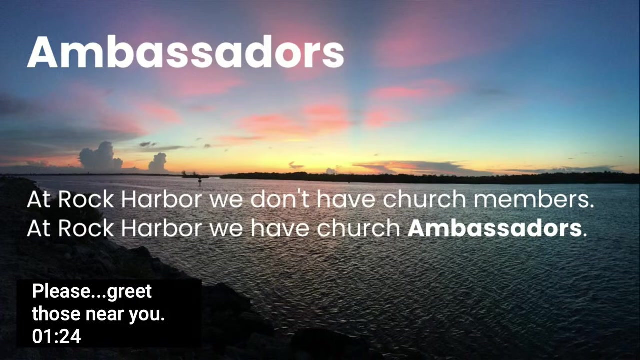 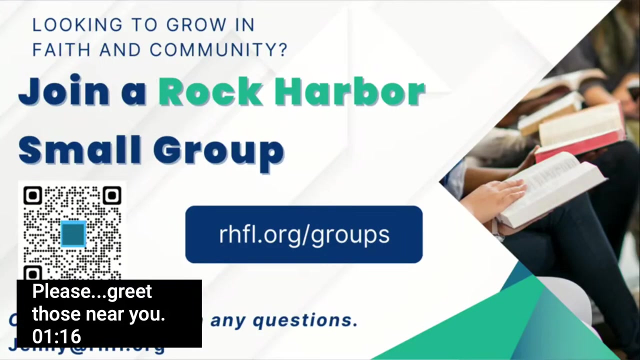 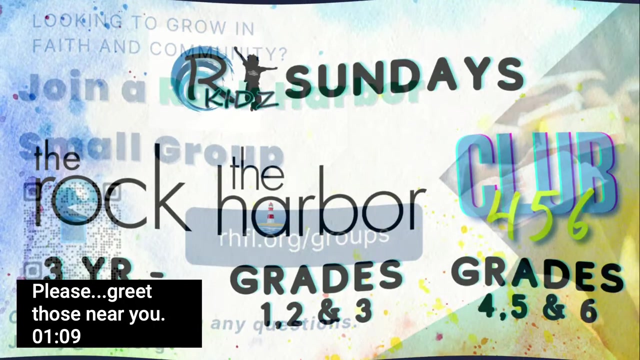 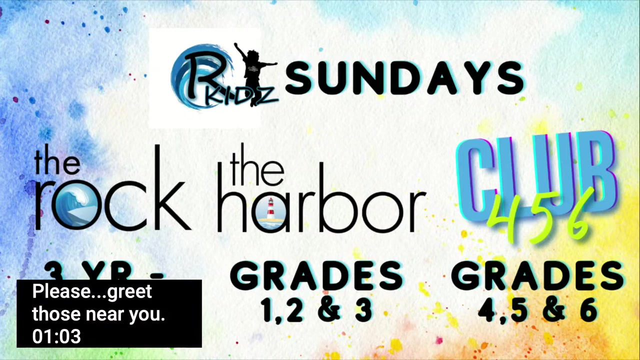 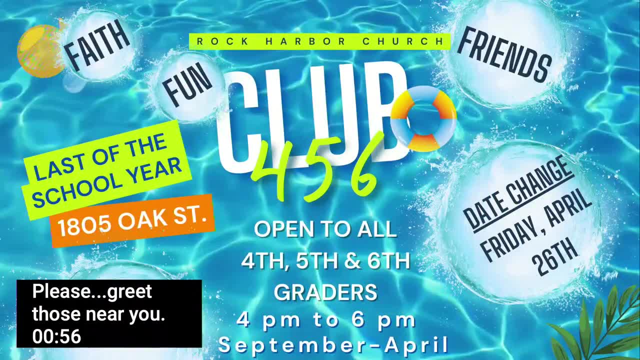 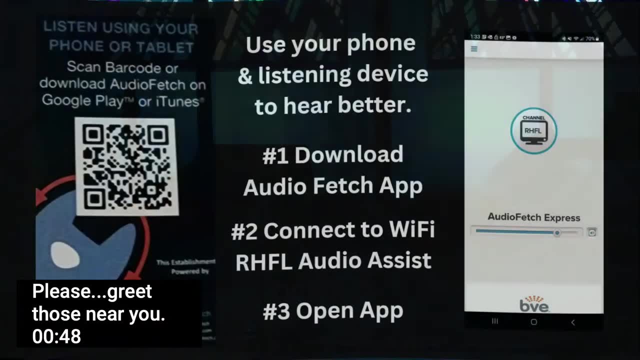 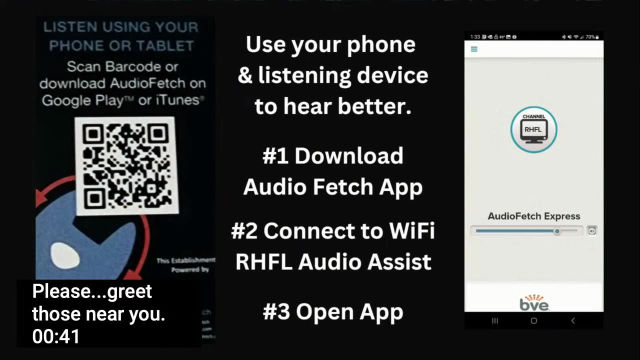 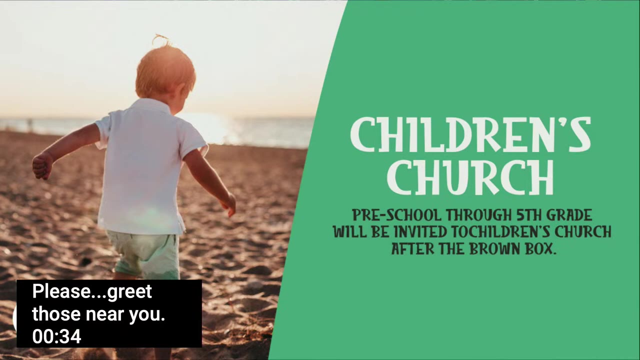 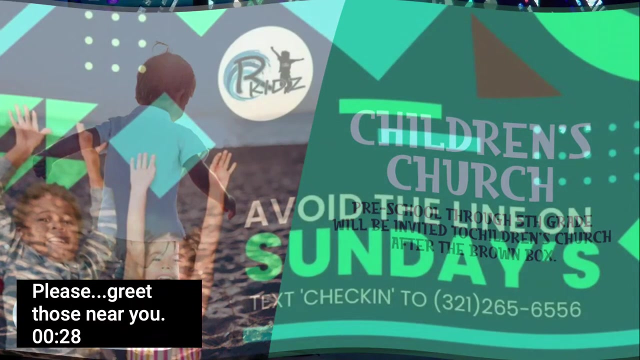 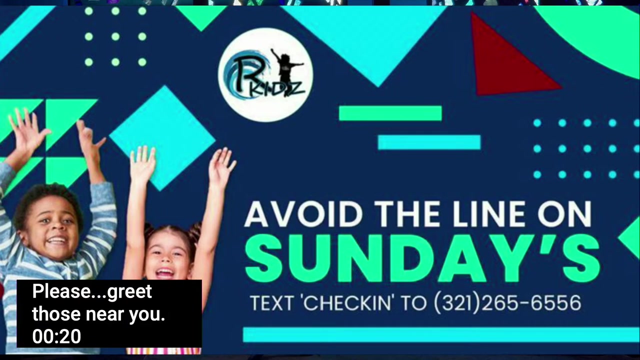 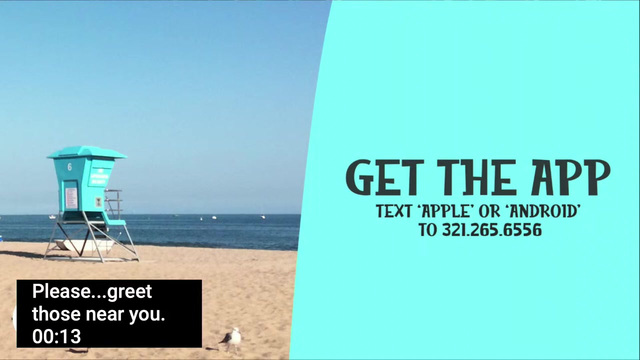 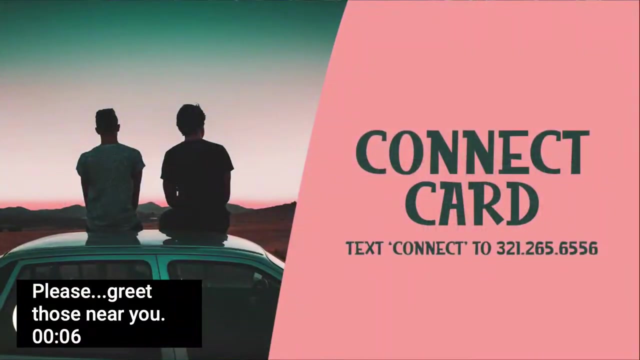 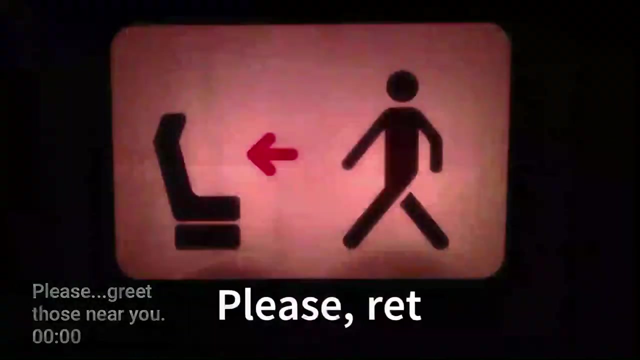 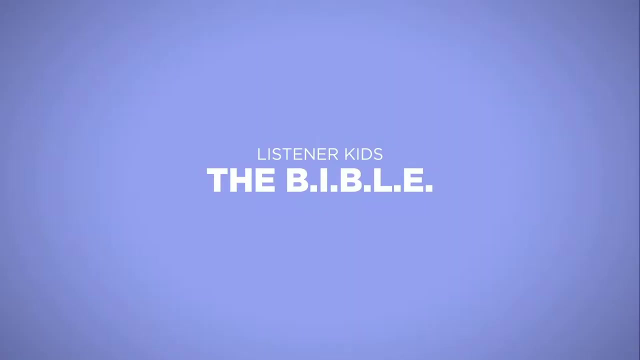 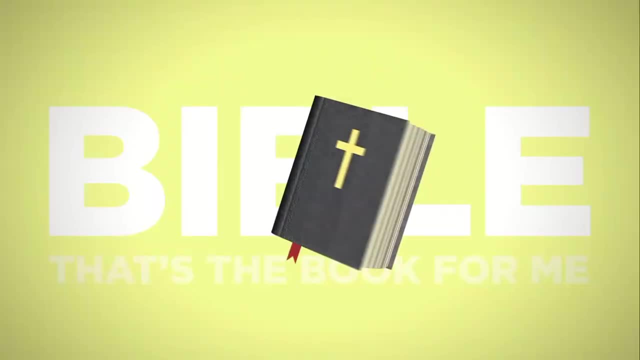 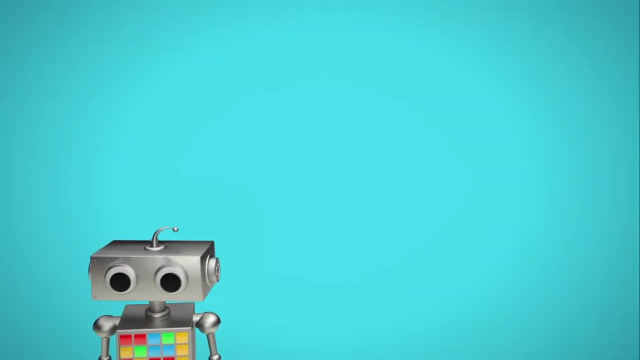 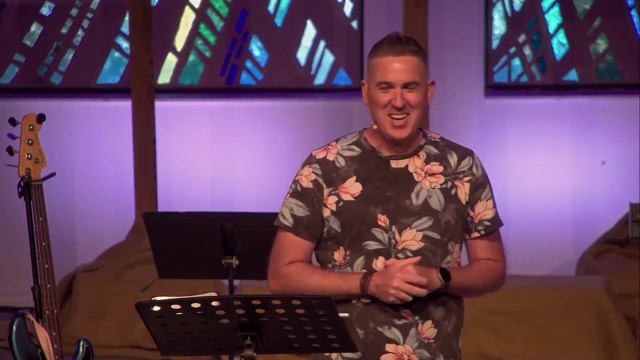 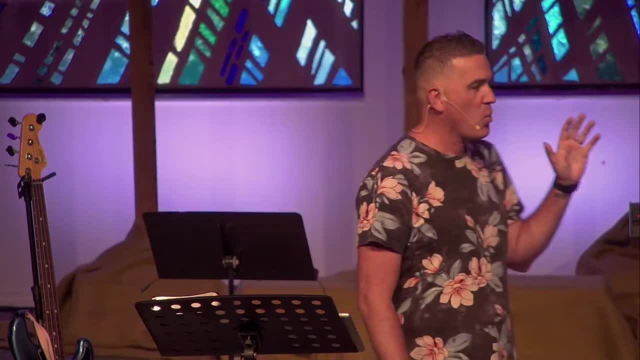 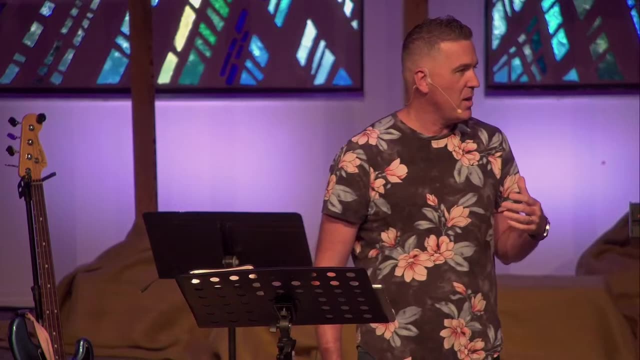 second week. This is only a two-part series. Next week we're going to go to a series and it's going to be called God Is, And we're going to really look at the character of God and the relationship that we can have with God through Jesus, And so we're going to do that through the second half. 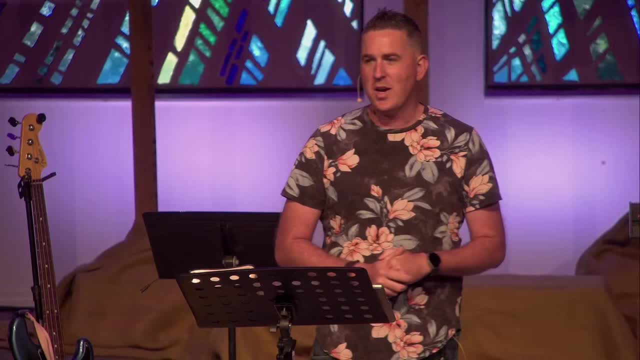 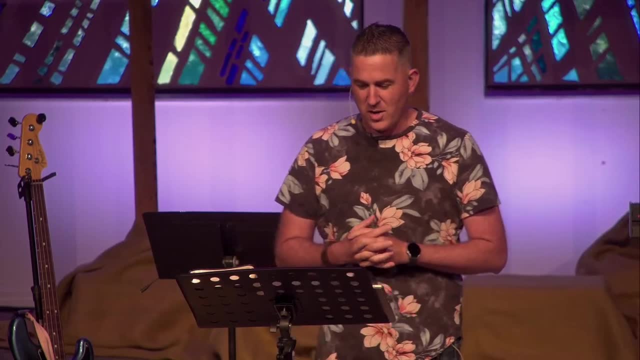 of April into May. But we are in this second week So we're going to kind of dig a little bit deeper. So last week was the beginner class, This week is going to be kind of the next level, mastering the art of studying the Bible, And really between these two weeks there's so much. 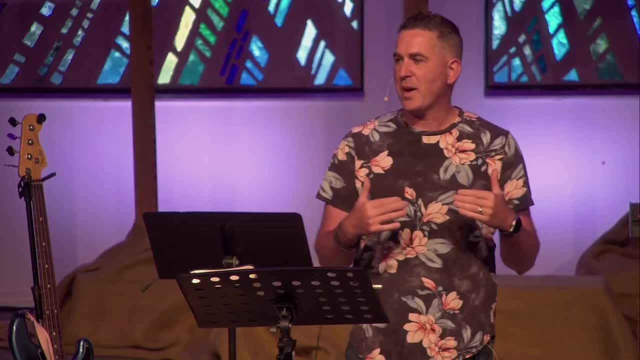 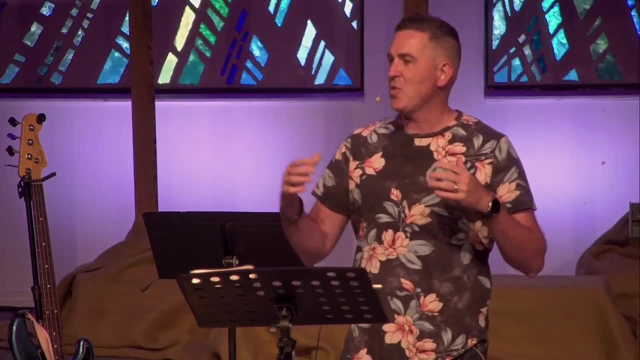 content in just last week and this week that I don't expect you to comprehend all of it right now, And so later on I'll give you a website you can go to And I'm trying to give you the tools. This is the whole like: don't feed the fish, but teach them how to fish. 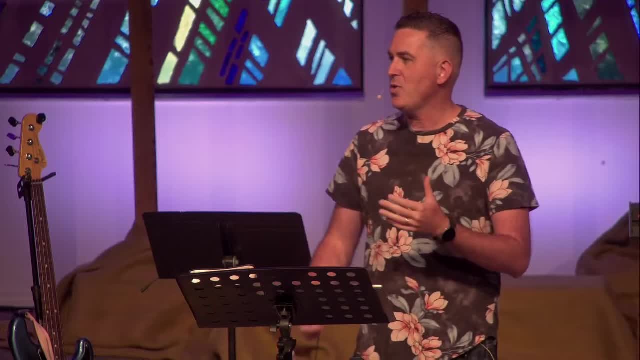 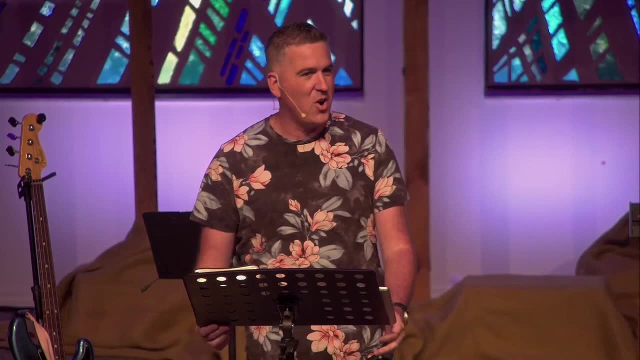 That's what we're trying to do with the Bible, is we're trying to teach you how you can use the Bible in your life in a way that can be transforming. So we're going to go back to where we were on Easter morning one more week. John, chapter 1, verse 1.. 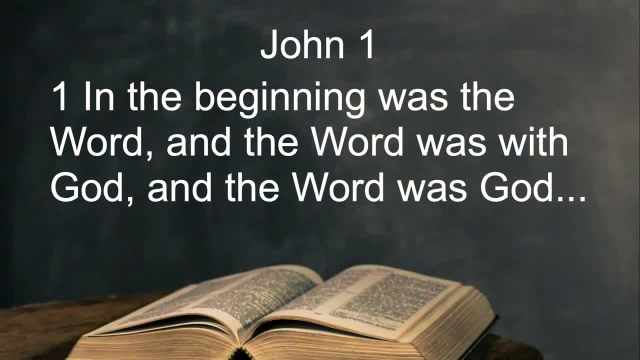 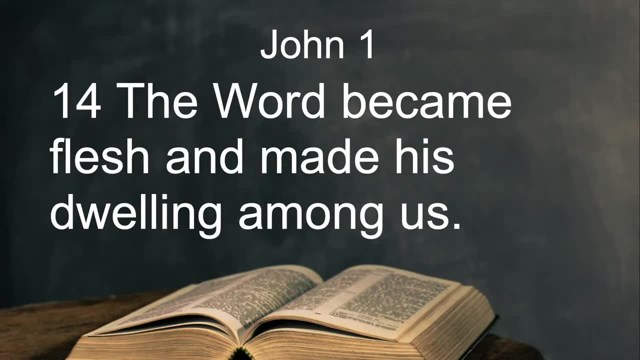 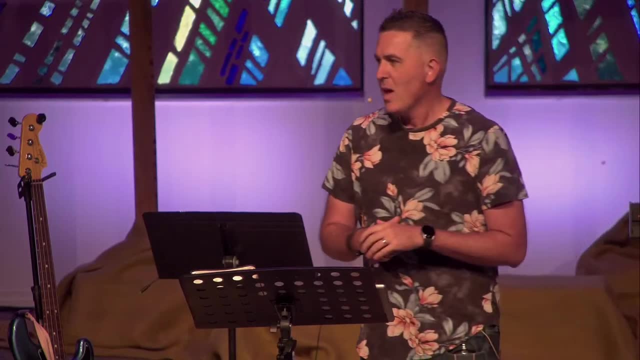 In the beginning was the Word, and the Word was with God and the Word was God. And then verse 14 says The Word became flesh and made His dwelling among us. So I love how John goes back and has that phrase in the beginning, But I actually wanted to also draw our attention back to the very beginning. 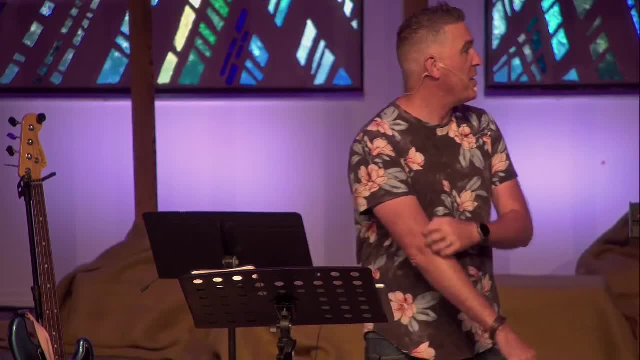 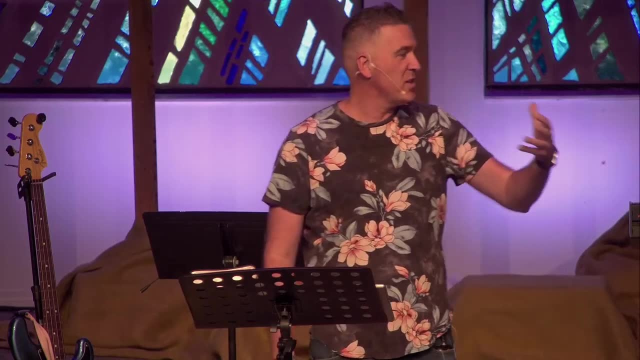 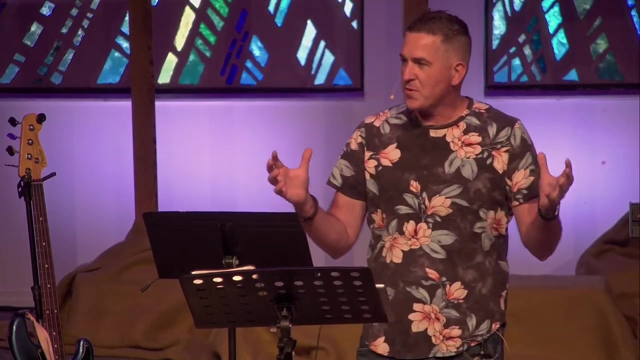 of the story back in Genesis 1.. And then it said: And God spoke. and He said: Let there be light, And the light shone in the darkness. And we can see that When God spoke, He spoke, And the waters were separated, The earth was formed, He spoke. 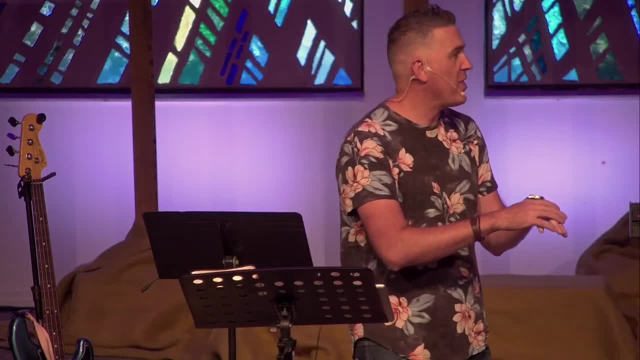 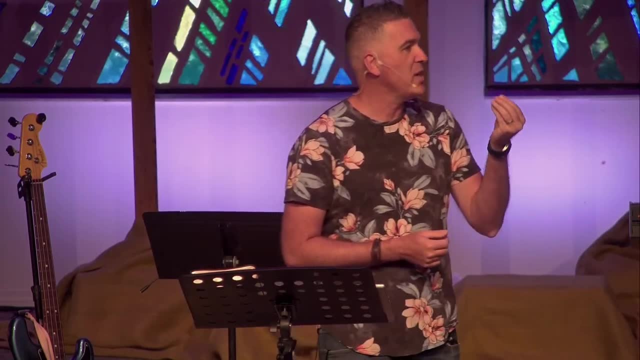 And the animals came into existence. He spoke. And there was fish in the sea, He spoke, And when He spoke there was birds in the air. And then He spoke and He dwelt down and He breathed His life into His image And He made us. 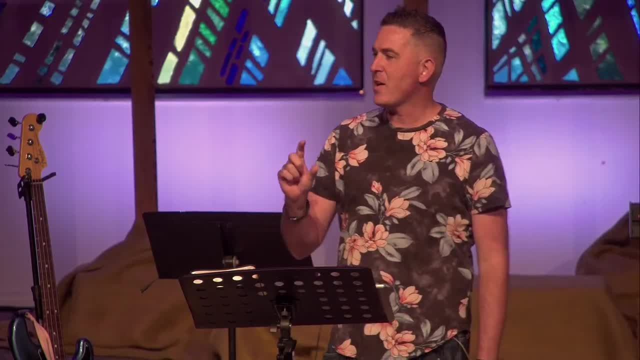 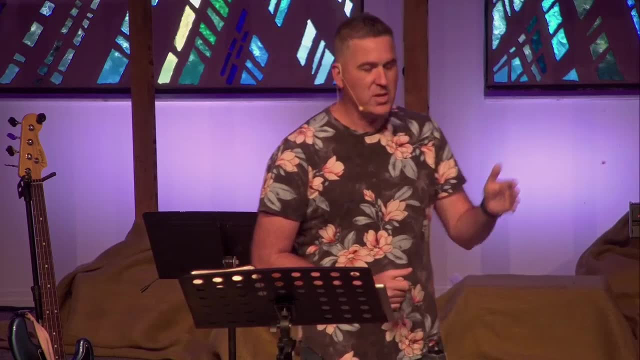 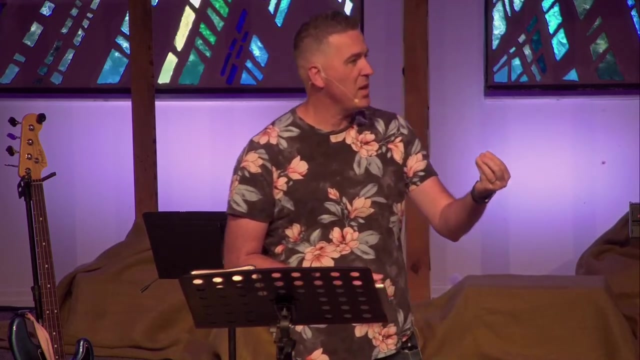 man and woman in His image, That the very power of God came when God spoke. He spoke the universe into existence, The single spoken sentence, And that through the power of God, through the power of God, speaking was the essence of His creation and His power. I'm trying to draw your attention. 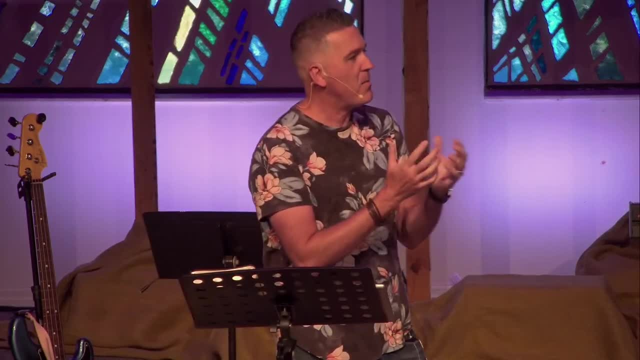 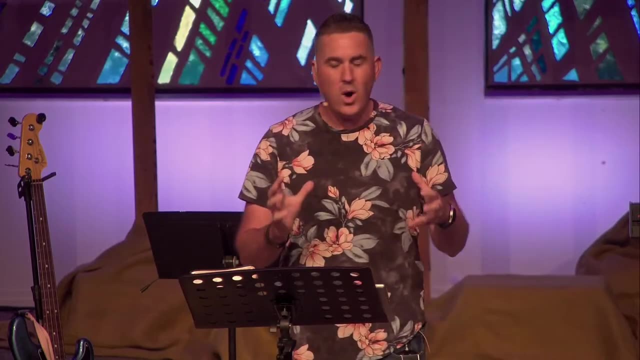 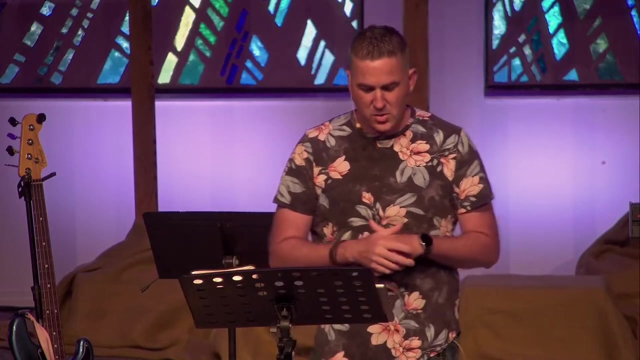 to understanding the power of the Word of God, The power of the Bible that we have, That God spoke all of this into His Word And it is the one thing that will continue into eternity is God's Word, and our soul will exist into eternity. The Word isn't just something for the beginning. 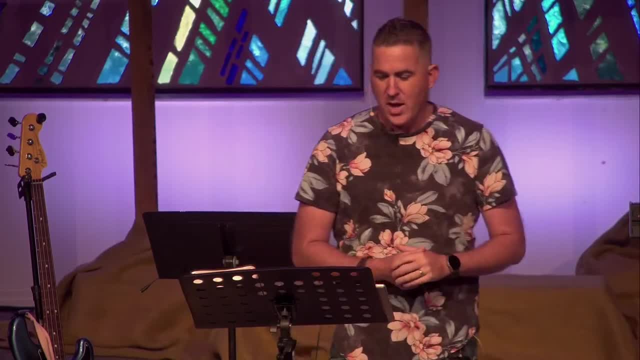 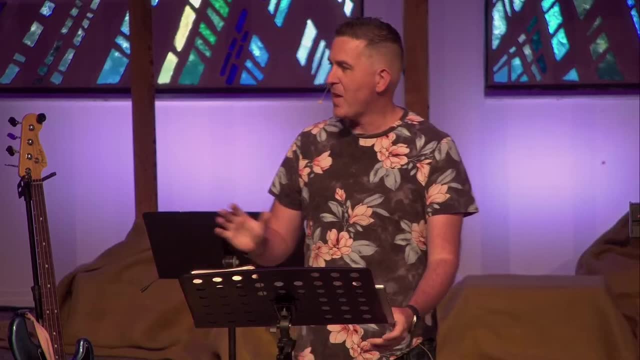 But last week we saw the Word of God come into existence And we saw the Word of God come into all that. the Word is part of our daily bread. It's something that we can use for every single day of our life. And 2 Timothy is the famous scripture on the power of the Word of God, where it says: 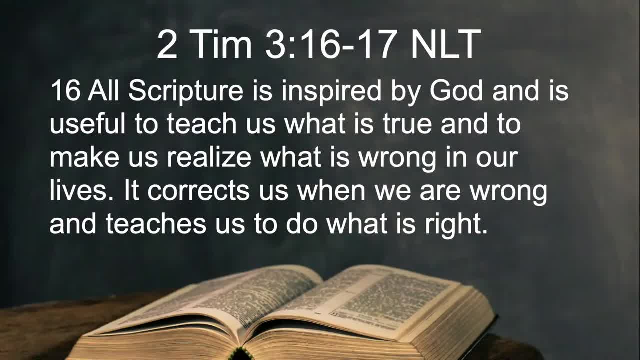 all scripture is inspired by God and is useful to teach us what is true, to make us realize what is wrong in our lives. It corrects us when we are wrong and teaches us to do what is right. God uses His Word to prepare and to teach us what is right, And that's what we're going to learn in this. 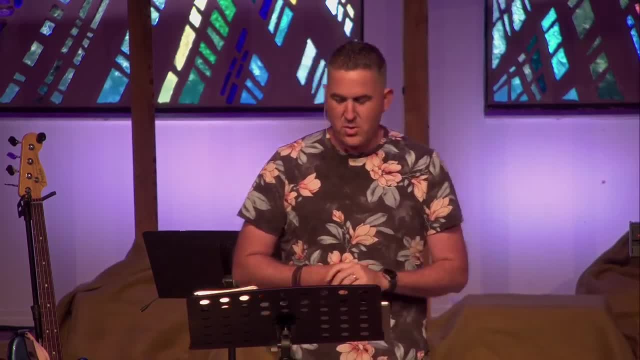 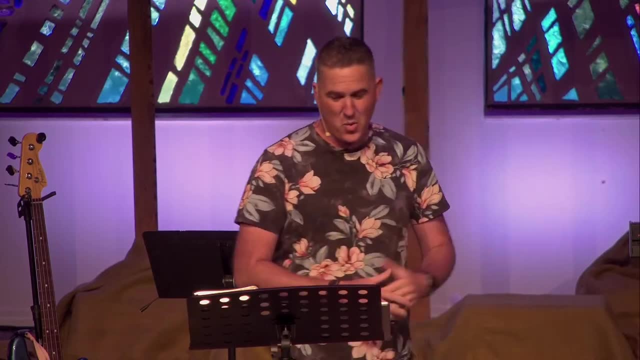 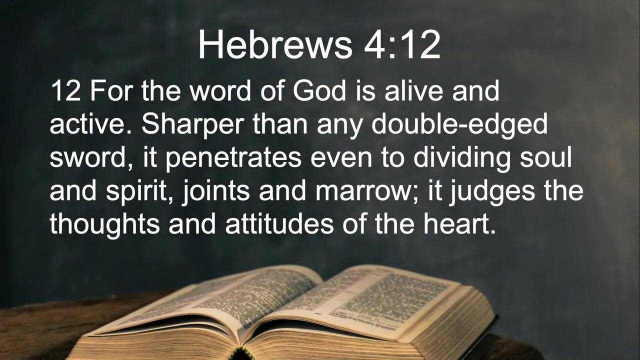 book. I want to open up by sharing with you how the inspired Word of God speaks of the Word of God We can see in Hebrews 4, where it says: For the Word of God is alive and active. sharper than any double-edged sword, It penetrates. 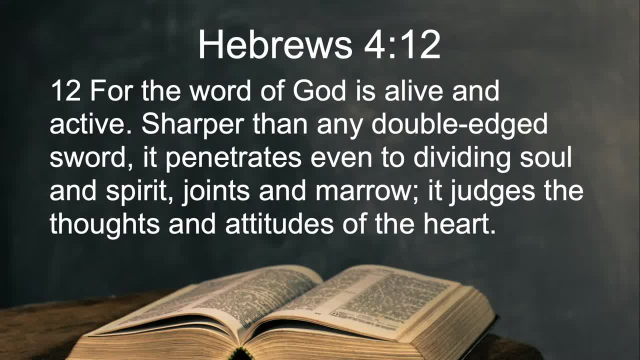 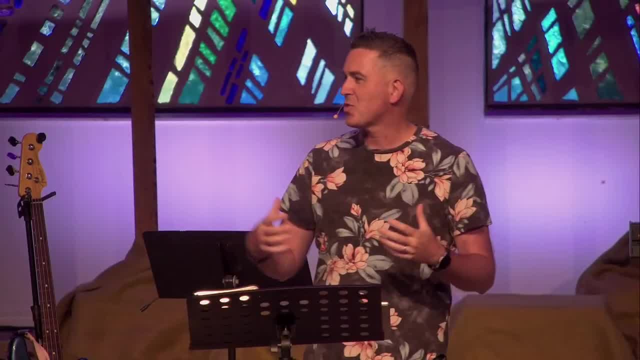 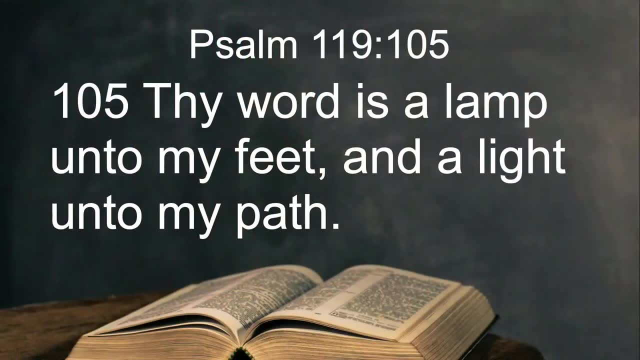 even to dividing soul and spirit, joints and marrow. It judges the thoughts and attitudes of our mind. The word of God is the sword that pierces. Psalm 119 says that, for thy word is a lamp unto my feet and a light unto my path. 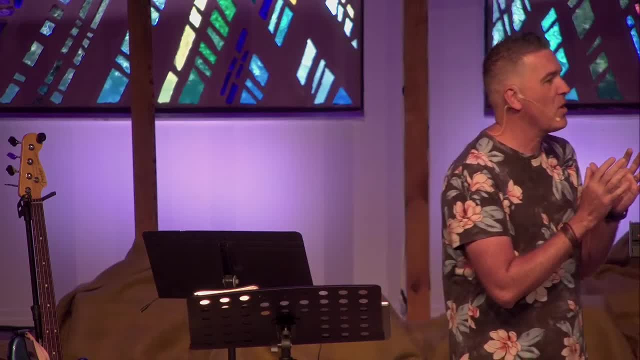 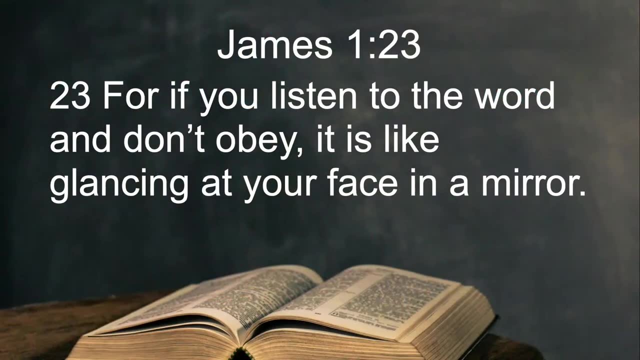 It is the light that shines in the darkness and can give our entire life direction. In James it goes back to that mirror language we just heard in Timothy, For if you listen to the word and don't obey, it is like glancing at your face in a mirror. 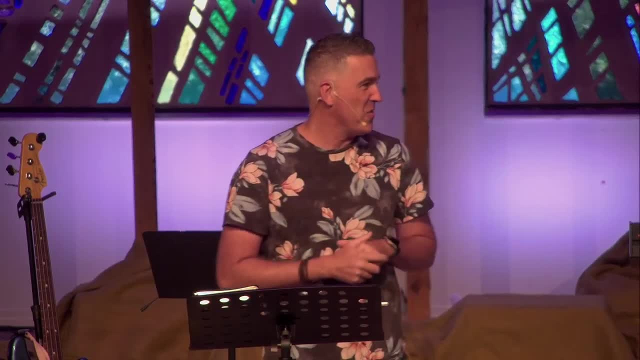 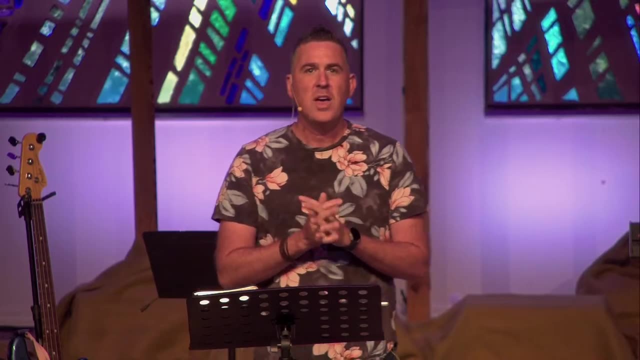 It allows you to see where you've got gunk: all over your face or all over your soul and all over our lives. We see in 1 Timothy 4, it says: if you explain these things to the brothers and sisters, Timothy, 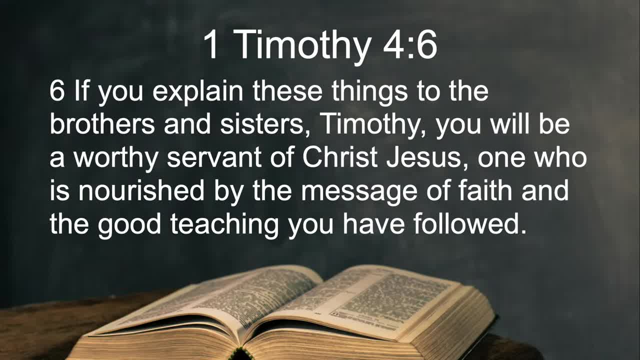 you will be a worthy servant of Christ Jesus, one who is nourished by the message of faith and the good teaching you have followed. We wanna be a church and we're so thankful. We're thankful for the amazing worship we get each and every week. 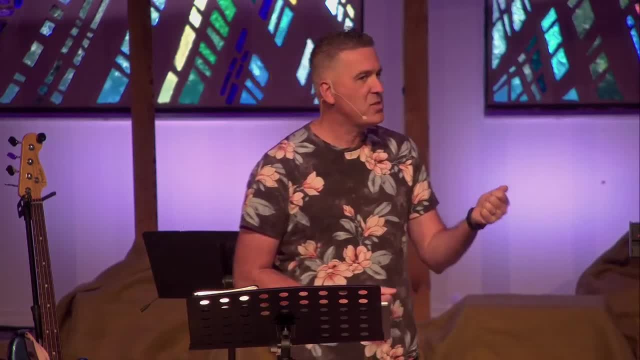 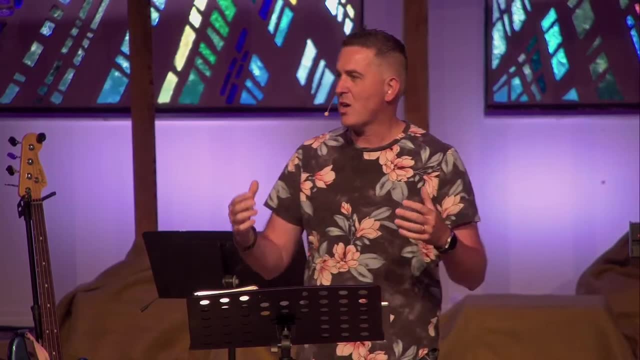 but we also wanna be nourished by the message of faith and the good teaching. That word, good teaching, is sometimes translated as doctrine. You'll hear churches talk about doctrine, and that means that what we teach, what we preach and what we believe. 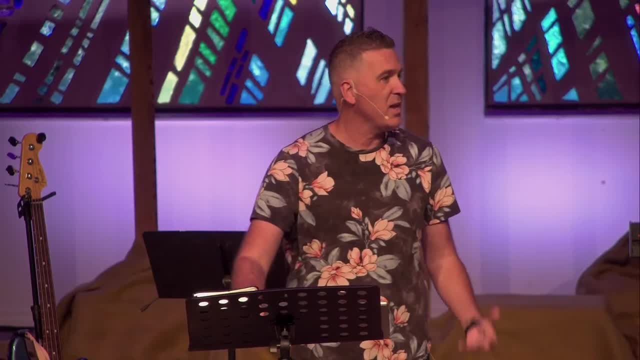 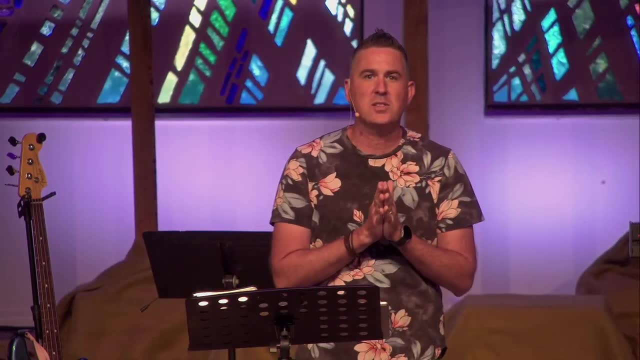 has a foundation in the word of God. It is not a preacher's opinion, but we are gonna teach God's word. 1 Peter 1.23 says: you have been born again, but not to a life that will quickly end. 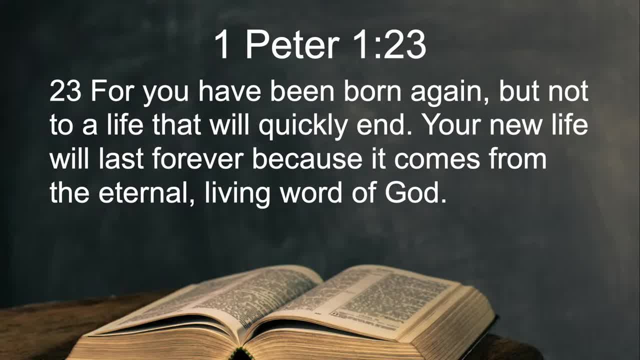 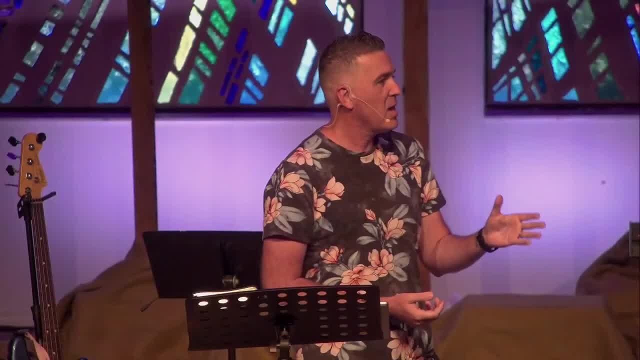 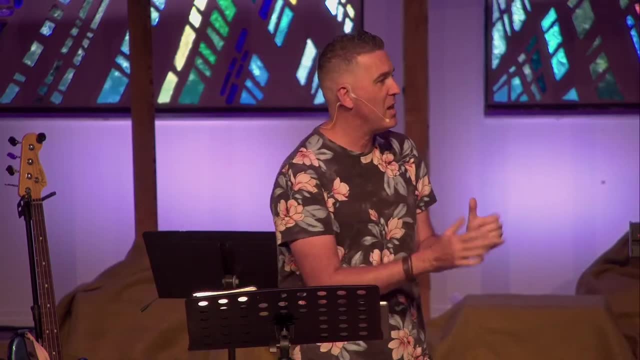 Your new life will last forever because it comes from the eternal living word of God. There are two things I said that will always exist, and that is that your soul will live on to eternity and the word of God will exist That even after the second coming of Christ. 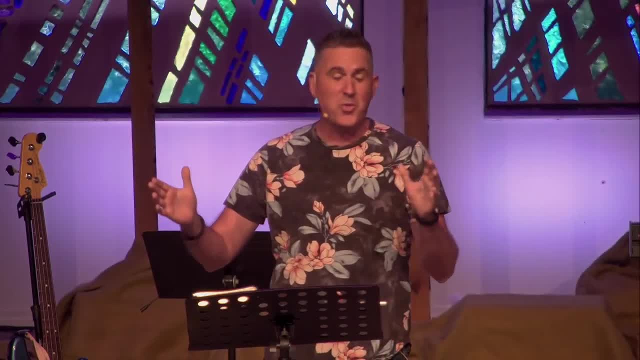 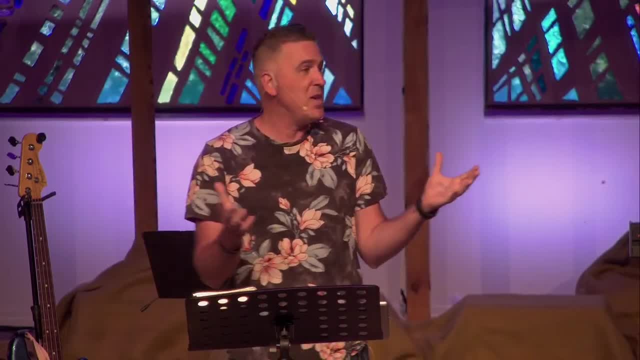 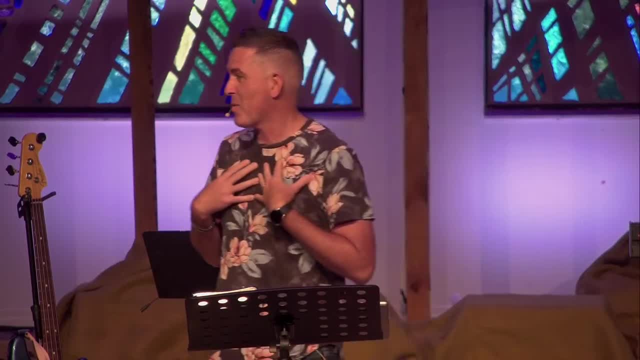 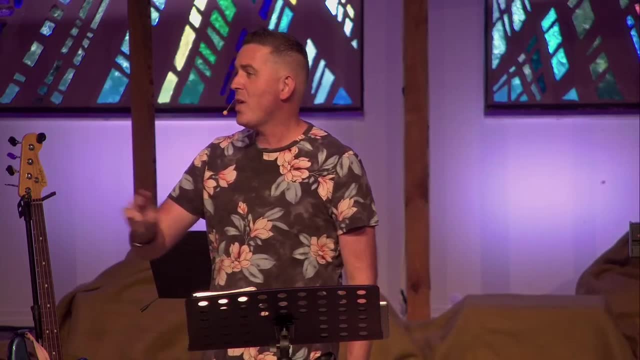 but what I know is that God wants us to be ready. We never know the time or place. It will come like a thief in the night, and that God wants us to be ready, but I do know this: The two things that will exist through eternity. 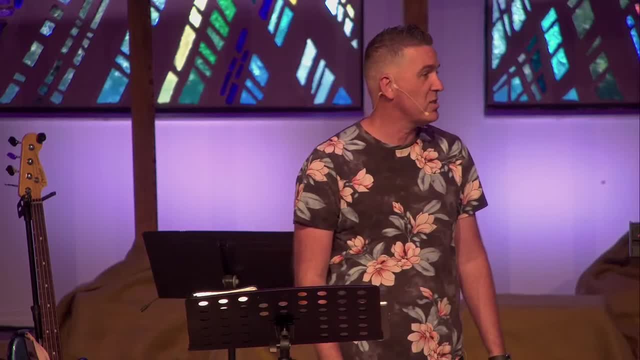 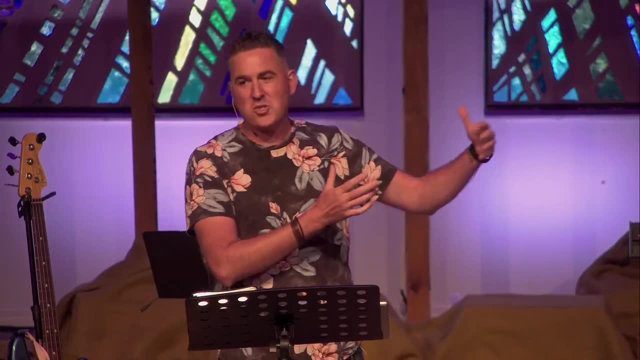 is your soul based upon your relationship with Jesus and the word of God That even when all the Bibles have been, you know the earth has been destroyed, there'll be a new heaven and a new earth. that everything that God has said in his word. 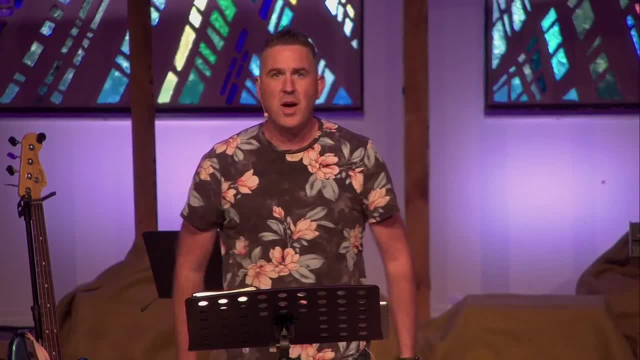 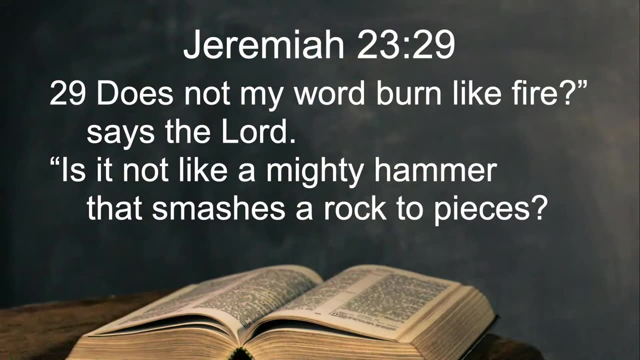 will still exist in eternity. Jeremiah 23 asks the question of: does not my word burn like fire, says the Lord. It is not like a mighty hammer that smashes a rock to pieces, And what Jeremiah is telling us there is that the word of God is a fire that consumes. 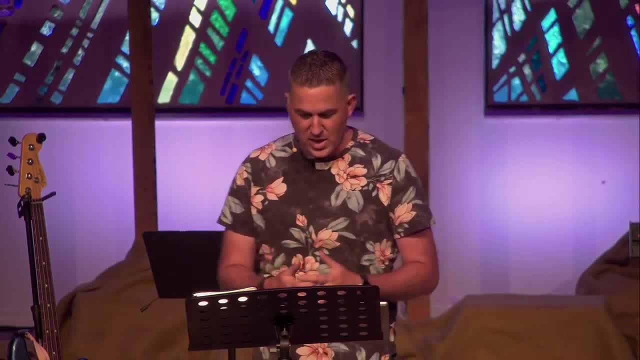 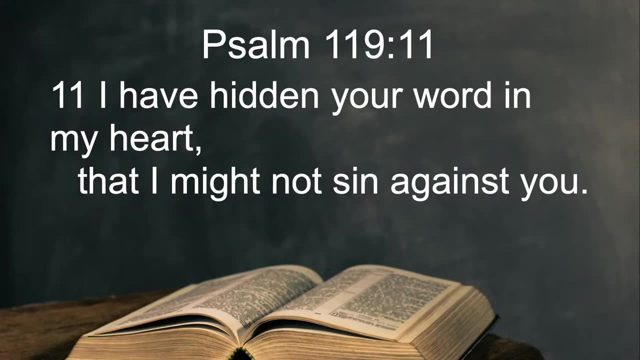 that we want it to consume our lives. It's a healthy thing that we desire. And then Psalm 119 says: I have hidden your word in my heart that I may not sin against you. Do you know that? knowing God's word, starting your day with God's word, 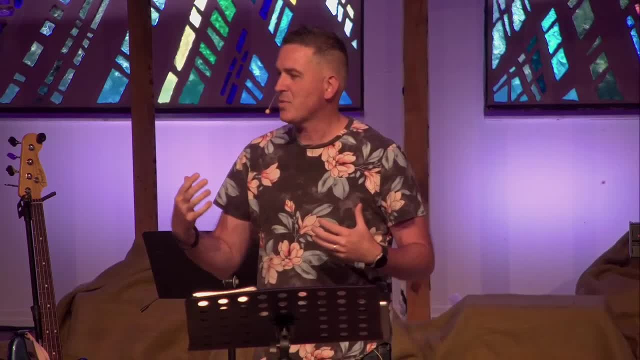 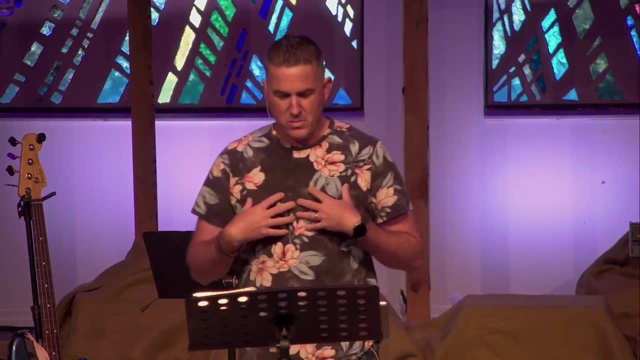 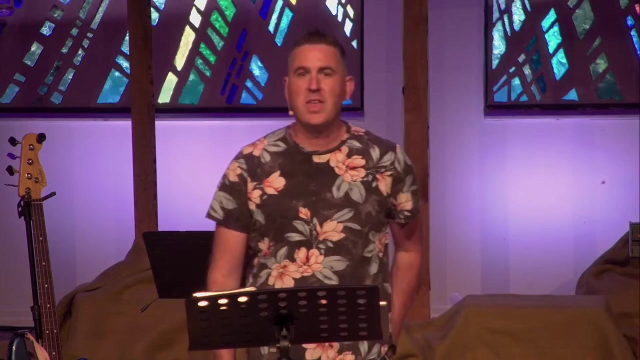 memorizing Bible verses that you can use in times of struggle, that you can have a defense against temptation, a defense against troubles, by knowing God's word in your heart. Romans 10 tells us that so faith comes from hearing, that is, hearing the good news about Christ. 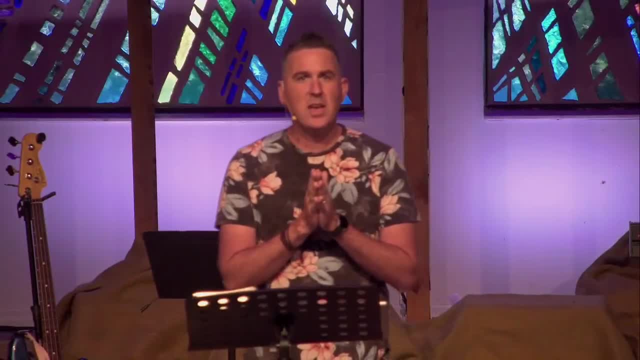 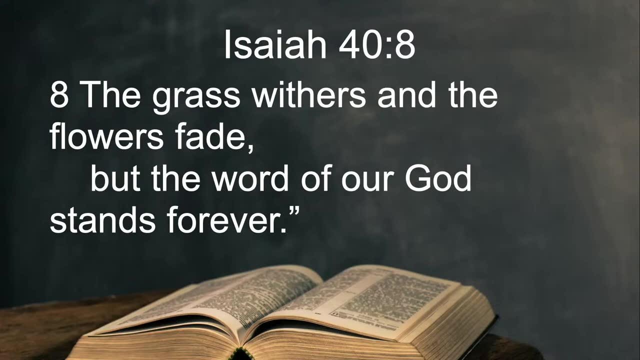 It's the source of our faith. And lastly, Isaiah says: the grass withers and the flowers fade, but the word of our God stands forever. And I will draw your attention Isaiah, which was hundreds of years before the birth of Christ. 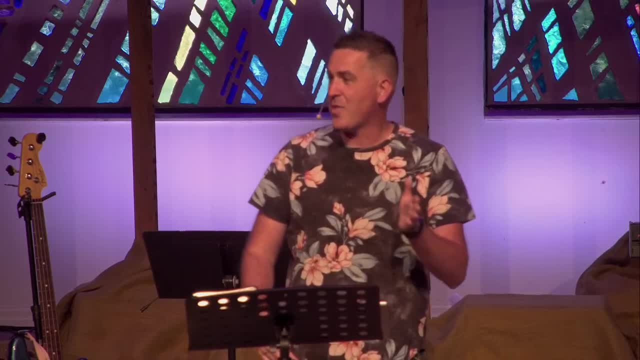 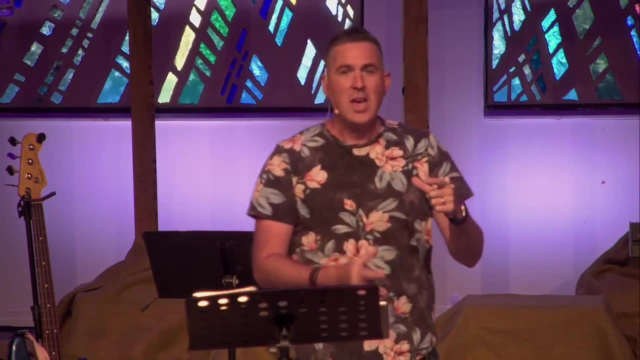 And then we've got 1 Peter that is written after the death, burial and resurrection, And the second ascension, the resurrection of Jesus Christ, are saying the same core teaching, And that is that the word of God stands forever. It's an eternal word of God. 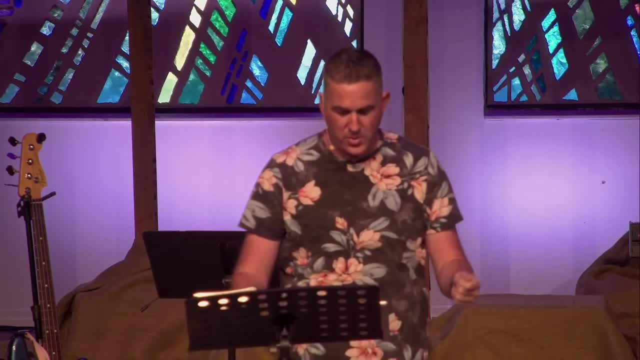 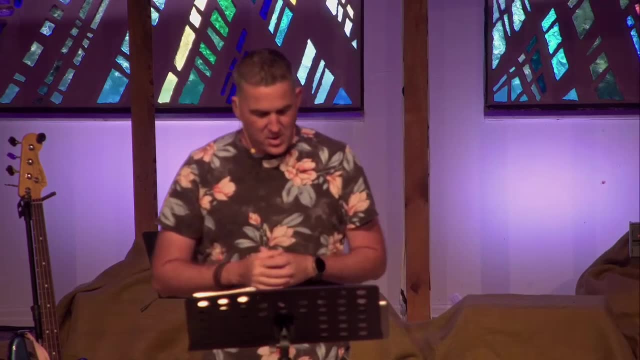 It's not a temporary idea, It's an eternal truth that is put before us. So today, as we open the word of God, let's also invite the spirit of God. So, our heavenly father, Lord, we come to you. We thank you that you are the word. 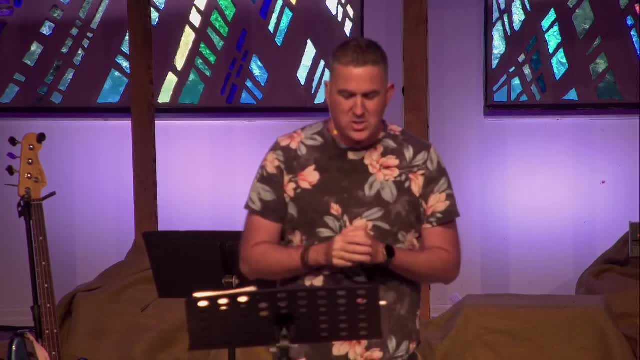 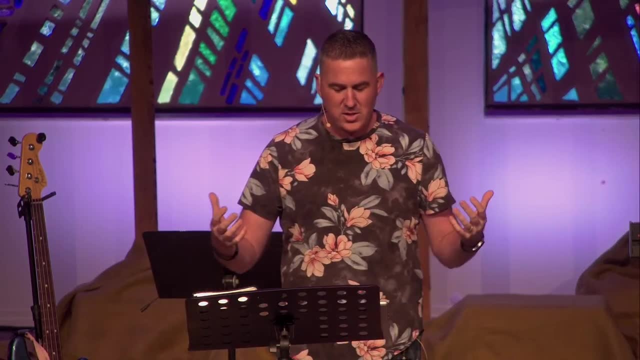 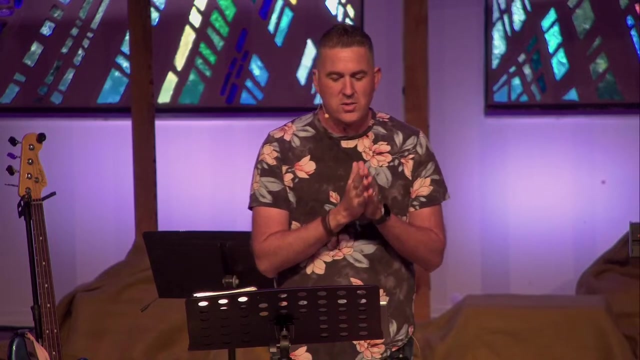 and the word became flesh. and the word made his dwelling among us And the person of your son, Jesus Christ. Lord, we're so thankful that Jesus was the living word and that, God, we pray that you would create in us a spiritual hunger to feed on your word. 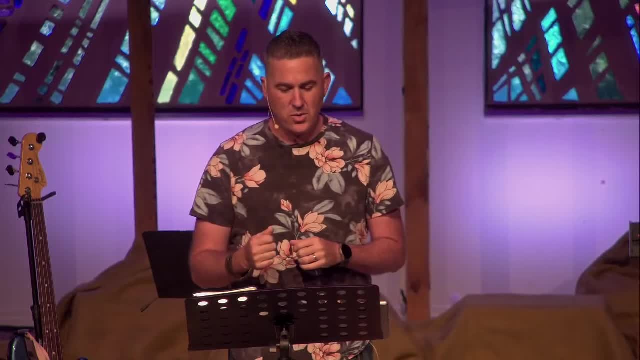 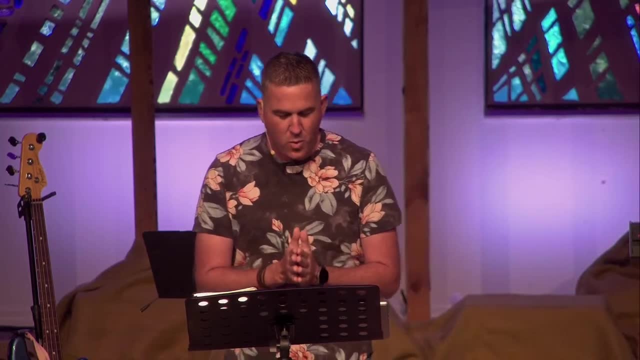 to know you through your word and to honor you and how we live by the power of your word that doesn't just inform us, but that it will also transform us to become like your son Jesus. So make us like your son Jesus. 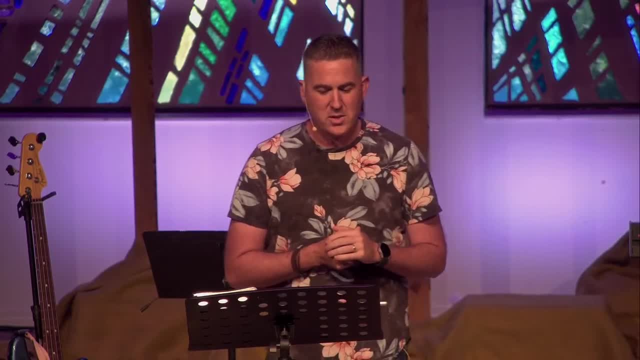 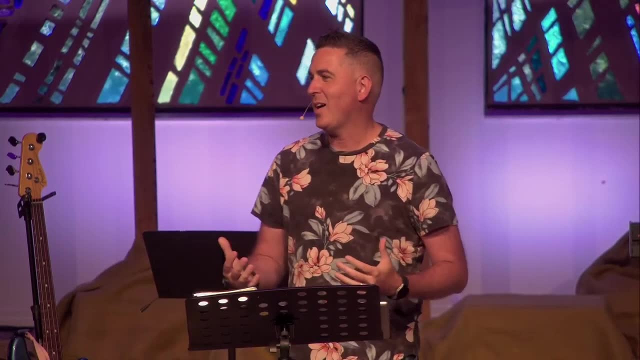 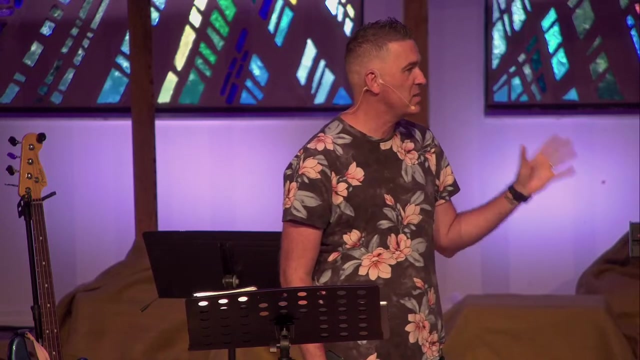 through your word and by your Holy Spirit. We pray this in Jesus' name, and all God's people said amen. One thing that I just wanna draw our attention to is that we have access to God's word in a way that has never existed in history. 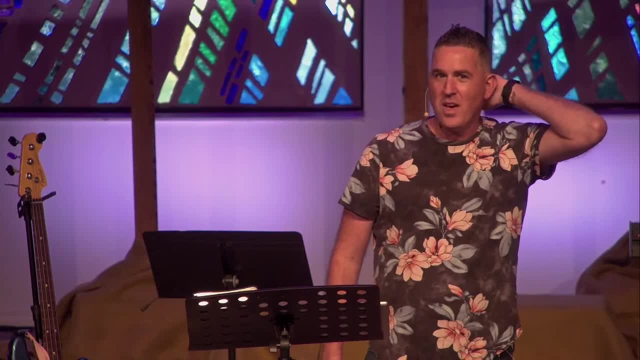 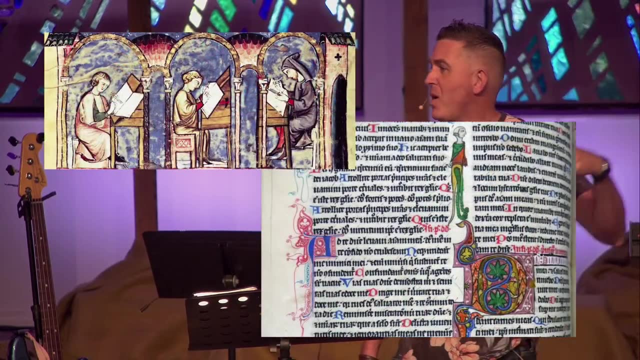 Here's a fun picture of kind of an ancient Bible And back in the day Bibles were just so expensive when they had to be handmade by a monk And pretty much they only existed in the church. The church would create these And you can go look at all the different ways. 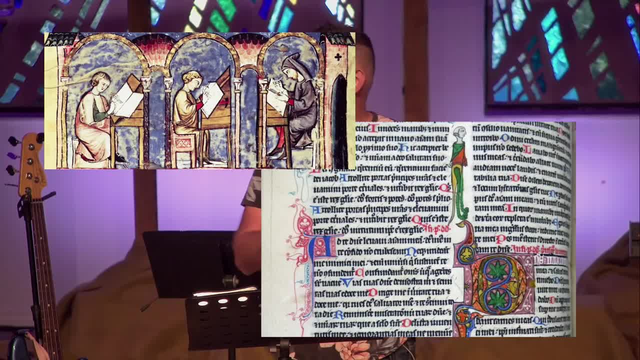 that they would make sure that the translation was accurate from one to the other And they would count every single character on the page And if there was one mistake they would tear up the entire page and rewrite it again. These monks who would give their entire lives. 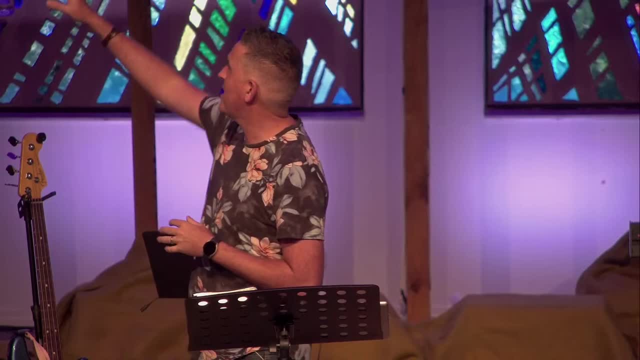 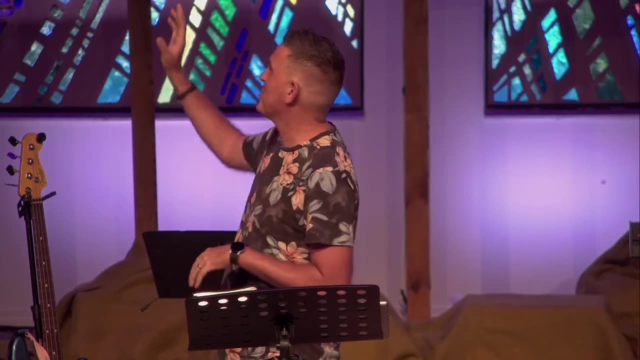 to create these beautiful, ornate scriptures, And that's kind of the picture. on the top left was the Bible, Two monks, also a nun, which tells you it's actually a later picture, because in the early years they wouldn't let the nuns do that. 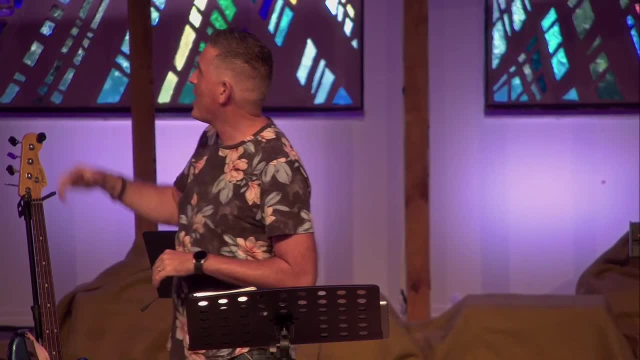 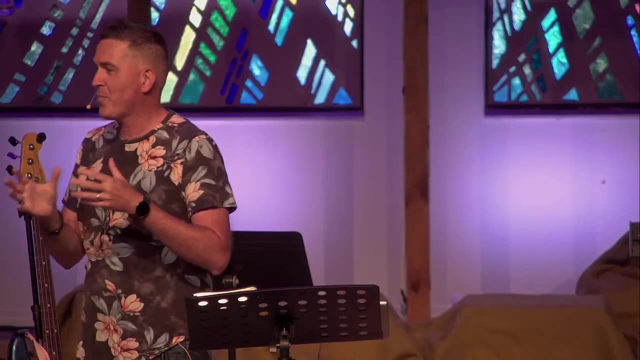 But later on the nuns became a part of the process too, And they were writing God's word out by hand. My son's name is Preston, which comes from Prieston, which is Preston was the priest and perhaps the only person to have a Bible in England. 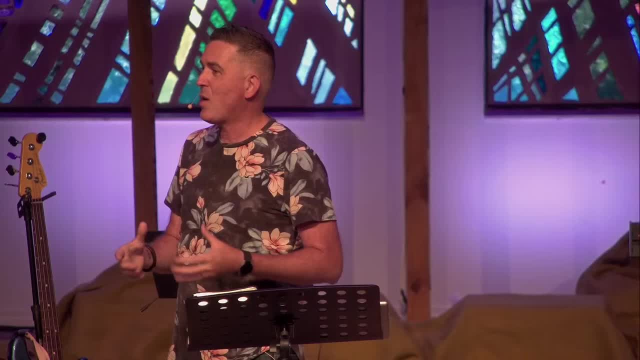 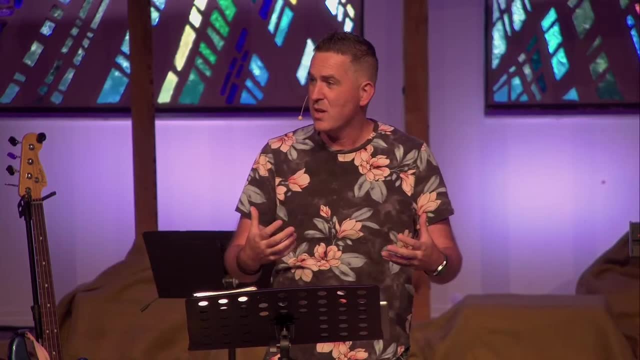 that would oversee like five or six towns, And they would take that Bible with them from town to town On different weeks And they would read God's word so that they could hear it. And now we live in this time where we've got it. 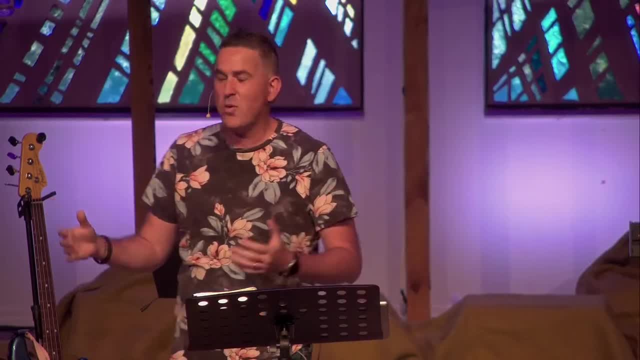 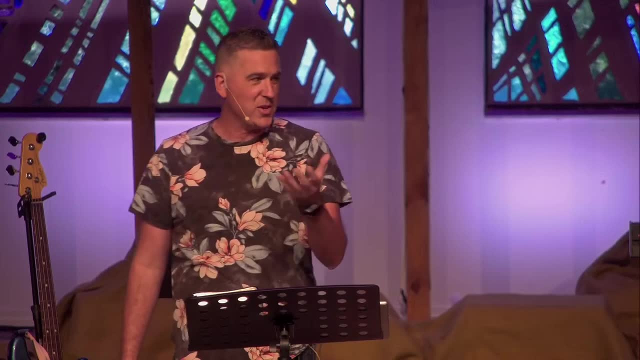 at our fingertips, In every translation, in every language. we can hear it read audibly by a guy with a Scottish accent, because I feel like God's power moves more when it's read with a Scottish accent. That's just my opinion. That's actually what I do for my devotions. 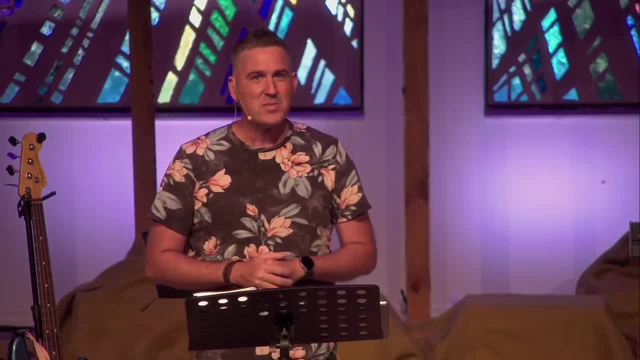 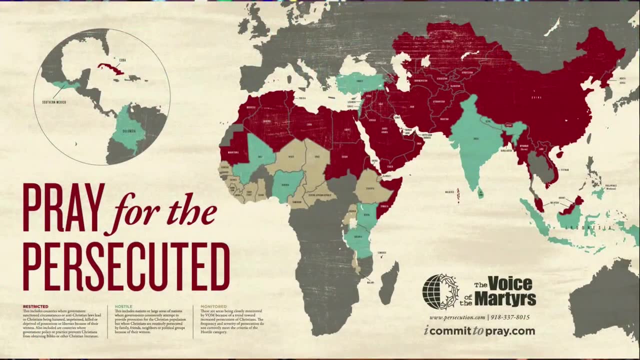 I'm not joking And I love it And it sounds great. But we also can look at the truth of today. Here's a picture of the persecution, the persecuted church that is around us today And everywhere you see and read the word of God. 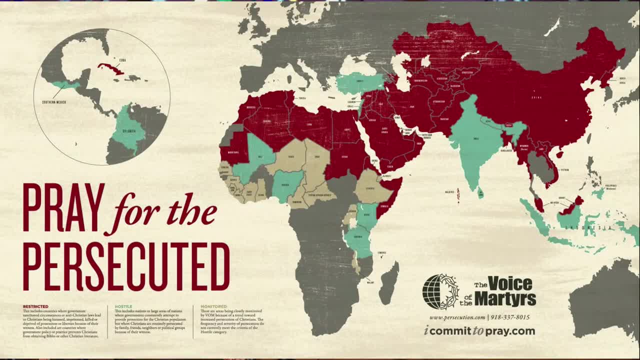 the Holy Bible, the Christian scriptures, old and new, are considered illegal in every country that you see there and read Places like India, other places of Africa. it's places where there's areas that are more free and areas that are more in persecution. 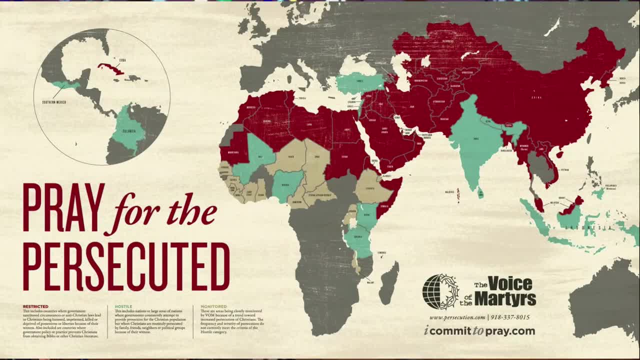 And so we can see that there's these areas that are still, but with so much more freedom, but with so much more freedom. the most significant is, we're talking about literally billions of people who live within these regions, And we see that China becomes increasingly hostile. 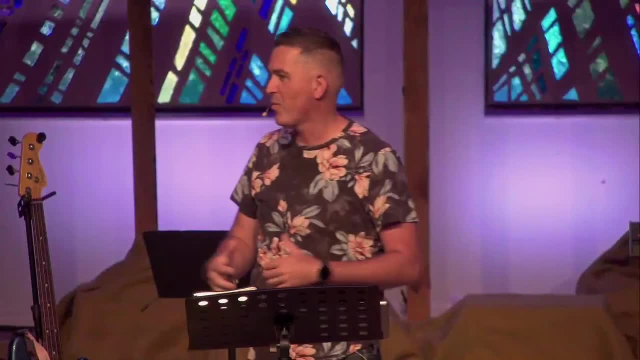 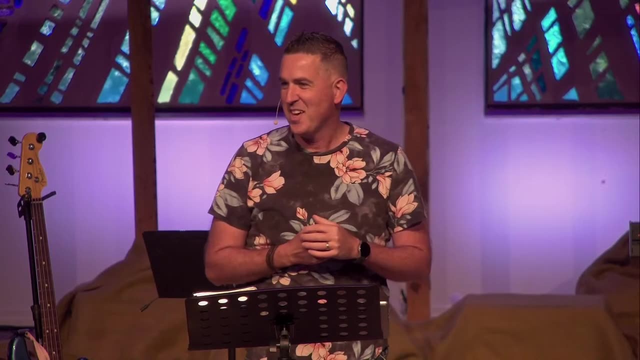 to any type of free speech or any type of word of God that is shared, And some of you did. you guys ever read back? the DC Talk published books called Jesus Freaks- a couple of volumes. Anybody here ever read those? 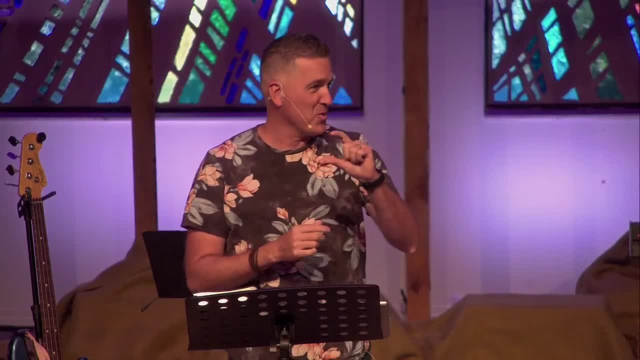 And they were really kind of fun like the way that well they- I can't say fun. It was a really difficult content. The book was beautiful And it was like torn and I think I have one back on my shelf there. 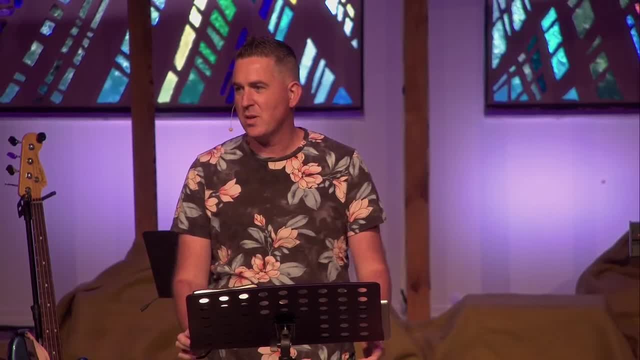 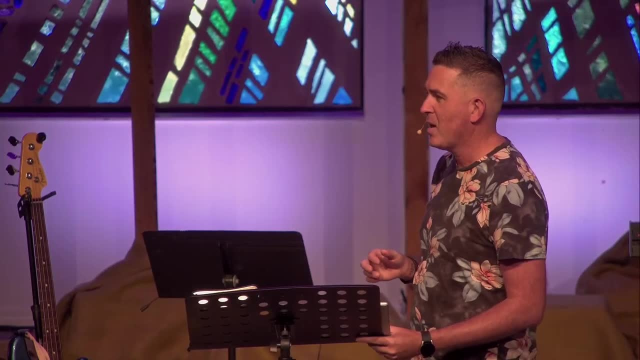 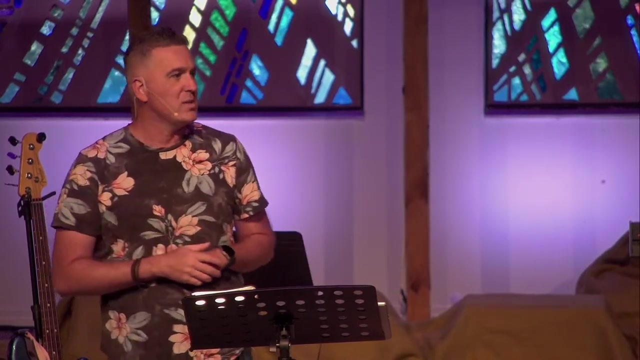 And I always remember. I think it was maybe like one of the first three stories in the book And it was a collection of stories of the persecuted church And it was somewhere in East Asia where a village was brought together under the Communist Party and they found a Bible in someone's home. 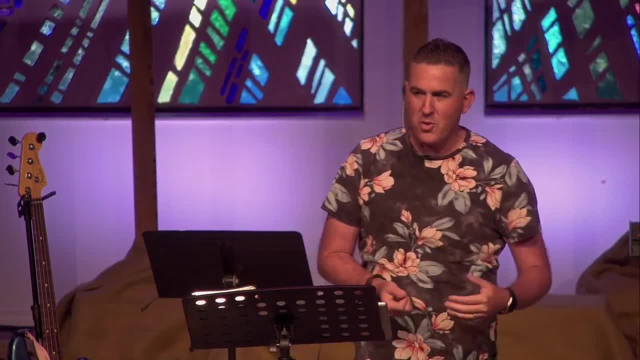 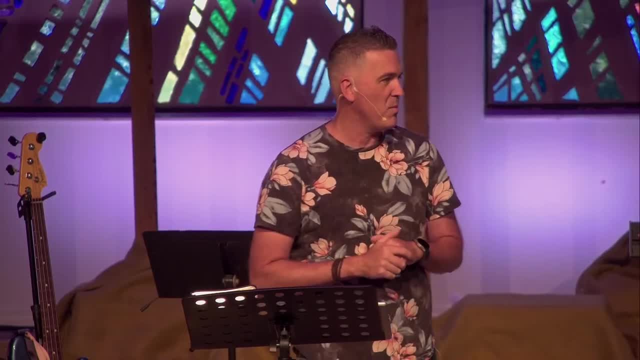 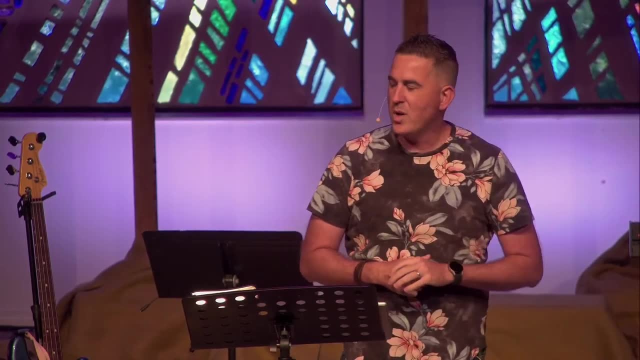 And every single person walk up to the Bible and spit on the Bible, And they wanted to declare that this was no longer allowed under the Communist regime. And finally one young lady goes up and it's her time to spit And she walks up to the Bible. 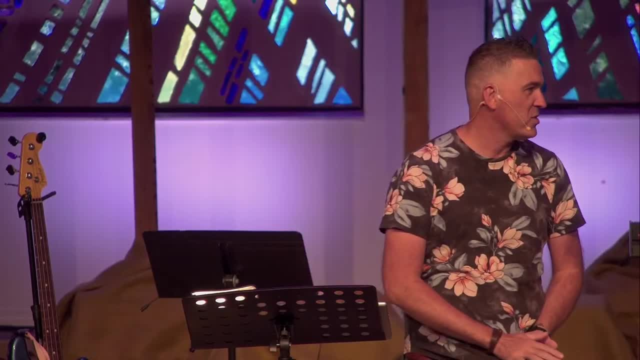 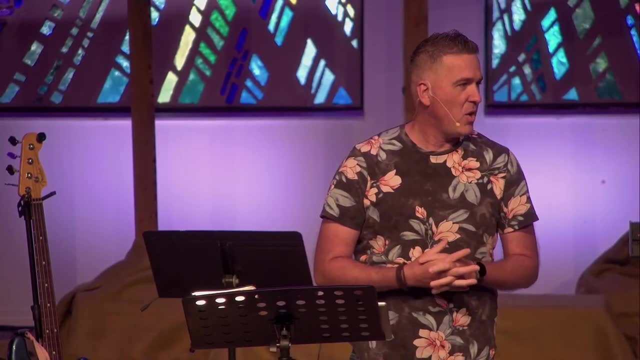 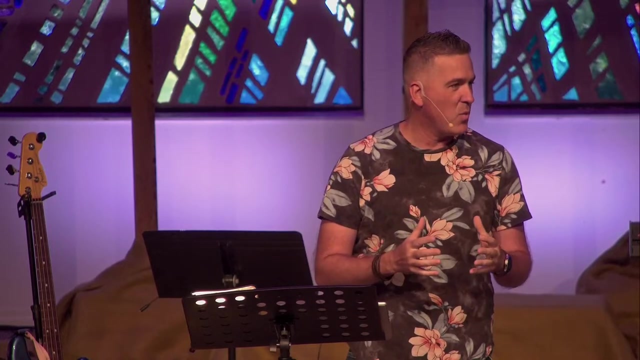 and she kneels down, She grabs the Bible and starts using her dress to wipe off the spit from all the people before her And ultimately, her life was taken over that Bible, right there in this spot, And I just want to share that with you. 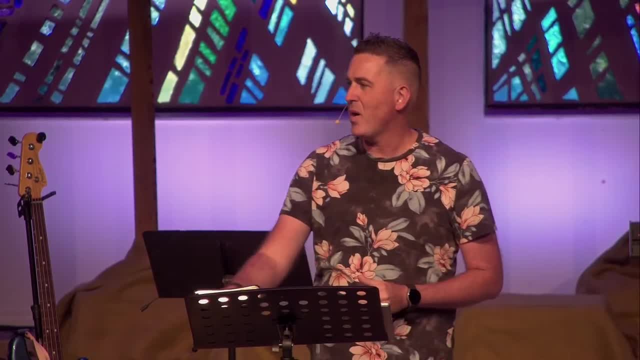 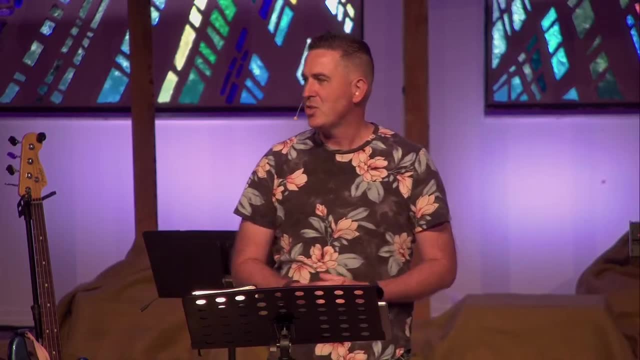 because we take for granted how easy we have a Bible accessible to us And we are so thankful for those who have given us this freedom that we can openly share God's word. And there are still places today where there are airplanes who fly at night. 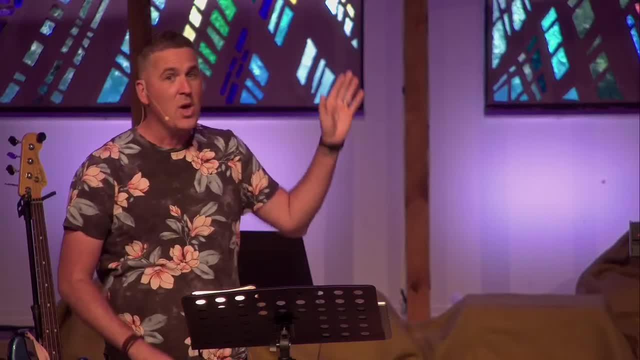 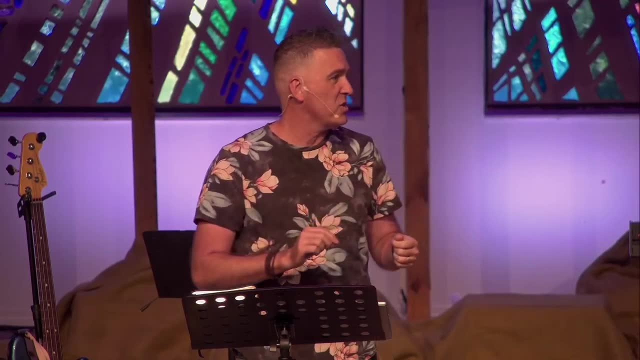 with no lights on wearing night vision, throwing parachutes out through the voice of the martyrs ministry. And in my youth group in the past we made those parachutes that we would make according to their specifications so that we could share God's word in these remote places. 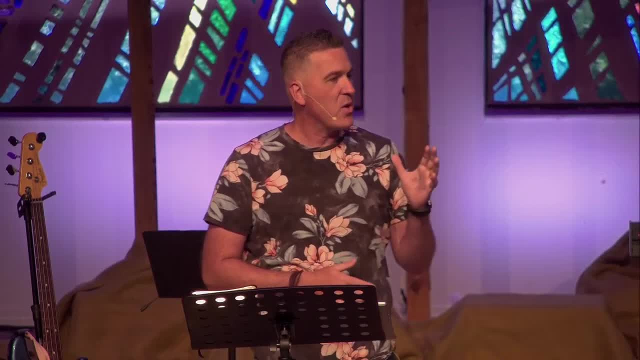 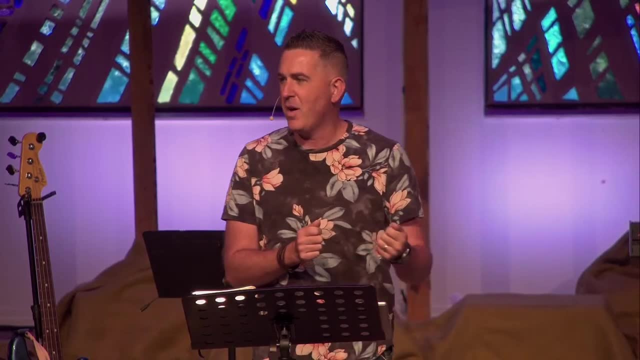 all around the world so they could receive God's truth. There are villages right now that are meeting in hidden places over a scrap of the Bible. they have been given so they can read God's truth, And yet we have God's word available to us. 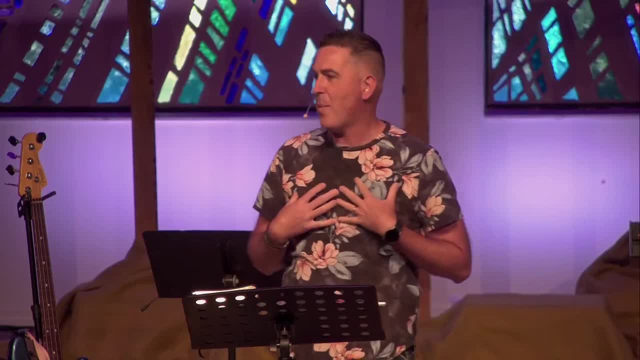 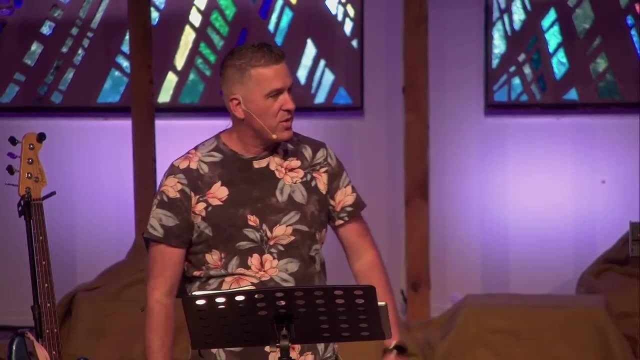 each and every moment of each and every day, And we would probably admit that there's many of us who don't take advantage of that. Many people, maybe, don't read their Bible because they don't care, They don't believe in it, They don't think that it applies. 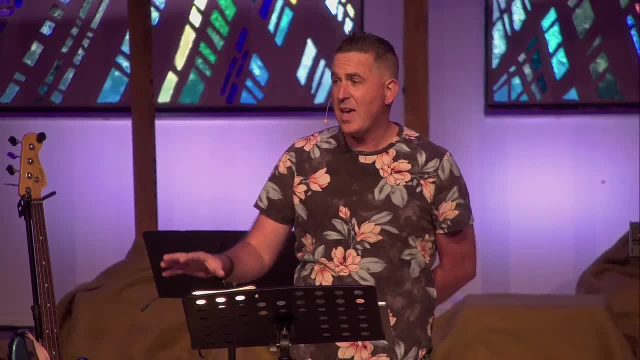 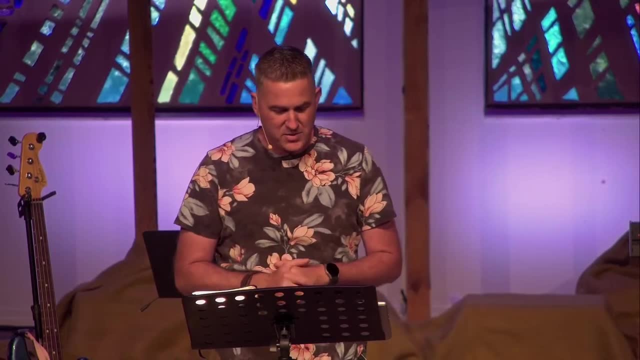 to our life today. It was an old-fashioned story. If they say that they haven't read it because there's not a page that you read, that you're not like man, I can't believe this was written then because it applies to my life today. 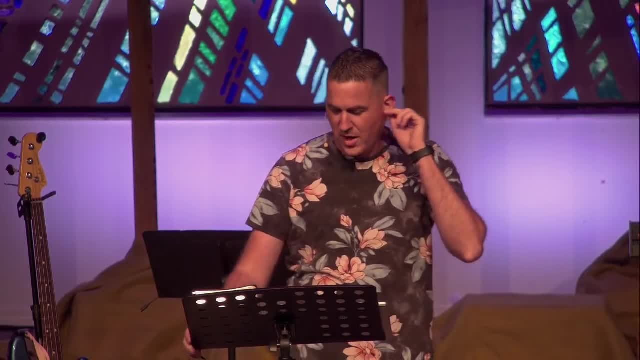 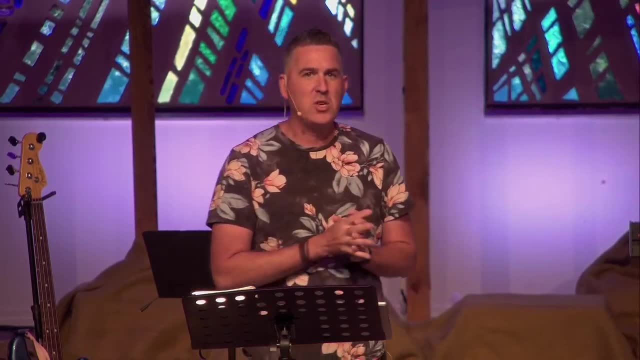 Some people have tried and they've got bored, Some don't understand, And so last week we went into kind of some simple, practical steps on how to read your Bible. Here's the QR code and the website that we're going to use. We're making for our church. 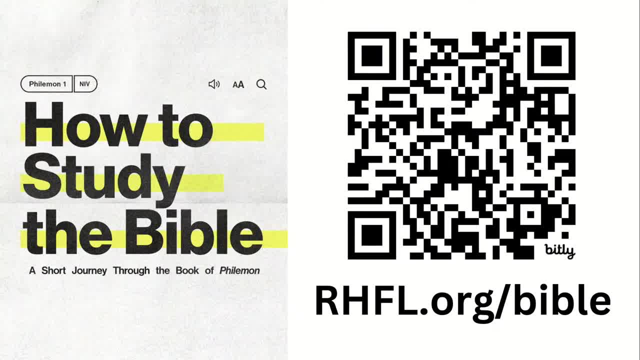 that you can go and you can get all the lessons from last week. I'm going to update some from this week and also give you some examples from other pastors in the area on ways that we can read God's word. But the one thing I shared with us- 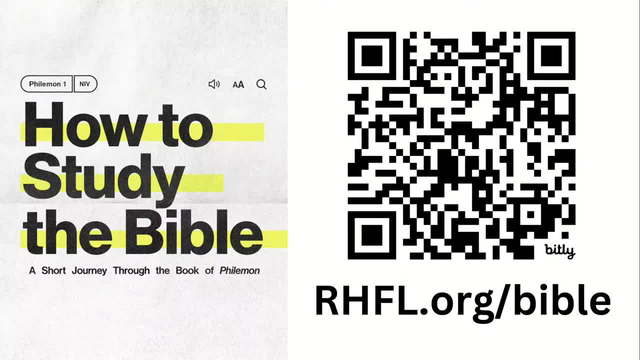 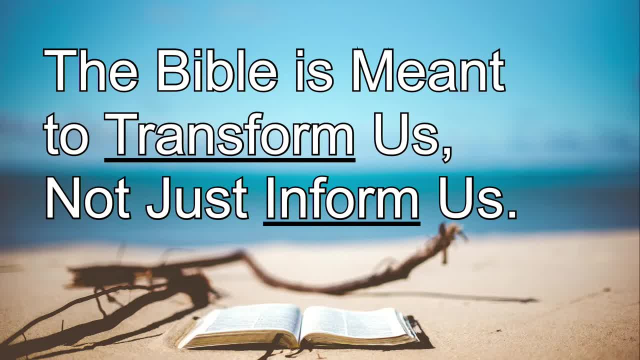 in the prayer is: the Bible is meant to transform us, not just inform us. We don't want to treat the Bible like we're preparing for a Bible trivia. I will tell you, I kind of feel like I grew up like that We would do sword drills. 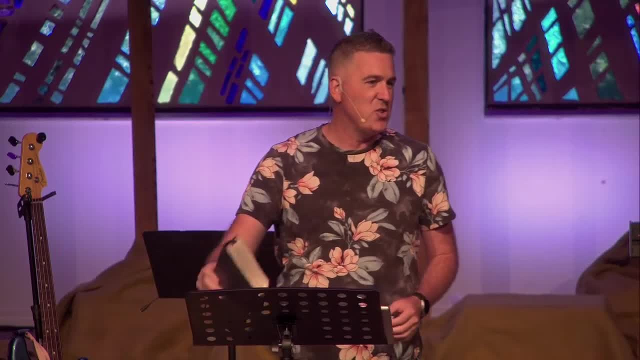 How many people have done a sword drill? The Bible is the sword, So you would have like two Bibles and they would be identical. They'd be up and they'd say: ready, set go. And you would compete to see who could open it up the fastest. 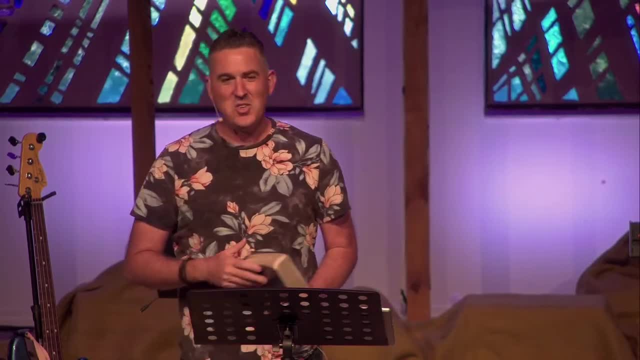 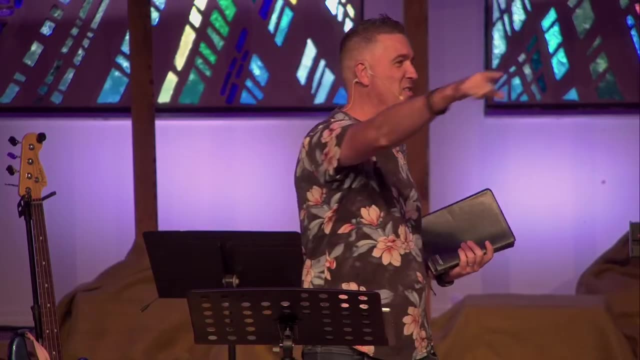 And I remember growing up this one guy was just amazing at it. So the kids would compete against the leader and he literally- this is a pretty big church- He'd be all the way to the back. They'd say go, And he'd have to run and do a lap. 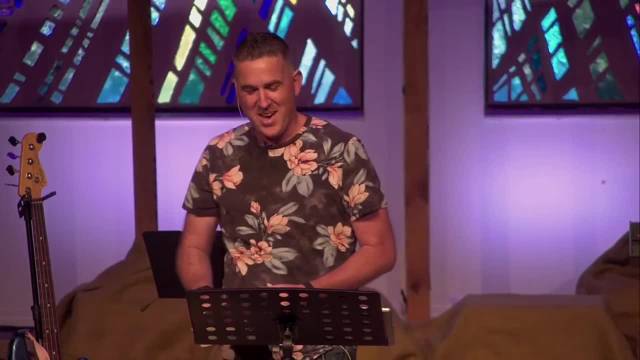 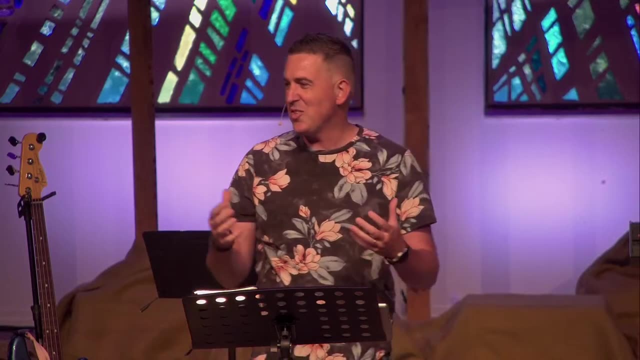 all around the kids and go up to the Bible And I still couldn't beat the guy. And I found out later he had like four people And I was like he's super smart, He basically memorized the whole Bible And so just you know. 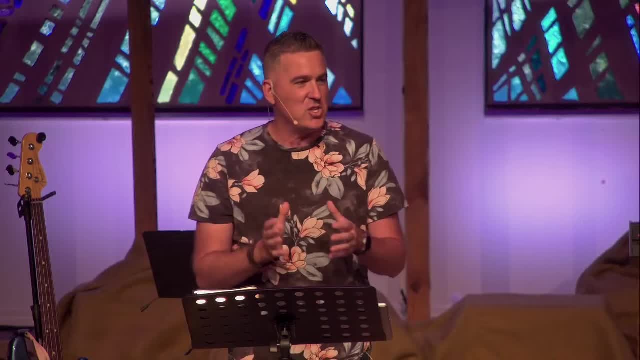 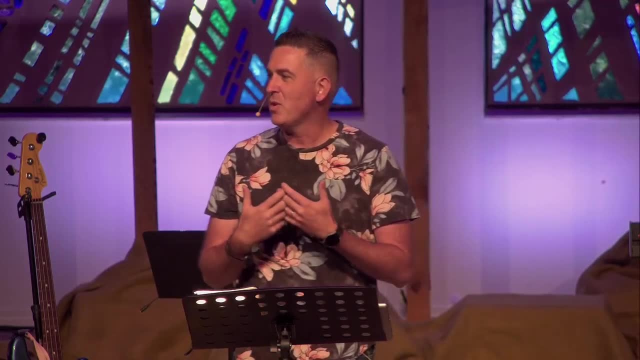 I grew up in that kind of idea of like, through Bible memorization, if you could pass Bible trivia, that's going to get you into heaven. And so we want to also understand that the Bible is meant to transform us, not just inform us. 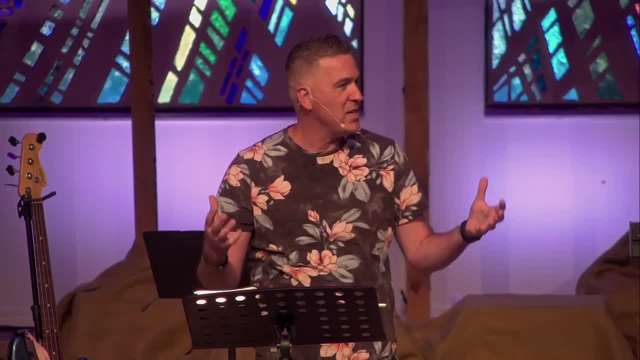 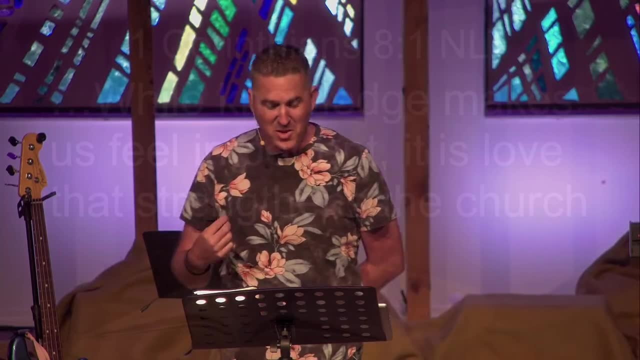 And so that's the perspective I want you to take into this entire idea of studying God's word. It says in 1 Corinthians 8, while knowledge makes us feel important, it is love that strengthens the church, And you guys have to be so proud of your daughter. 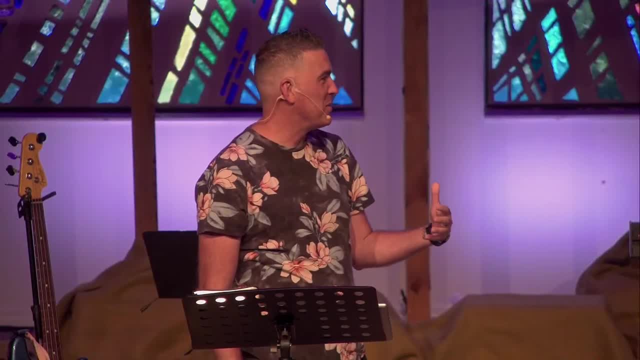 that. that was her response when we asked the question of like: you know what are we supposed to be, And she's like: well, what brings us here is God's love. You know that she understands that at a young age. 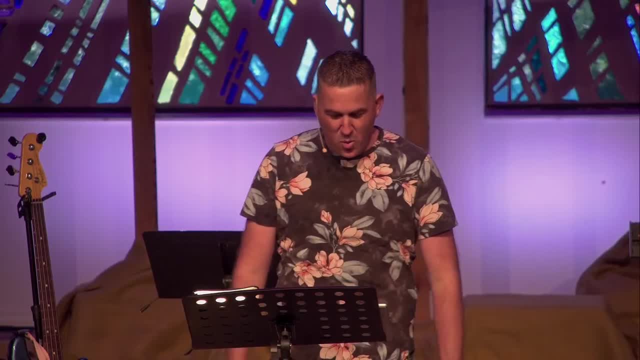 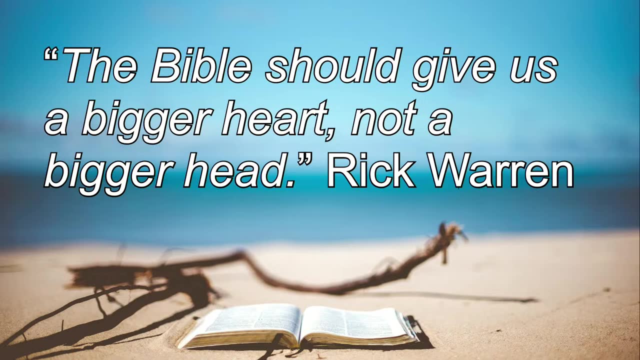 that it's God's love that brings us together. Rick Warren said the Bible should give us a bigger heart, not a bigger head, And it seems like I've seen the battles where people are like trying to like. two Christians are trying to compete. 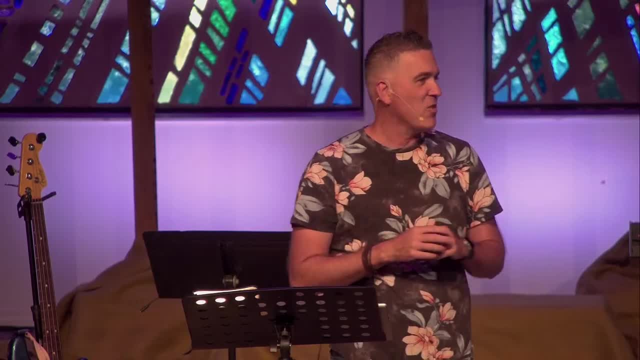 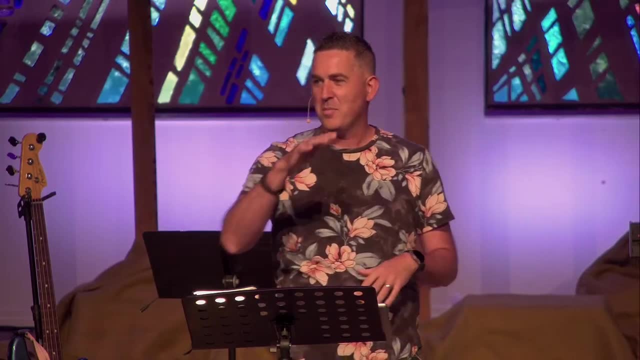 with who knows the most Bible verses can win the argument And they're like: well, the Bible says this and the Bible says that, And it's kind of like you know the joke is, you're looking at a football play. The right coach is the one who has the chalk last. 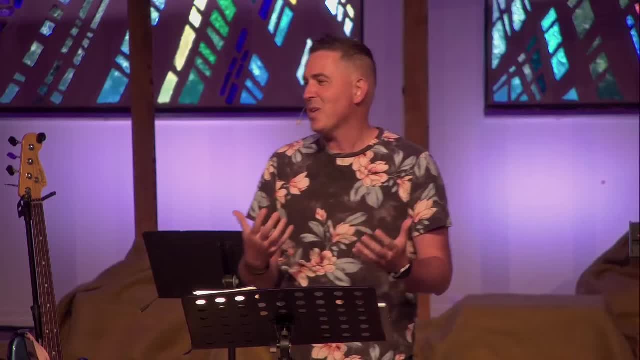 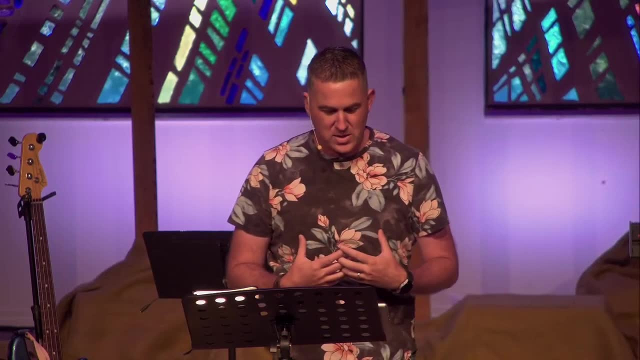 And they're like just trying to compete with who's got the best Bible verse. That's not what God wants us to do. He wants the word of God to be nourishment to our soul. He wants us to crave it. It says in James 1,. 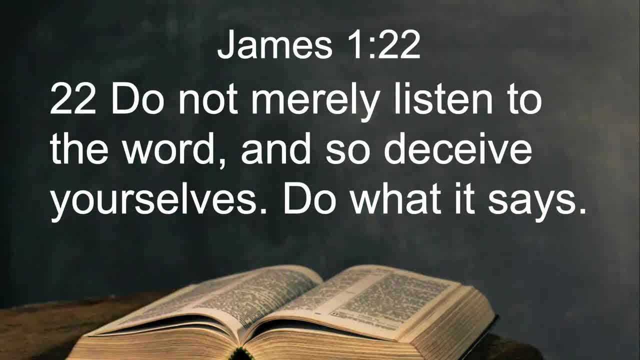 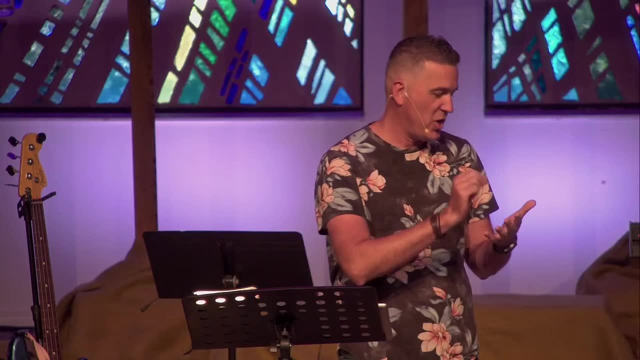 do not merely listen to the word and so deceive yourselves, but do what it says. If you forget everything I say today, remember that verse That we don't just want to hear God's word and say, okay, we went to church check. 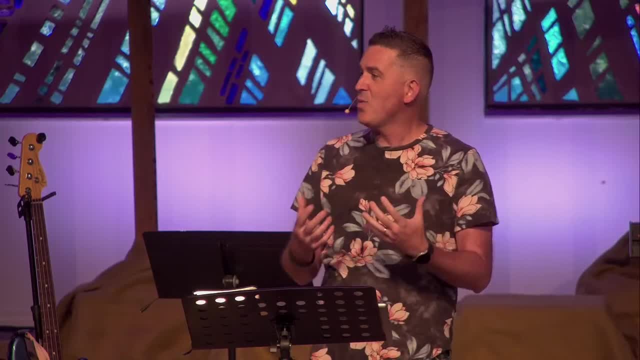 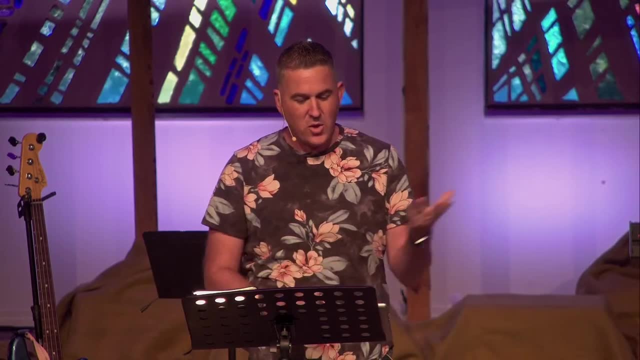 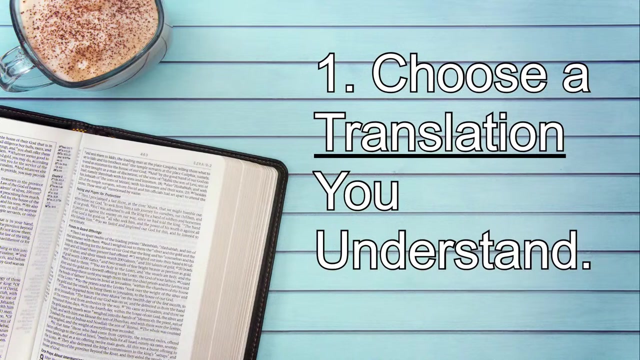 Okay, Monday morning I did my devotion check. No, he wants us to let it transform us from the inside out to be like the person of Jesus. So last week these were our five points on how to study the Bible. The first. the first is: choose a translation you understand. 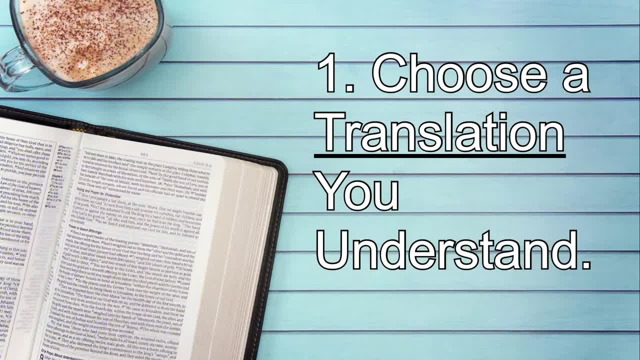 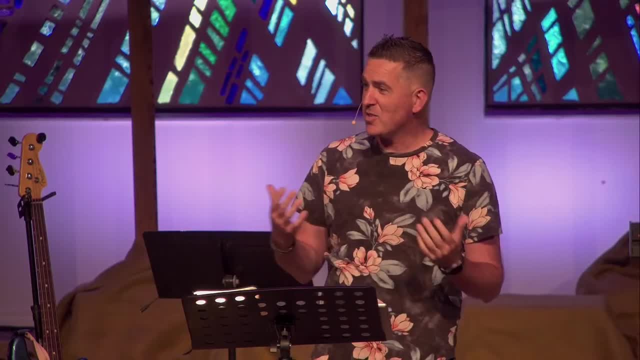 Yesterday the lady who cut my hair. I was talking to her about my message for today. She goes: yeah, you know, my struggle is I always get lost in the begotten's. And my response was: if your Bible says the begotten's? 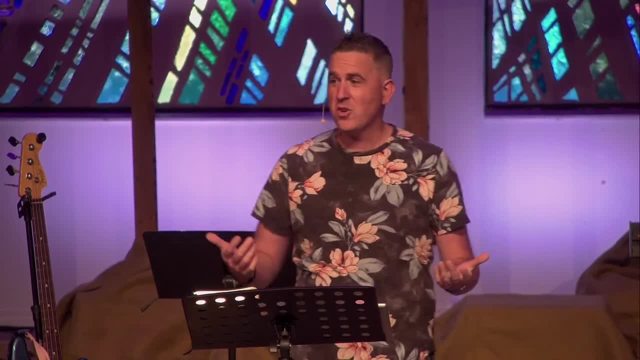 you probably have the wrong translation for you. You know, for some of you you're like it ain't the word of God. If it doesn't say begotten, that's great If that works for you. but I said I encourage you. 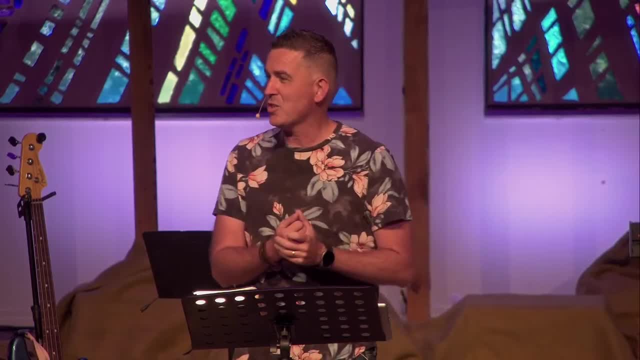 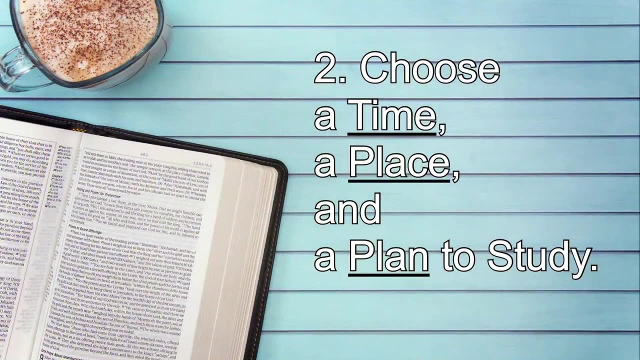 If you get lost in the translation, you're going to get lost in the Bible. Get in the new living. That was my encouragement to her because you know I just wanted her to get started. The second was choose a time, a place and a plan to study. 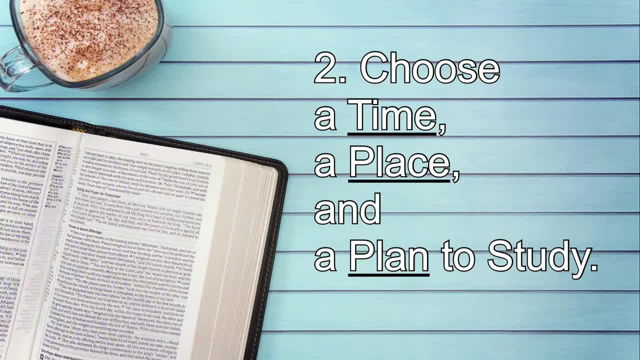 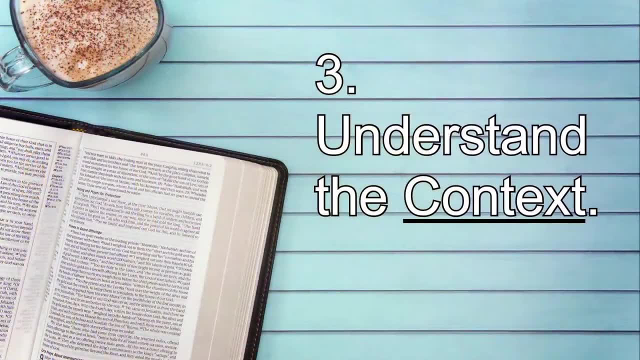 So here we are. we're in week two, So I'm hoping that this past week you identified your time, your place and a plan to study. Number three was to understand the context of what you're reading. Who wrote it? 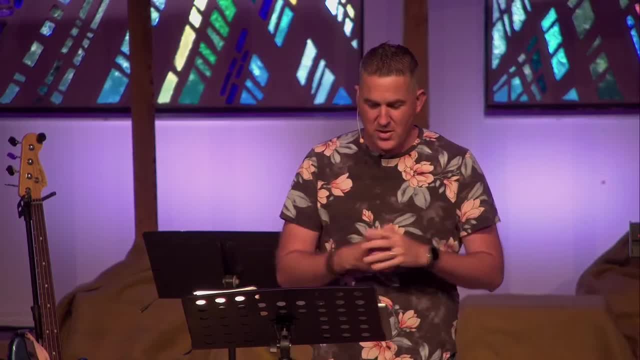 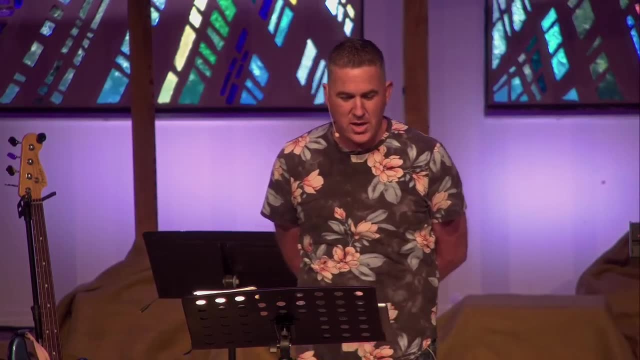 Who is it written to? What type of literature is this? Understand the context? Is this before Jesus? Is this after Jesus? Number four is we're going to read slowly and ask questions. Number five: we're going to pray for God to speak to you. 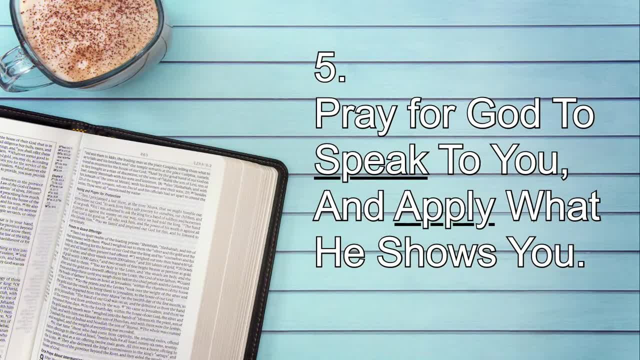 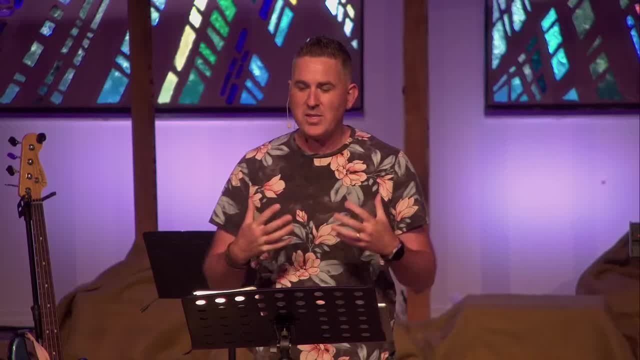 and apply what he shows you, And so I kind of assume that we've been through some of those steps. If you were here last week for the message, you've got your time. I like to do mine in the morning, but I do want to just share with you one thing. 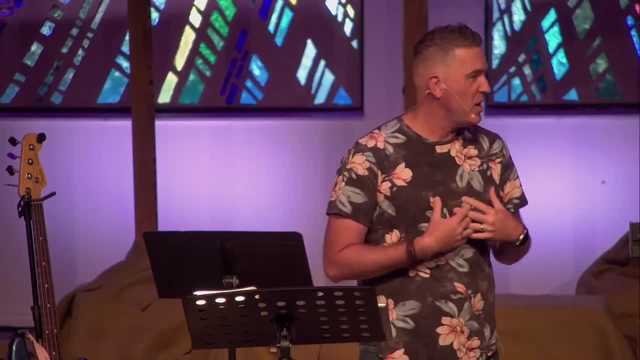 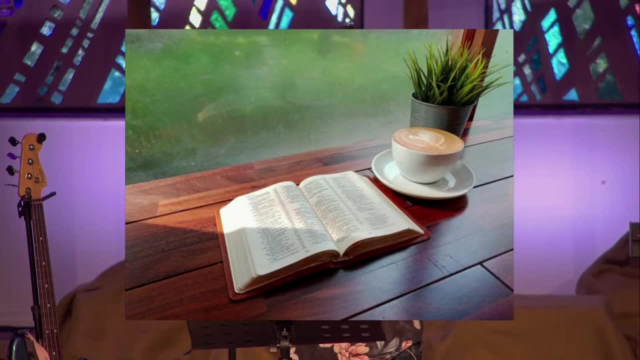 And that is like I feel- like we even get challenged in our Bible study- that it needs to be like on Instagram, Because you know we see these pictures. Here's a picture that I found just on the internet And I will tell you there's also nothing wrong with this. 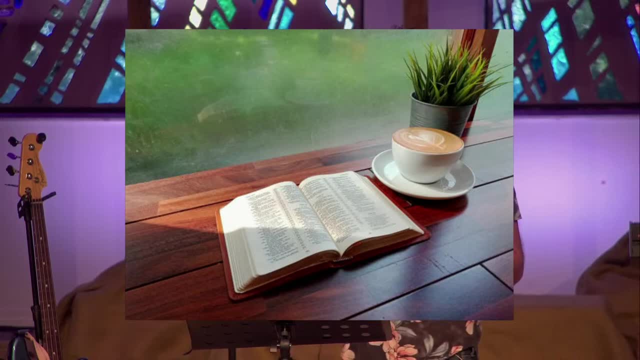 I actually really enjoy making a cappuccino every single morning And, yes, I will admit to you, I try the little pour over to get the designs. Haven't mastered it yet, but I'm trying. I love the mornings, In fact, tomorrow morning, Monday mornings are my morning where I can do this. 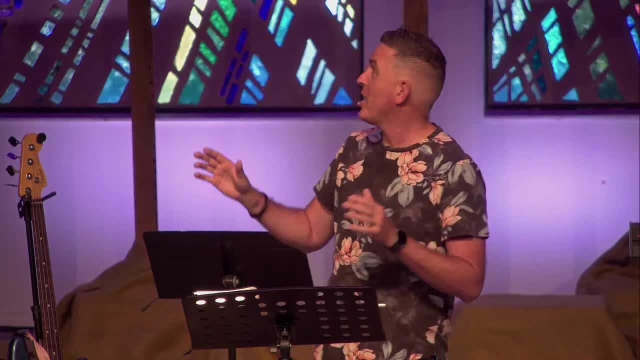 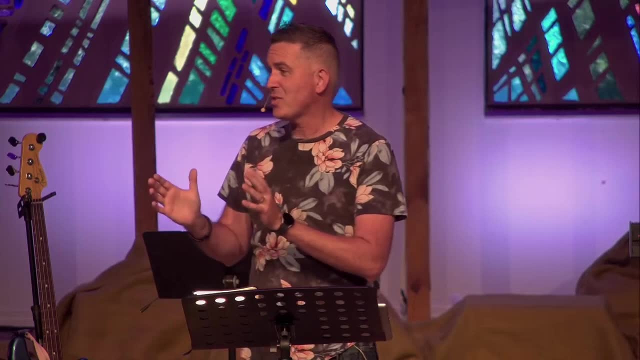 Where I can sleep in a little bit more. I can take my time and I can get my cappuccino, get my Bible, Go out to the beach and spend that time with the Lord. I can pretty much tell you every Thursday morning. 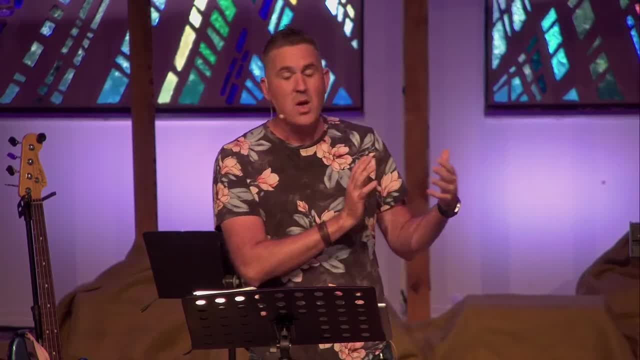 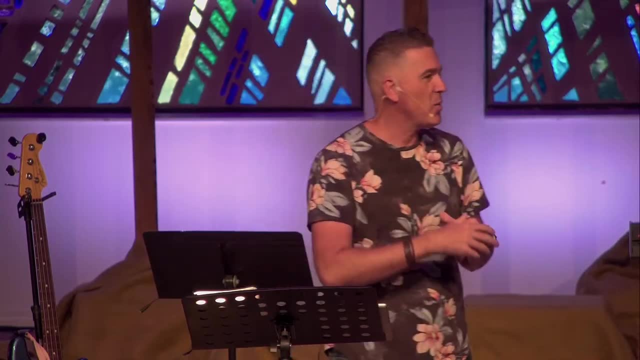 when I'm driving both my kids to school for about an hour, I listen to our devotion in the car together while we're going to school and we talk about it, And so what I'm trying to share with you is that your Bible can't always be this like perfect Bible study, and that's okay. 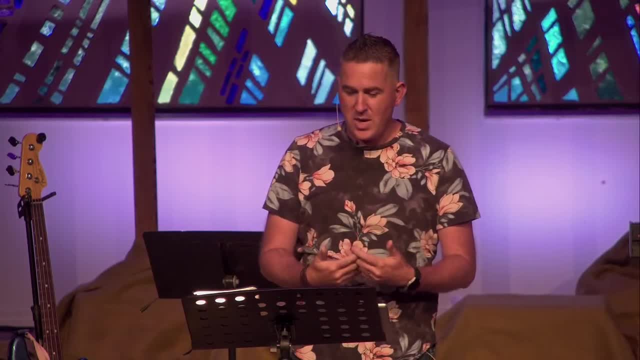 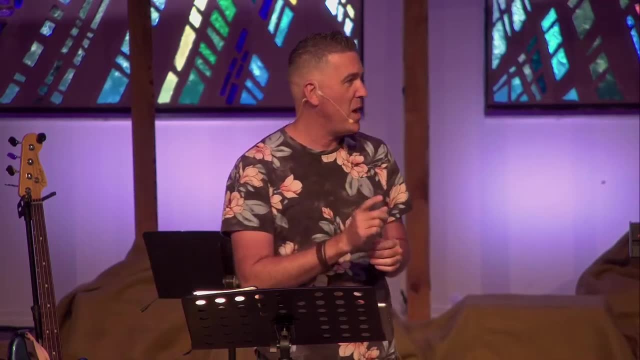 But we got to find that way that works for us, that we can be in God's word on a daily basis. And I will tell you that the only bad plan on reading the Bible is what You're going to guess it: No plan at all. 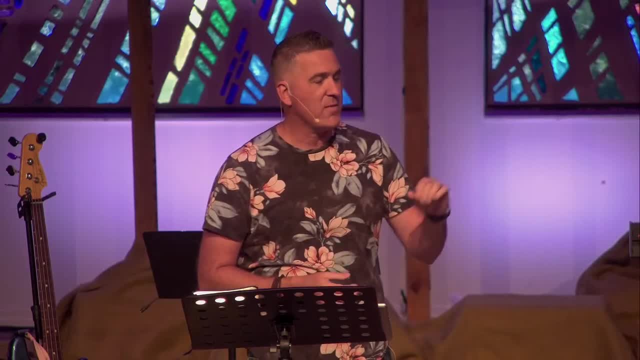 So we want to have a plan. So when you wake up in the morning, you're getting ready for school, you're getting ready for work, whatever it is. we execute the plan in the morning. We make the plan the night before. 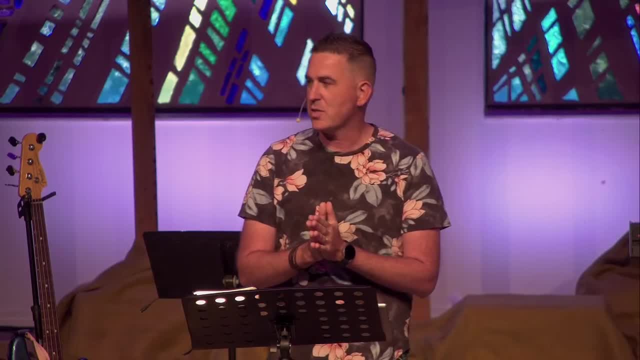 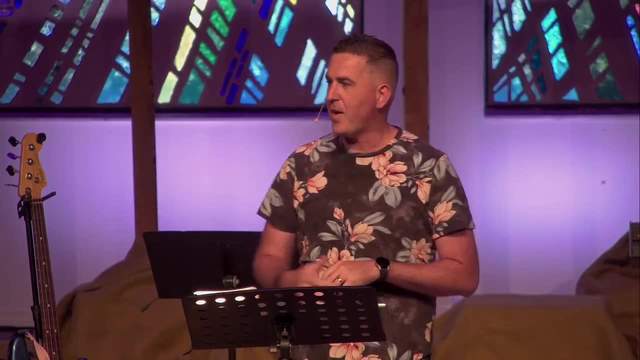 So today we're going to look at the five different approaches on ways that we can approach a plan to read the Bible. And I had some fun. I sent out a message to our staff. I sent out to like some fellow ministry leaders in the area. 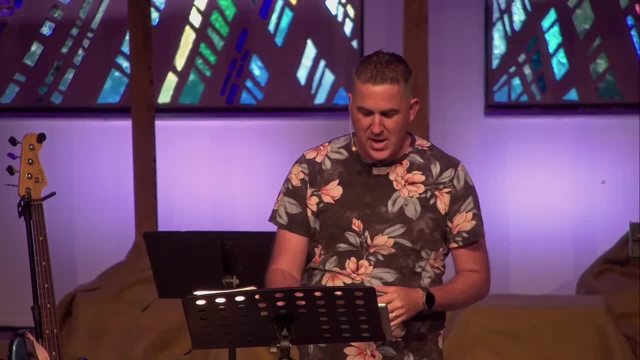 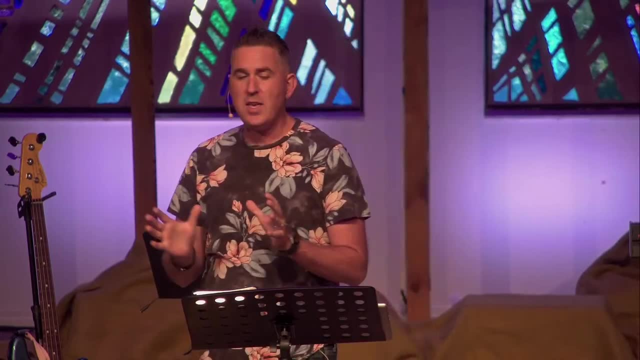 And I got back a lot of different responses from other pastors And I'll share some of that with you as we go through these points. So the first one is we're going to look at you can study a book of the Bible. So if you're trying to understand your plan, 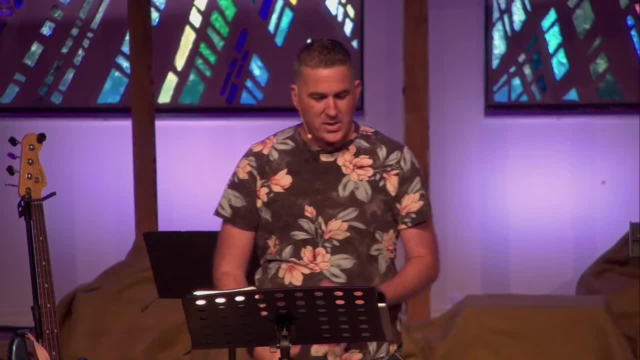 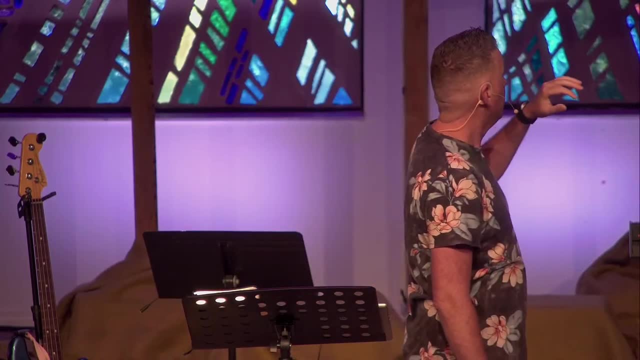 the first thing is you can study a book of the Bible, And so I reached out and I asked people kind of, what do you like to read? If you look at this next slide here, this took the survey and kind of gave us a fun. 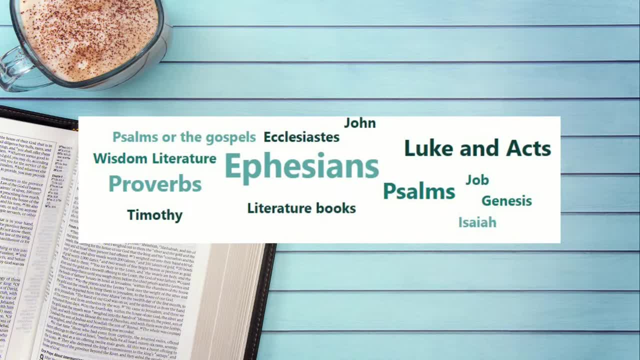 word graph with it, And actually the number one that jumped out was Ephesians Dan Carter, one of the directors of Fellowship of Christian Athletes for our community, Jim Capel- he's the pastor of Church for the Beach- And Jenny Zents. 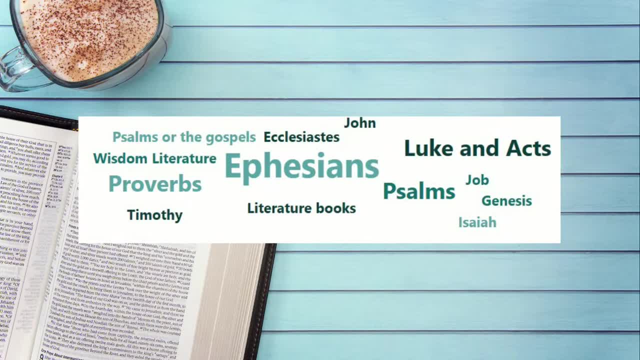 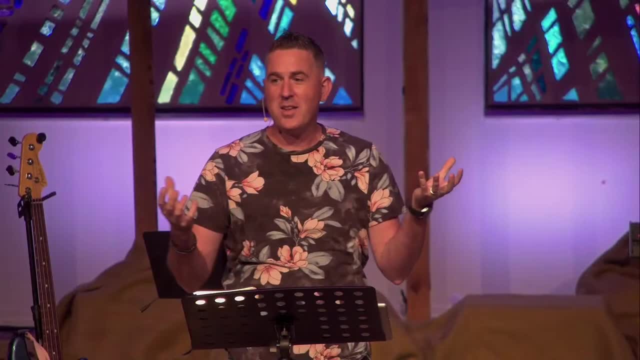 our discipleship pastor. They all said Ephesians. Jenny, why did you put Ephesians as the one that you like to read How the power of God meets our intertwined life? And that's the name of her podcast. So it's just in my mind. 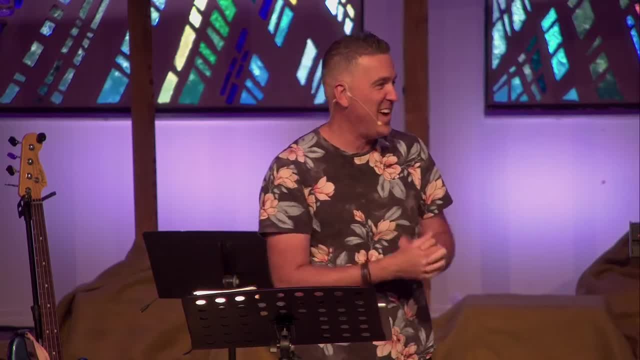 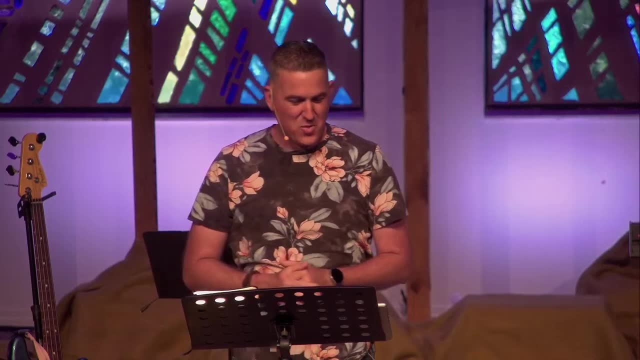 And so that's what you love and this service. you knew I was going to ask you, So you were really prepared. It's great, And if you want to understand deep theology, you can read the book of Romans If you're hurting or you're just feeling like you're overwhelmed in life. 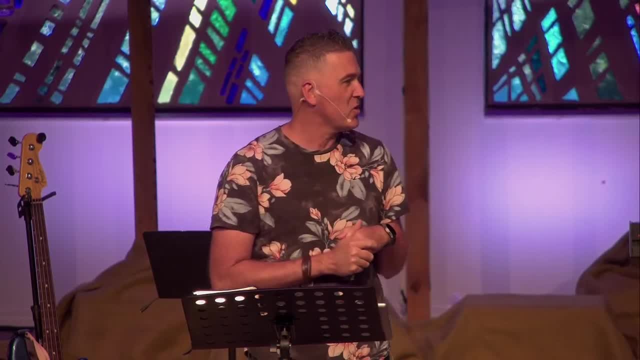 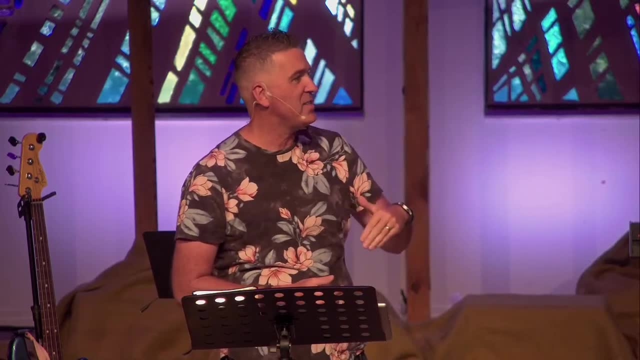 read the Psalms. Billy Hoffman, who greets us as an usher most weeks, he shared with me that he likes to take the date and read the Psalm and the proverb for that date, And so he knows. all he has to do is know the. 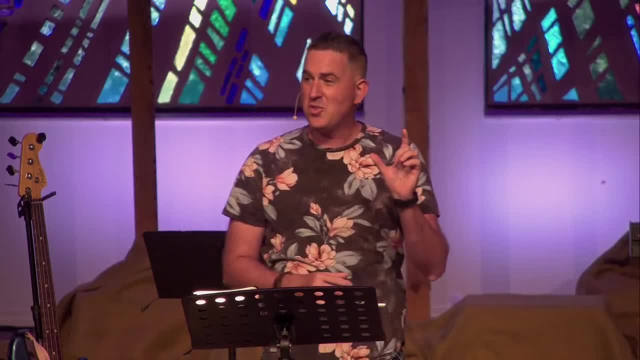 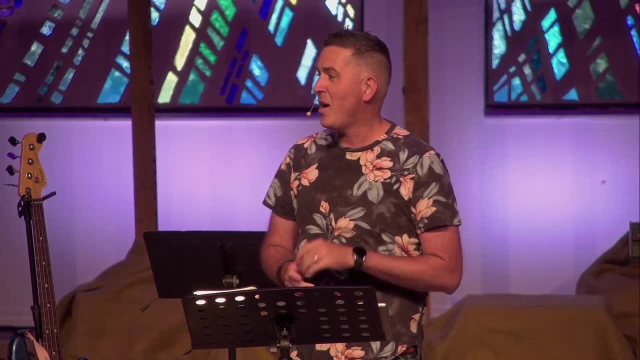 what the date is and then go find that Psalm and Proverb. It gives you a little bit of encouragement. It gives you a little bit of wisdom. It's a great combination. If you're going to read the gospel, Pastor Jonathan from First Baptist in the Atlantic and I both said: 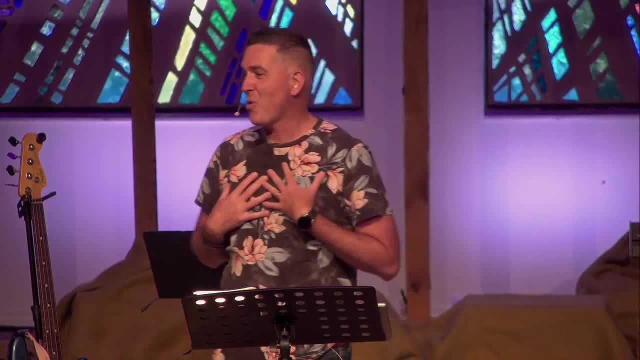 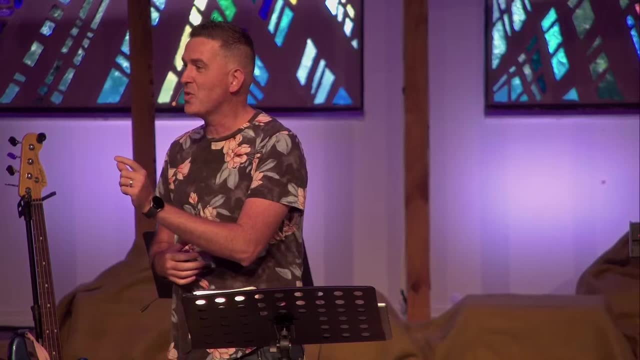 start with the gospel of John. My pastor that I worked for for 10 years, Pastor Tim Heinzelman, out of Columbus, he said to read the gospel of Luke and then read the book of Acts, because Luke wrote them both, And so it's the same type of. 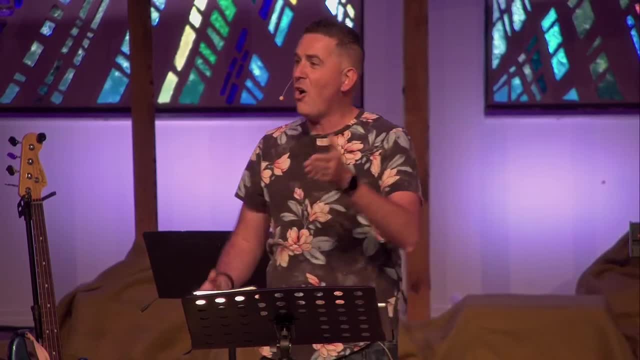 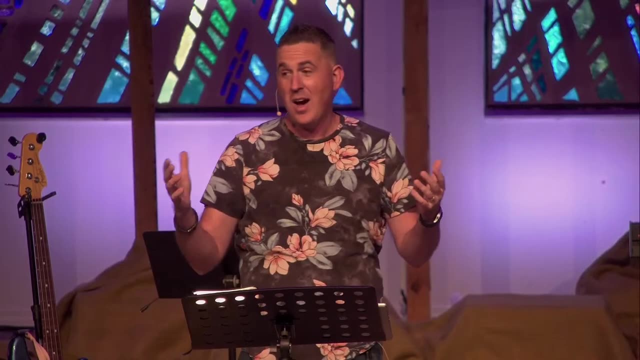 it's the same kind of word composition and it goes all the way from the birth of Jesus, all the way through the acts of the early church and into Pentecost and so much. That's not what I thought of. I think that's a great idea on how to read God's word. Or you can go back and understand the beginning, get into Genesis and Exodus And then, unless you've read through the Bible a few times, I would probably stop at Exodus and move on to Kings, If you want to be in the story or get in the New Testament. 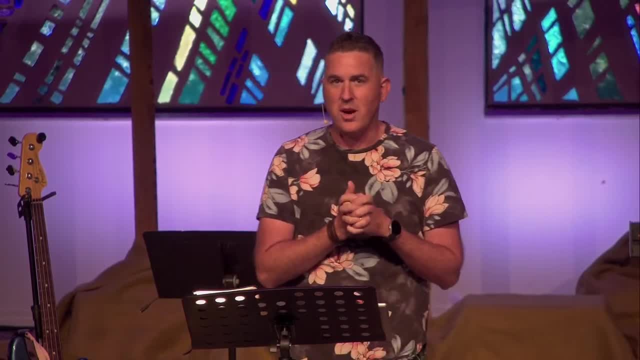 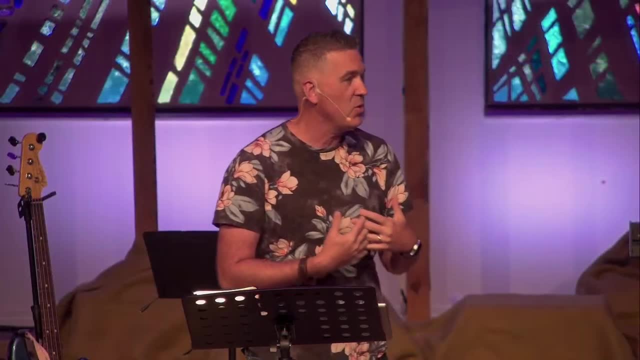 Another idea is that you can study a person of the Bible So you can find a character from the Bible that you enjoy, a person that you feel connected to. One person I love to study is Nehemiah. I think Nehemiah is just great because he says: 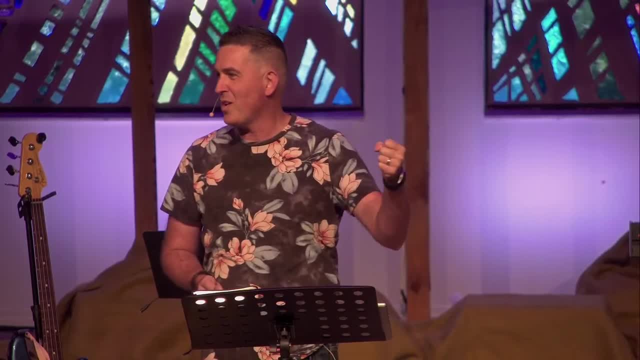 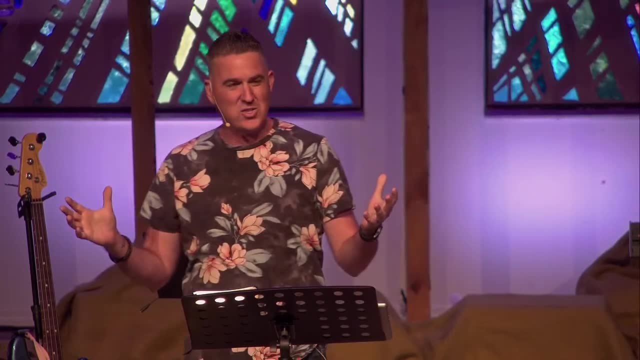 let's have our shovel in one hand, let's have our sword in one hand and the shovel in the other. And so he says: let's do the work and let's be prepared. I just think it's a great story. I love to read Nehemiah. 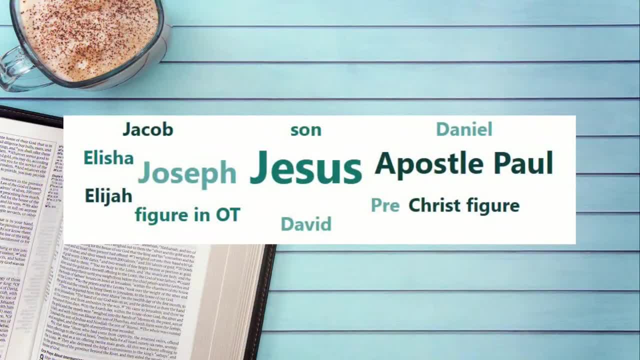 Here's some others that people in the community responded. I should have said, like you know, you can't pick Jesus, because everybody wanted to pick Jesus. But also Joseph was the pre-Christ figure in the Old Testament. Somehow those words got all kind of scrambled up. 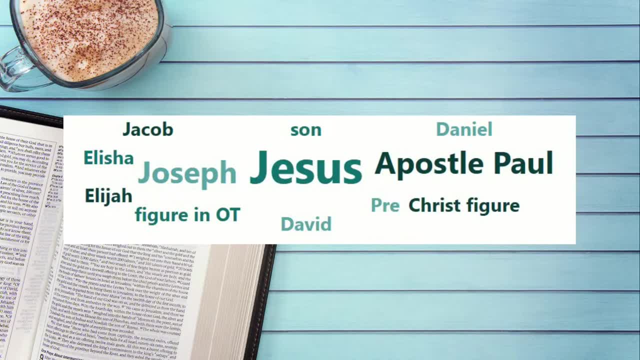 But David is a great person. We can all understand that David did great things for the Lord. David had the heart for the Lord. but David also sinned publicly and openly against the Lord, And there's a story of forgiveness and redemption there. 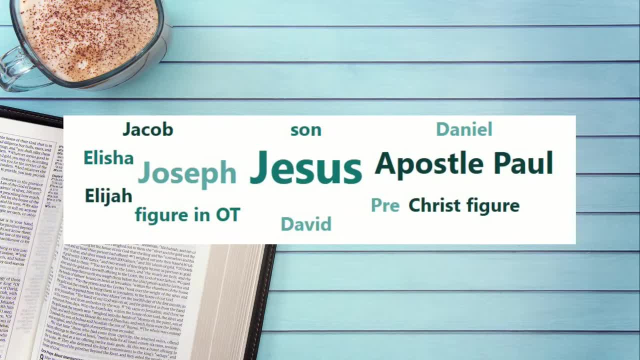 It's a great journey for some people to go through. Daniel is just an amazing prophetic character to look at. So you find a person that you want to study and you can look up and find their story and follow their story- Another way to study the Bible. 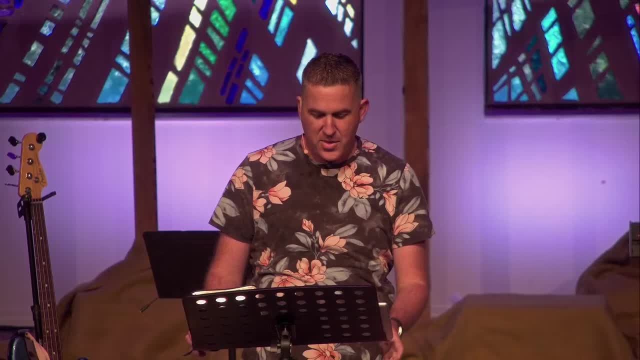 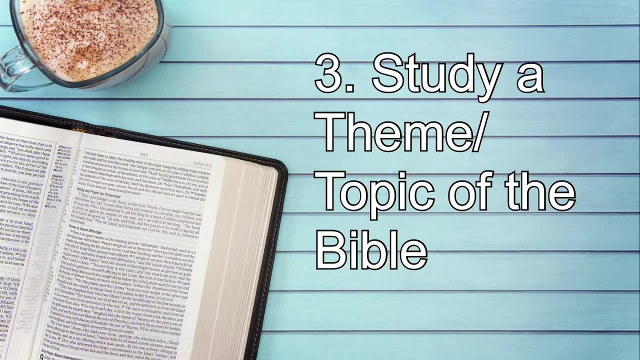 that perhaps is going to work for you is to study a theme or a topic of the Bible. You know, maybe in your life you've just been dealing with a lot of guilt and you want to understand God's grace, And so you can go to the YouVersion Bible app. 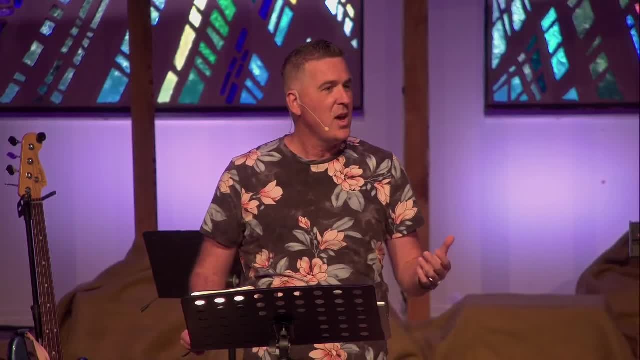 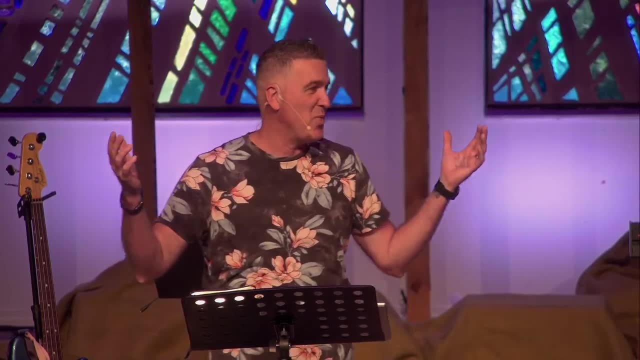 And, by the way, last week I told you there was 32,000 plans. Well, that was actually going off of some old notes that I had. I actually looked again this week and there was 53,000.. So they've increased 21,000 plans. 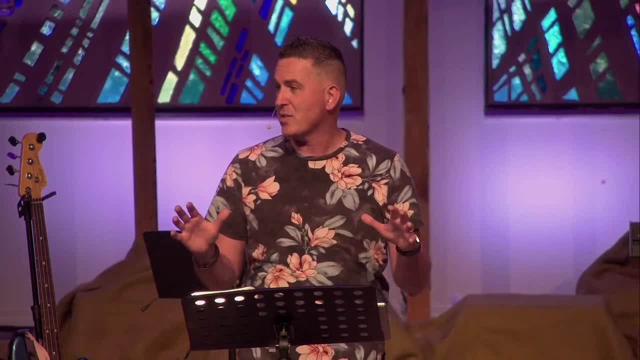 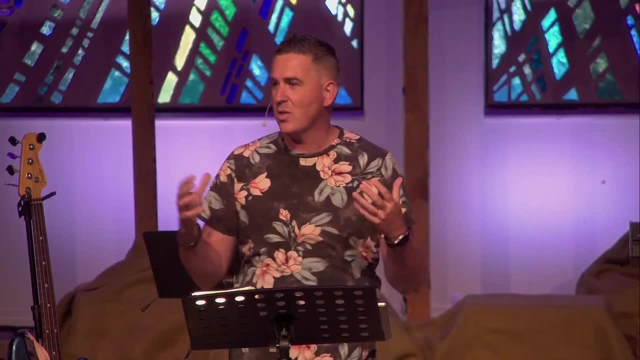 over the last couple of years And you can just type in grace and you can get a reading plan on grace. Maybe you've been dealing with anxiety in your life and you can look up peace and find a whole devotion plan. And you can look up peace. 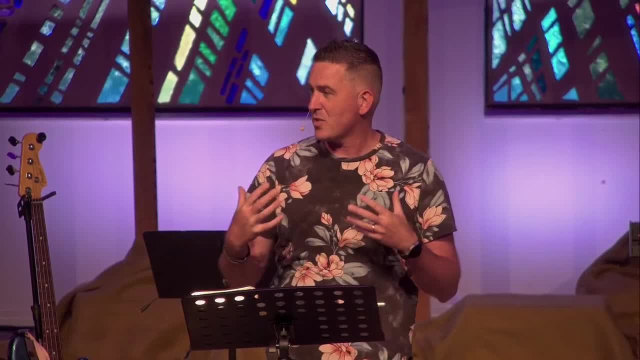 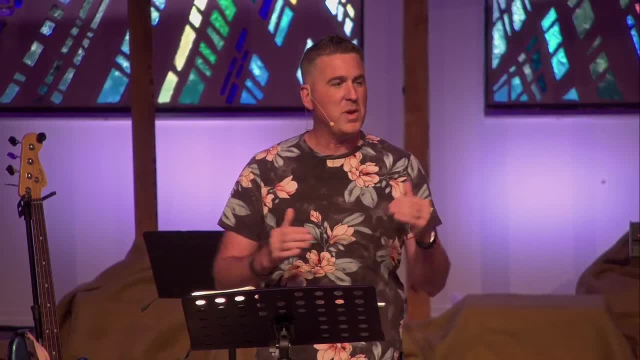 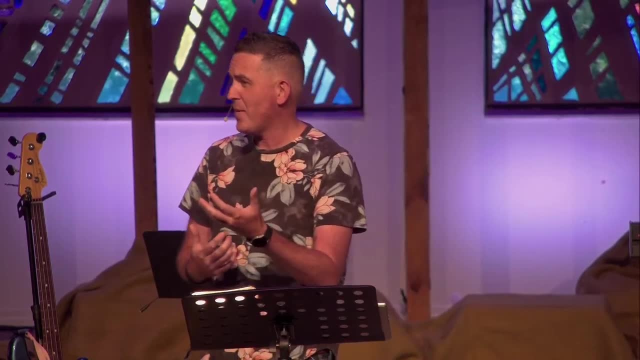 And the next step with that, on all of these, would be to find someone else who can read that with you, That can hold you accountable. The YouVersion Bible app is great because you can read it with a friend, with a partner, and they can actually see your notes. 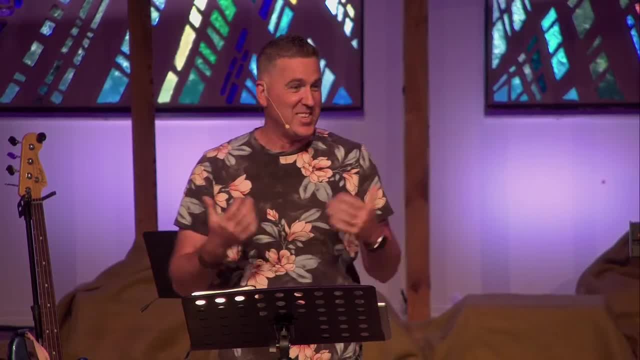 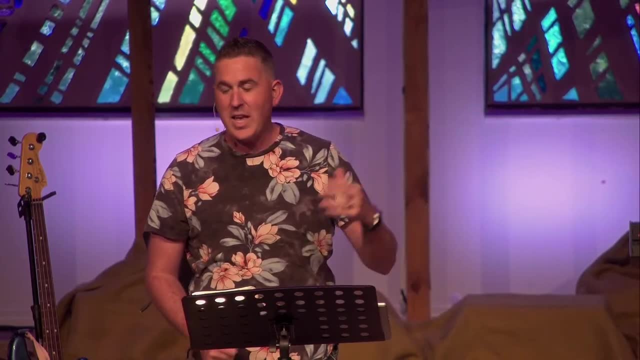 and you can pray for each other along the way. I see some heads nodding because you're like, yeah, that's so good, It's so helpful for me. Another thing that we asked questions to the people was on daily devotionals. 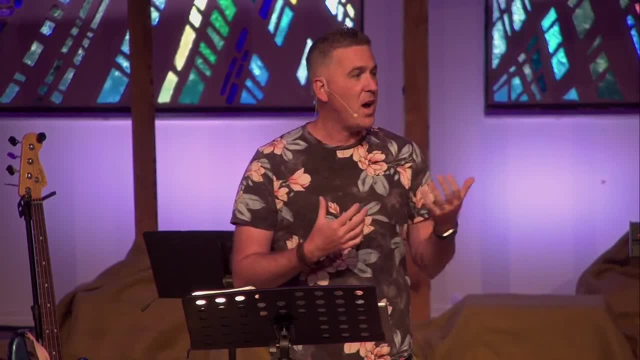 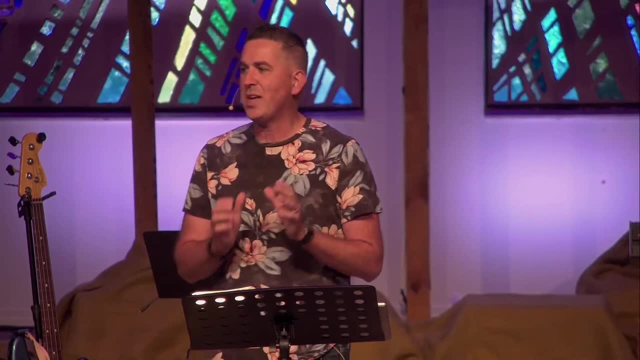 You can do a daily devotional. You can simply find a devotional book that will help you every single day. I would encourage you to find a devotional that does have some kind of emphasis on scripture, That we're not just hearing people's opinions. 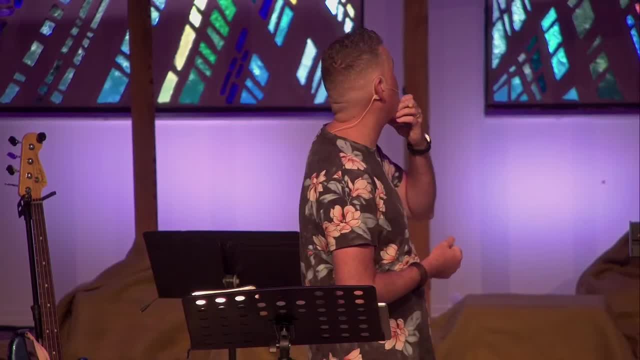 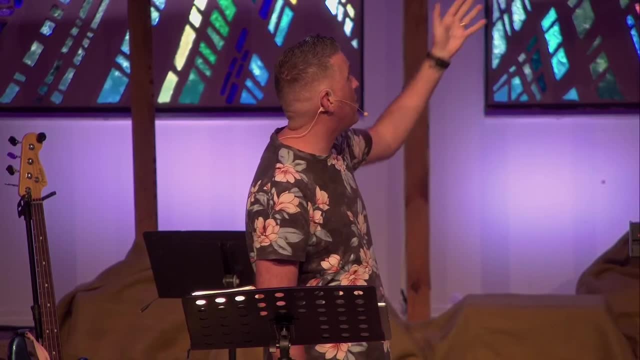 but we're getting in God's word every single day. So I asked a number of pastors in the area and Tim Keller was mentioned quite a few times. Like I said, Proverbs and Psalms utmost, first, highest, which I read. 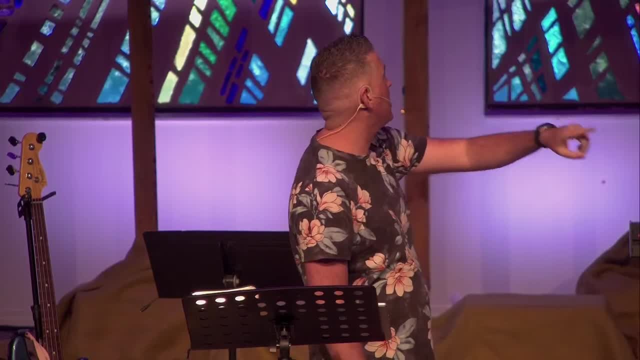 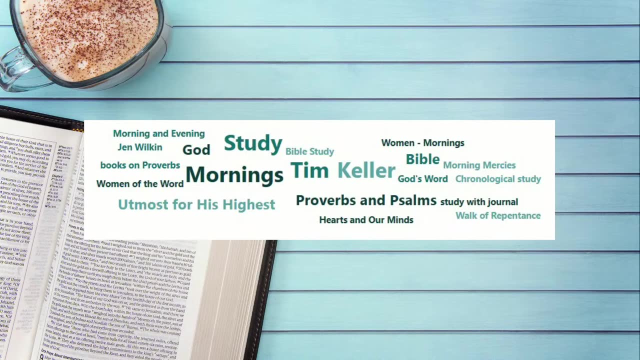 The Walk of Repentance and Jenny, yours was Okay. Women of the Word, How to Study the Bible is a great tool for this whole process. There's a book called Morning and Evenings and that's a really fun one where you actually like. 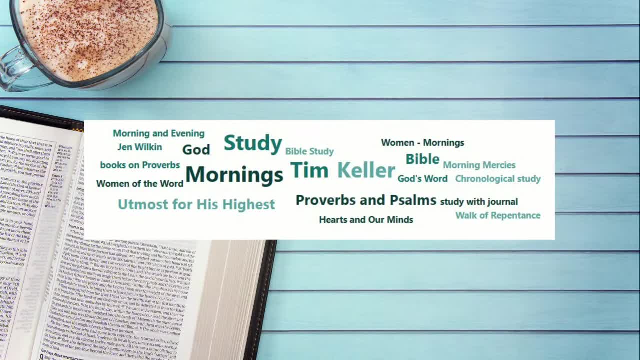 it gives you a little devotional to start your day and to end your day, and it's contextually written to kind of bookend your day. And I will tell you, I've done that one and it's a really, really special journey to go through. 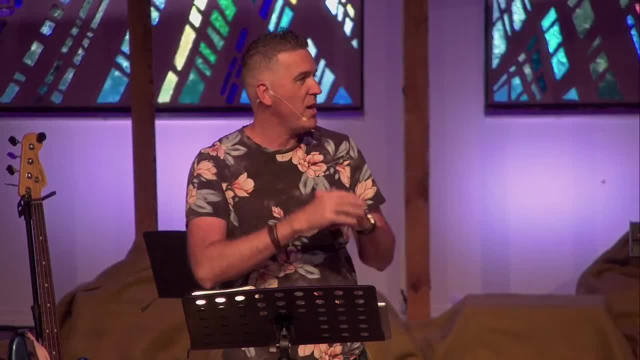 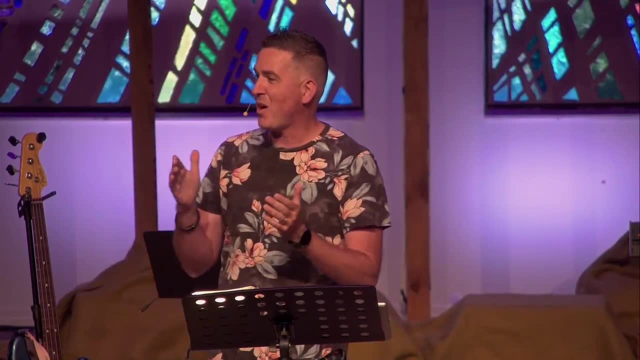 to kind of start and close your day out with the Lord. One thing I didn't say in the 830 service I encourage you to is something fun. that I do is when I wake up I say a prayer almost first thing when I start my day and that's my conversation with Jesus. 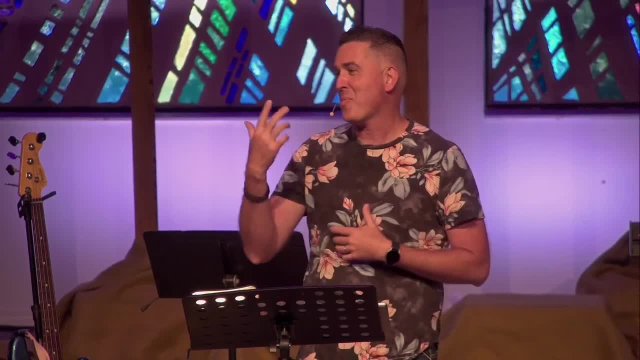 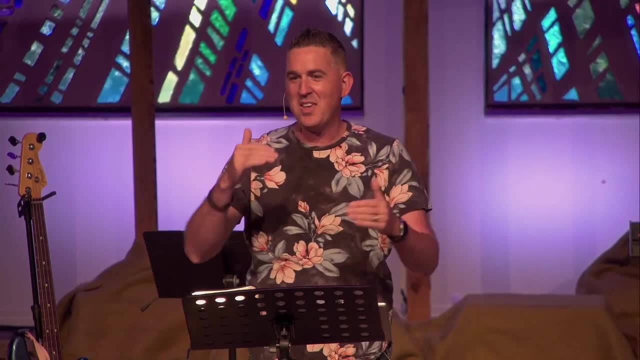 And I don't say amen for my prayer of Jesus until I go to bed at night. And it just kind of puts me in this mindset that hey, Jesus, you and I we're gonna spend our day together. We're gonna be together. 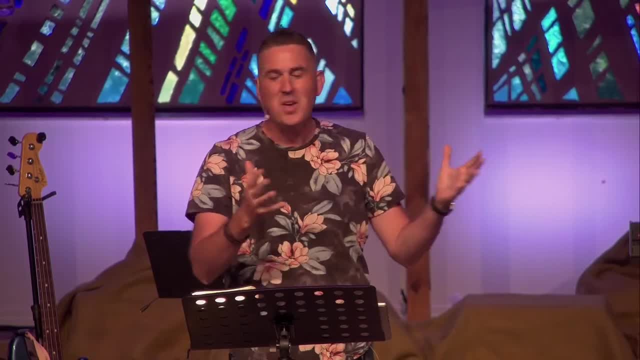 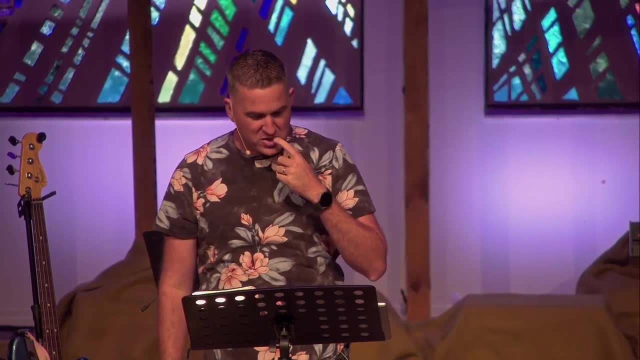 We're gonna be in constant communication and fellowship. Try it out, See how it works. Maybe it's helpful for you, like it's been helpful for me. One last one was Marcy Rahill, Alex, who preached here a few weeks ago. 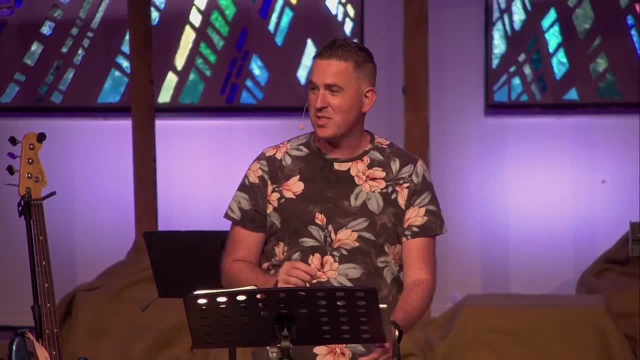 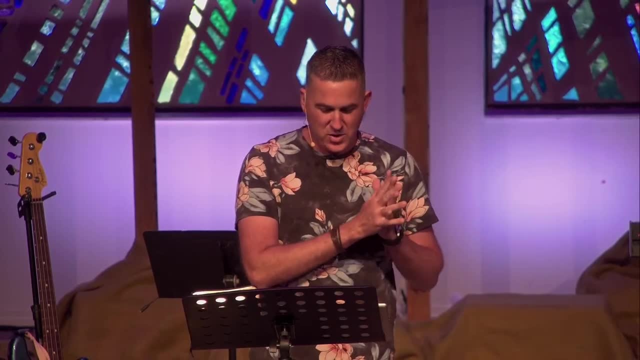 his wife said there's an app that she uses called Lectio 365.. If you like more of an ancient sacred book of worship approach, that's a good one there too. The last one I'm gonna recommend that we're gonna apply this in the Philemon is: you can do. 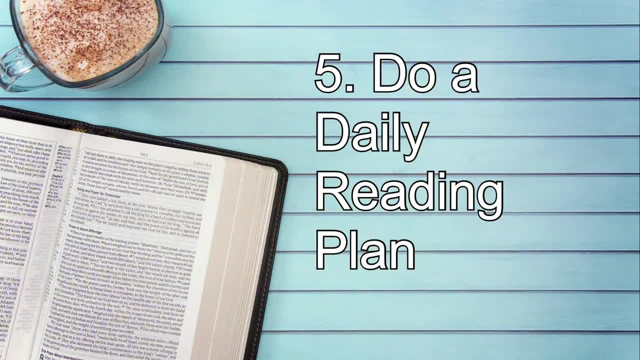 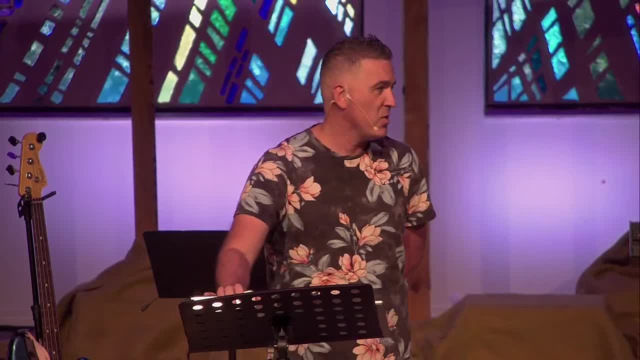 a daily reading plan of the Bible. Most of these- a great resource is perhaps the back of your Bible that you can just go through and check box. I will tell you, reading the Bible in a year is kind of a lot. It really is. 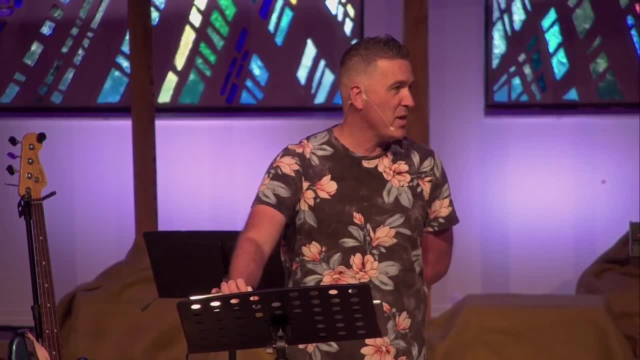 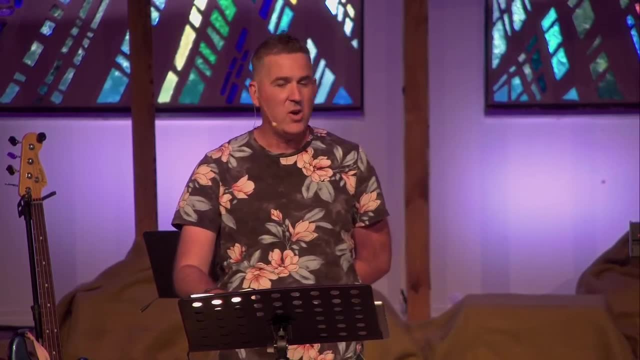 Like you're talking: almost five chapters a day to get through the Bible in the year. Getting through the Bible in two years is a little bit more of a bite-size approach, but it's a great challenge if you wanna get through the Bible. Nikki Gumbel has a great one. 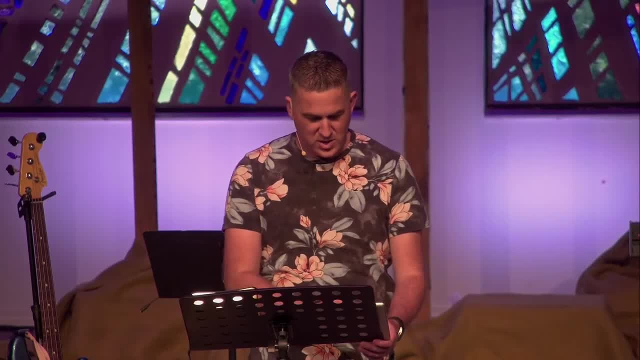 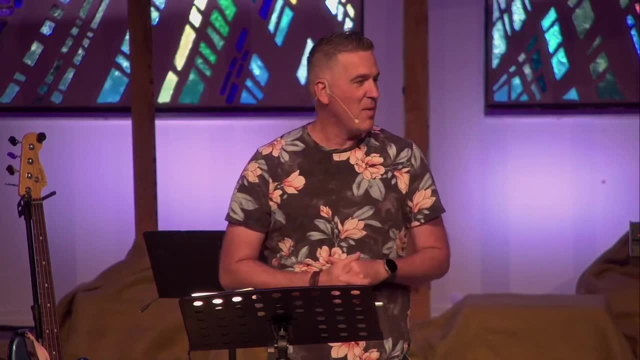 My wife does. what is it she does? The Bible Recap. thank you that you guys know The Bible Recap. in fact, when I was working on this message, I heard from the other room: hey, Bible readers, this is Laretz Terah Lee Cobble. 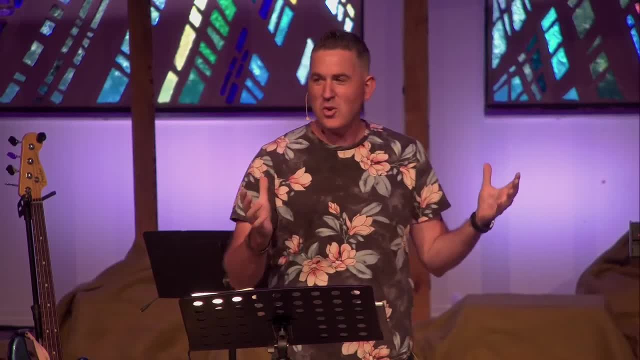 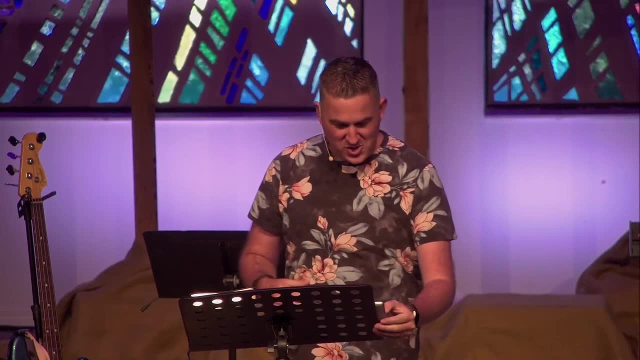 and I hear that every single day. It gets a little annoying after this many days, but I also praise God that my wife is reading the Bible each and every day, And so I'm just trying to think through. there's just so many different things. 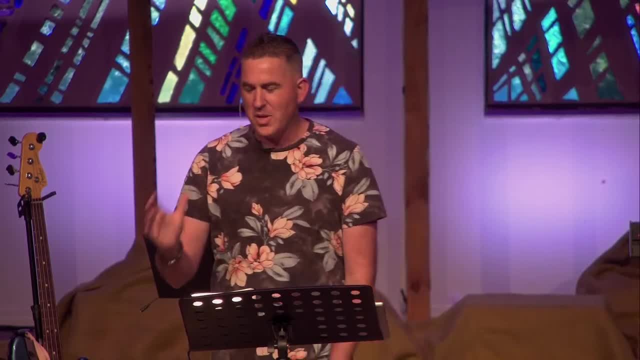 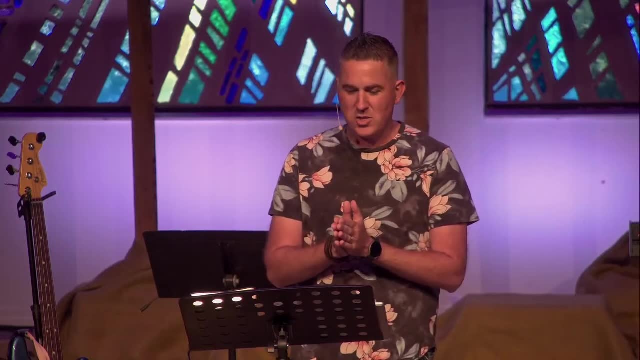 I'm just trying to share with you the idea that please, before the end of today, have your plan, Go through that time, the place, but then also make your decision on what you're going to study. And let me tell you this: 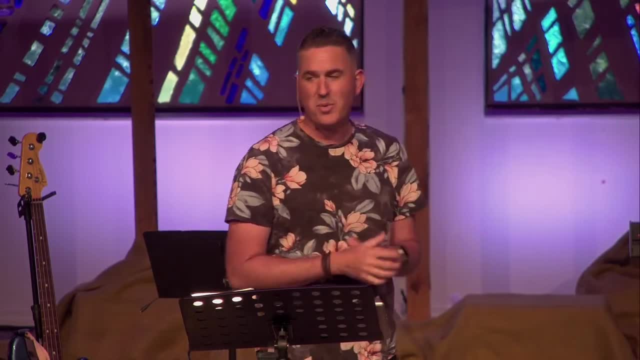 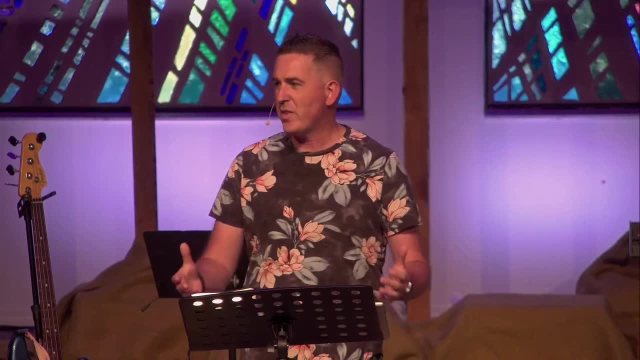 if what you're doing isn't working. change your plan. If you get bored in what you're doing, if you wake up and you're like, oh, I just don't wanna read this again, maybe get in a different book, maybe try a different plan. 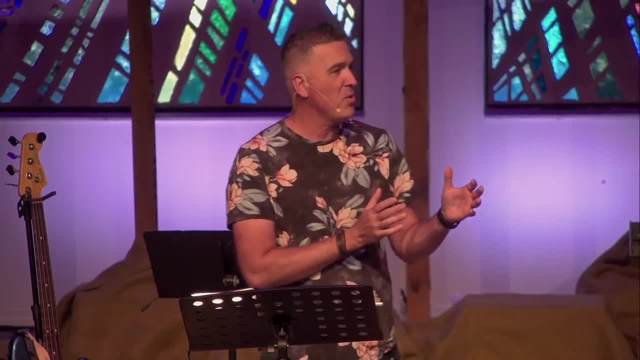 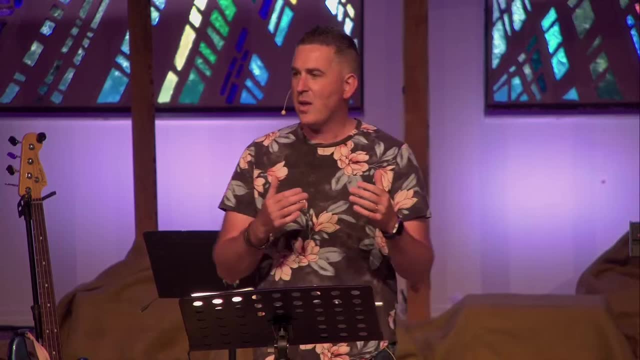 Maybe for you reading through an entire book, an entire book of the Bible, just is really difficult for you at this stage of life. Then maybe just try getting into a study on forgiveness and allow these different studies Find that plan that when you wake up each and every day. 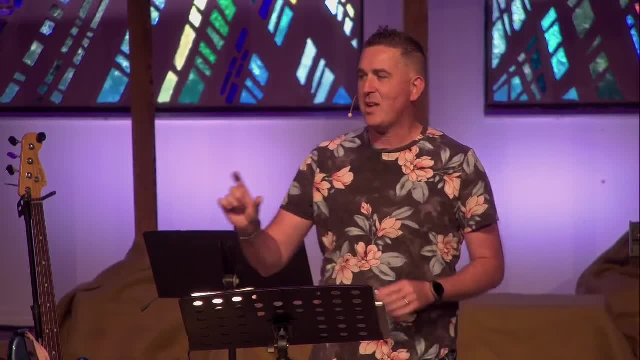 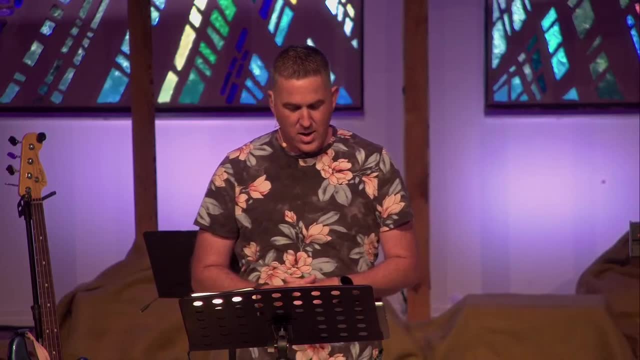 you're thinking, man, I can't wait to get in God's word, because I can't imagine going into my day without spending that time with the Lord and find that plan that works for you. So you've got your good translation, you've got your place and you're ready for your plan. 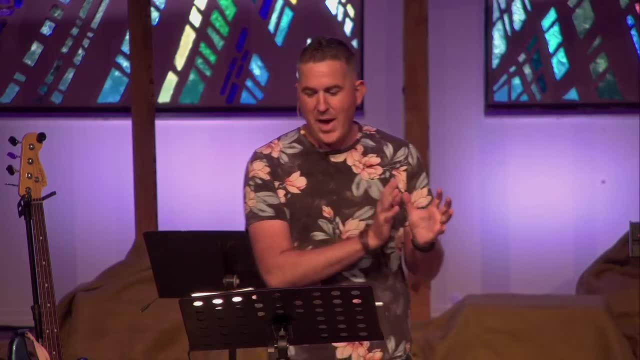 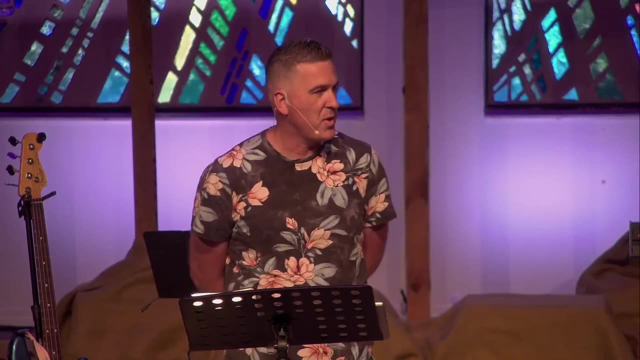 You're ready to apply this into the book of Philemon, And so, as we're getting back in, we're gonna start at verse 12.. As we're reading the book of Philemon, we ask the questions of who wrote the book of Philemon. 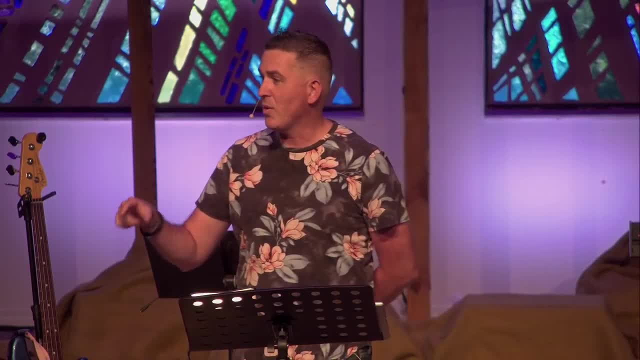 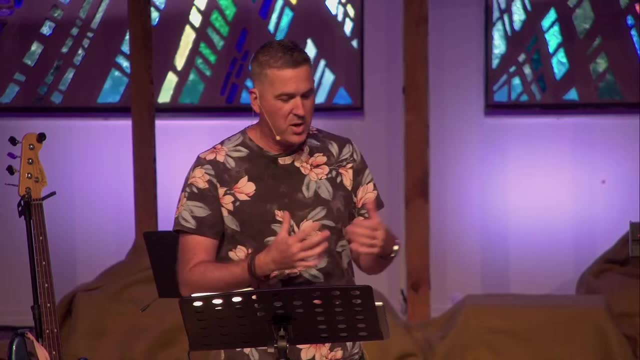 And it was Paul, the apostle. Paul wrote this. Who was it written to? It was written to the person, Philemon. And what's the literature type? The literature type is it was a correspondence, it was a letter. What do we know about Philemon? 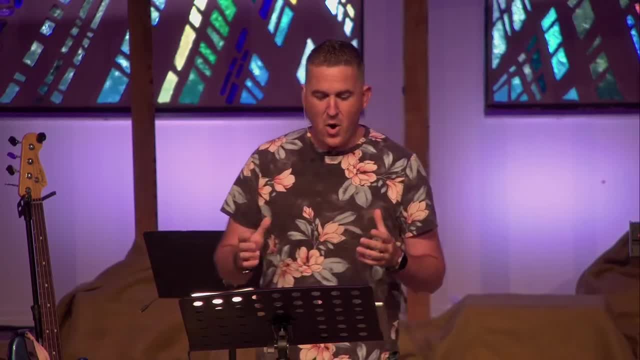 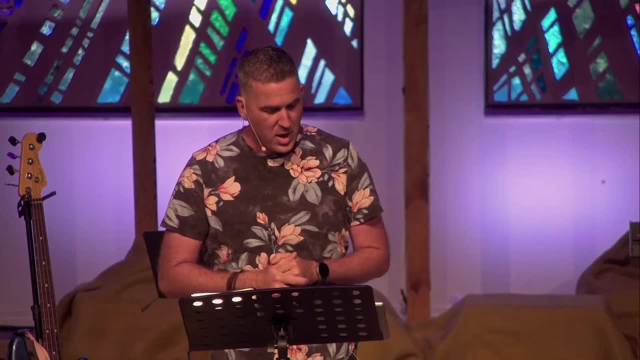 We know that Philemon was a wealthy, wealthy man. We know that Paul led him to Christ And we know that he had a pretty big house, that he could have church in his home, And we also know that he had a person who worked for him. 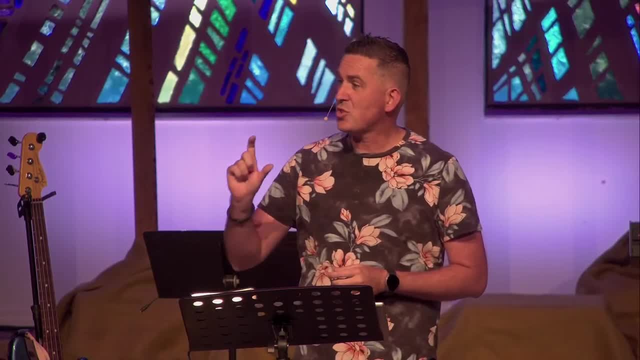 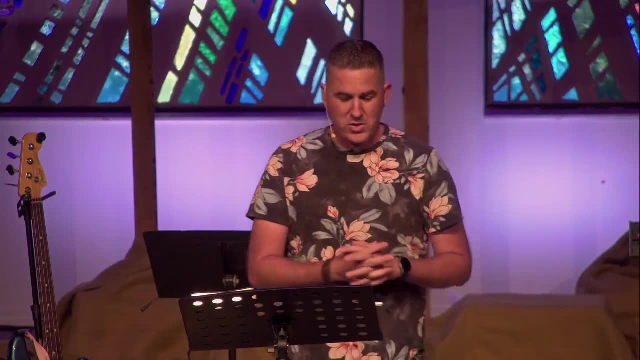 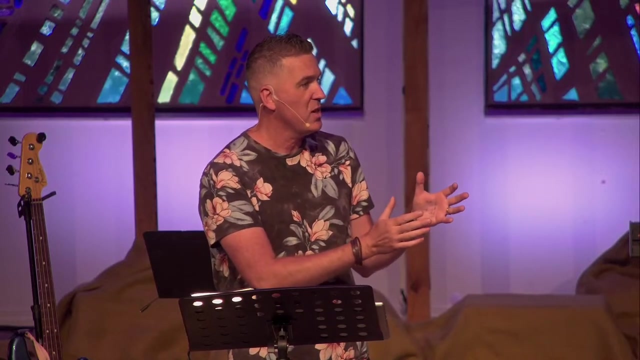 whose name was Onesimus. We know that this individual stole from Philemon and then ran away and escaped to Rome, And what we learn in the first 11 verses is that in Rome, Onesimus met Paul. Paul introduced him to Jesus. 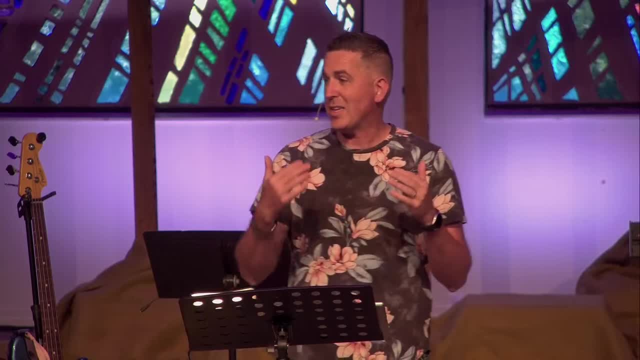 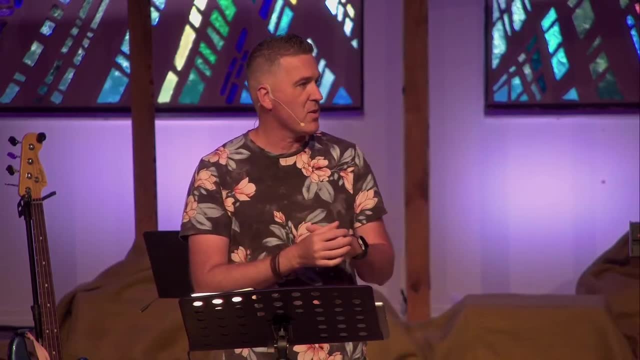 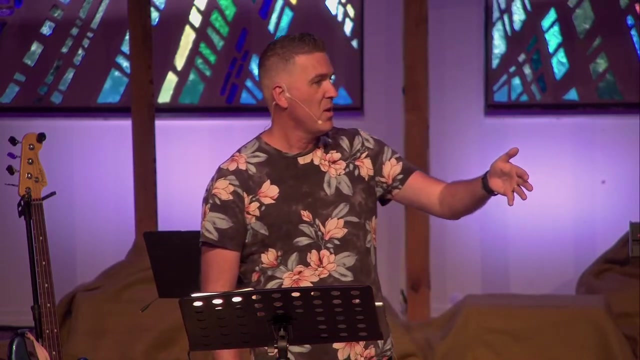 And Onesimus accepted the word of God, accepted salvation and gave his life to following Jesus. So what's the purpose of this letter? The purpose of this letter was that Paul is asking Philemon to forgive Onesimus for what he had done. 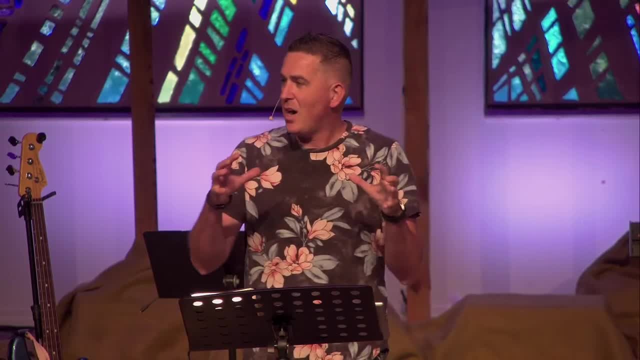 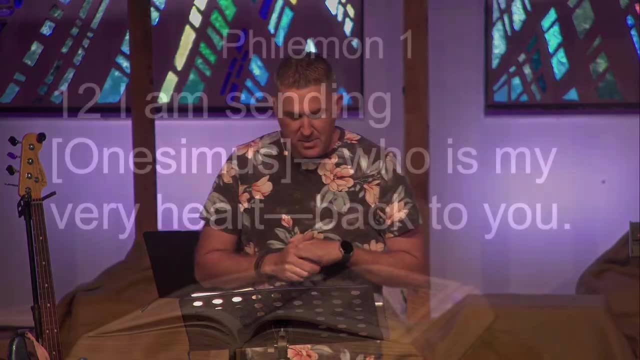 for stealing from him and then running away, And so that's the context that this whole book is in. Let's look at verse 12.. It says: Paul says I am sinning. I am sinning Onesimus, who is my very heart, back to you. 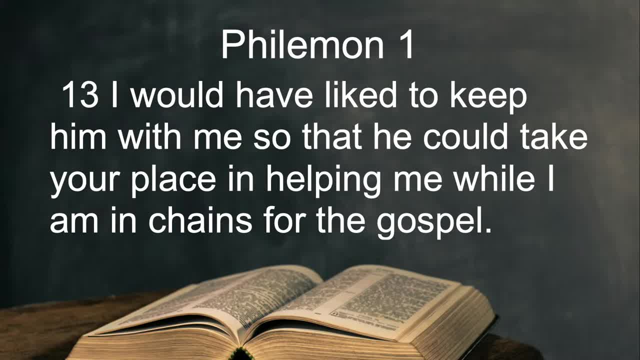 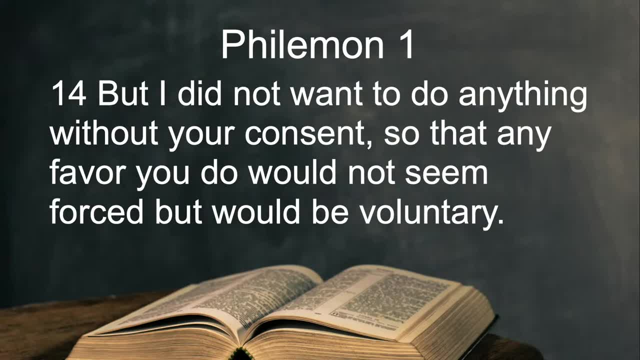 I would have liked to keep him with me so that he could take your place in helping me while I am in change for the gospel, But I did not want to do anything without your consent, so that any favor you would do would not seem forced but would be voluntary. 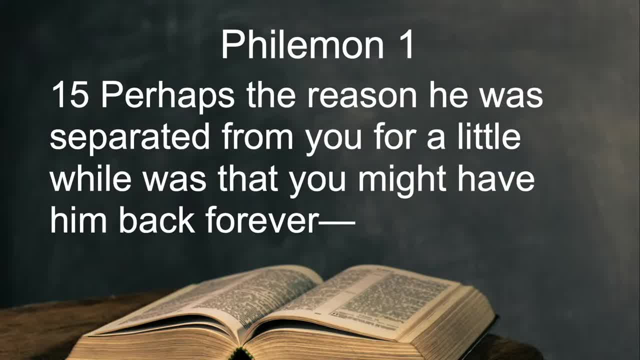 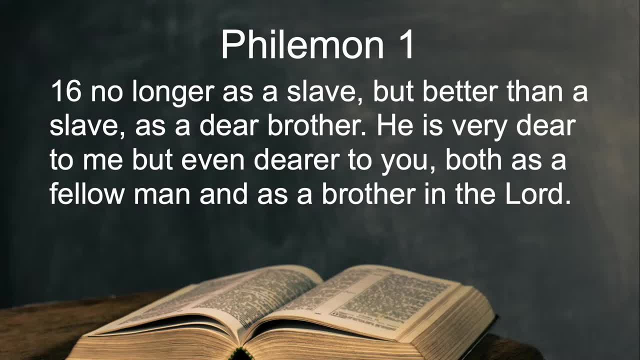 Perhaps the reason he has separated from you for a little while was that you might have him back forever, no longer as a slave, but better than a slave. as a dear brother. He is very dear to me, but even dearer to you. 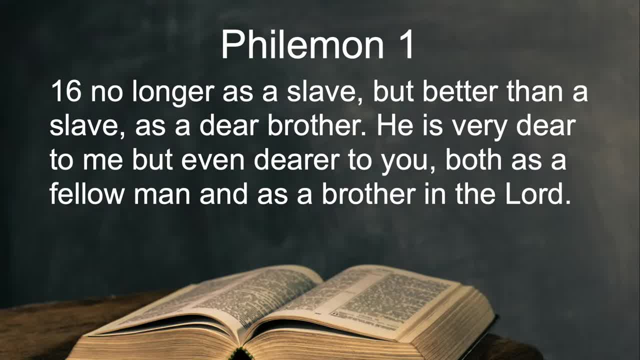 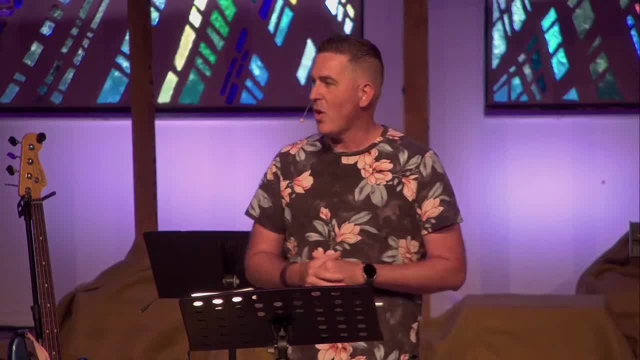 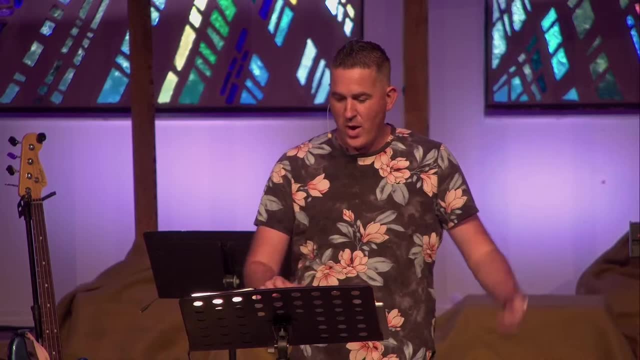 both as a fellow man and as a brother of the Lord. So you can see there's some language there. He's trying to help Philemon go from this person who wronged him, this person who stole from him and then escaped and ran away. 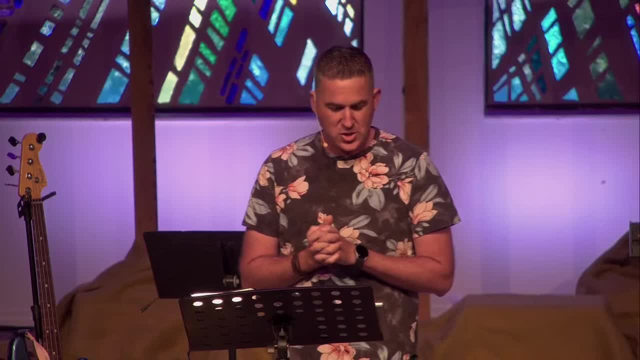 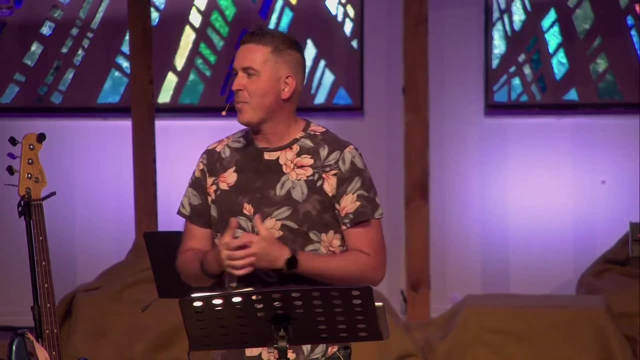 and he's trying to help him understand this relationship. So one of the things that I want to teach you is that when you're looking at your Bible, is that you have the opportunity for doing cross references. I'll show you a picture of my Bible. 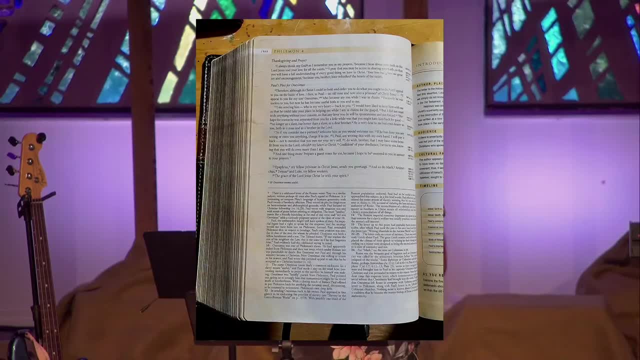 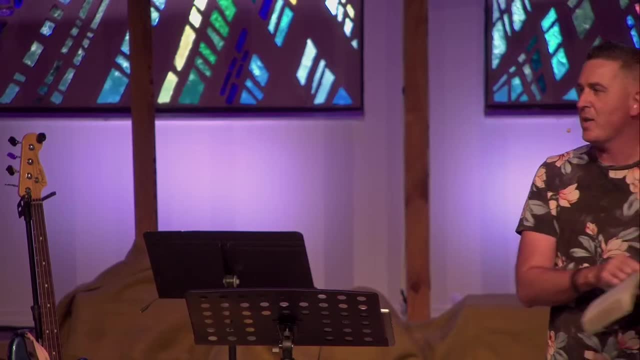 but you can't see anything. but that's my Bible. And if you've ever noticed in your Bible, at the middle section there'll be other verses, right there on the spine, right there on the binding, You'll see that there's some other verses that are there. 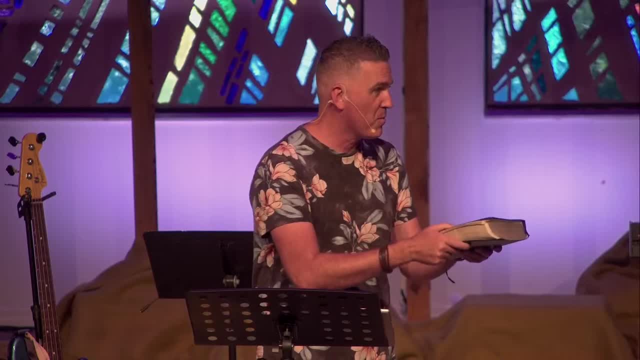 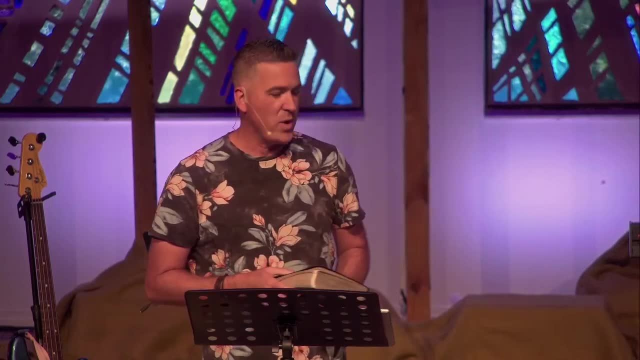 And what the author of- not the Bible, but of your book, your compilation- is that he's giving you other verses that connect with the text that you're reading, And so it's a really helpful thing If you don't understand what you're reading. 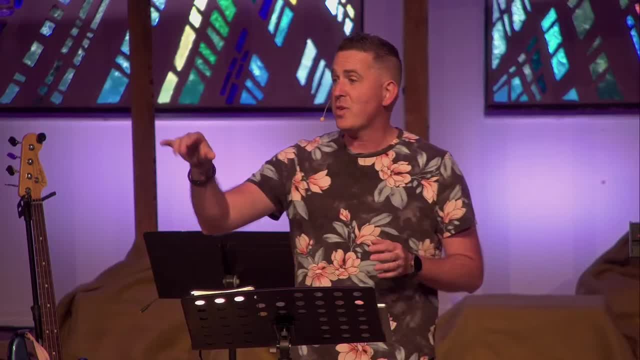 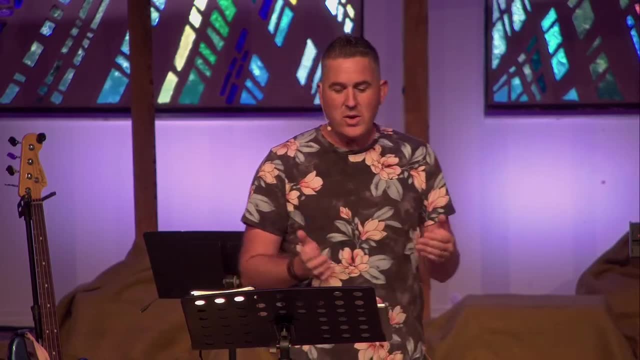 you can take those verses on the inside and even Bible Gateway will have little buttons you can click and it pops up those verses right on your screen for you to see. You can look at other verses that will give you context to other stories. 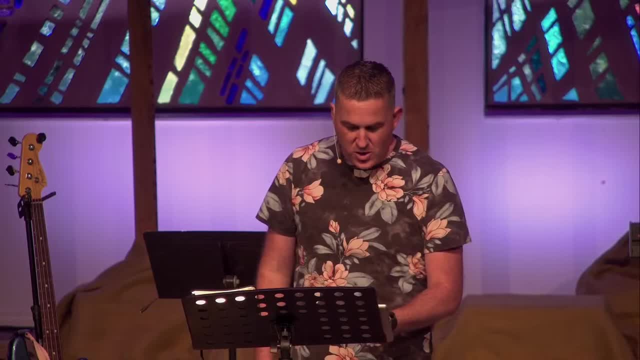 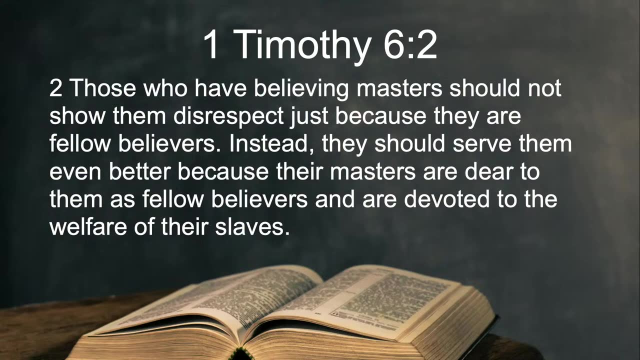 There's scripture that relates with this idea, So you can see if you go to Timothy. there's a verse that says: those who have been believing masters should not show them disrespect just because they are fellow believers. Instead, they should serve them even better. 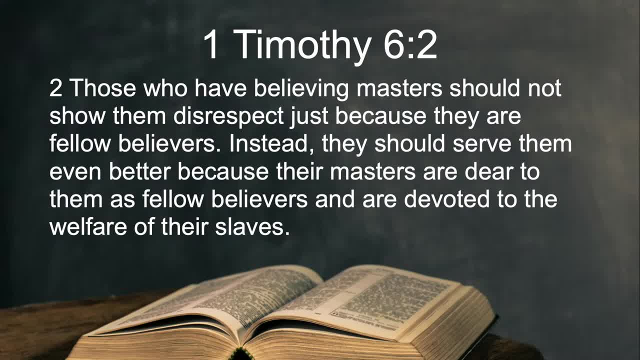 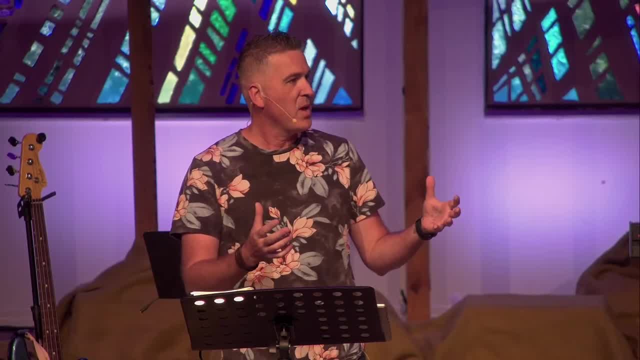 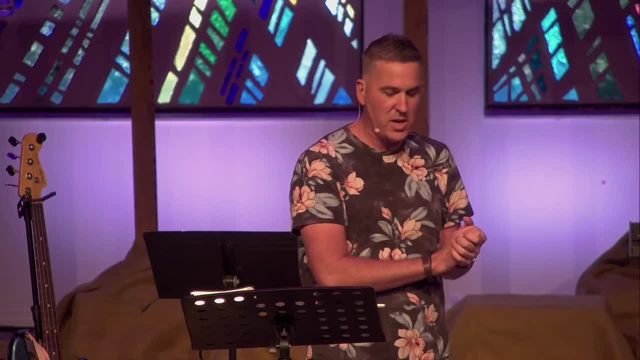 because their masters are dear to them as fellow believers and are devoted to the welfare of their slaves. And I just have to say this verse is not condoning slavery. This verse was dealing with much more of a boss-employee relationship than we understand American slavery. 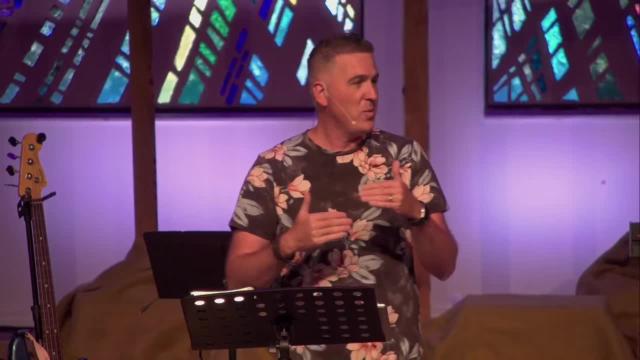 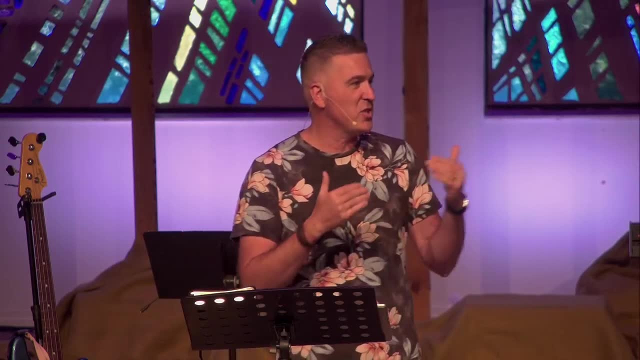 And this is saying that just because you're both believers, well, some of you might have a boss that attends our church, right. That doesn't mean that when you go to work, all of a sudden you disrespect them as an equal. No, we still recognize that there's still those relationships. 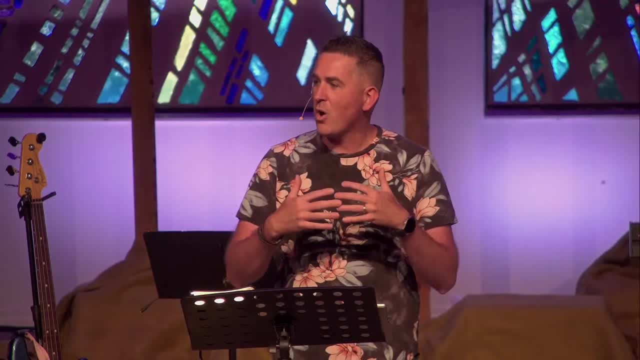 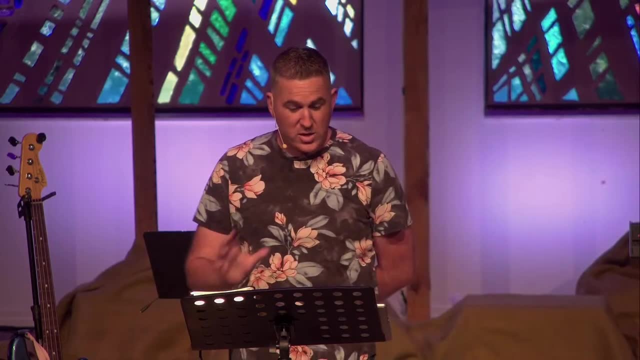 that we still have levels of authority in our society, but that we're also believers in Christ and that we can come together in that moment. And, Matthew, it was another cross-reference from my Bible. it says: but you are not to be called rabbi. 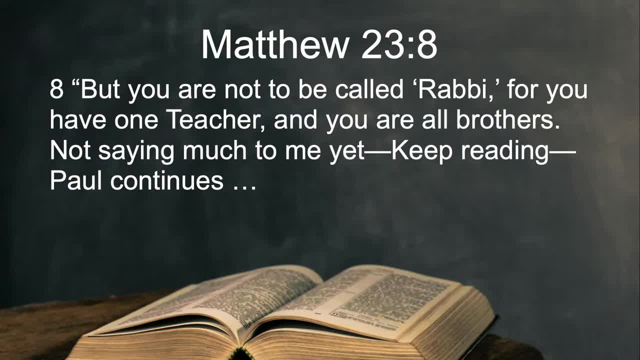 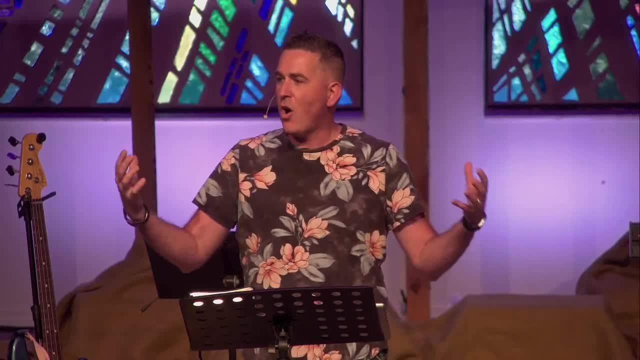 for you have one teacher and you are all brothers, And so it's given us that cross-reference, that there's this teaching across the entire New Testament that we are all brothers and sisters in Christ Jesus. And then we go to verse 18.. 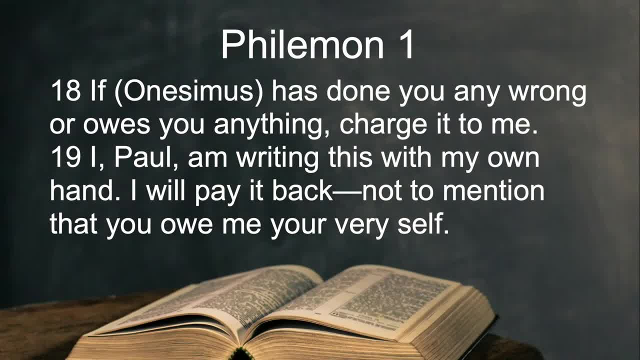 If Onesimus had done you any wrong. Paul writes or owes you anything, charge it to me. I, Paul, am writing this to you with my own hand. I will pay it back, not to mention that you owe me your very self. 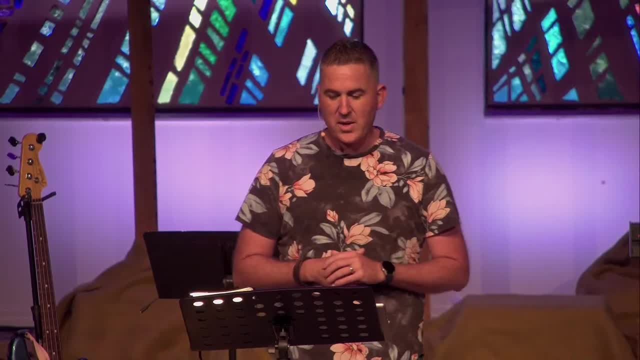 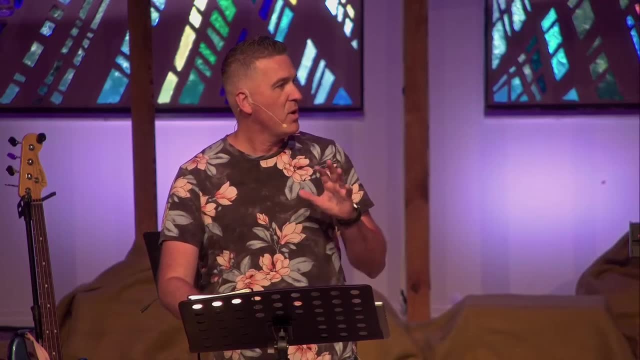 So Paul says: I know he has a debt and I'll pay it. And I'm gonna do one more cross-reference here. The next one: right on verse 18,. it said in my Bible, Isaiah 53.. I go to Isaiah 53, verse four, and it says: 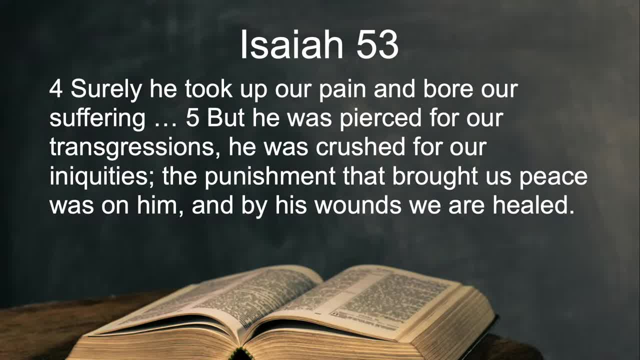 surely he took up our pain and bore our suffering? but he was. he was pierced for our transgressions. He was crushed for our iniquities. The punishment that has brought us peace was on him, And by his wounds we are healed. 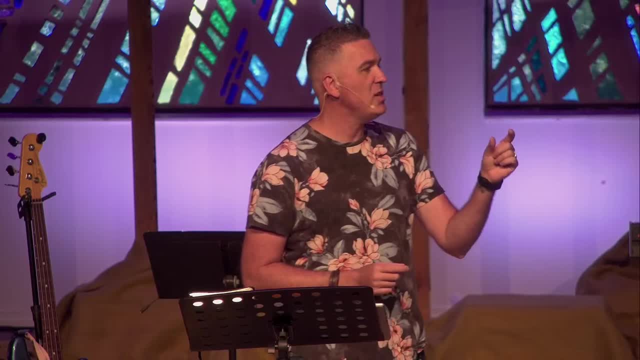 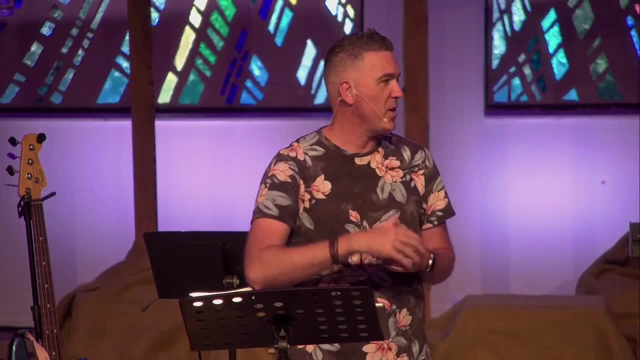 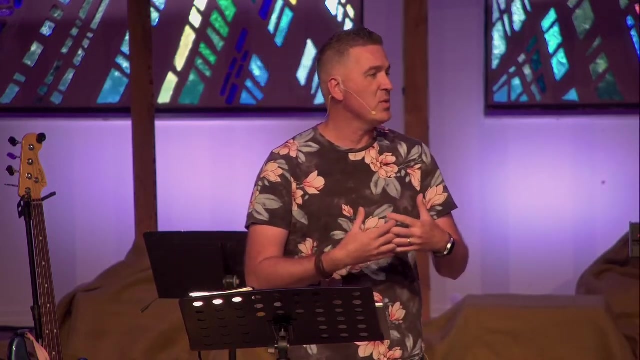 So what we see here is Paul is recognizing that Jesus took all of our sins, He paid the price and he choose to forgive us. And the reason why Paul is saying I'll take on his debt is because Paul knew that he was a sinner. 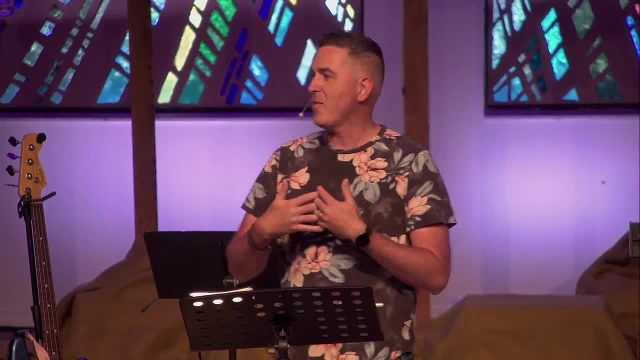 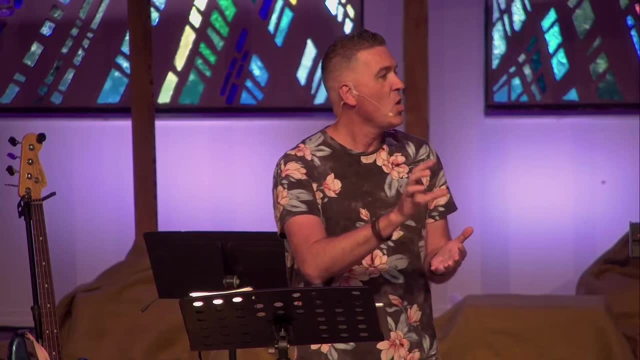 that had been forgiven for much. And he said: if I have been forgiven for what I have done wrong, let me pay the price for what he has done wrong. And Paul is identifying with the ministry of Jesus Christ and said: I will do likewise. 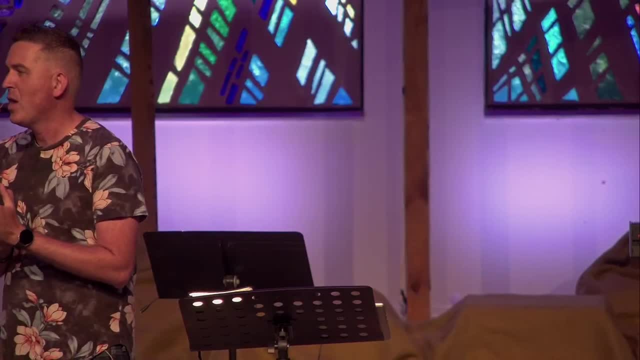 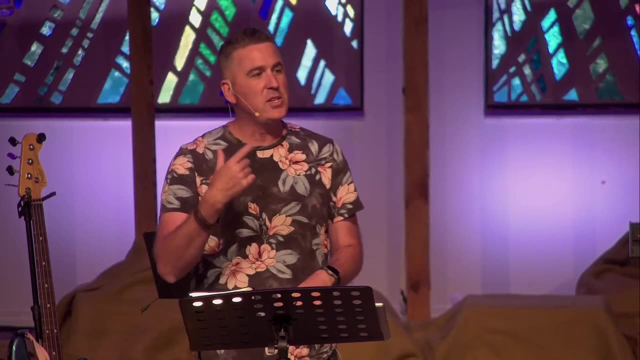 And that's exactly how we should always read our Bible. We should read our Bible from old to new Testament and say: what does this say about Jesus And what is this teaching me to do, based upon how it points to Jesus, One of the things we get in trouble. 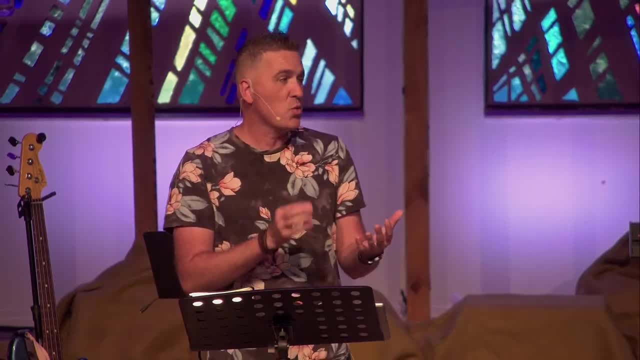 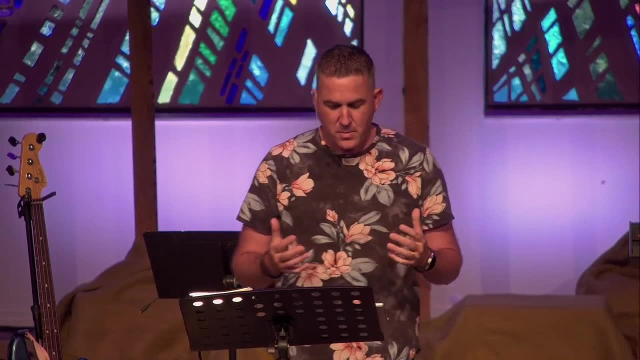 is when we try to think that everything in the Bible is written directly to us, instead of recognizing that it's all about Jesus and we apply it to our lives. In Philemon, we get three different characters here, And we can take these examples. 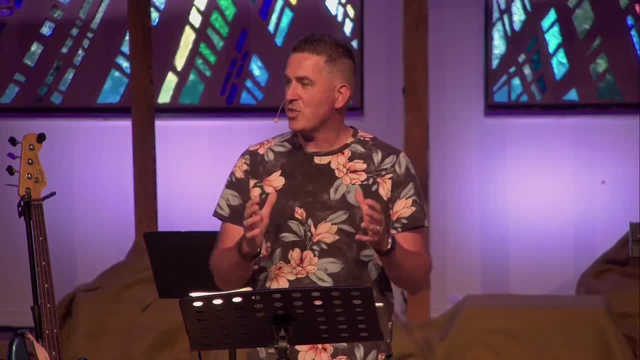 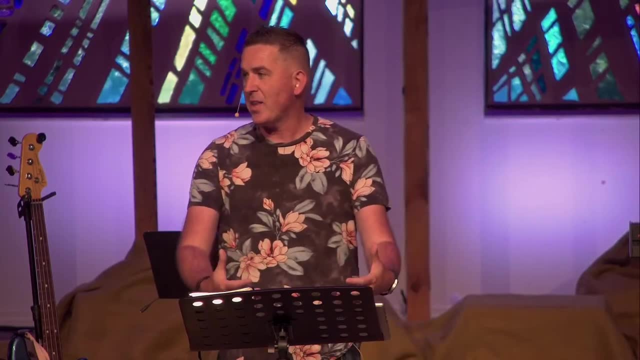 within the grace and forgiveness that we see in Jesus. And we can understand that there's a few different people here, and this is the living word of God That when I preach this message on Philemon, that different people in this room that are here 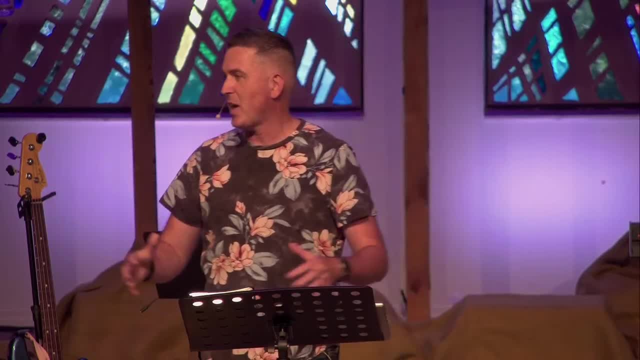 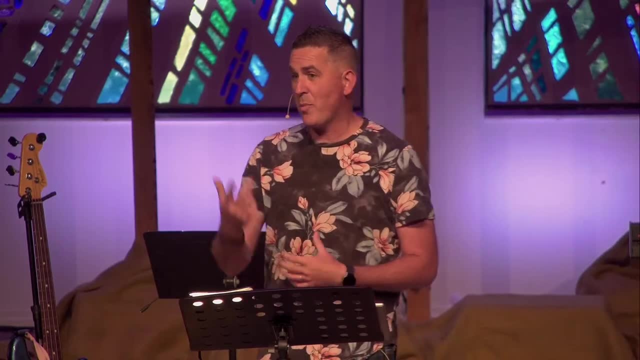 that are hearing this message online. they're in different circumstances in life And when I say these words, it connects with different people. And then all of a sudden, I'll have a week where a person comes up to me afterwards and be like: oh, I love your message. 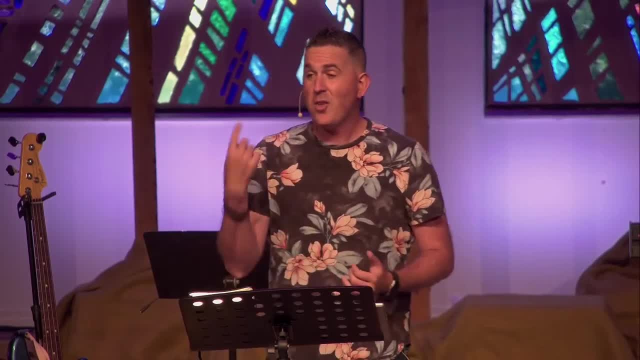 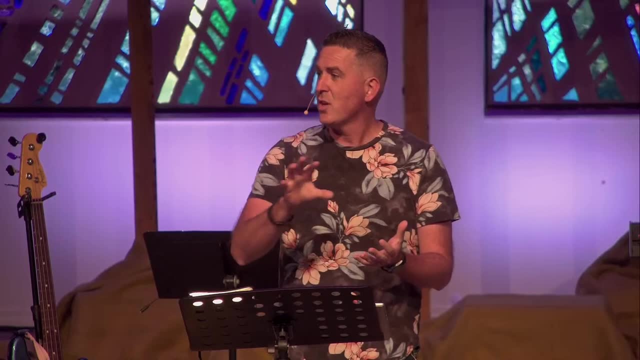 because it did this, this and this my life And it meant this to me. And the whole time I'm saying praise God. I had no idea that I preached any of those words, But God uses the living word of God to transform, not just inform. 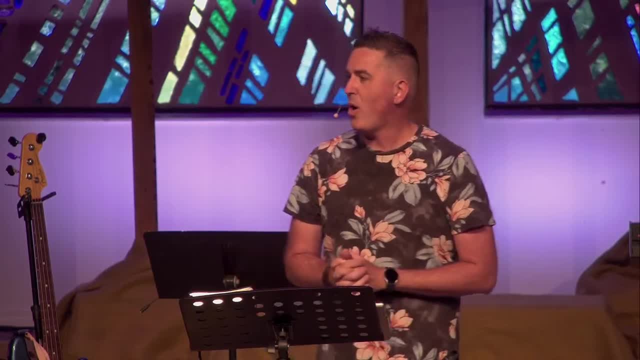 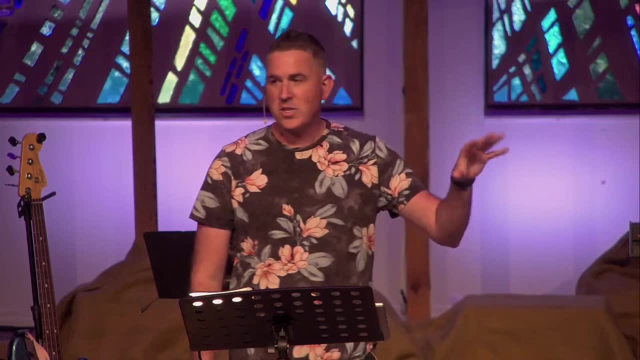 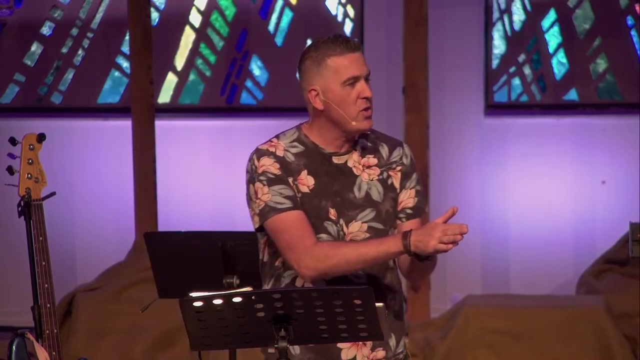 And so he's using God's word. So what is Paul in this text? Paul's a person who is risking his entire reputation for the sake of another, And maybe God is gonna speak to you in this text at this time and say: I'm calling you out. 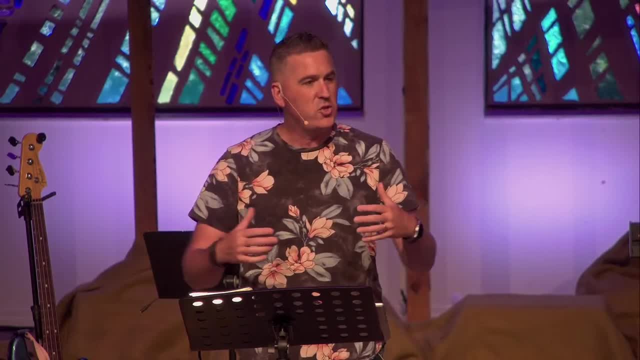 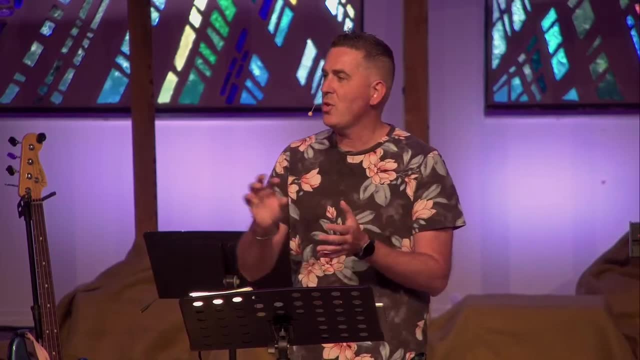 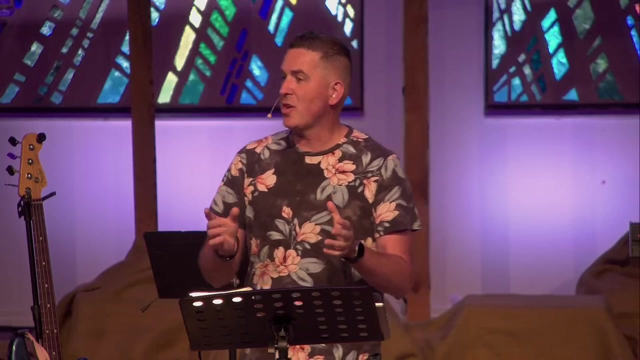 to go on behalf of another and I want you to help them seek forgiveness. I want them to seek a relationship that's been broken and God's calling you to come alongside another. Or you look at Onesimus: He was the slave that legally could have been branded. 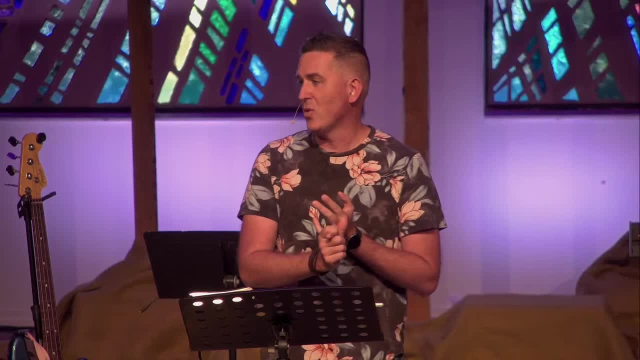 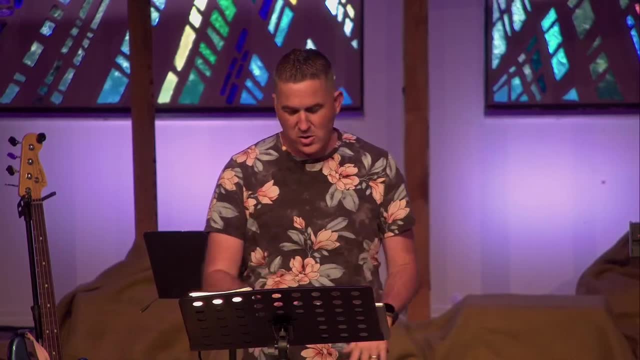 on the forehead with an F. He could have been beaten or even killed. And you're looking at this and saying, man, I'm a person right now who needs forgiveness And you can understand this text from his perspective, Or maybe you can understand this text. 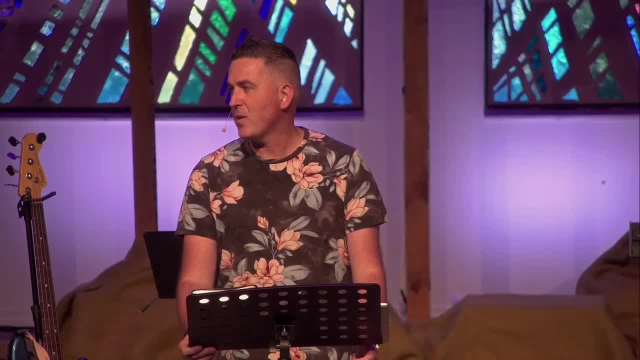 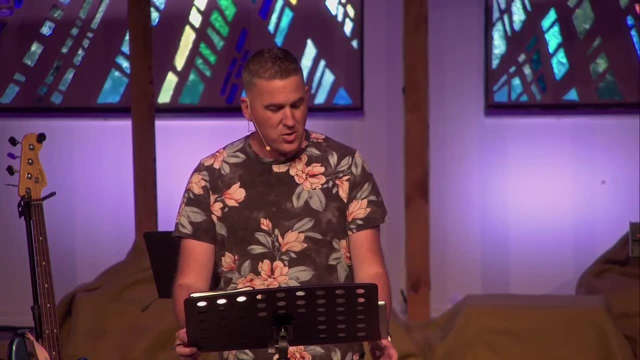 from the perspective of Philemon, Who's being called to forgive. Maybe a person has hurt you, stolen from you, lied to you, cheated on you, And God is speaking to you right now and saying that you need to be the person. 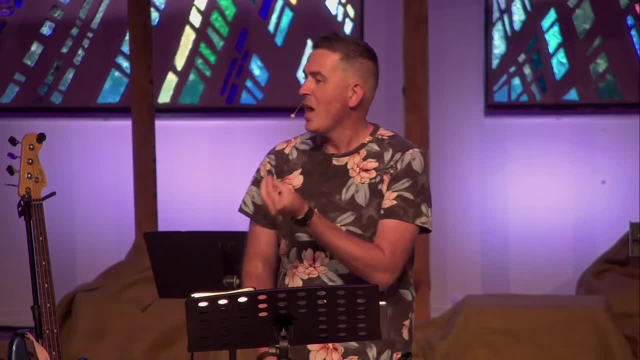 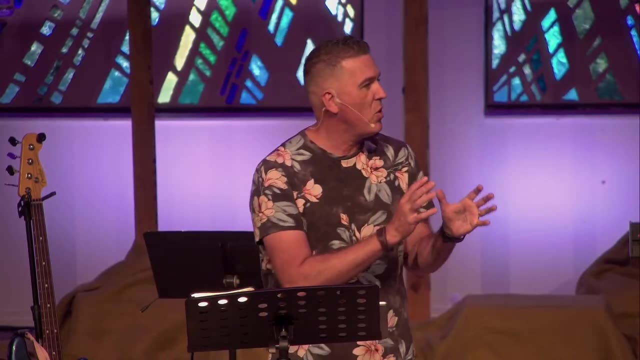 that is gonna step in the place of Philemon and that you are gonna begin to have a forgiving heart so that you can have a forgiving action. You know that you understand that God is calling you to be like Jesus and to forgive, because our transgressions were forgiven. 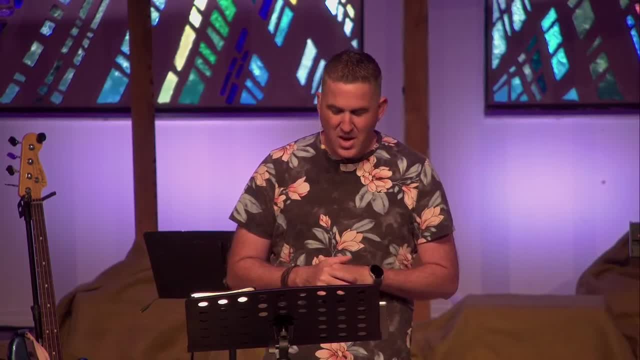 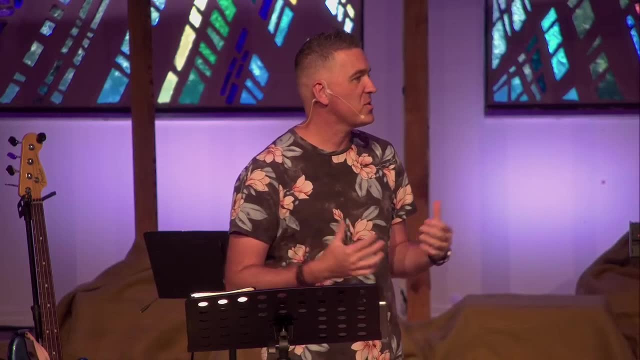 The last thing I'm gonna teach you, and then we'll come back to it And then we'll close. Another tool that's great to study in God's word is man. you're reading this text and you're like I wonder what else God's word says about forgiveness. 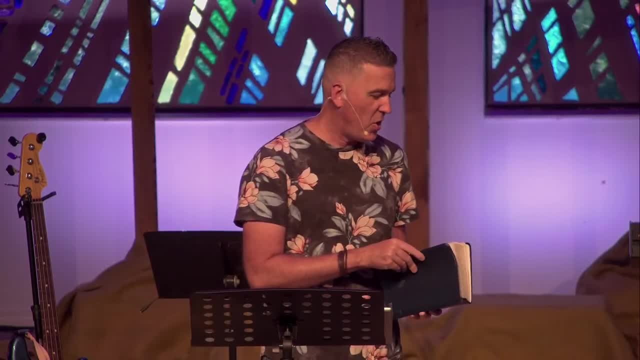 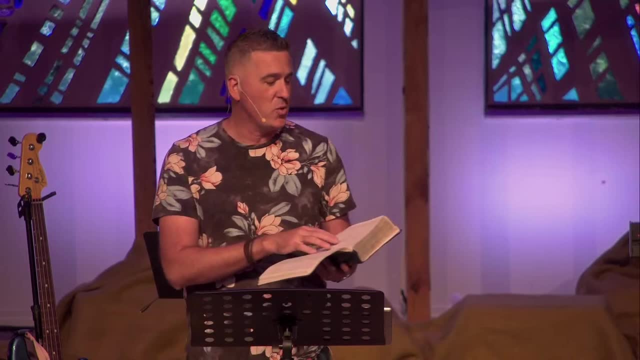 And you can go to the very back of many Bibles and it's called the concordance, And this is really where I started writing sermons, Like when I was like a teenager or younger. this is the only tool that I had was literally like this exact Bible. 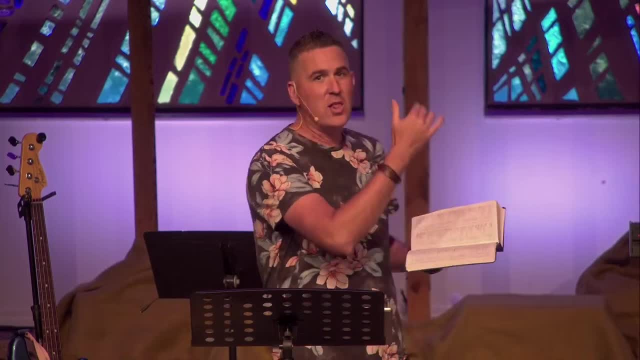 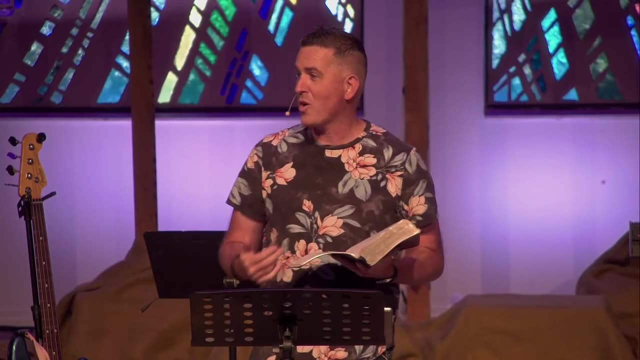 And I would go to the back. Here's a picture. I can't really see it, But I looked up the word And you can see the word forgiveness in every place in scripture that that word is used, And so I just would start going through Old and New Testament. 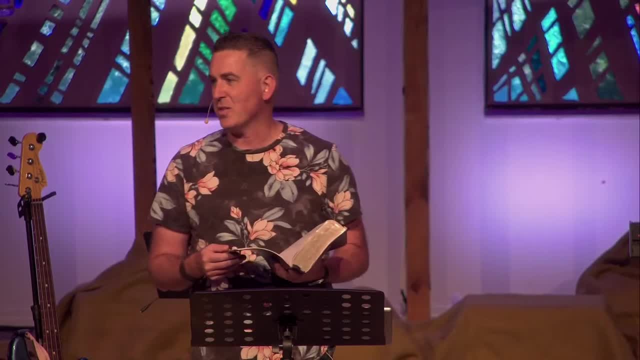 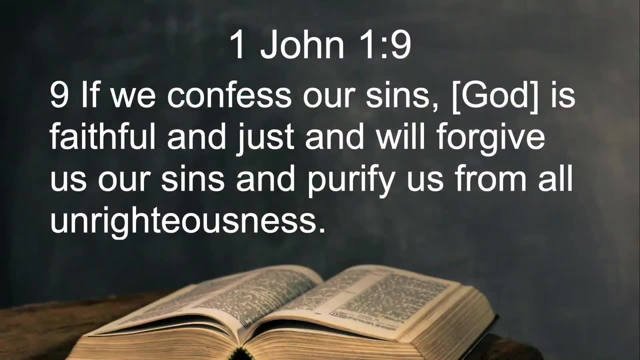 to see what God was teaching on forgiveness, And as I worked through that text, I found verses like 1 John 1 that says: if we confess our sins, God is faithful and just and will forgive us of our sins and purify us from all unrighteousness. 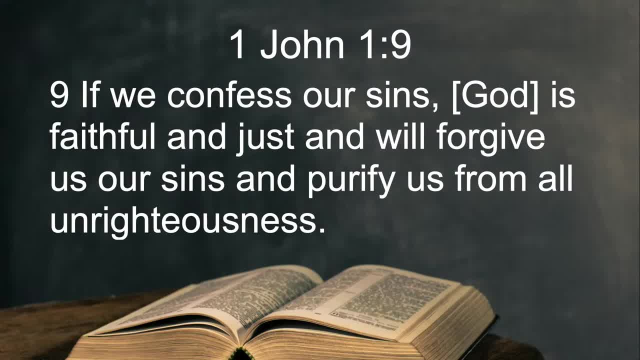 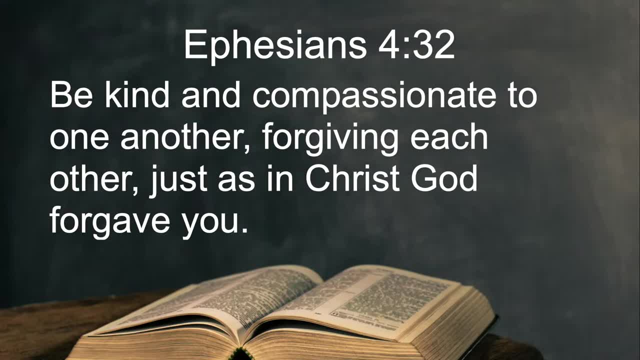 I continue to work from the concordance and I found a verse that says: be kind and compassionate to one another, forgiving each other, just as in Christ God forgave you And I'm like man. that verse right there from Ephesians. 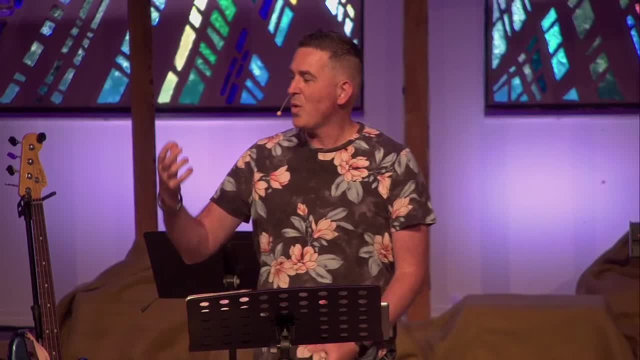 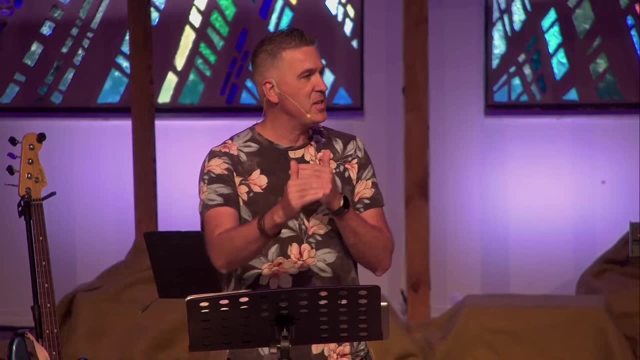 sounds just like what Paul is telling to Philemon about Onesimus in this context And you begin to see the depths of God. forgiveness, as now they always say like I want to go deeper in God's word. What does that even mean? 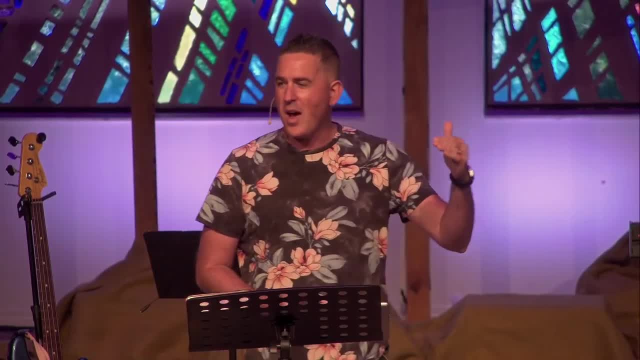 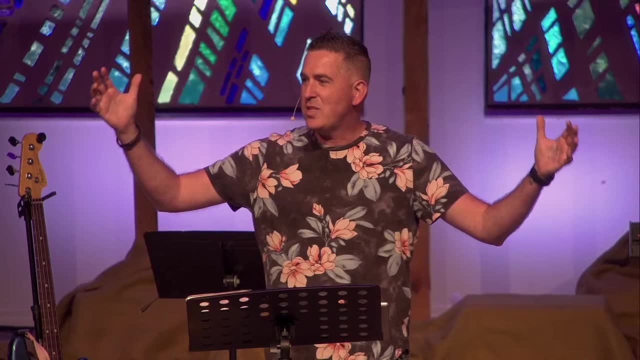 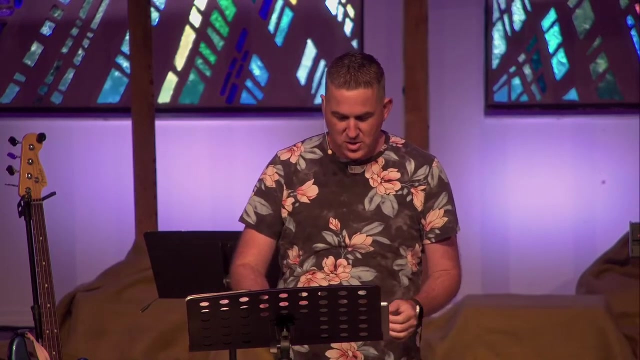 Well, here's an example. Is you start studying every verse in the Bible that talks about forgiveness And you're like, wow, I didn't realize how deep and wide God's grace and forgiveness was, that he calls us to forgive because we've been forgiven of much. 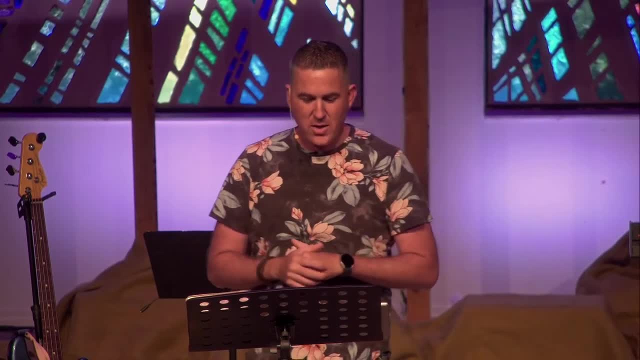 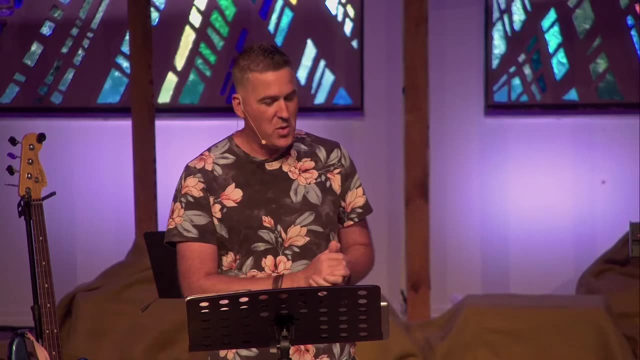 And you continue just to pour yourself and you understand that the Bible isn't just to inform us, but it's to transform us. And then the last thing is: I showed you last week that we can dig deeper. I've got commentaries. I've got commentaries. 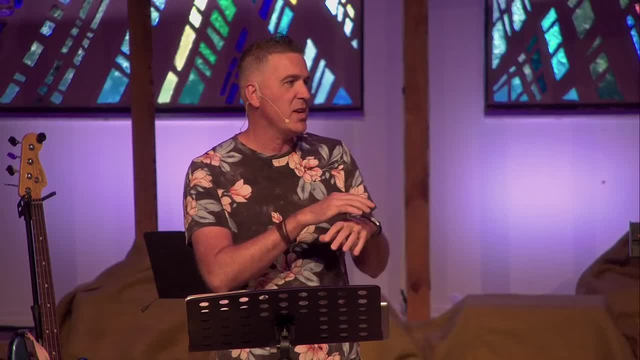 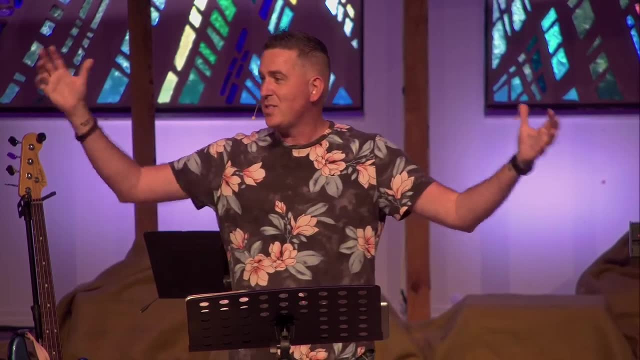 I've got commentaries that write 33 pages on one verse And they really just dig into all the Greek, all the Hebrew, all the correlations, all the historical documents that we have in existence. And I found one little Easter egg from Philemon. 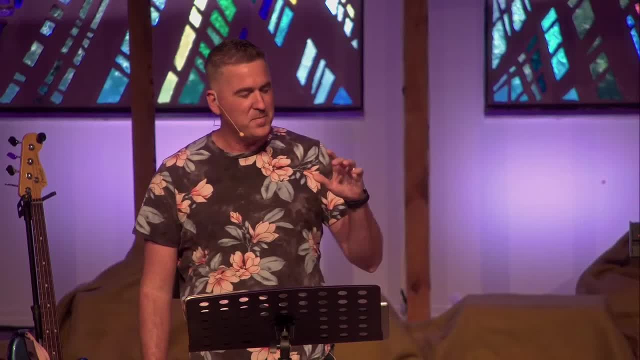 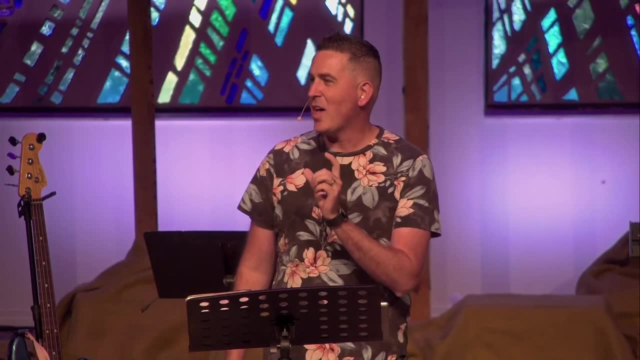 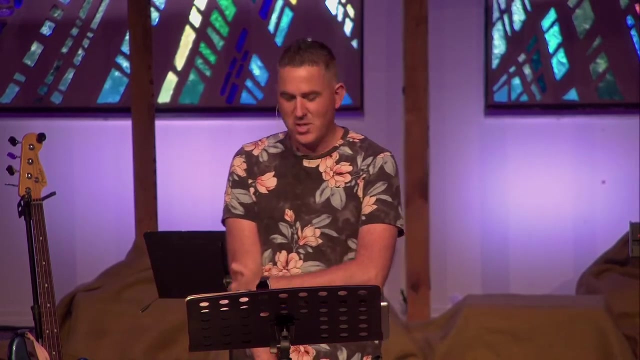 that I want to share with you, And this was going through the NIV life application commentary and just on the book of Philemon, And they have found a letter that, if you fast forward about 50 years from this story- and it was written by St Ignatius- He was the Bishop of Antioch. He became a famous martyr who also gave his life serving Jesus Christ. Ignatius was most likely a disciple who served directly underneath John. the Apostle John Ignatius wrote a letter to the church in Ephesus. 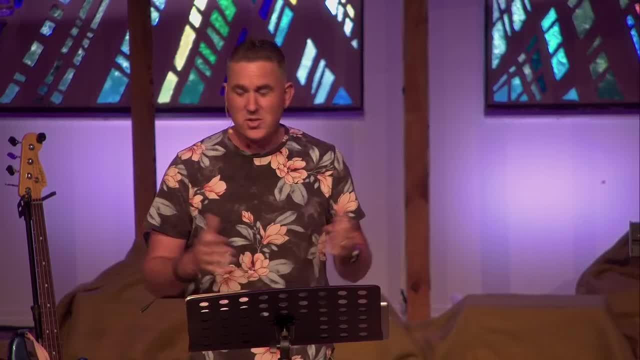 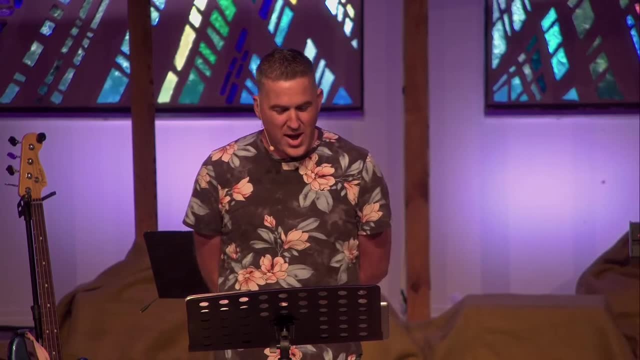 that we still have the copy of to this day, And so it's almost 2000 years old and we still have the letter. We still have the copy of the letter today In the letter Ignatius brags to the church in Ephesus. 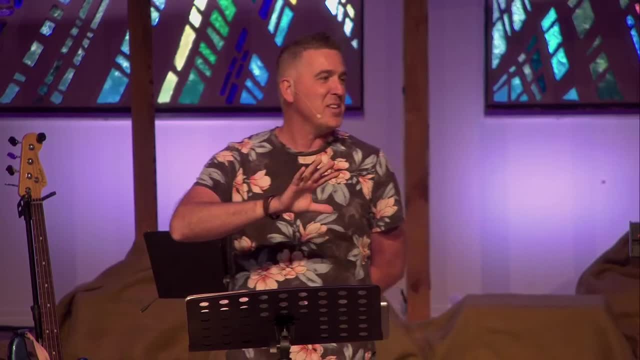 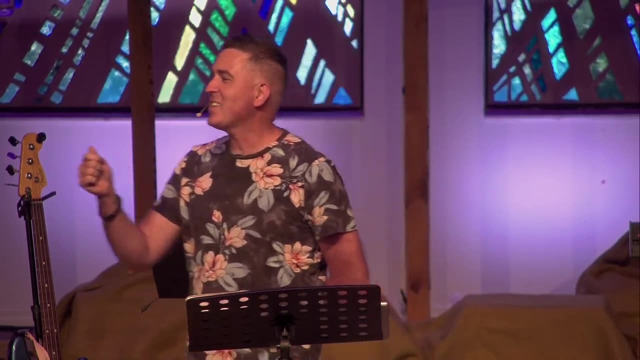 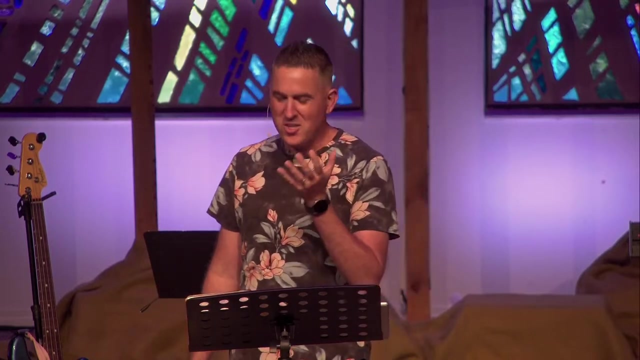 that they've got the best Bishop out of all the churches. And he actually writes a letter and says: your Bishop is a man of inexpressible love. And he says in the letter: blessed be God who granted unto you such an excellent Bishop. 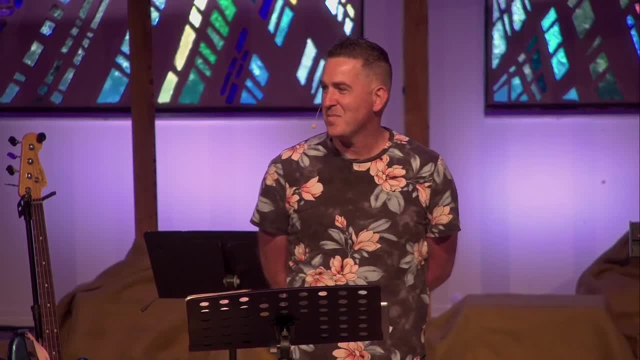 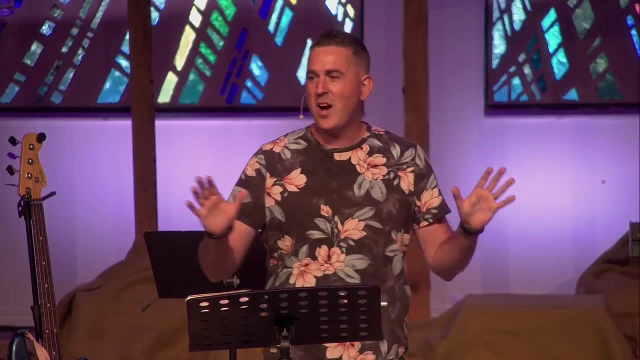 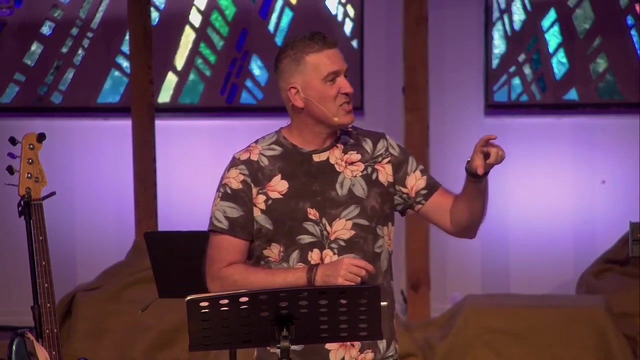 Can anybody guess the Bishop's name, Onesimus? you see, I can't tell you without like a shadow of doubt. I'm about 99.5% sure this is the same Onesimus. Why? Because Ignatius was a disciple of John. 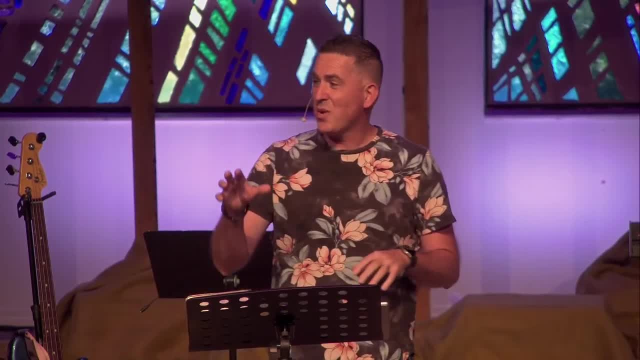 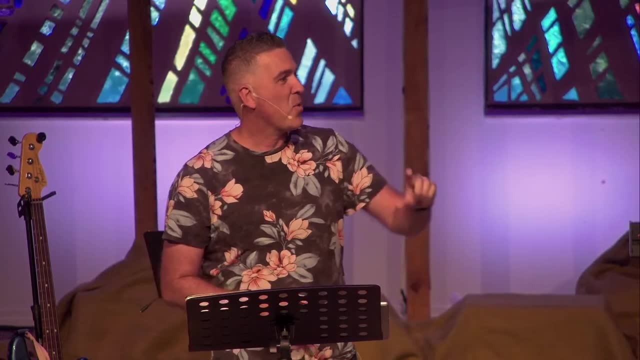 Onesimus was a disciple of John. You look at the regions, you look at the timeline and it all lines up that this is the same person, That the person that was the slave that went back to where Philemon was, which would be near Ephesus. 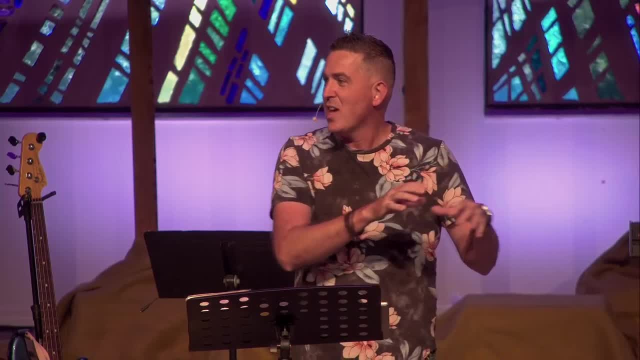 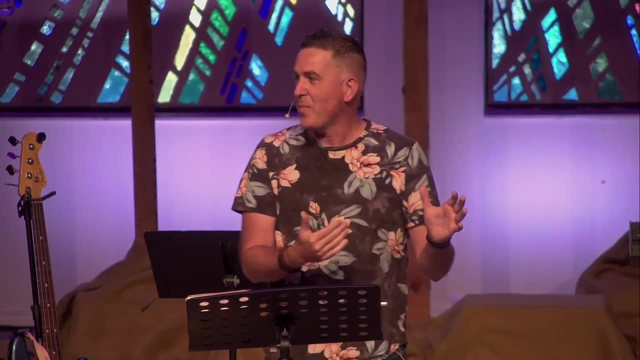 when that whole region of Galatia, that's where that church was, that all these pieces came together. And so then we can see, we can play, chosen for a minute and play the rest of the story- that what happens is he goes back to Philemon. 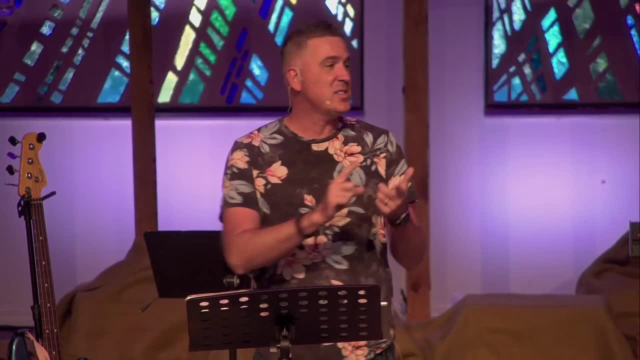 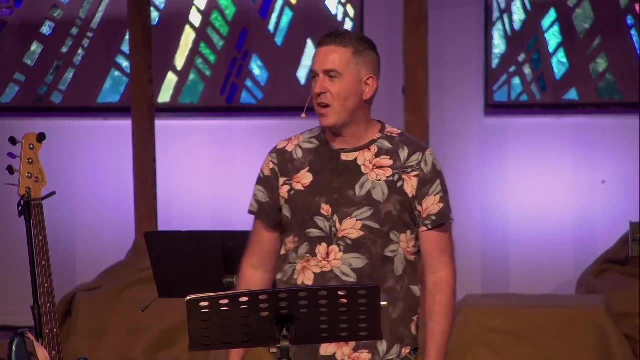 Philemon doesn't brand him with an F, doesn't have him beaten, doesn't have him killed, but he declares: you are a brother in Christ, and I forgive you for what you have done to me, For what you have done against me. 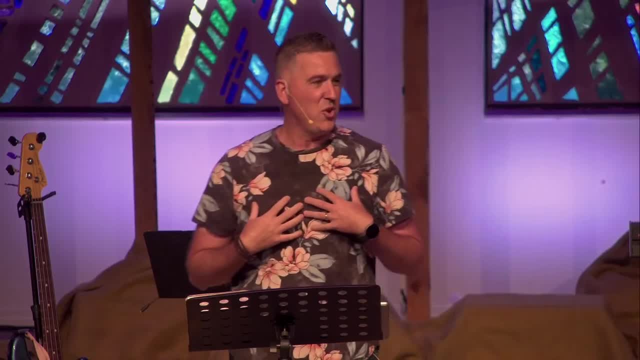 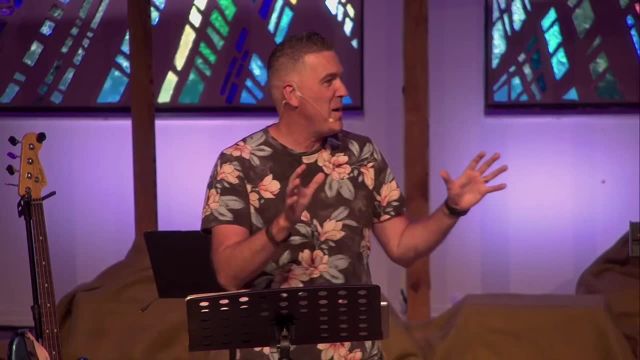 and I now accept you as a brother in Christ and I hold you close to my heart, And that you can see that Philemon perhaps even had the ability to send him out and be a church planter, to send him out to do great work. 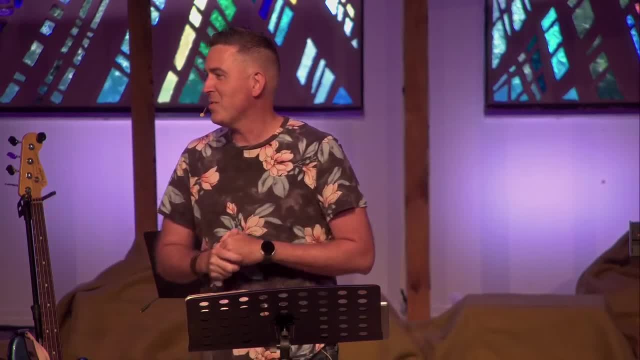 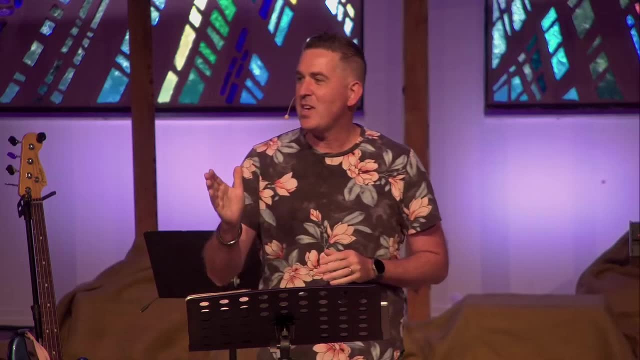 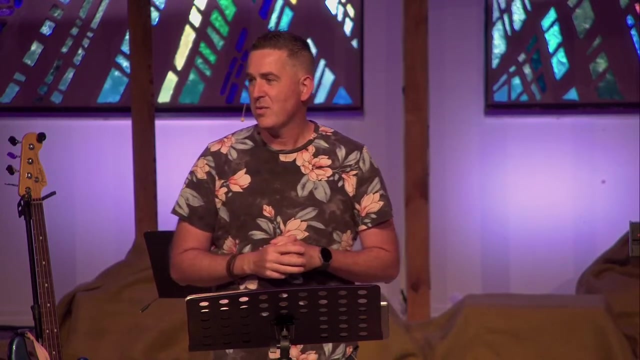 But it also said that this Bishop Onesimus was a person of inexpressible love. The Bible tells us that he who has been forgiven for much loves much, And I see people who have. they have health. they have health situations that bring them to the brink. 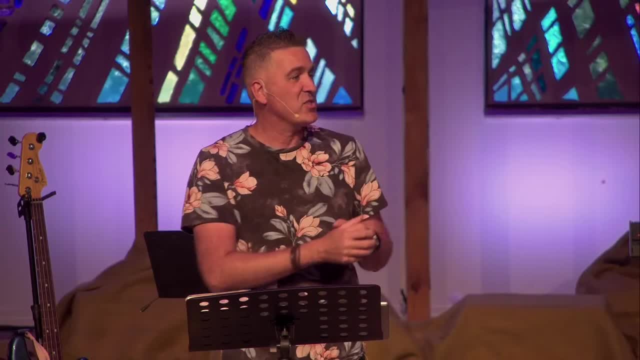 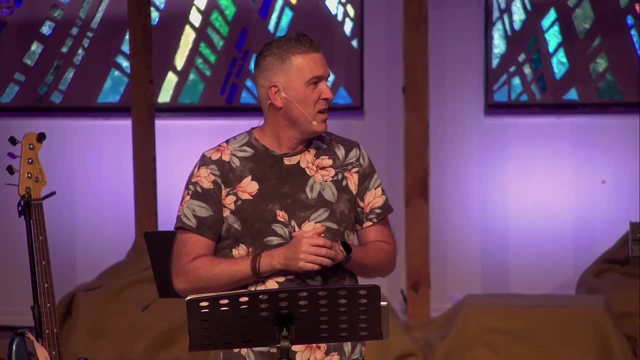 They don't know if they're gonna make it, And they survive and they come out the other side with an expression and an appreciation of life that is just beyond anybody else that I see. I've seen marriages that were on the brink of disaster. 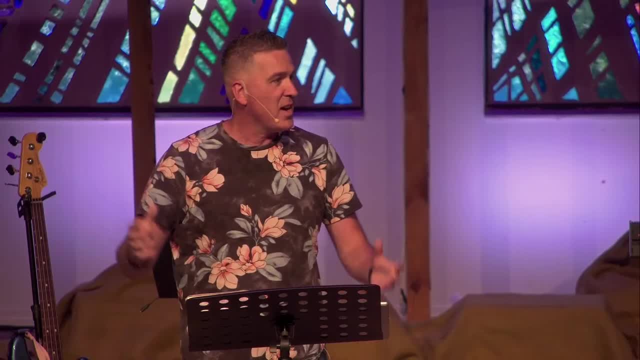 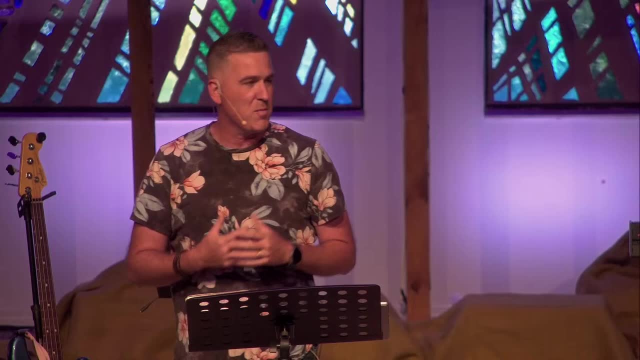 on the brink of falling apart And God brings them back together from what seems like the end And they have an appreciation for their marriage and love like no other. I see God take people who are who hurt, have it and hang up addicts. 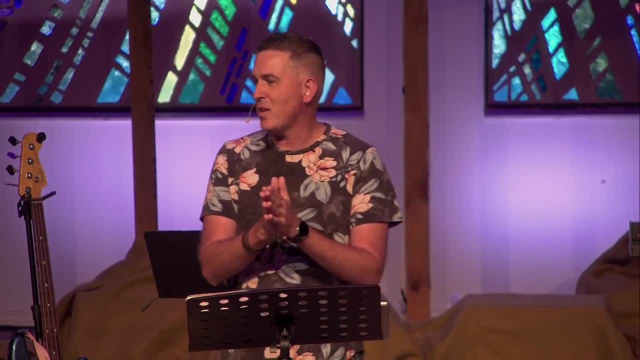 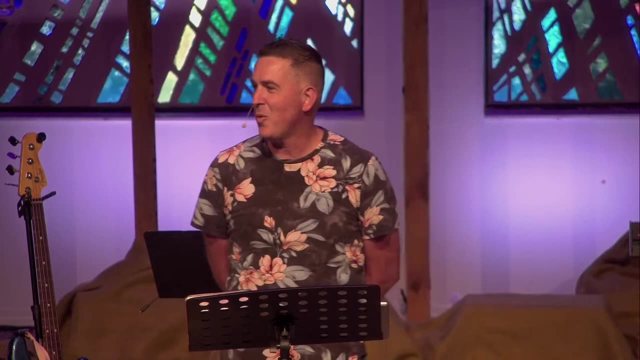 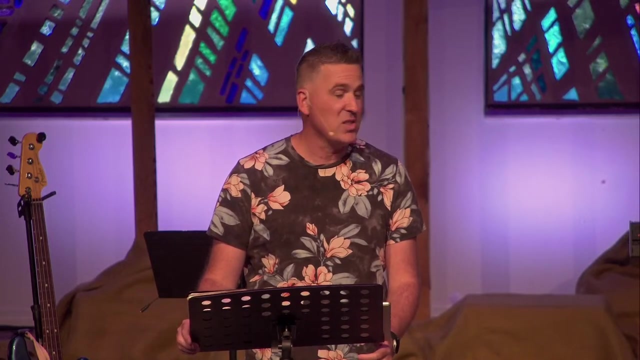 And God helps them find grace and freedom. And they are the people who wanna share God's love, unlike anybody else. So what will God's do, what will God's word do in your life? And the answer is: it's living. So it depends on what you need. 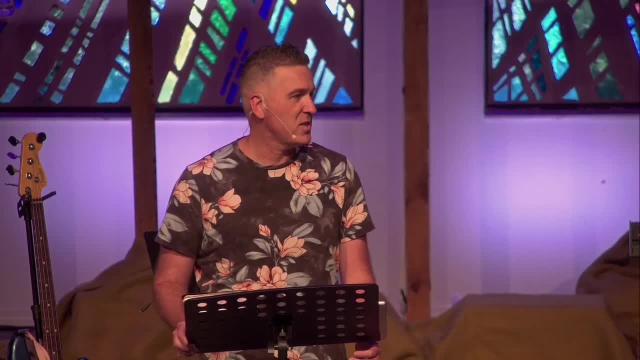 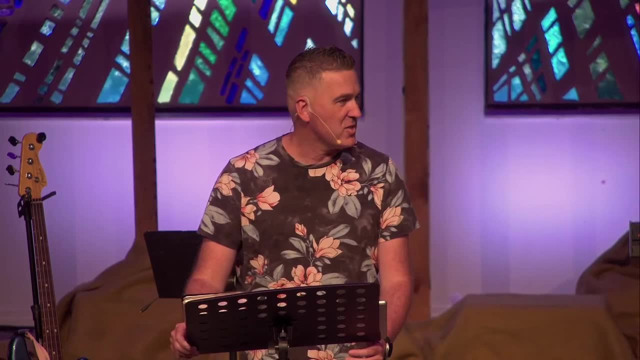 If you're hurting, it can bring you hope. If you're lost, it can give you direction. If you're doubting, it can build your faith. If you're anxious, it says: cast your anxiety and cares upon the Lord and he will bring you peace. 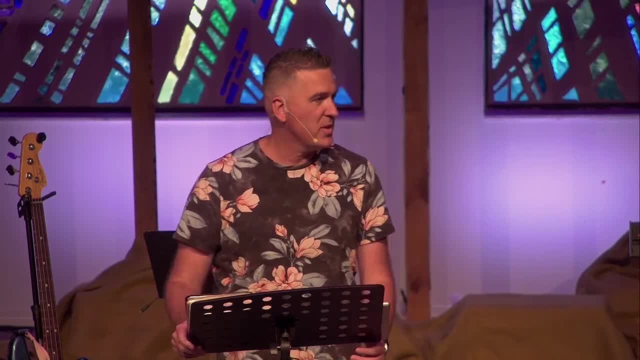 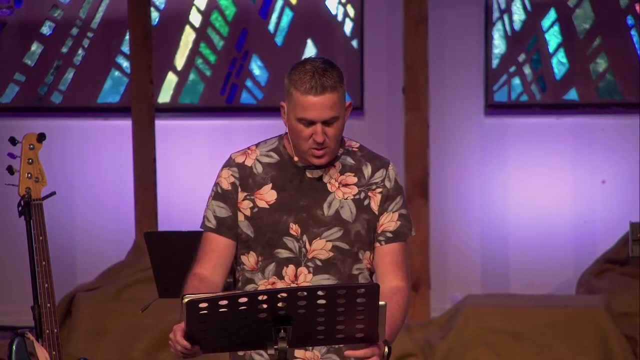 If you're trapped in a life that you never wanted, the truth can set you free. Would you pray with me, God? we're so thankful that we can hear your word, that your word can speak to us, that your word can transform us. 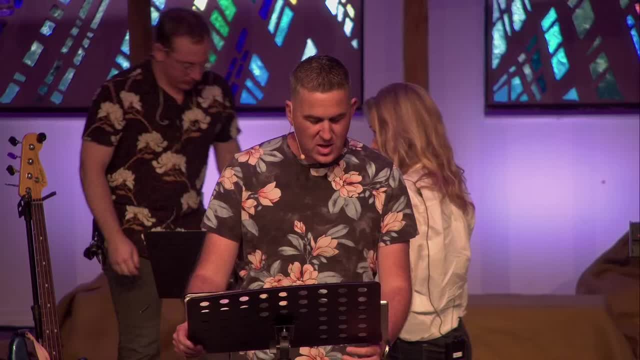 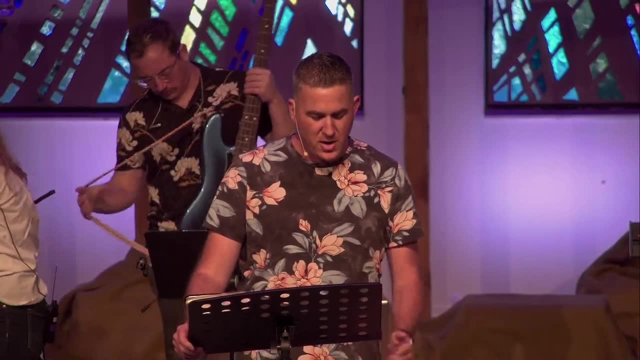 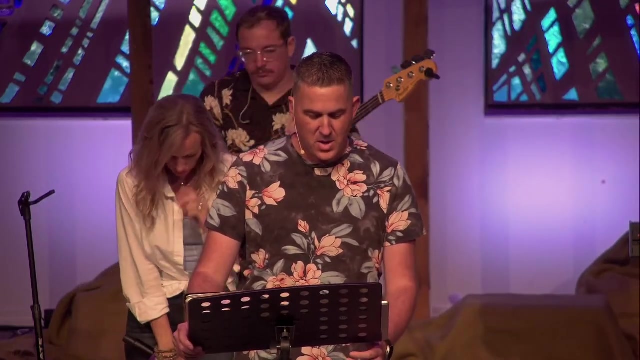 God. I'm so thankful that Solomon and all of his wisdom, after looking at all the things under the sun, he said: this is my conclusion: Fear God and keep his commandments, for this is the whole duty of man. Lord, I pray that we become people. 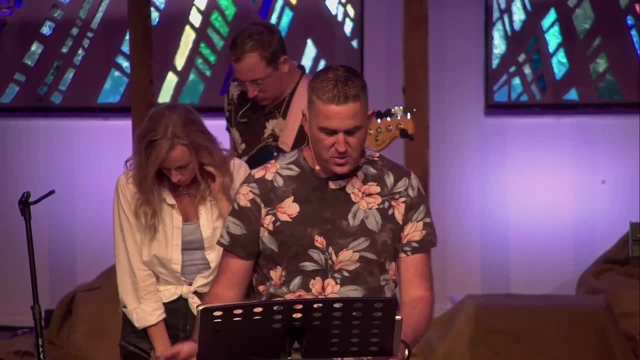 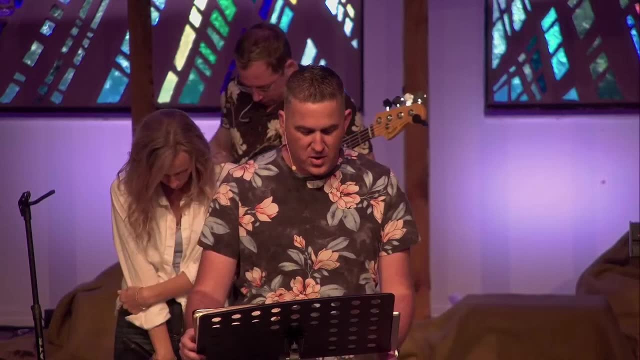 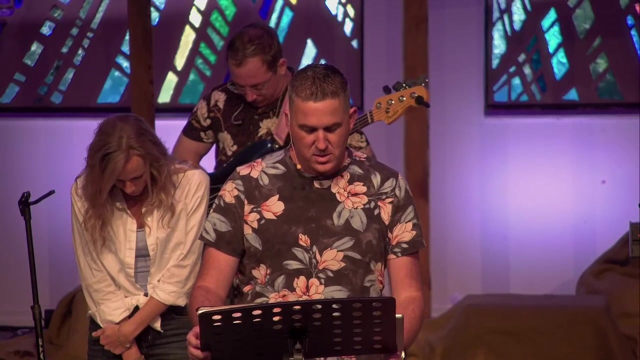 so that we can be a church that fears you and keeps your commandments. So, Father, I pray that your word would be a part of our daily conversations. Lord, I pray that everyone who has heard these messages would make a commitment for the time, the place, the plan. 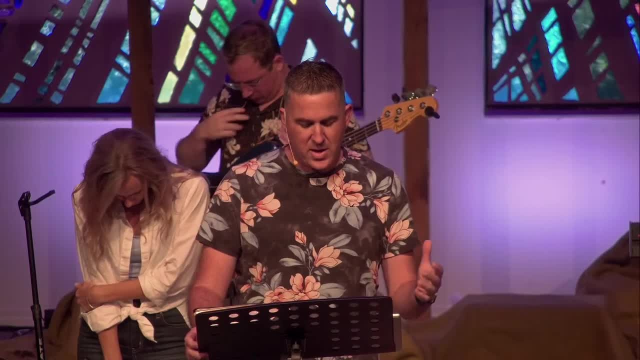 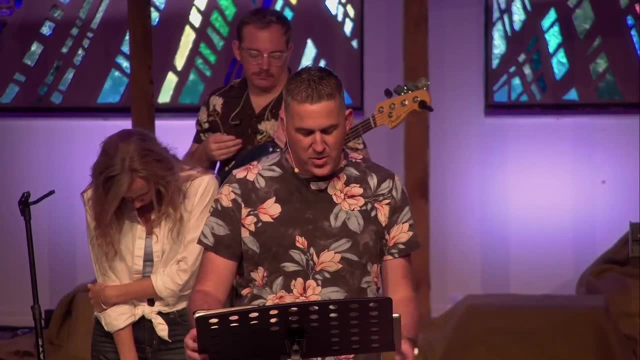 that they're gonna use, so that they can come before you each and every day, That some will gather in small groups, some will gather with their family at the table, some are gonna have a journal that they spend time with each and every day. 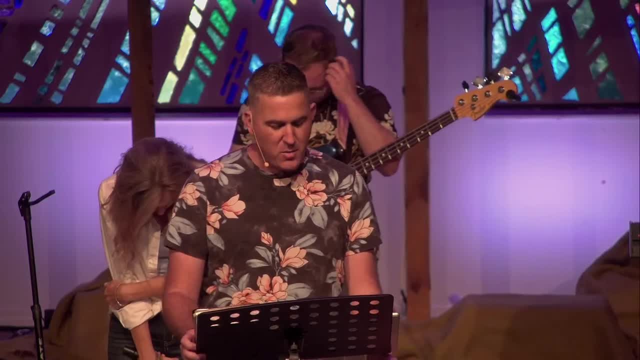 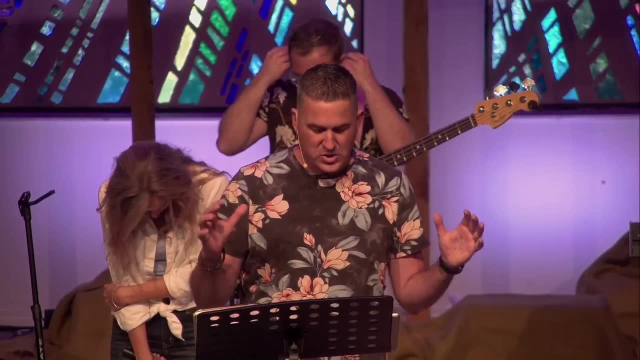 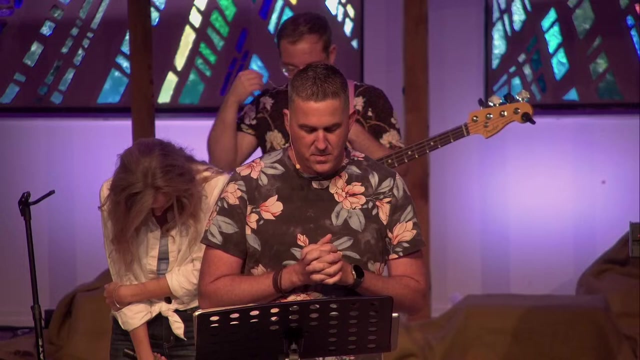 just with you, God. I thank you that tomorrow that we can see not just a Sunday morning gathering but we can see hundreds of people responding by spending time with God Jesus, I'm thankful that you will meet them there. I thank you in advance. 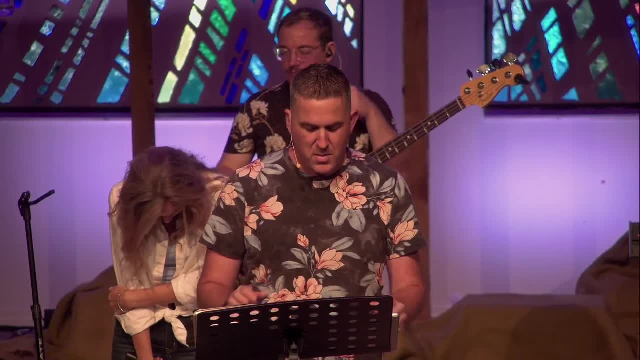 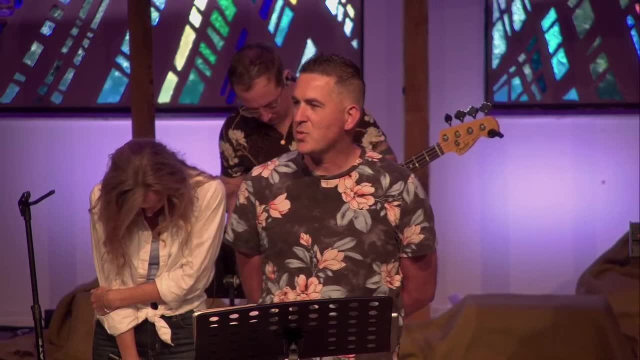 for the way that you're gonna speak to them and they commit to meet with you And church. we said there's two things that live forever: God's word and our soul. The Bible says you'll live forever in the presence of God. 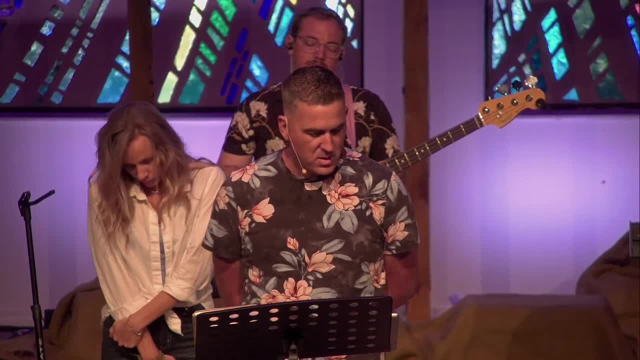 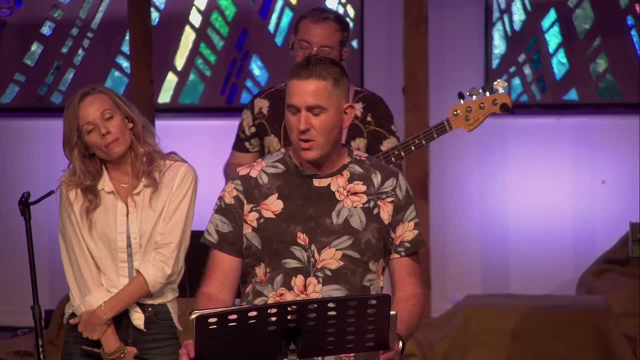 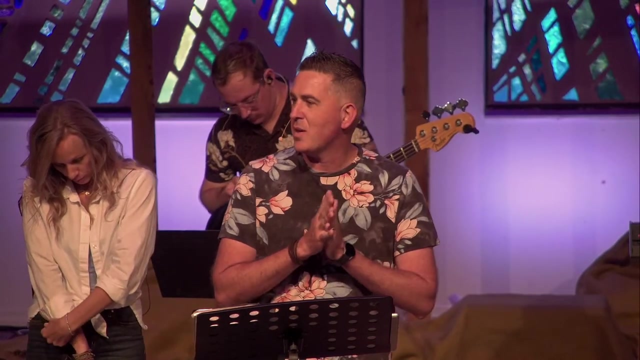 but we will live forever separated from God. That two things will live on: God's truth and our soul. We're reminded that in the beginning was the word, and the word was God, and the word became flesh. What does that mean? It means that God sent his son. 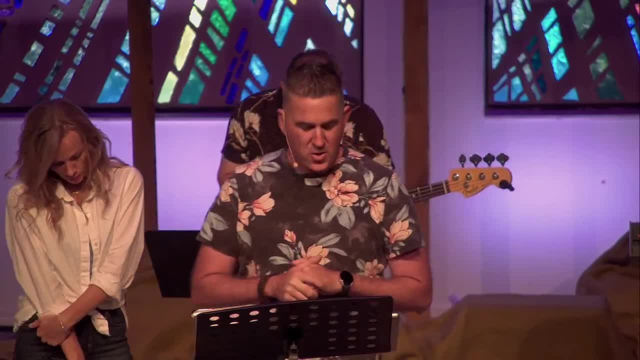 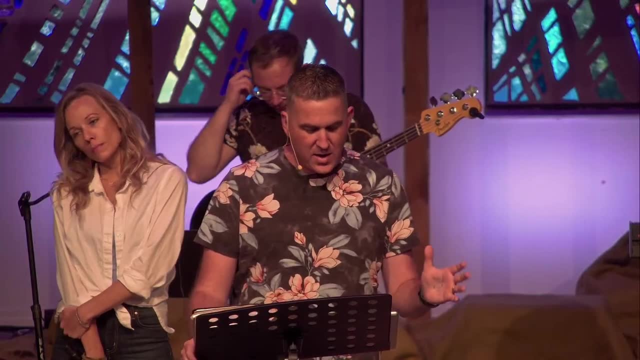 the person of Jesus, That Jesus, the son of God, who lived without us, could be forgiven. And that's why we hear in the gospel of John: for God so loved the world that he gave his only son, that whoever believes in him. 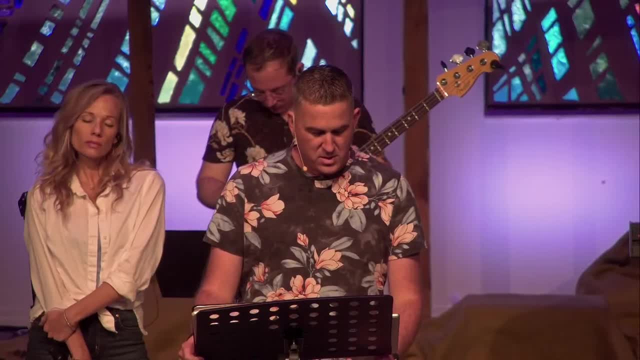 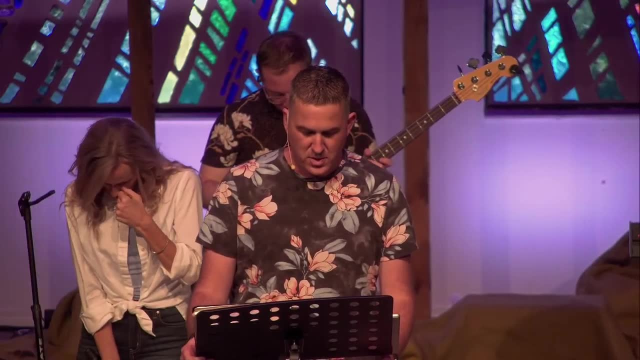 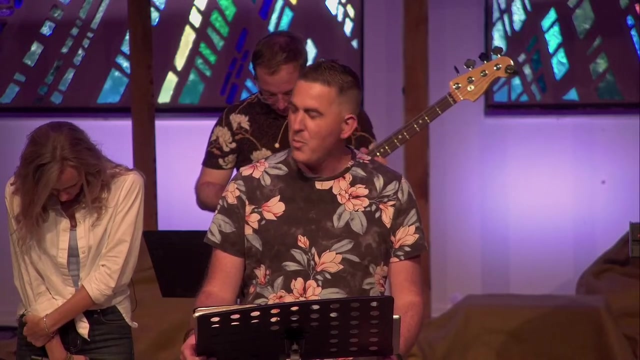 shall not perish but have everlasting life. So if right now you feel like you're far from God, know that forgiveness exists for you. Scripture says that Jesus will forgive your sins and they will be separated from you. You don't become better, you become new. 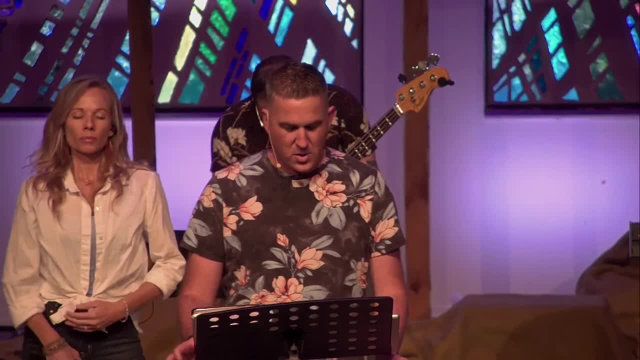 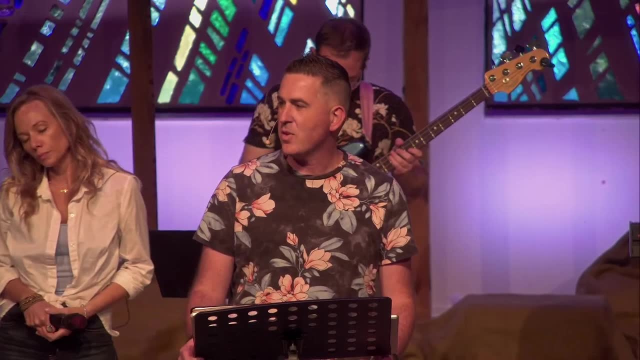 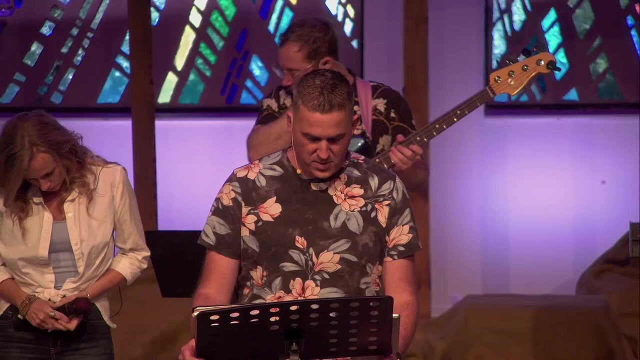 The old is gone, the new has come. So, wherever you are right now, just cry out to Jesus and say: Jesus, I need you, Jesus, I believe in you. Jesus, I surrender to you and I call upon you. Give me the strength to be in your word each and every day. 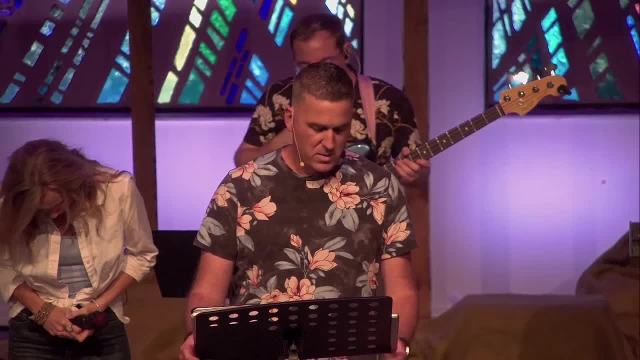 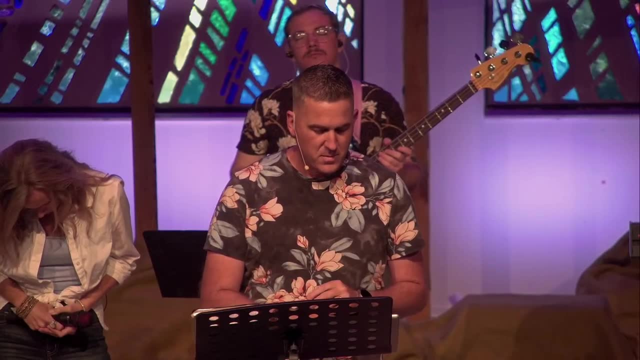 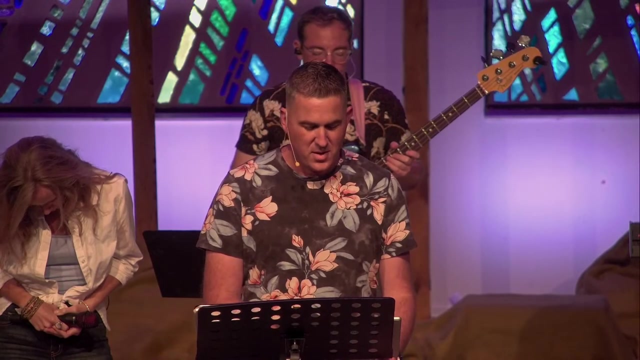 as we pray together. Heavenly Father, forgive me of my sins. Jesus, save me. Be first in my life. Be my Lord And fill me with your love, And fill me with your Holy Spirit So I can know you, So I can know your word. 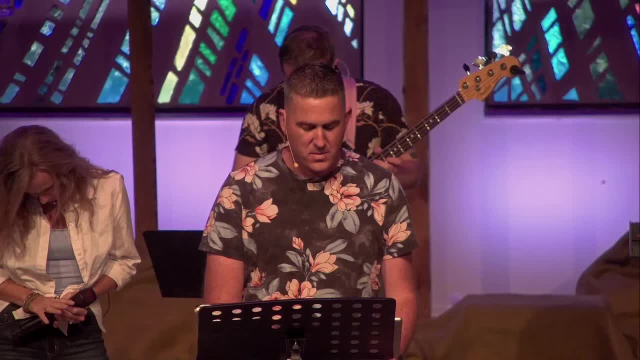 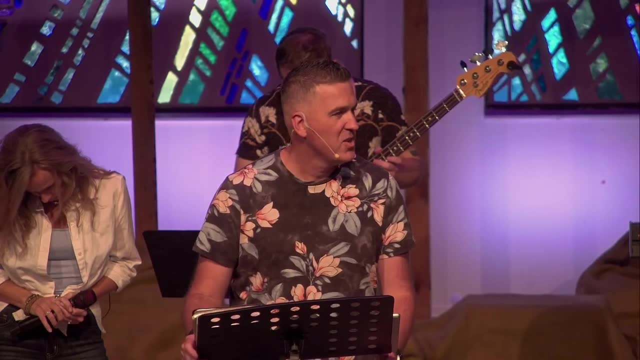 So I can live with you and within your will. forever Use me, God, to show others your forgiveness, as I've been forgiven Just as we stand and we close in worship. if we can be praying with you this morning, we'll be up here to pray with you. 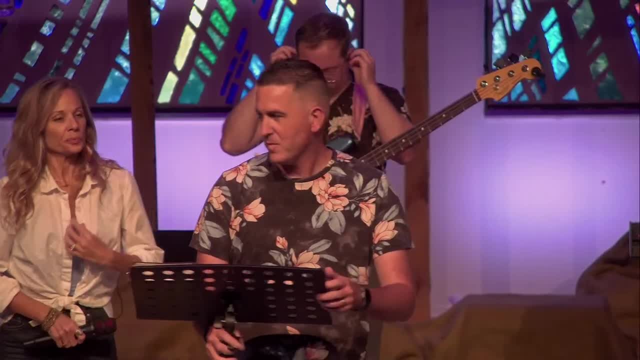 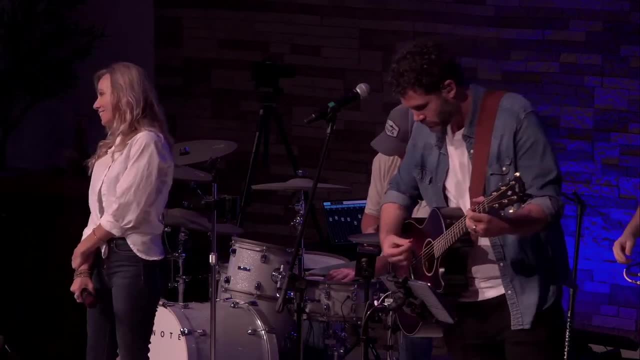 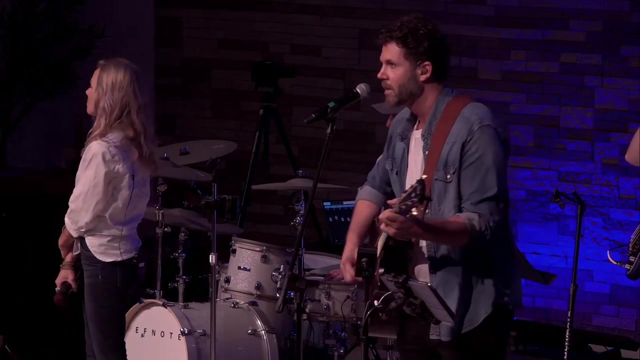 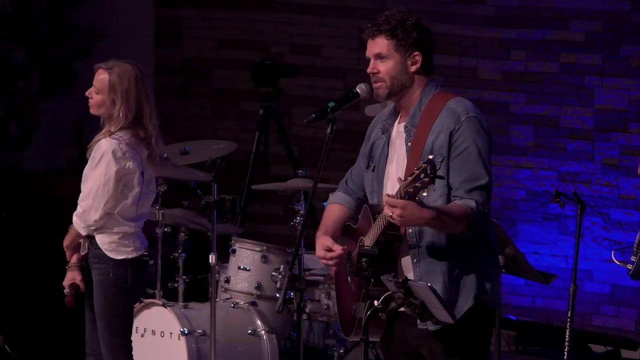 But let's stand and let's close in worship together, As we sing this last song together, let us make room for the Lord in our hearts and our minds and watch what he can do, Because he can do anything with the smallest things. So let's just give him our voices. 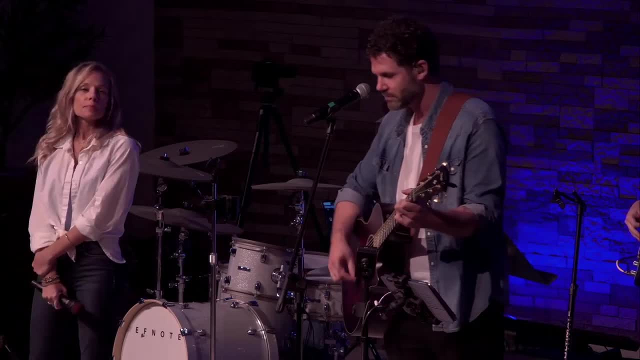 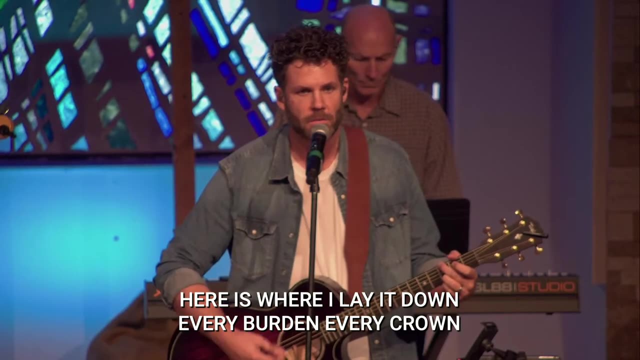 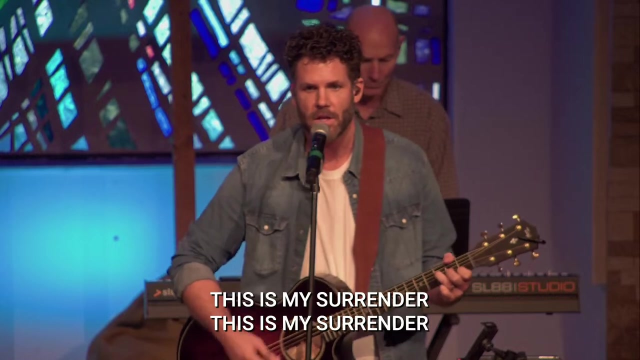 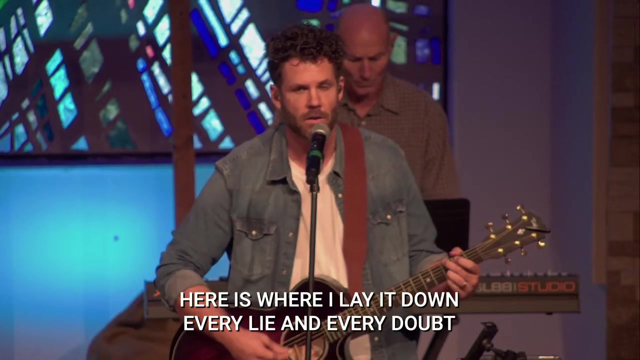 give him our hearts as we sing this final song together. Let's do it. Here is where I lay it down. Every burden, every crown: This is my surrender. This is my surrender. Here is where I lay it down. Every lie and every doubt: This is my surrender. 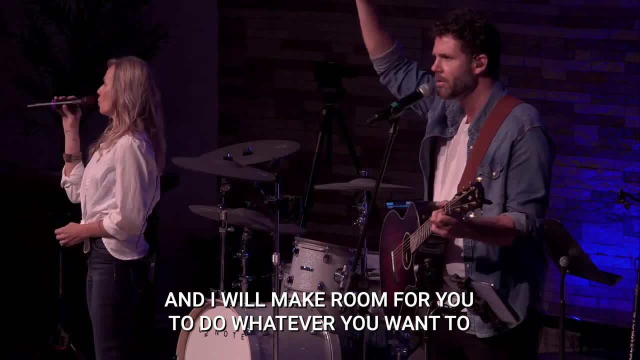 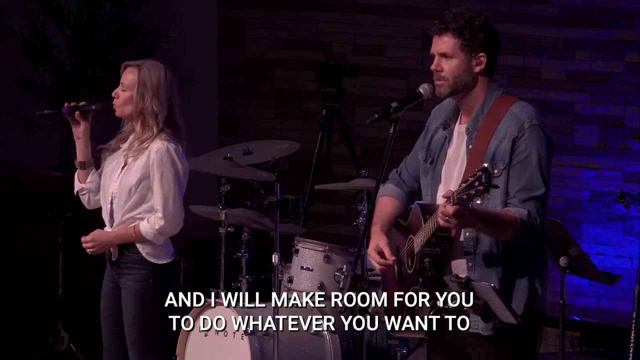 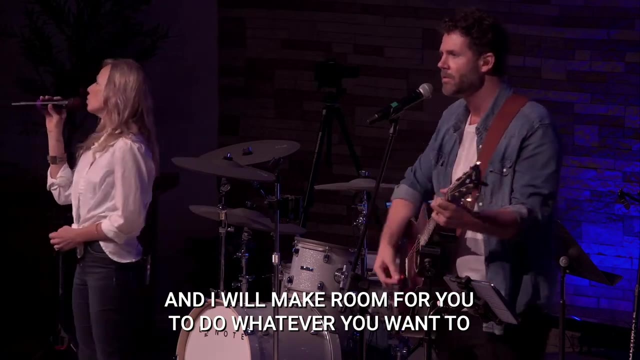 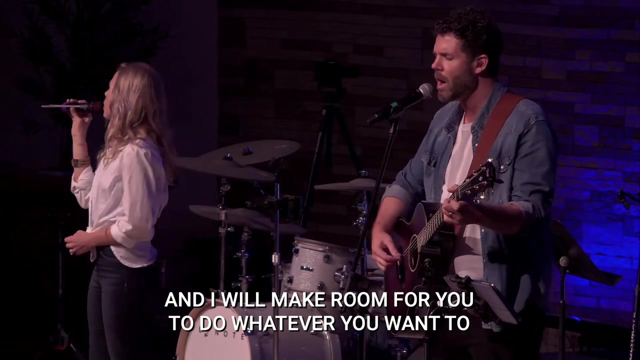 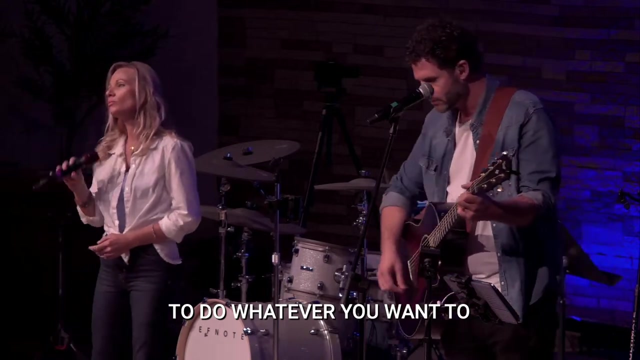 And I will make. I will make room for you To do whatever you want to. To do whatever you want to. I will make room for you To do whatever you want to. To do whatever you want to, I will make room for you. Here is where I lay it down. 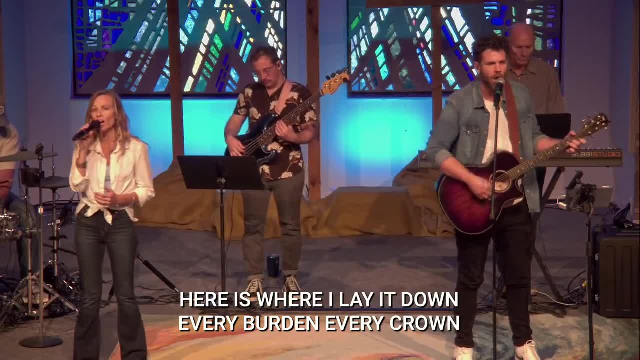 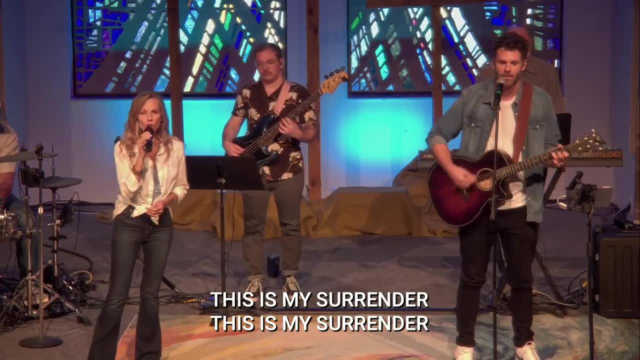 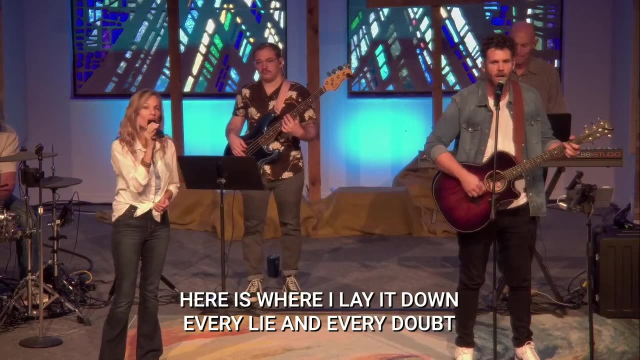 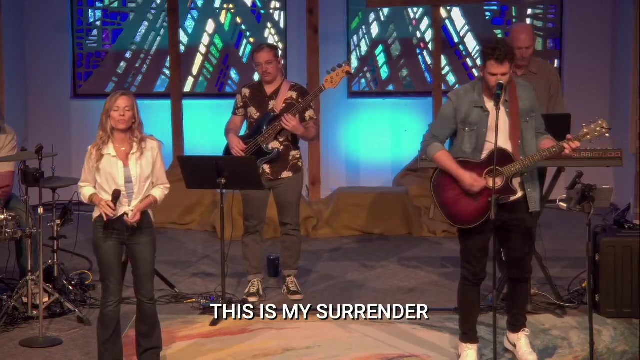 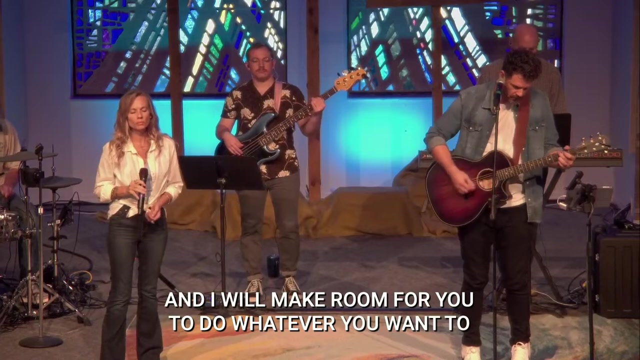 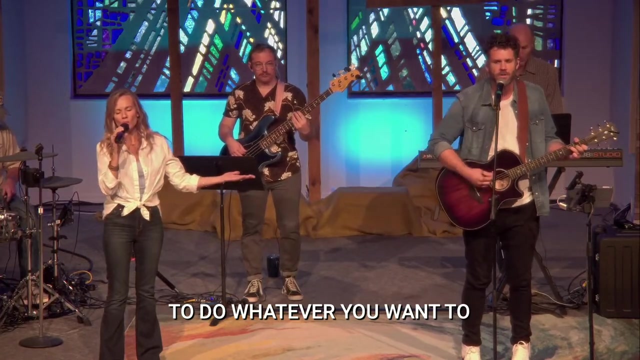 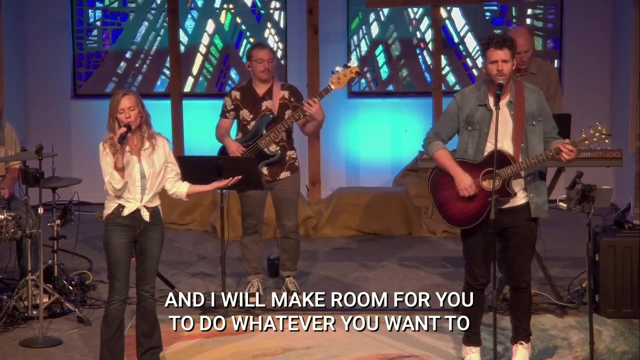 Every burden, every crown. This is my surrender. This is my surrender. Here is where I lay it down. Every lie and every doubt, This is my surrender, And I will make room for you To do whatever you want to. To do whatever you want to, And I will make room for you. 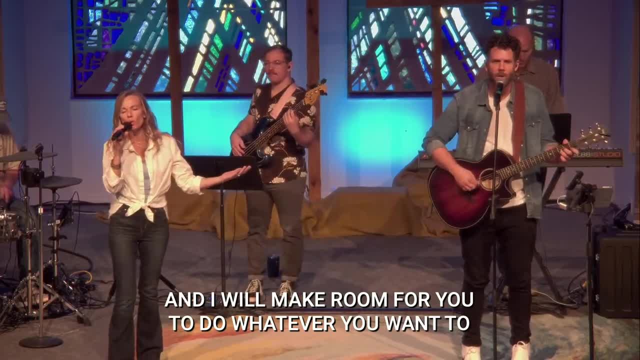 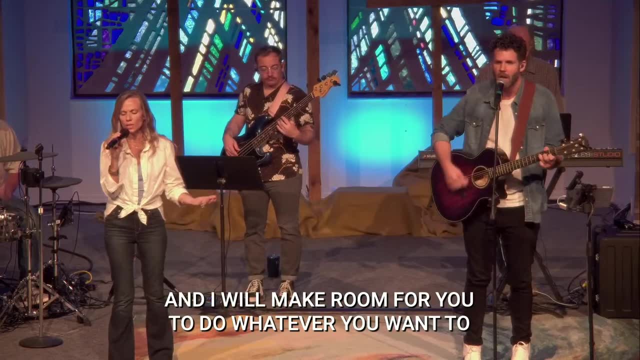 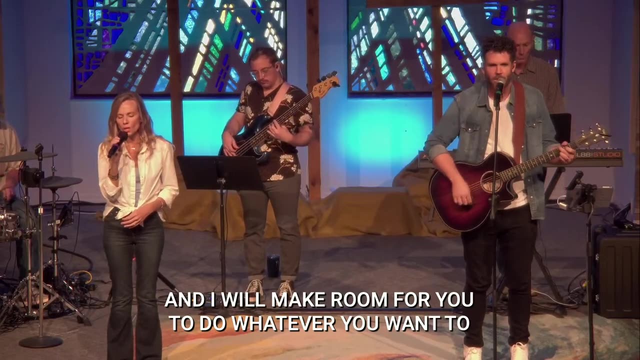 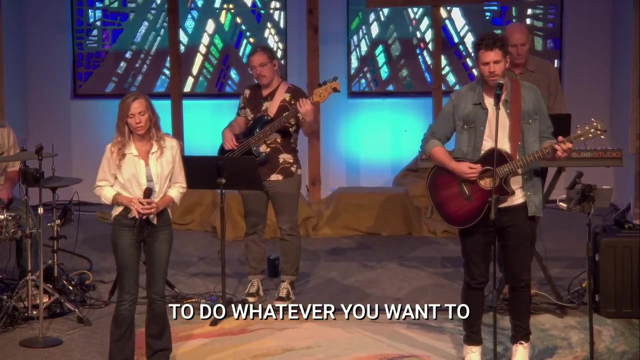 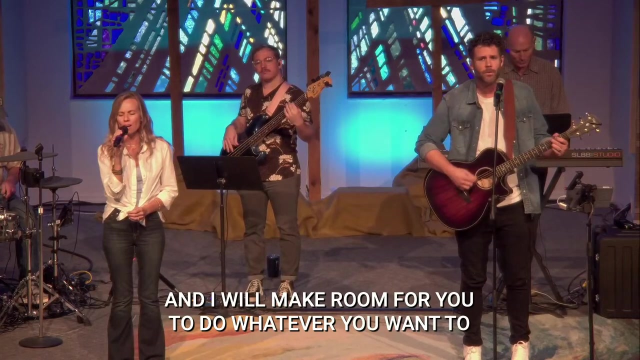 To do whatever you want to. To do whatever you want to. To do whatever you want to, Do whatever you want to. I will make room, And I will make room for you To do whatever you want to, And I will make room for you To do whatever you want to. 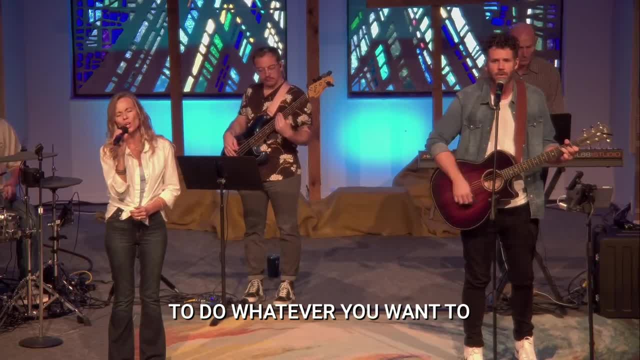 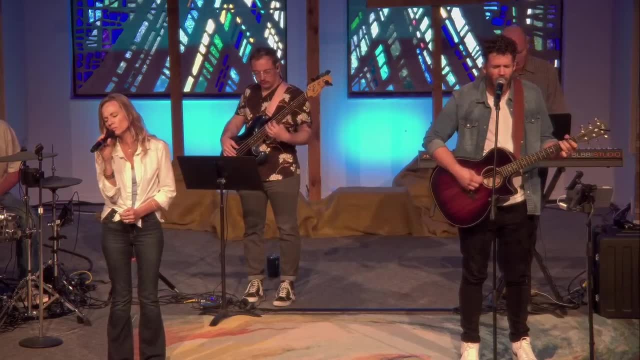 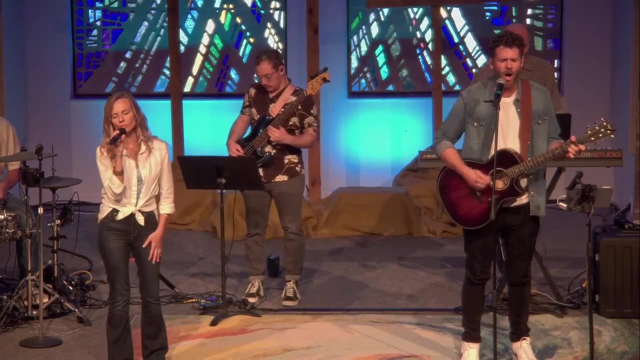 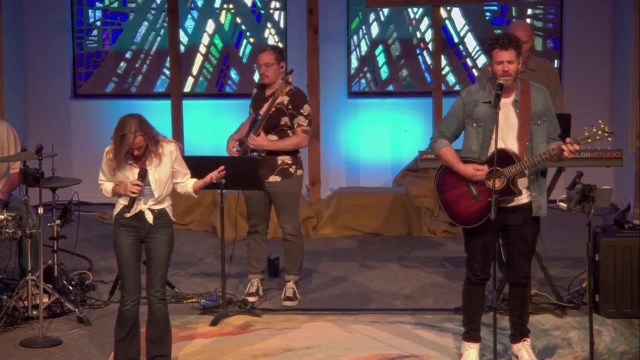 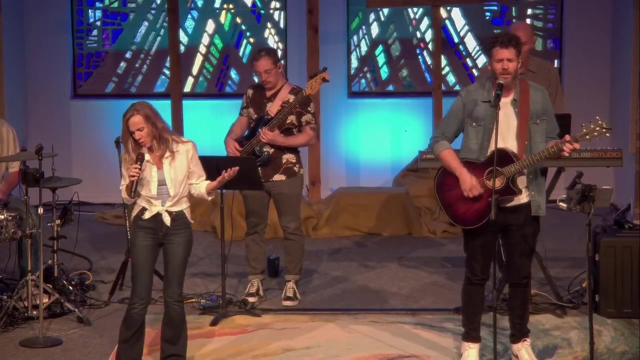 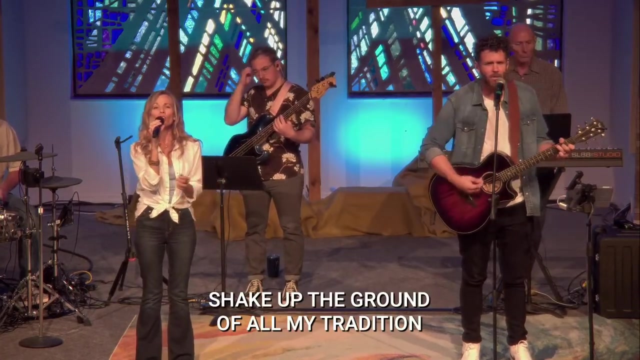 To do whatever you want to. Oh, pour it out. pour it out. Oh, show us the glory. Show us the glory. Open up our hearts. we open up our minds. Fill us with your Spirit, God. Fill us with your Spirit. God, Shake up the ground for my tradition. 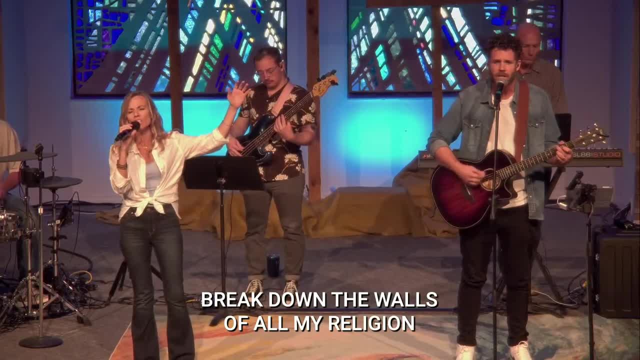 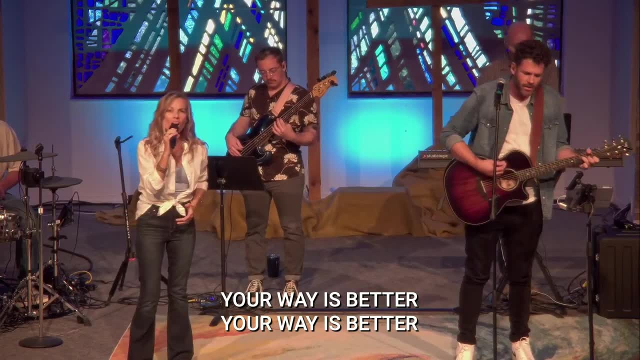 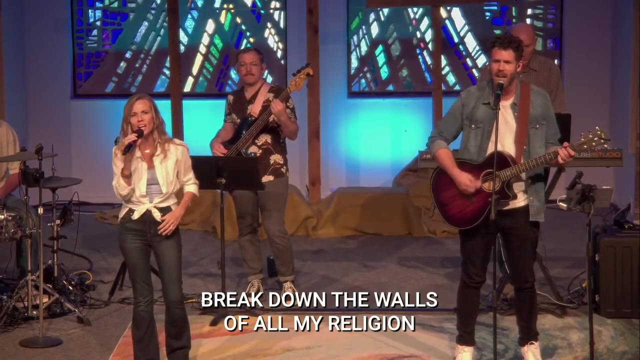 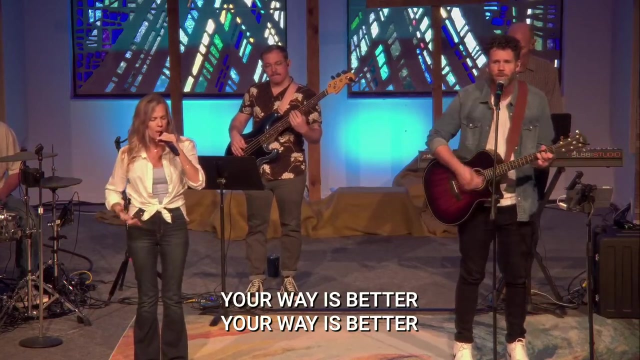 Break down the walls for my religion. Your way is better, Oh, your way is better. Shake up the ground. Shake up the ground for my tradition. Break down the walls for my religion. Your way is better. Here we go Your way. your way is better. Shake up the ground for my tradition. 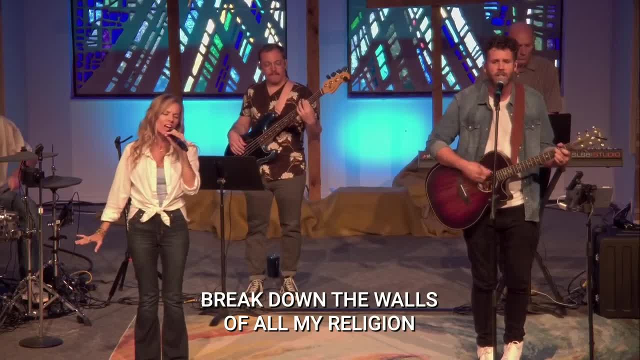 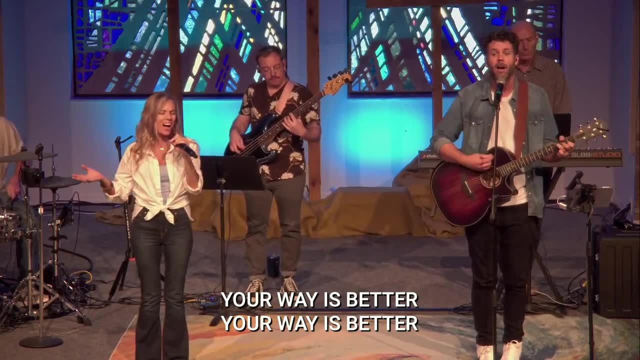 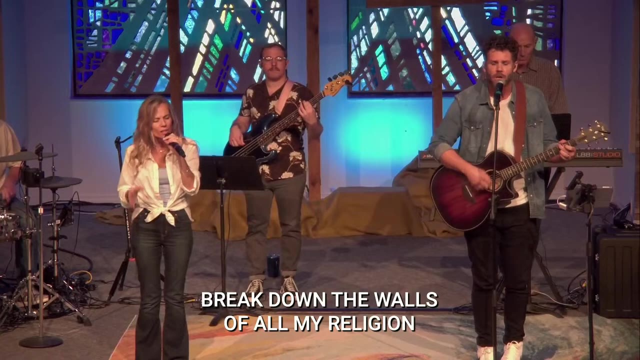 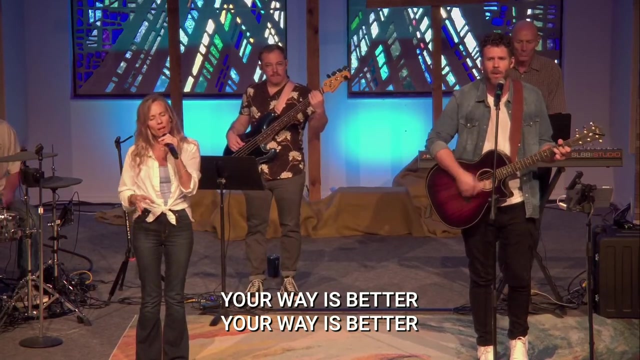 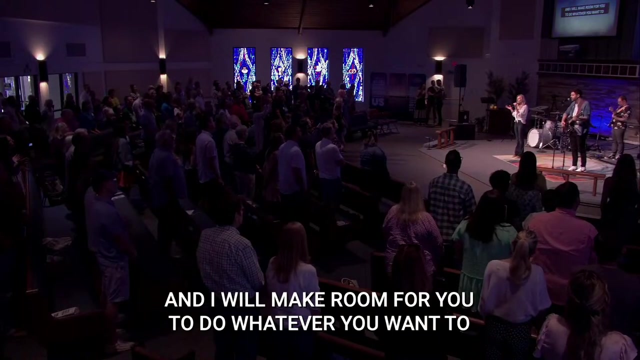 Break down the walls for my religion. Your way is better. Your way, your way is better. I will make a room for you And for my vision. I will spread that out. I will spread that out. I will show our love, I will show our power To do whatever you want to. 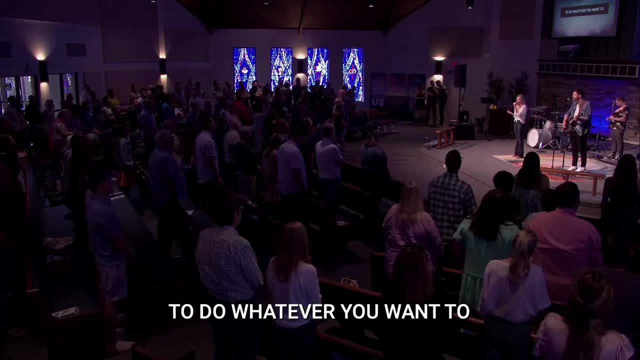 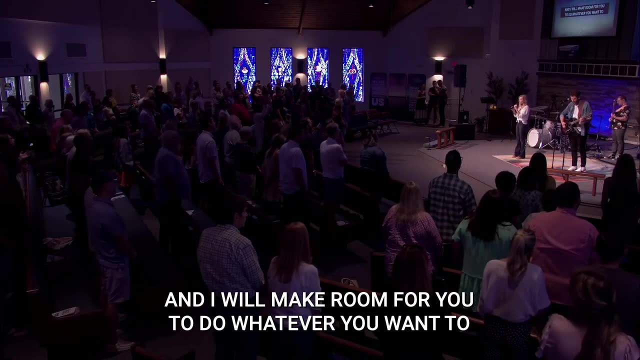 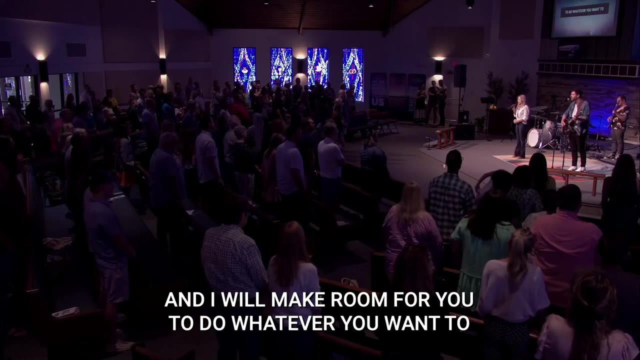 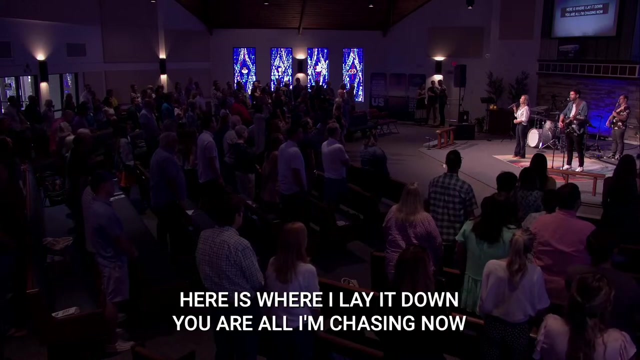 To do whatever you want to, And I will make a room for you To do whatever you want to, And I will make a room for you To do whatever you want to. Come, do whatever you want to. Here is where I lay it down. You are all I'm chasing now. 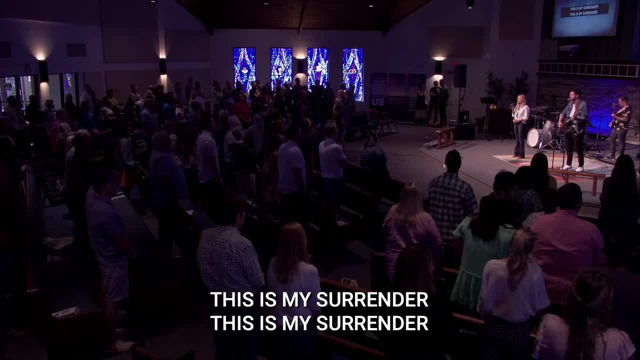 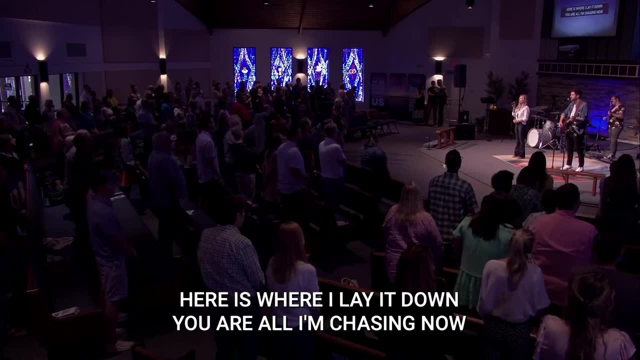 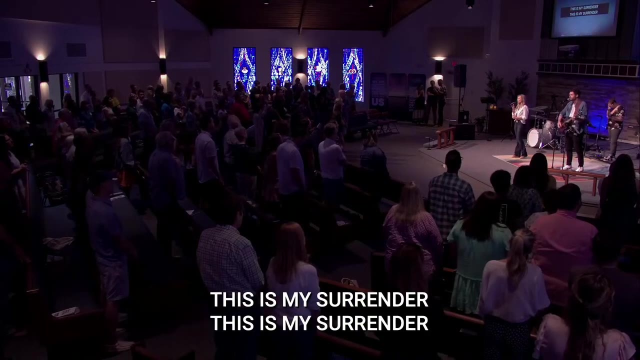 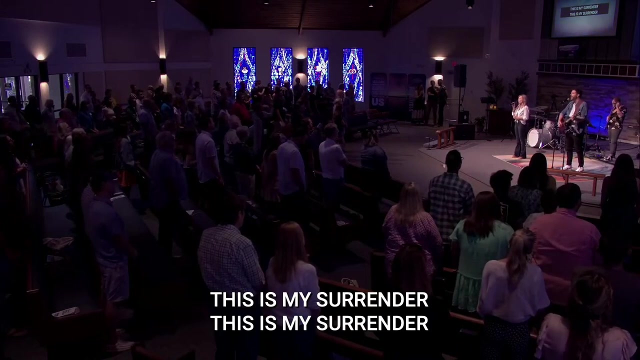 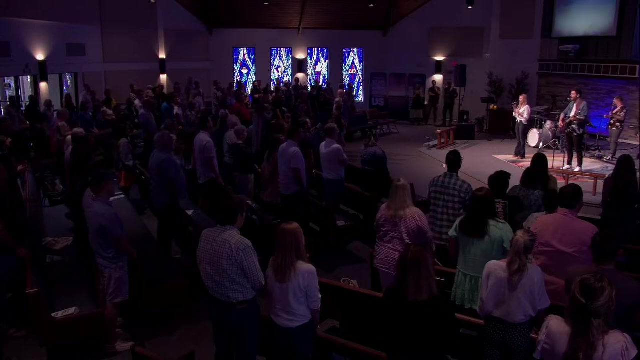 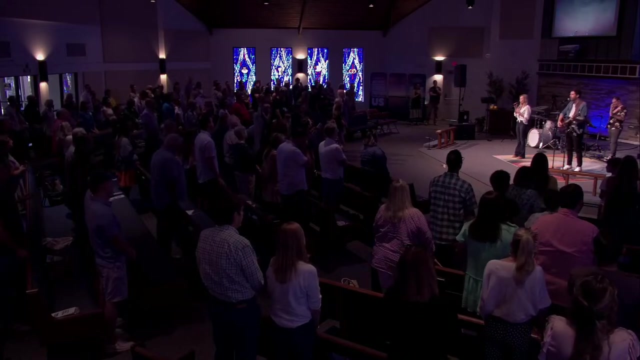 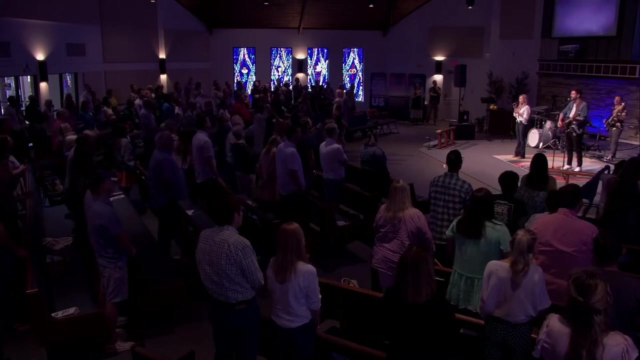 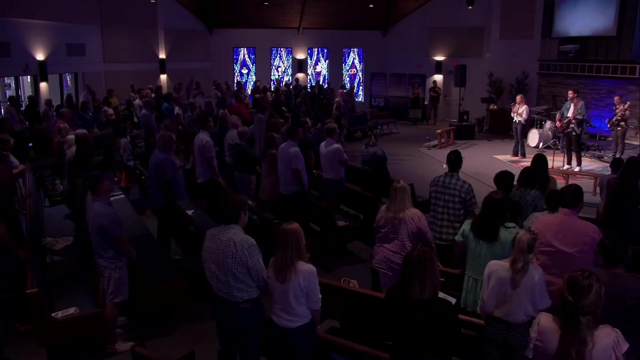 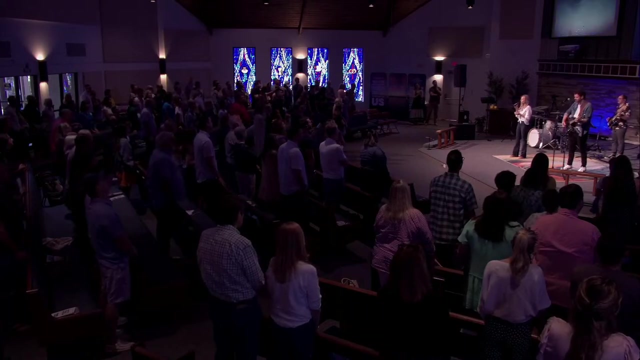 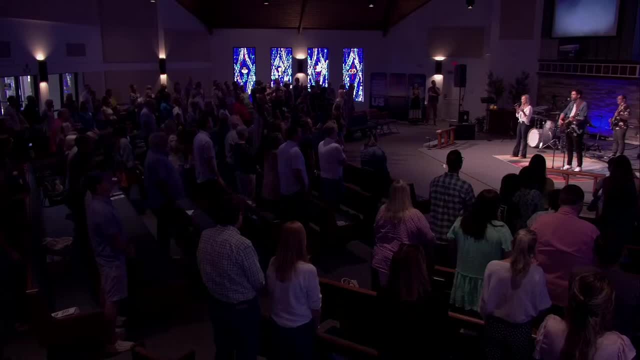 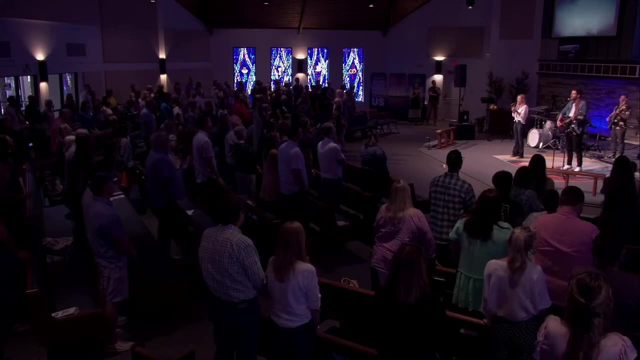 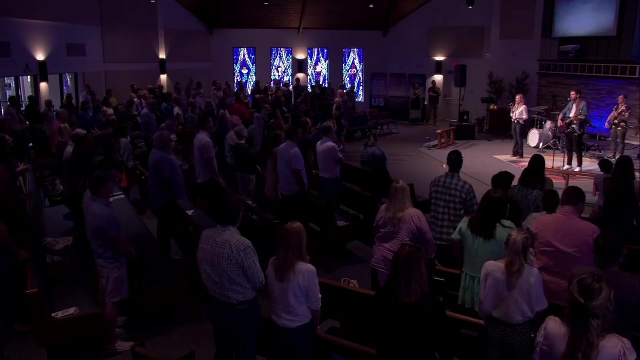 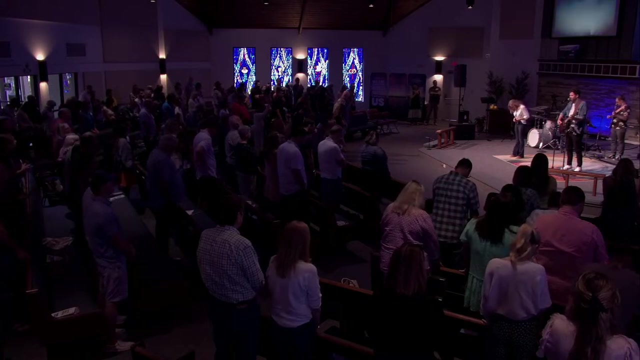 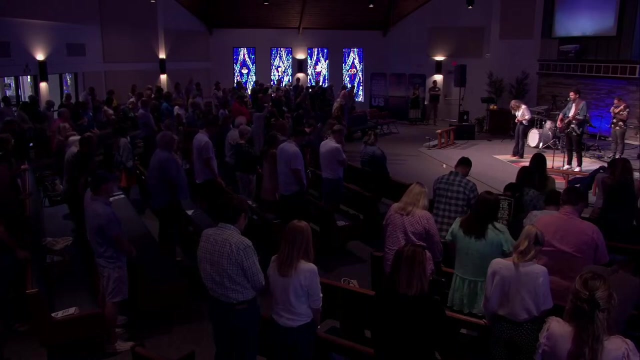 I surrender all, All to Thee, My blessed Savior. I surrender all, Jesus. let that be true as we We think about all the things you've done for us, God, And all you ask of us is just to be with you, God. So, as we leave this place today, 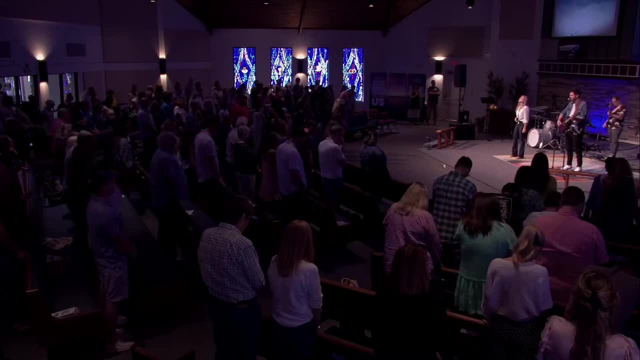 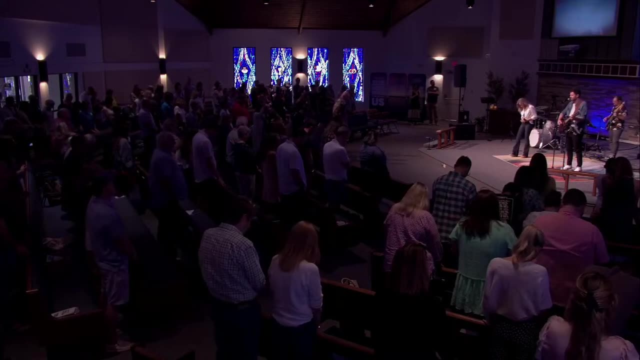 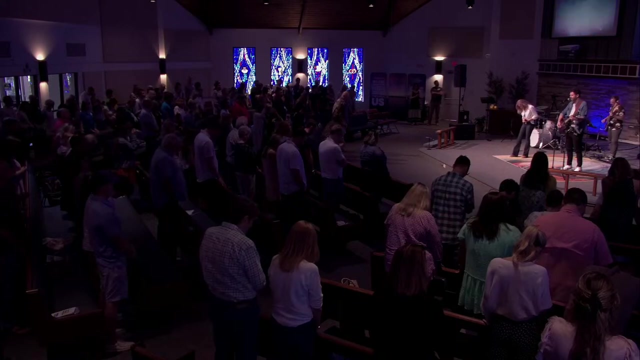 Let that surrender be in our lips As we surrender our time. We surrender our commitment to you, So that we can go deeper with your word And go further, Because you have so much left to show us, God. We can never get enough of you, God, But let us take this challenge. 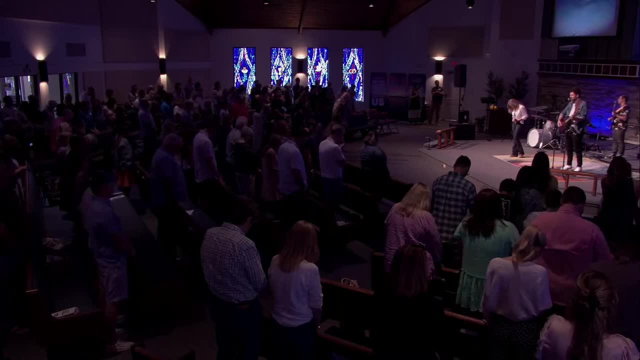 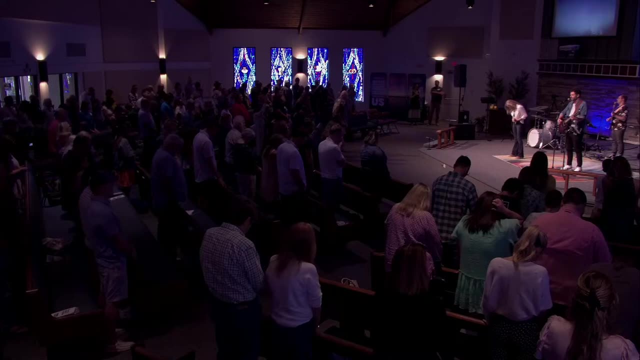 Just to go deeper, To learn you better, And then we'll see how much our lives can improve. Even if we don't get enough of you, God, Even if we have the best life ever, A life fuller of you is better still. So let us take you up on that amazing challenge, God.